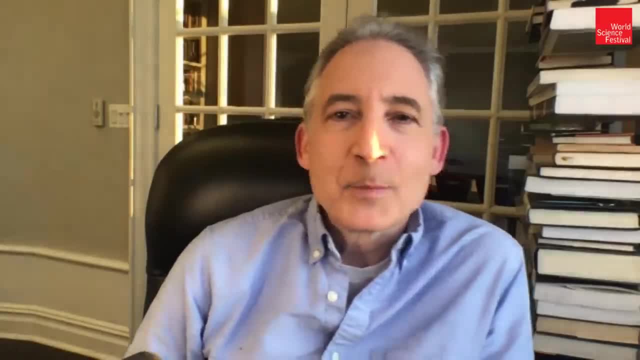 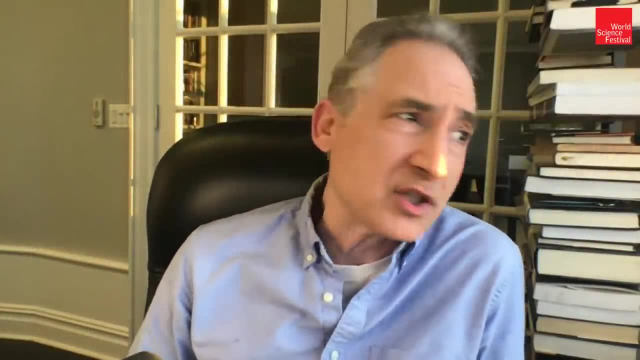 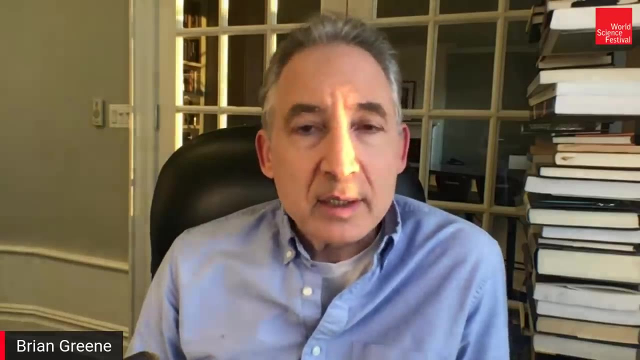 Hey, everyone, Welcome. It's been a long time since we did one of these sessions. Thanks for joining us here. You may know this is a special week for us at World Science Festival. We're in the midst of our Australian version of the World Science Festival, World Science. 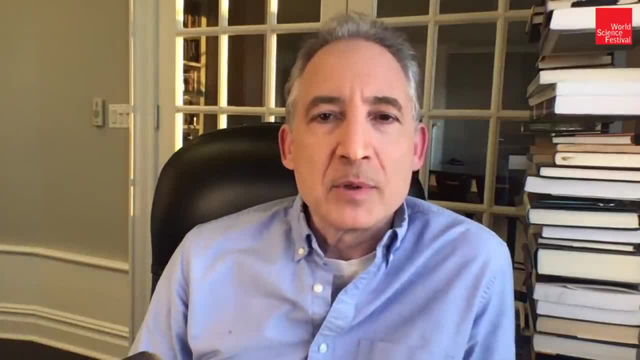 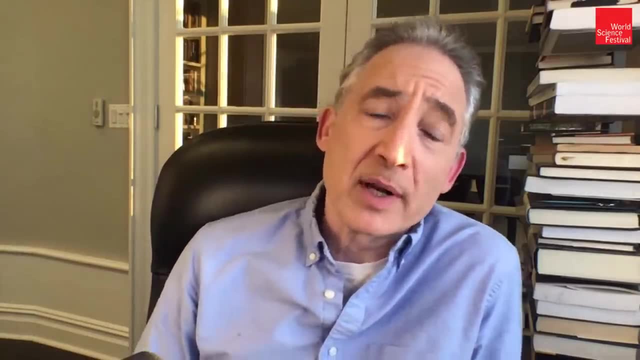 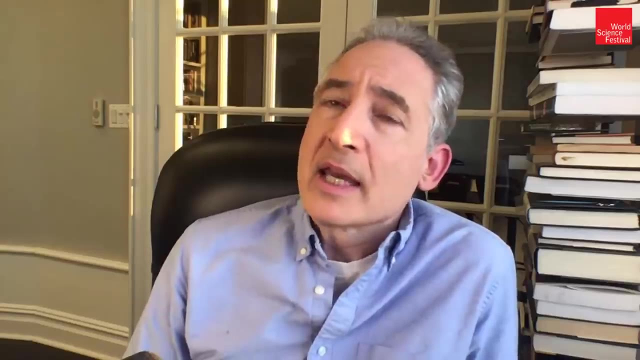 Festival, Brisbane. So welcome to all of you folks from down under. Thanks for joining us here for this conversation with Brian Schmidt, who, of course, is in Australia, And we're going to talk about his work in understanding the accelerated nature of the expansion of space. 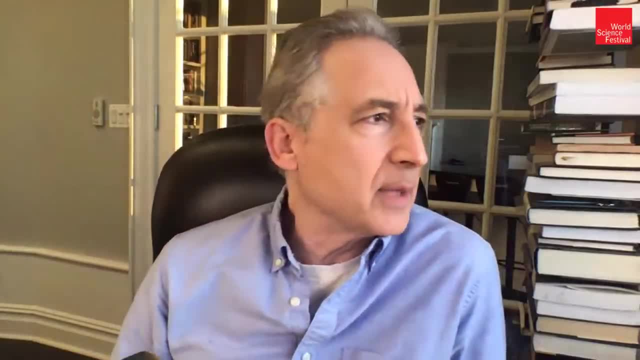 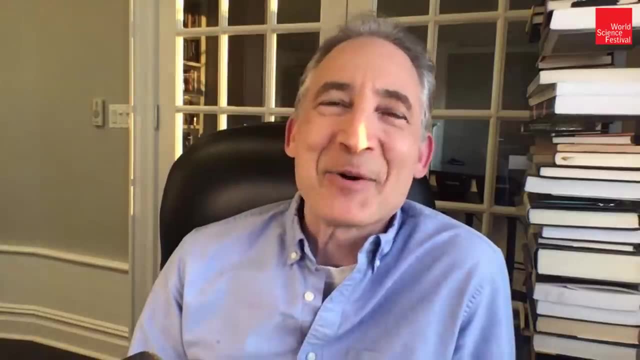 the future of the cosmos. I think it's set on the still image: the role of science in shaping the future. Yeah, we'll talk a little bit about that, but that makes it sound almost like a policy talk. That's not what we're doing. We're talking about science with perhaps 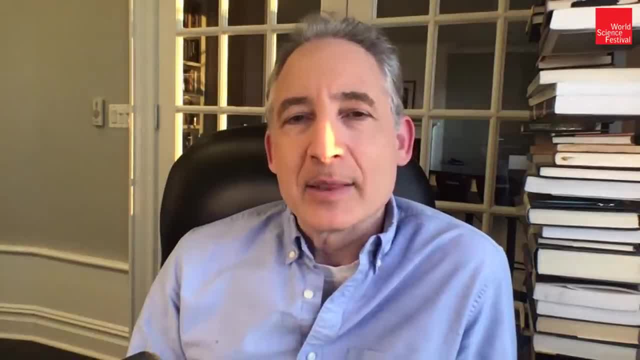 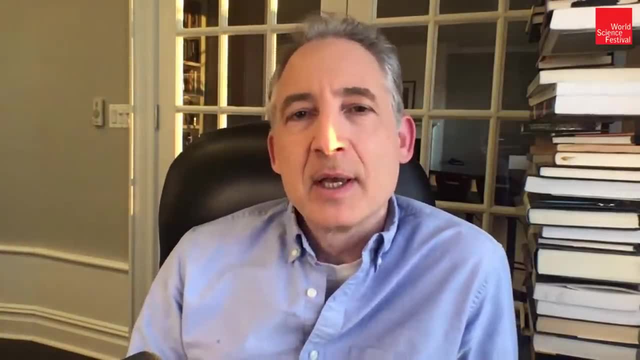 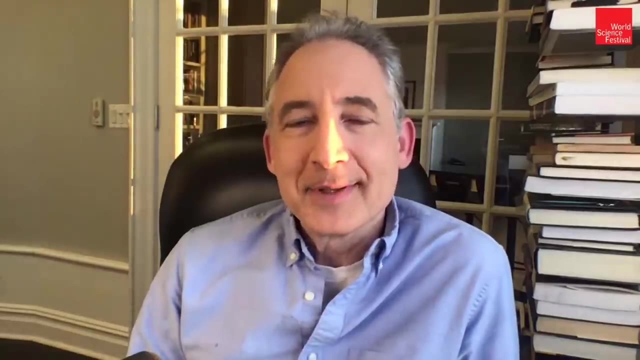 a little bit of a policy mixed in There. at the end you may notice that my background is a little bit different Those of you who are familiar with these conversations from the past. for the last year, we have been in upstate New York, hiding out, if you will, from the scourge that has been ravaging. 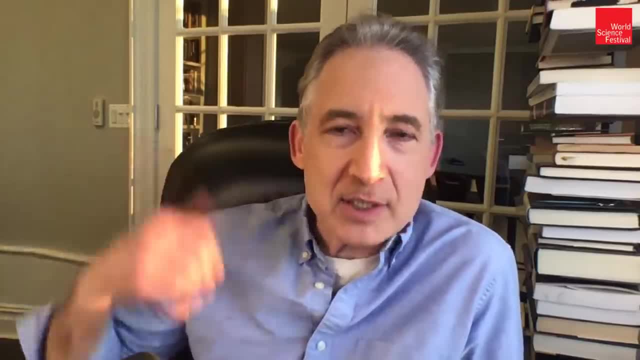 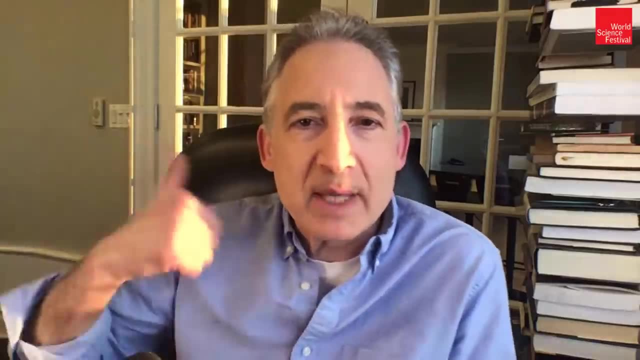 the world. We are back now in New York City, So actually this is my home in Manhattan, not far from the campus of Columbia University. So on occasion you actually may see my kids walk by behind me. Maybe they'll even pop in their head to ask me: you know what are we having? 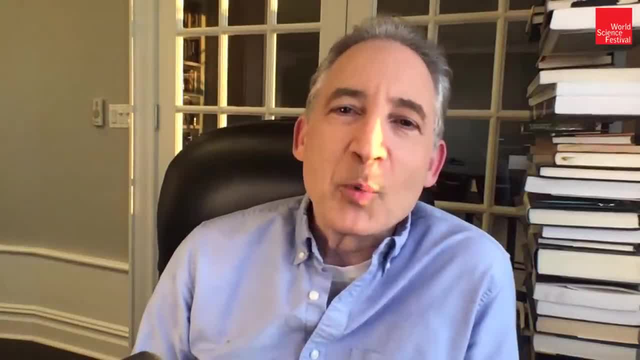 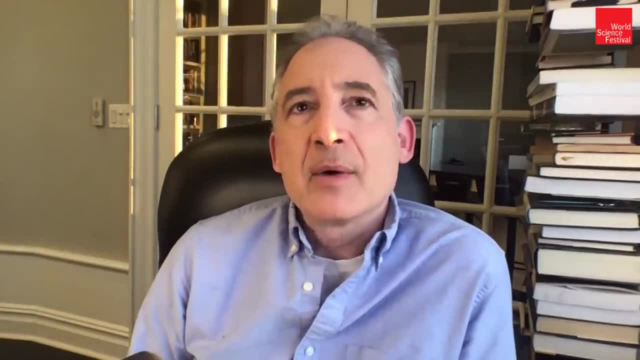 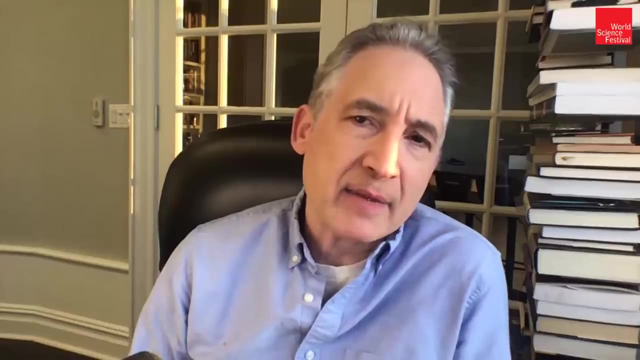 for dinner or something like that, But we will just roll with whatever happens. So before we begin, I'll bring Brian Schmidt in in just a few minutes. I always like to have a little discussion about some news things that have been happening in physics, And it's been kind. 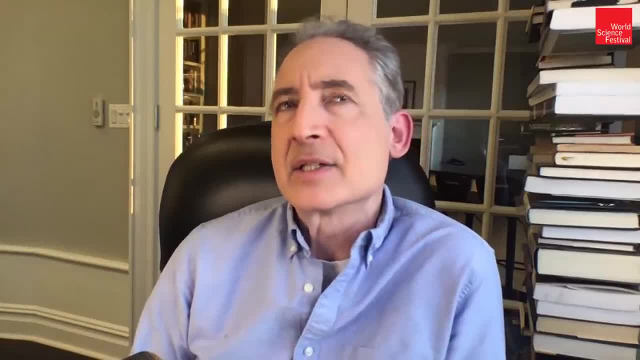 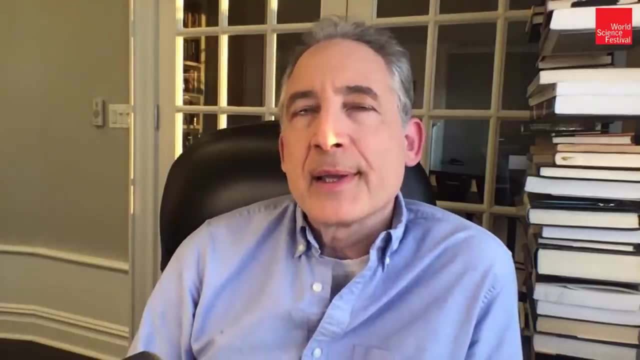 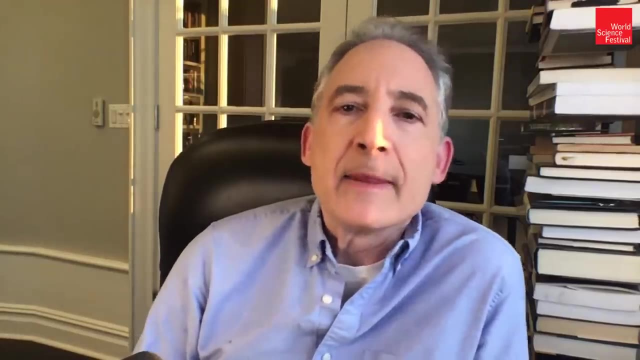 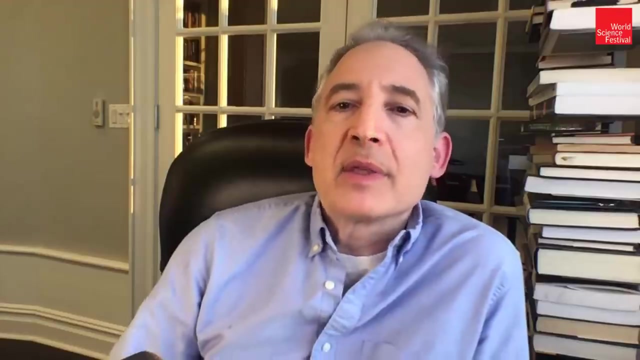 of an interesting couple of weeks for those of you who've been following these ideas. There is data- tentative data for sure- of CERN regarding some decay products of a cork known as the B cork or the beauty cork or the bottom cork, however you want to call it, where the decay products are not quite 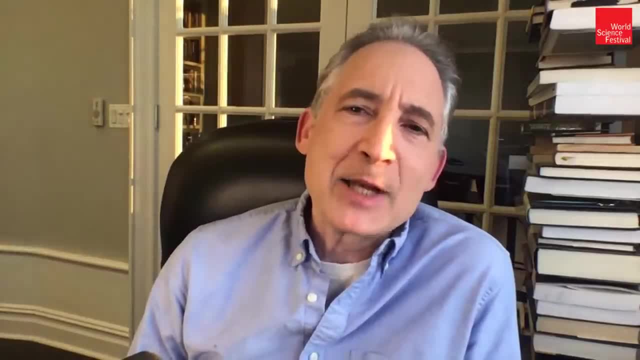 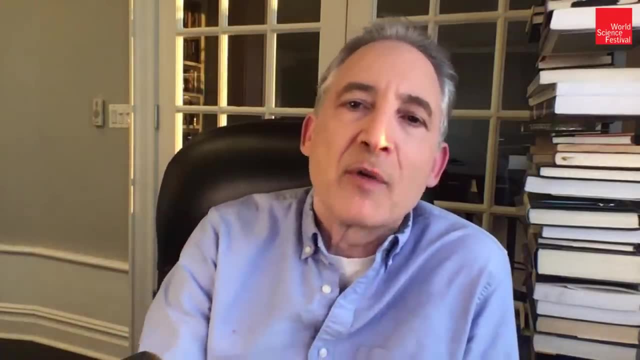 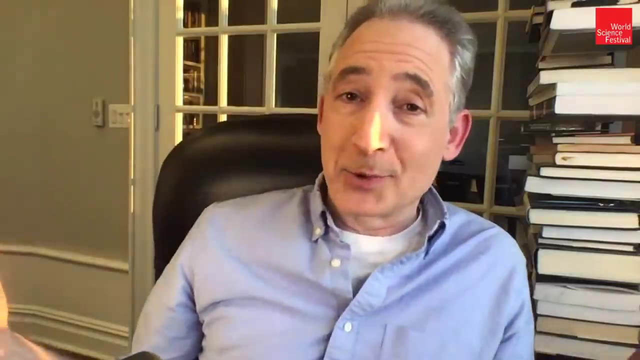 in line with what we would expect from the standard model of particle physics. Standard model of particle physics, as many of you know, is the fundamental description of all of the stuff, the particulate ingredients, that make up everything in the world around us and beyond the things in the world around us, even the more exotic things that we don't. 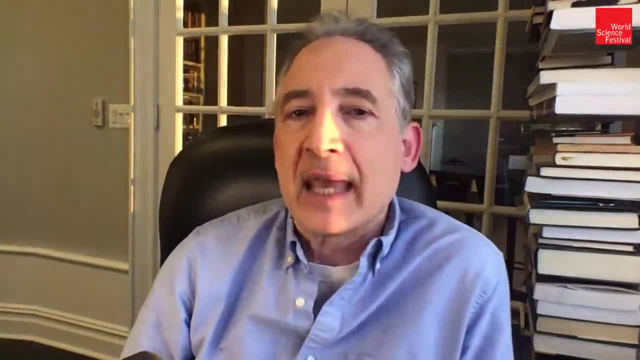 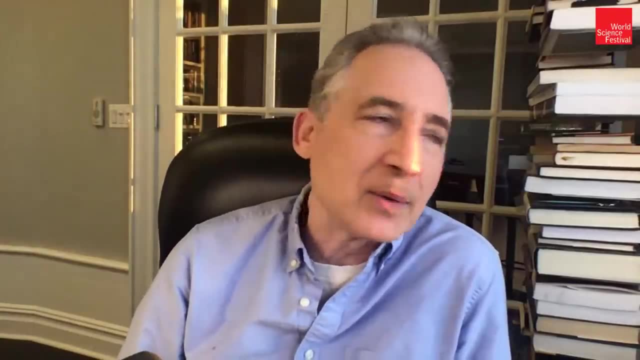 encounter in everyday life which makes use of some of the heavier of the cork species. You and I we're made mostly of up corks, down corks, gluons with electrons and a few other smattering of particles mixed in, But there are more exotic versions of corks that 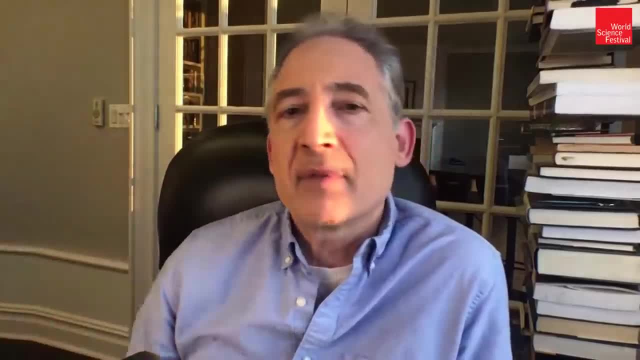 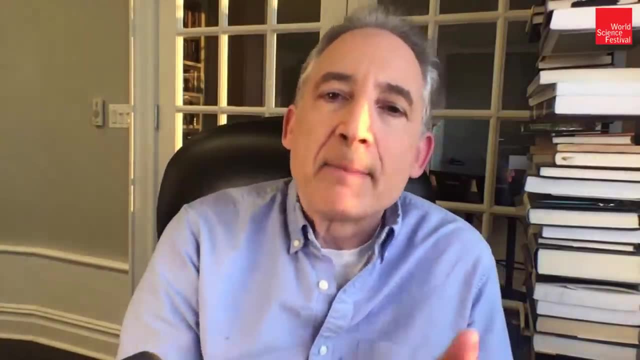 you are familiar with the top cork and bottom cork being the two heaviest of those. And the beautiful thing in the standard model of particle physics is that the particles can be organized in what we call families or generations. right, You've got the electron. 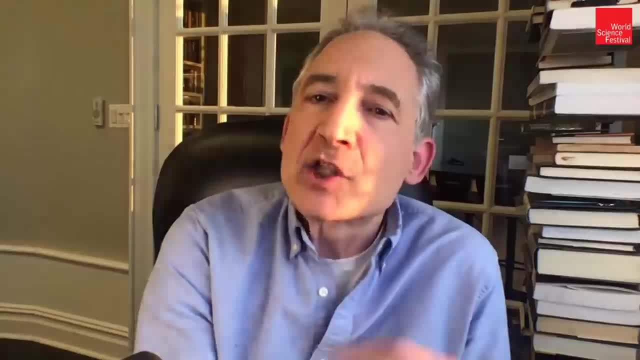 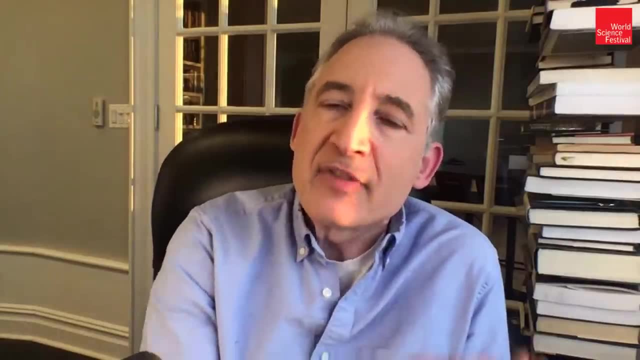 you got the muon, you got the tau. These are three electron-like particles that differ as far as the standard model of particle physics is concerned. They differ only in their mass. They don't differ in their interactions. They don't differ in their electric charge. how? 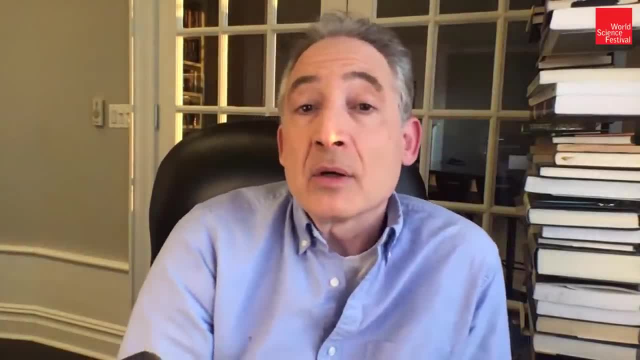 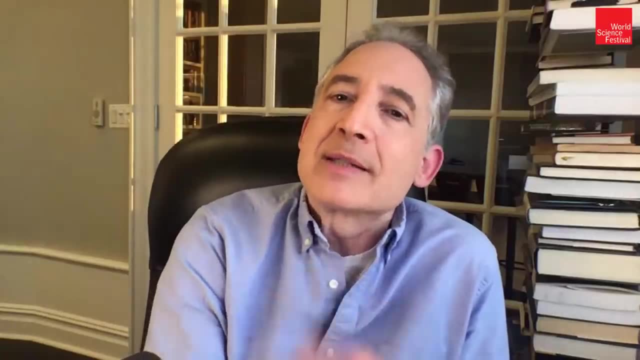 they talk to the electromagnetic force And they don't differ in their mass. They don't differ in their weak nuclear charge, how they talk to the weak nuclear interactions. But the data coming out of CERN is suggesting that maybe they do differ in their interactions. 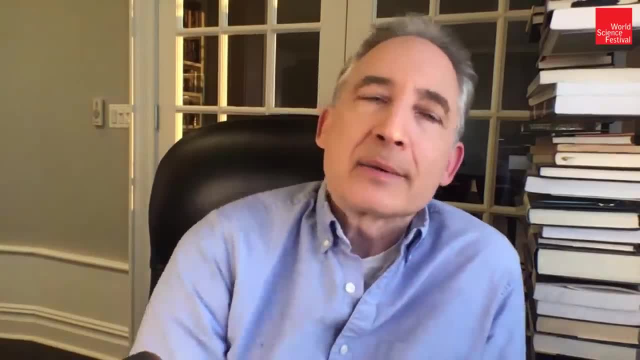 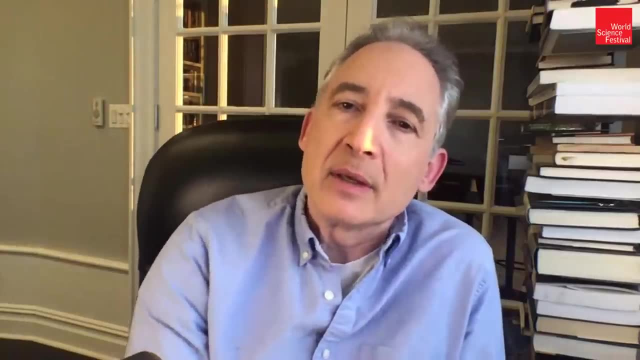 in some subtle way, because the decay products that are being witnessed are not following the pattern that you would expect if there was so-called lepton universality, that the different leptons, electron, muon, tau and so forth, that their interactions may not. 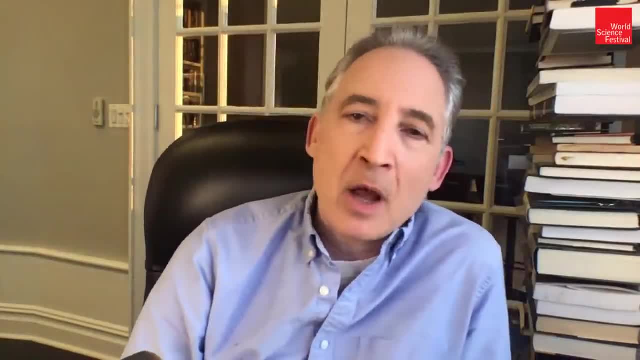 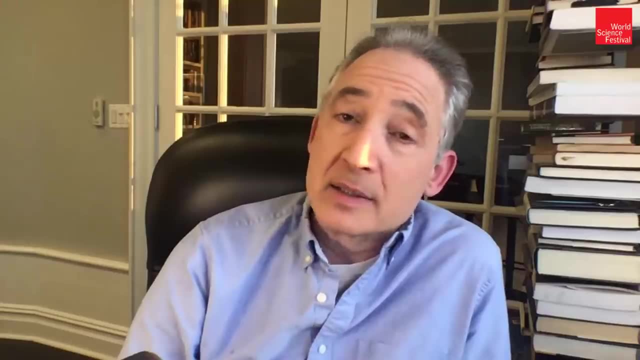 be identical. Now, are we confident of that data? No, not at all. It's what's called a three sigma effect. Three sigma effect: It's not a trivial effect, but there's a chance that it could be a statistical fluke, an anomaly. Normally, 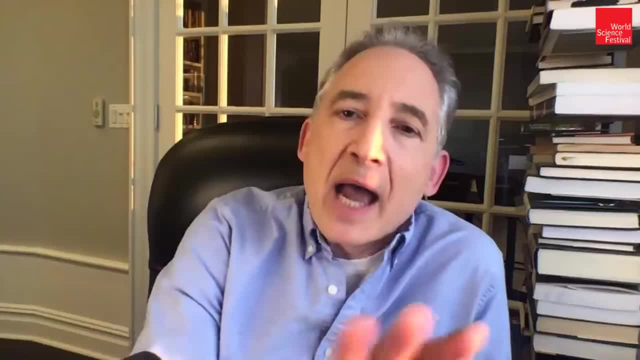 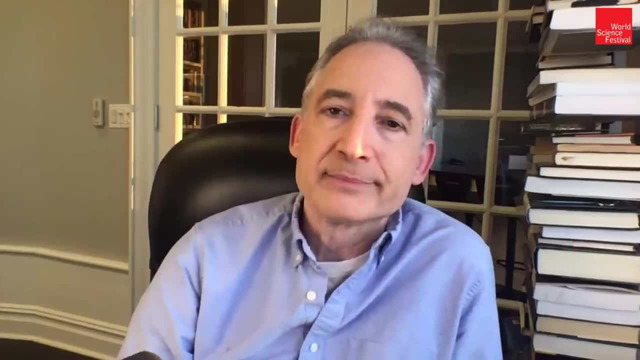 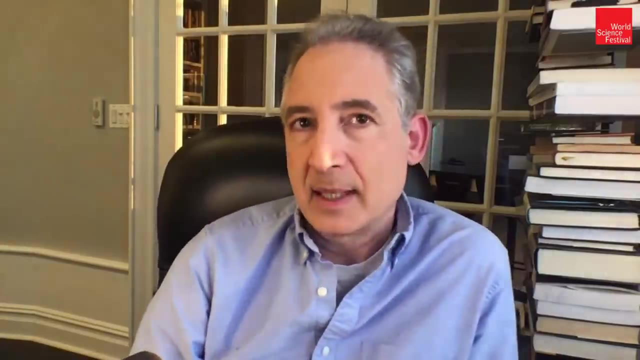 the gold standard for achieving a discovery is a five sigma level effect and we're not at that level as yet. So this could certainly go away, could evaporate, excitement could dissipate. But it is interesting to see that there is, even today, the capacity of experiments that are 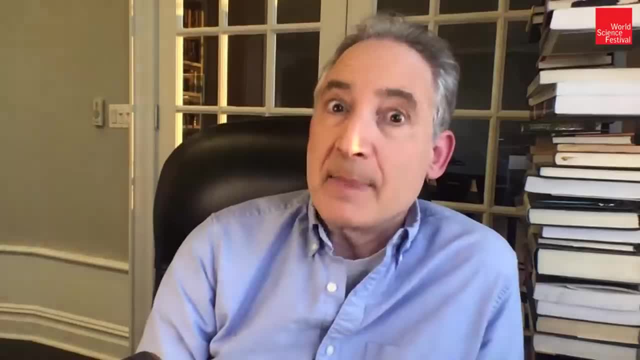 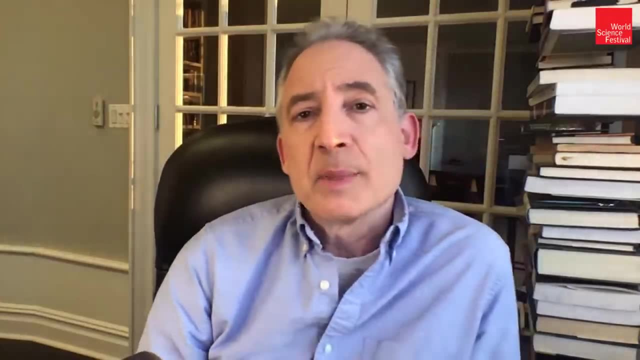 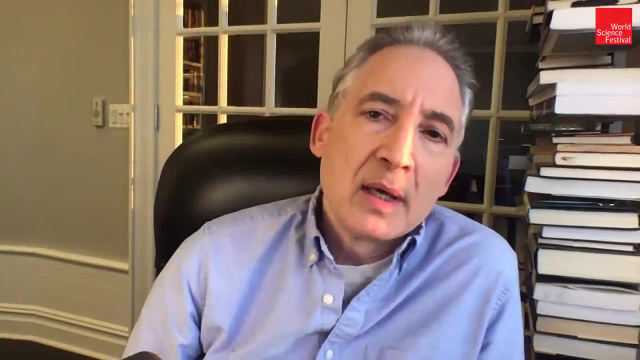 ongoing to perhaps give us deep insight into the nature of the world- surprising insight. So we'll see how that one goes. Another big announcement that you may have followed, perhaps closer to the conversation that we're going to have with Brian Schmidt, is to do with the Event Horizon. 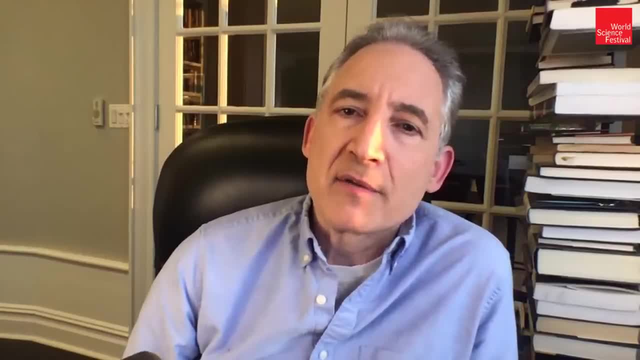 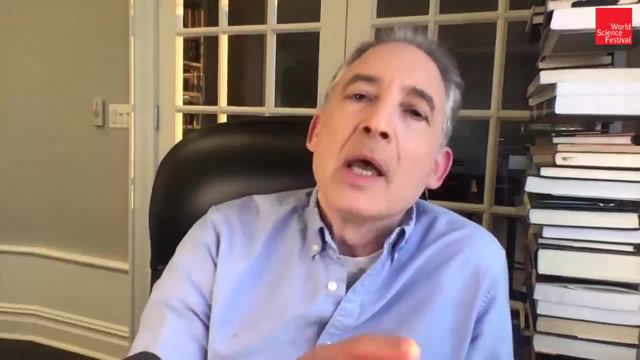 Telescope. Remember the Event Horizon? It gave us our first ever image, direct image. We often call it a photograph. It's not exactly a photograph, but it's a radio telescope version of a photograph of a black hole. I think we have that image here. 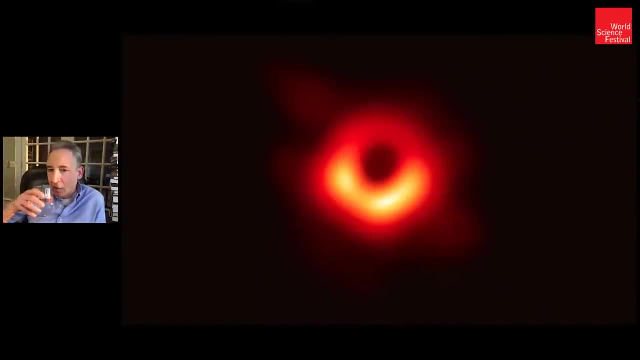 if we can bring that up. Yeah, there it is, that famous black hole image. That's a black hole in the galaxy M87, giant elliptical galaxy, 55 million light years away. That is a monstrous black hole, billions of times bigger than the Earth. It's a black hole, It's a black hole, It's a black hole. 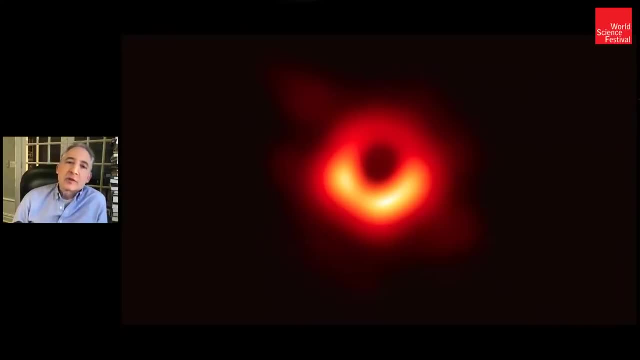 the mass of the sun And that, of course, electrified the physics community, the astronomy community and the world when this image was released by the Event Horizon Telescope team, Shep Dolman and his colleagues, because it's the most direct evidence that these 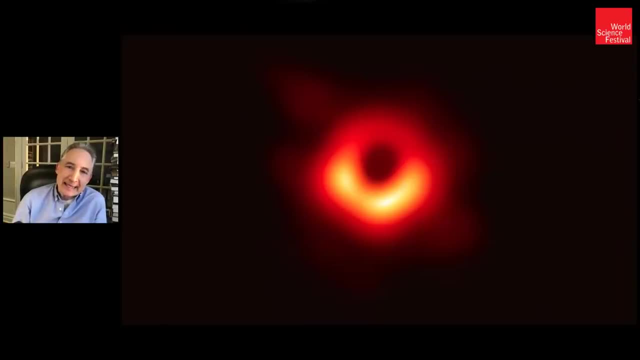 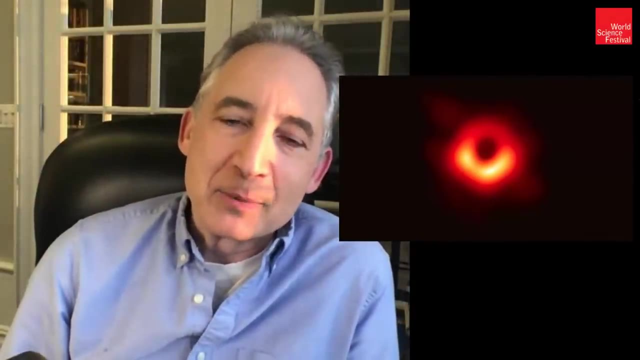 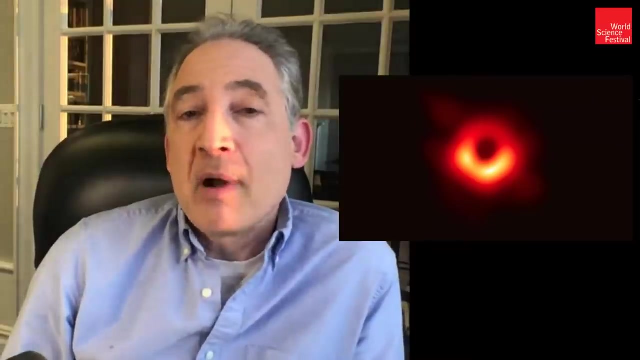 monsters of the cosmos actually exist. Einstein's mathematics, which Einstein himself resisted long ago, showed the possibility of black holes being real. but how wonderful to actually see one. And you of course know that the Nobel Prize this year was awarded for indirect data establishing. 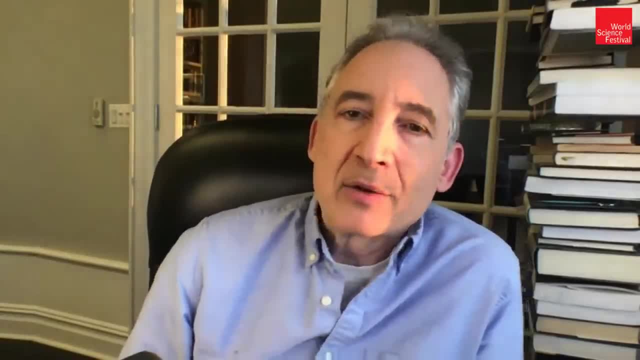 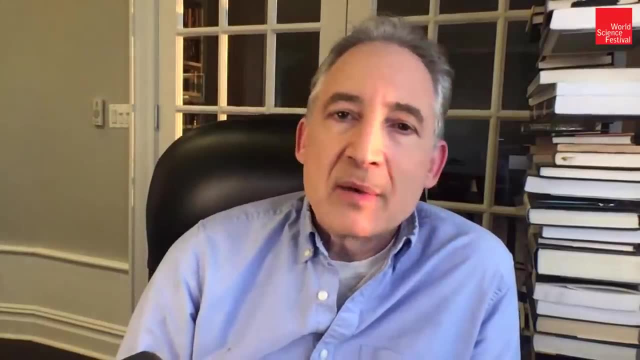 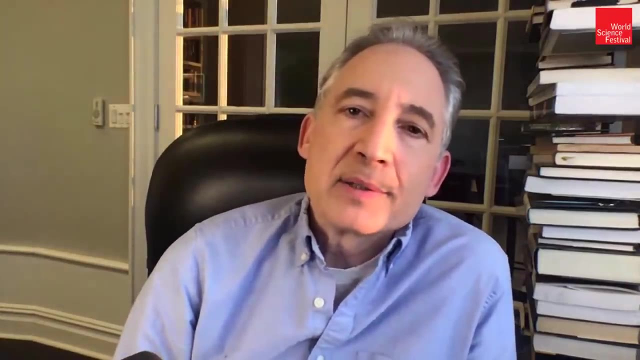 the existence of black holes. Roger Penrose: mathematical insights. of course we had a nice conversation with him in one of these interviews that we've been taking, that we've been having over the last year or so, And Roger's work of course was all mathematical, But the other work had to do with the motion of. 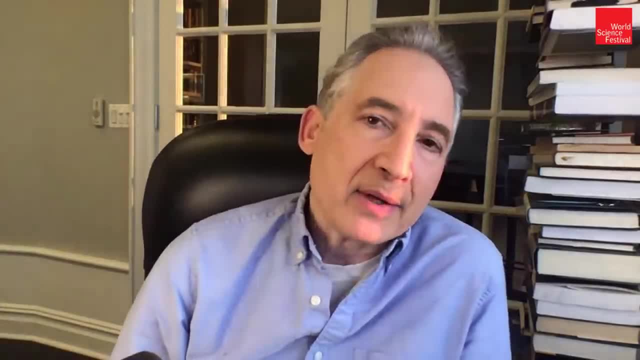 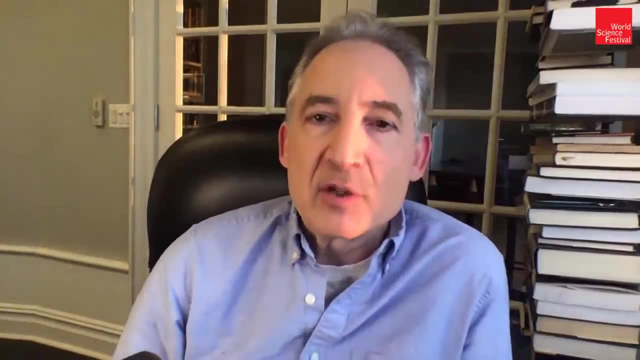 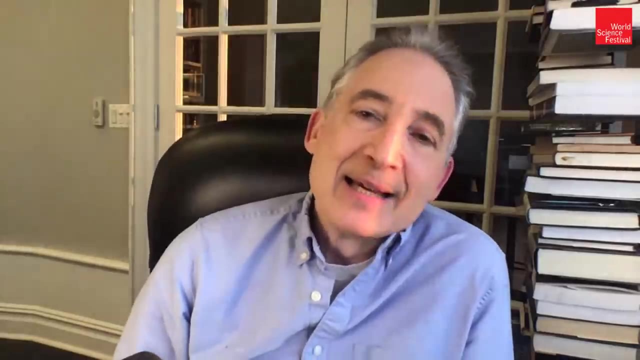 stars whipping around the center of the Milky Way galaxy, giving us strong but indirect evidence that a black hole resides at the center of our galaxy. And then the Event Horizon Telescope subsequently gave the world this very direct image of a black hole. But what has happened since is that the Event Horizon Telescope has done a lot of work on the black hole And it's been a lot of work on the black hole. But what has happened since is that the Event Horizon Telescope has done a lot of work on the black hole And it's been a lot of work on the black hole, And it's been a lot of work on the black hole And 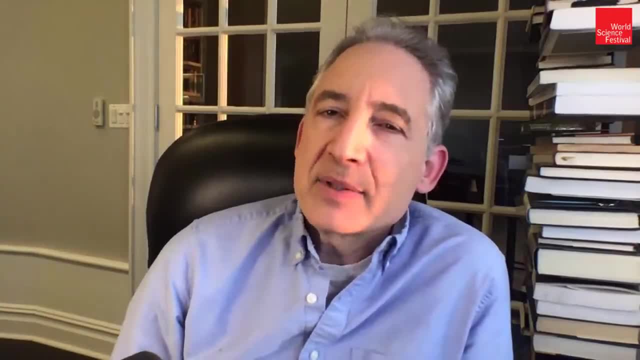 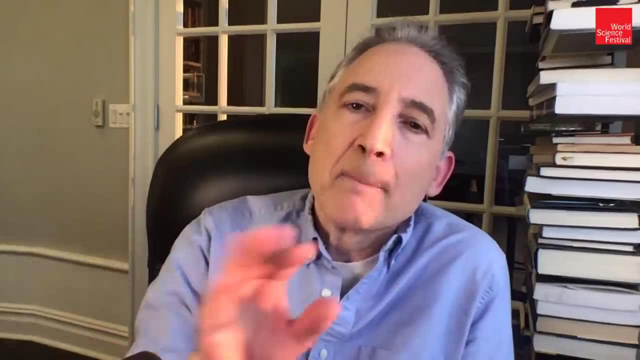 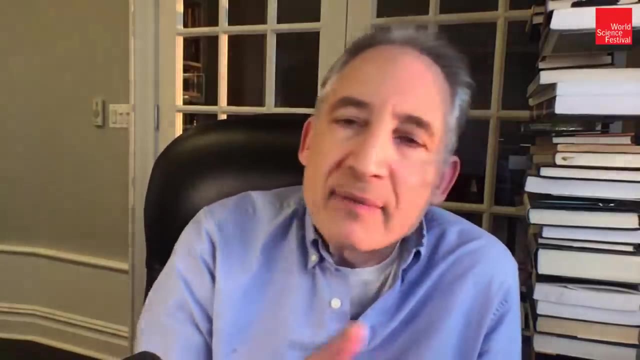 more refined analysis of the data. And the analysis that they've done is to measure not just the intensity of the radio waves but their polarization right. You may recall that radio waves it's a form of light and a particular wavelength of light And, as light oscillates, the electromagnetic fields. 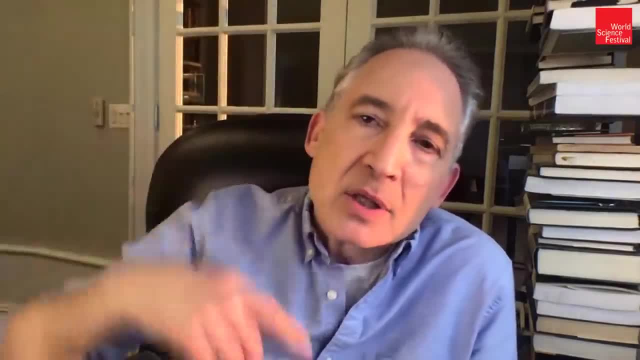 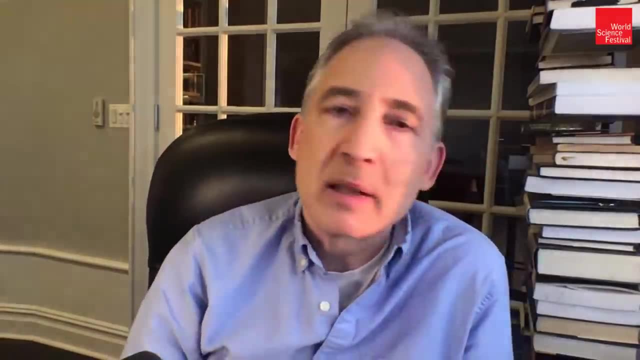 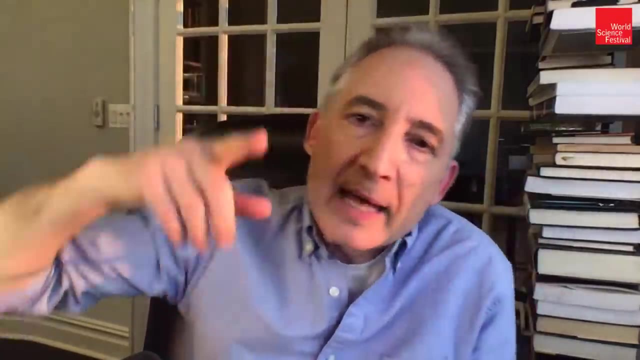 oscillate, there can be a directionality to those electromagnetic oscillations. That directionality is called polarization. That's why you have polarized sunglasses. right As light bounces off a surface, it typically becomes polarized. So if you have these glasses that only allow 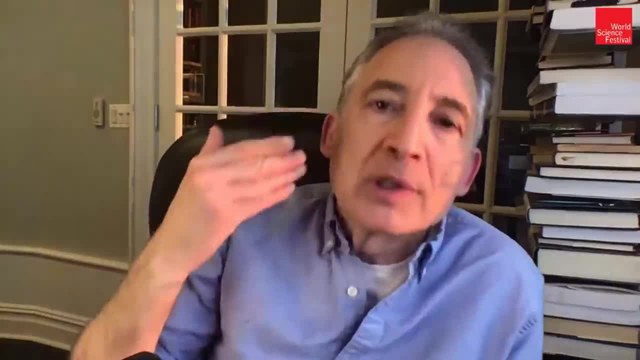 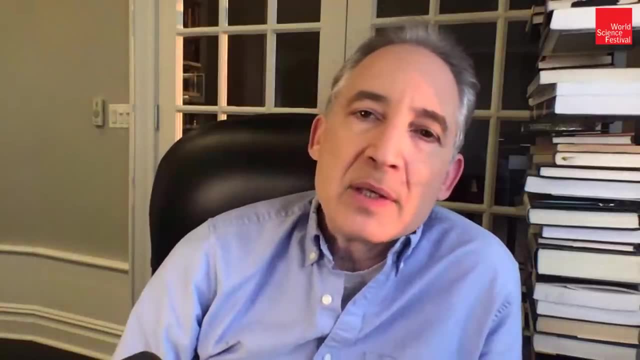 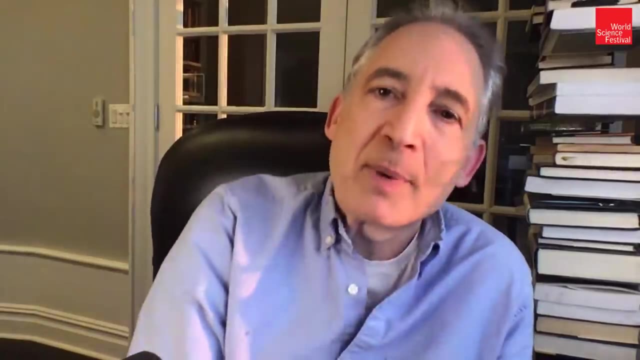 light that oscillates in one orientation through the lenses. it will help to block some light, block the glare, make it easier to see. So these folks at the Event Horizon Telescope have in essence used a polarized version of the earlier experiment to have a more refined. 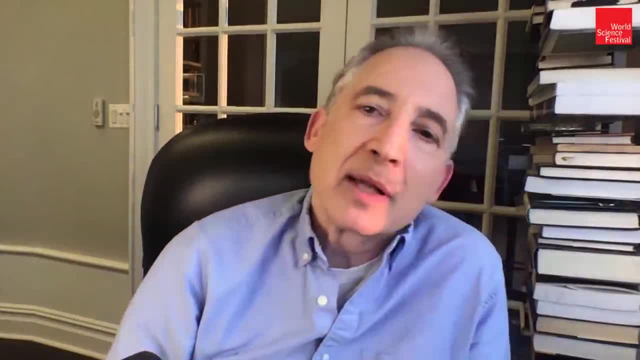 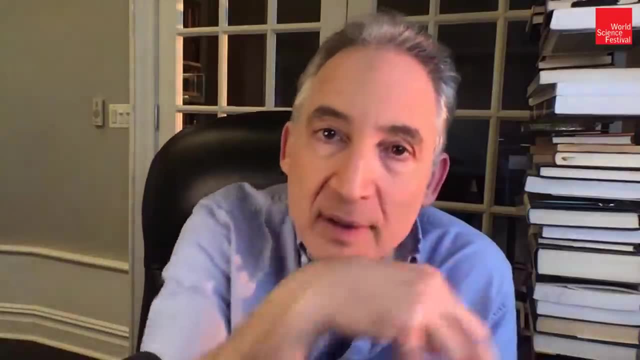 measurement of the plane in which the electromagnetic fields are oscillating, And that data gives insight into things like the magnetic field that is swirling around the black hole itself. So I think that image we probably have that one too. Yeah, it kind of looks like. 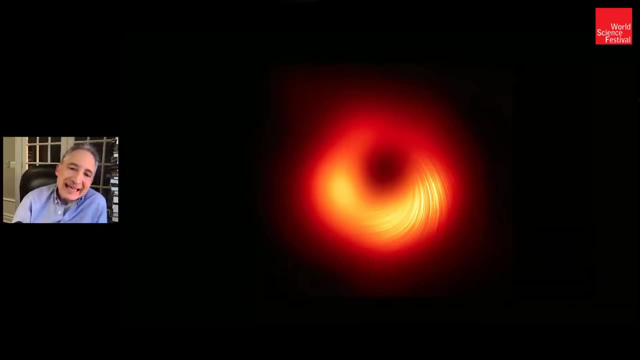 the other image. but you can see there's kind of striations in the data And those striations are giving information about the polarization of the light which ultimately will be used to give insight into the electromagnetic field. And that data gives insight into things like the magnetic field. 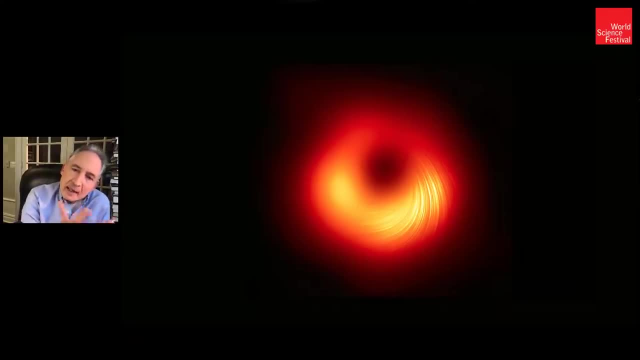 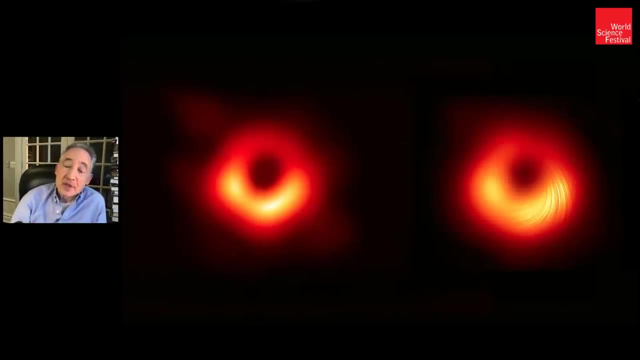 And that data gives insight into the nature of the electromagnetic fields, the magnetic field in particular that is twisted up in the vicinity of the black hole itself. So this is exciting. Here's a nice- yeah, comparison. Thank you for whoever brought that up on the screen So we can see the 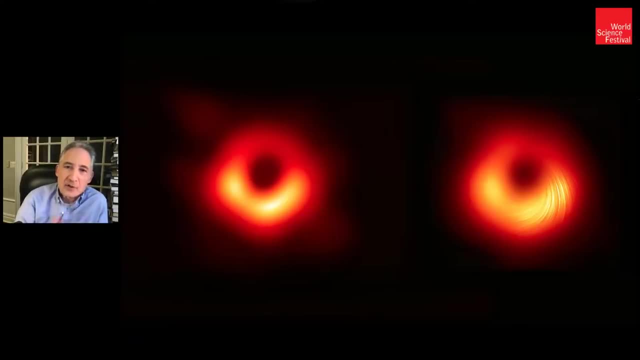 original image on. well, it's on my left as I look on the screen. I don't things may be reversed as you're looking at it, But you see this striated version on my further to my right And that is. 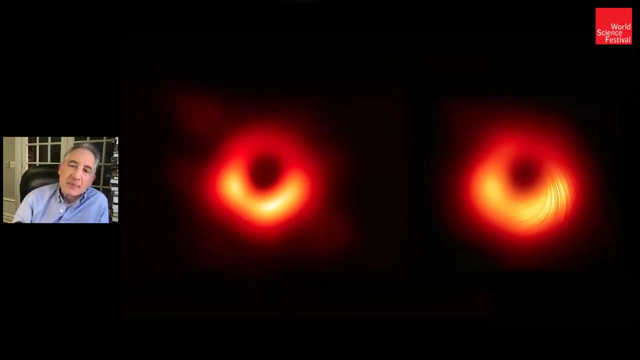 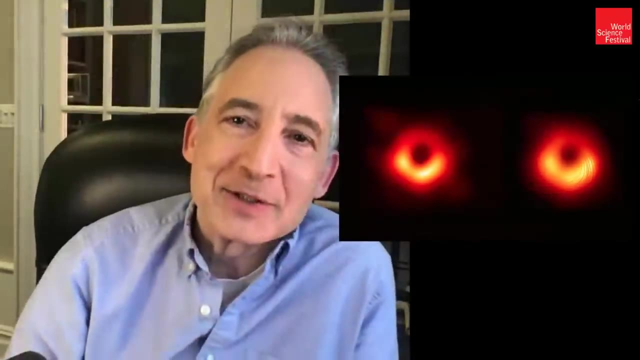 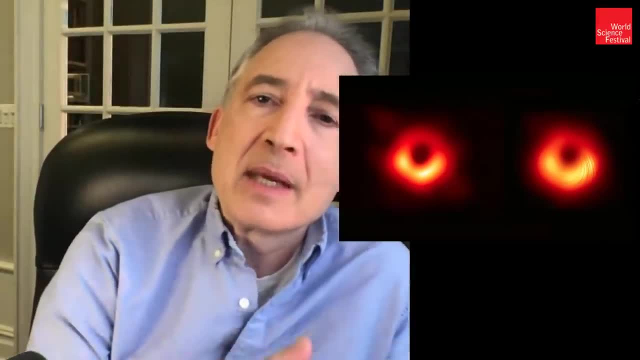 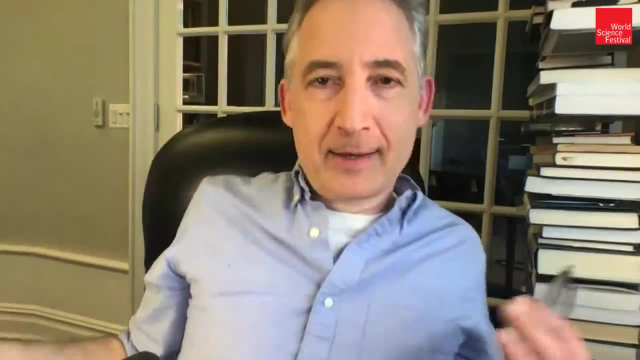 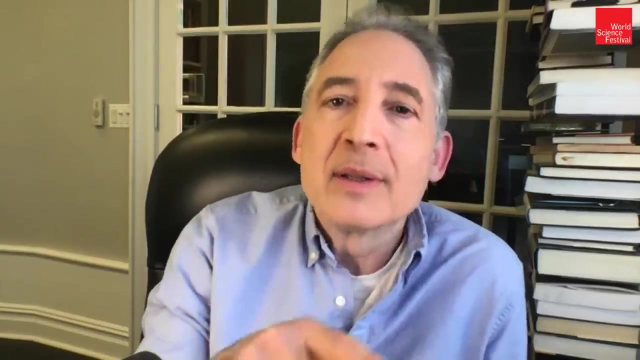 noted that the step that he imagines pursuing is to not just have static images of black holes, but to have cinematic, radio, telescopic images of black holes, of movies, And those movies will allow the black holes to be able to be seen. And that's what we're looking for, And that's what we're. 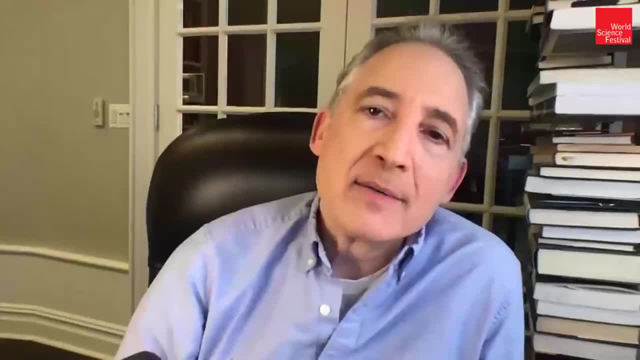 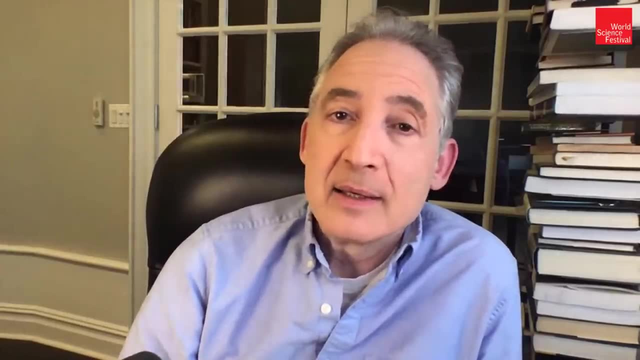 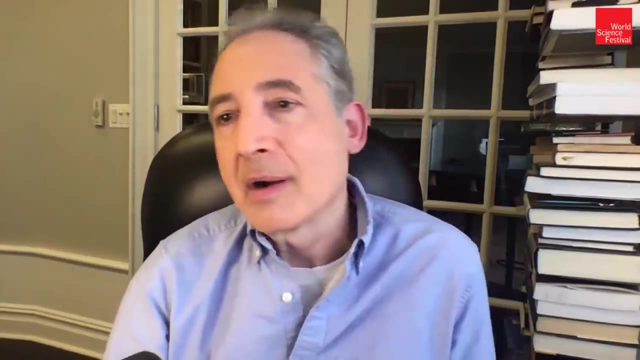 wondering is: are we really going to try to get the scientists to track the qualities of the radiation around a black hole, the magnetic fields around a black hole as they change over time? And that is an exciting next step. I don't know when that will be achieved, but that's what the astronomers are headed toward. So in a couple minutes I hardest. 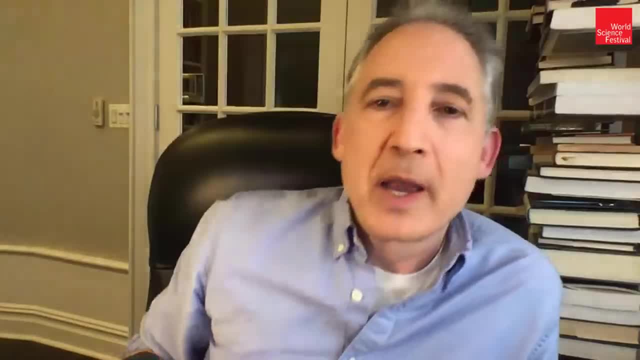 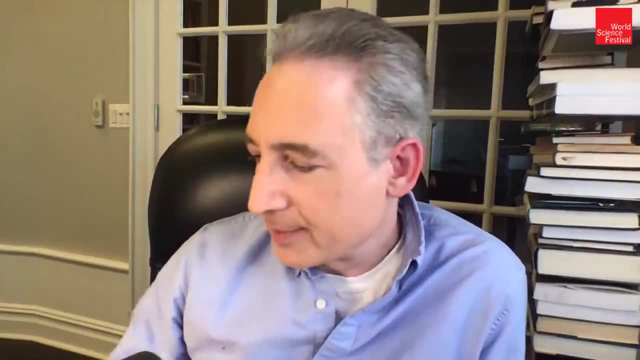 to darker. so in a couple minutes I'm going to bring in Brian Schmidt, But before I do that I just want to give a little bit of an introduction to his work. You know that I always try to frame the examples which I see, And for many of us. you know a lot of the things we observe. you know almost most of the time that we determine such things, something you 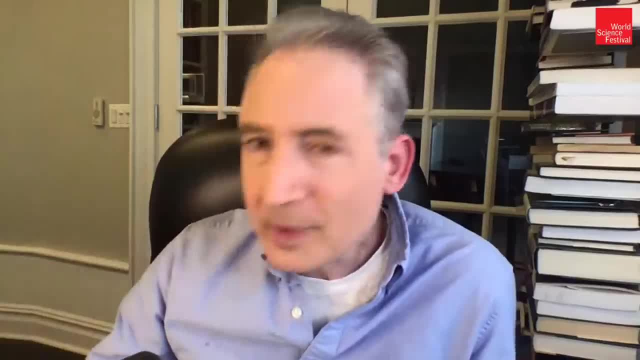 think about such things as days or some aspect, And then came when maybe the size did change, these things get more or maybe something like that. And that's what I say toください again the conversation a little bit. brian has made profound contributions to our understanding of. 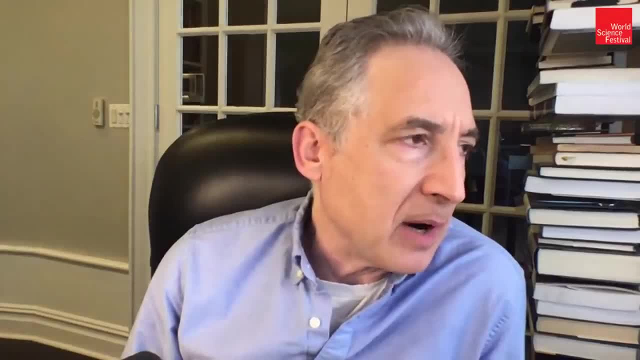 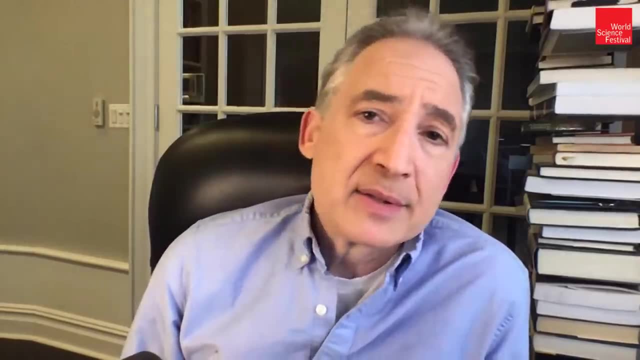 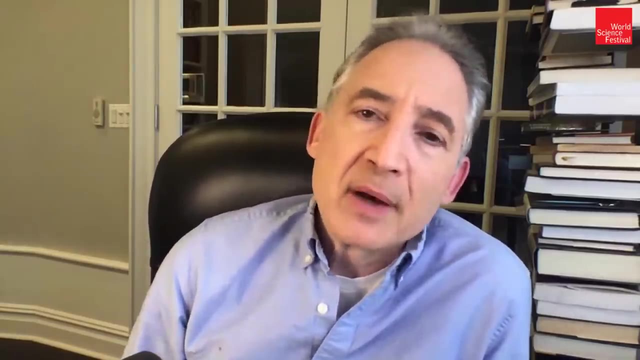 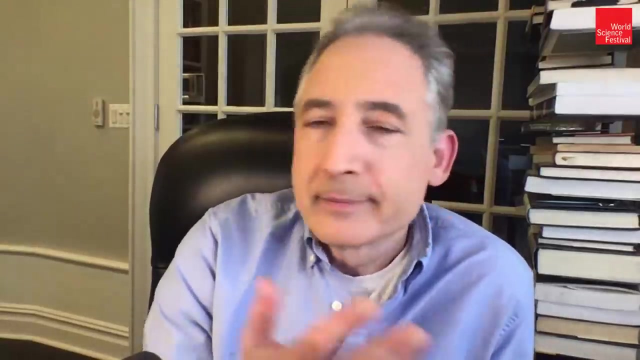 the cosmos, and the perhaps most well-known and the most profound insights came from his work some years ago studying the rate of expansion of the cosmos, as we've discussed many times in these conversations, the expectation that went all the way back to the early years of the 20th. 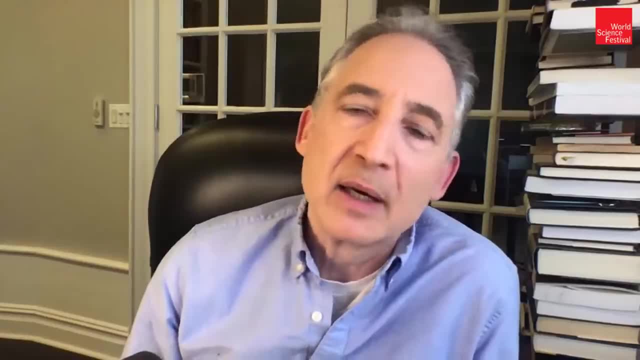 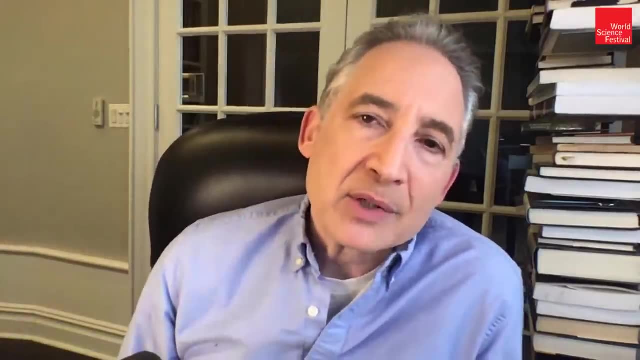 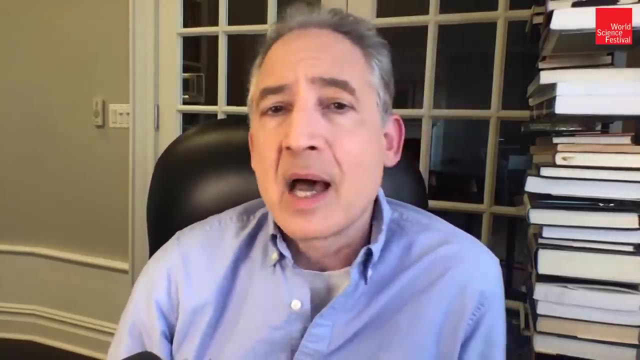 century, with albert einstein's general theory of relativity in the hands of the belgian priest george lemaitre, in the hands of the russian physicist alexander friedman and others as well, who were applying einstein's ideas to the entire cosmos. the expectation was that sure the universe. 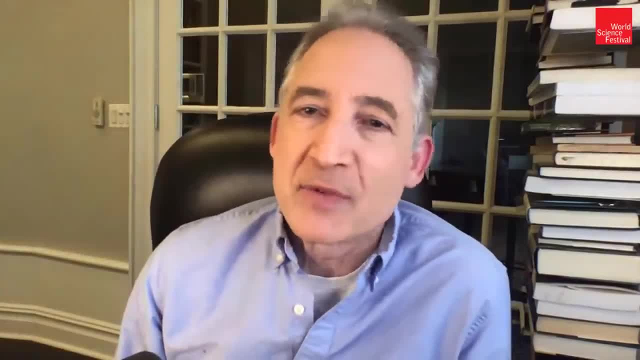 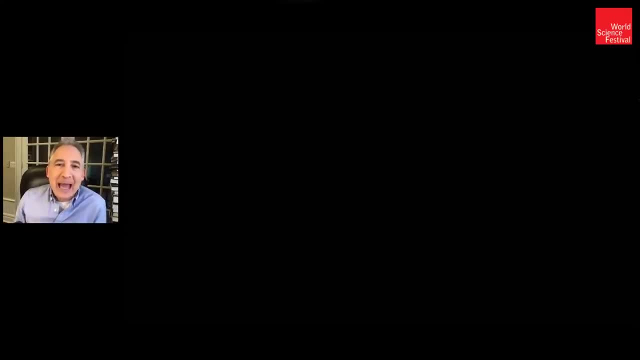 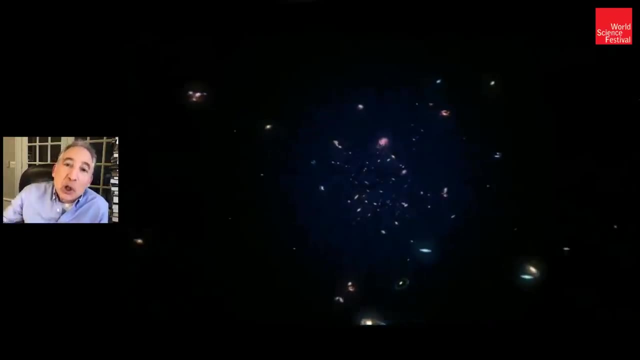 is expanding, but it should be slowing down in its expansion. the reason for that is completely intuitive. you have like a little video. if you, if you, were to toss an apple up into the air, right, we all know what happens. the apple goes up, but it goes up slower and slower over time because the earth pulls on it. similarly, the pull 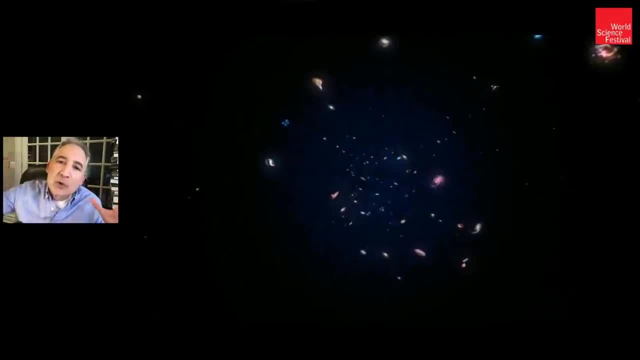 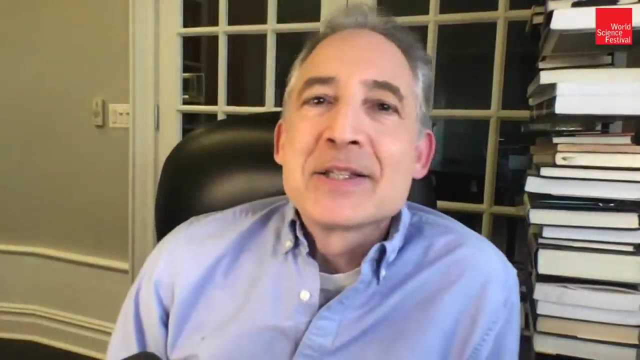 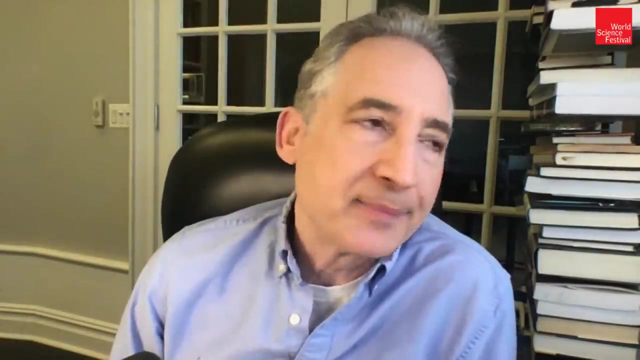 of each galaxy on every other. the expectation was it would slow down the cosmic exodus. that was what was supposed to happen, right? so, brian schmidt, others as well, that we have spoken to spread out on a couple of teams, adam reese, all perlmutter, others as well. 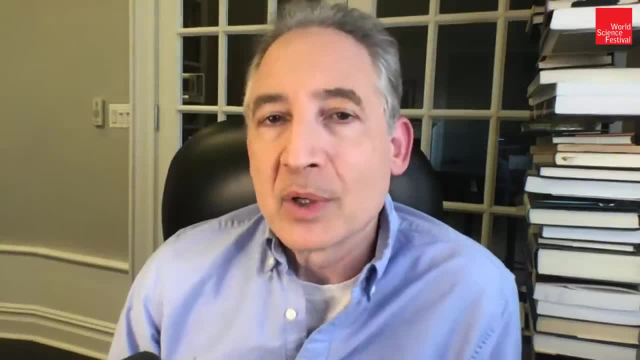 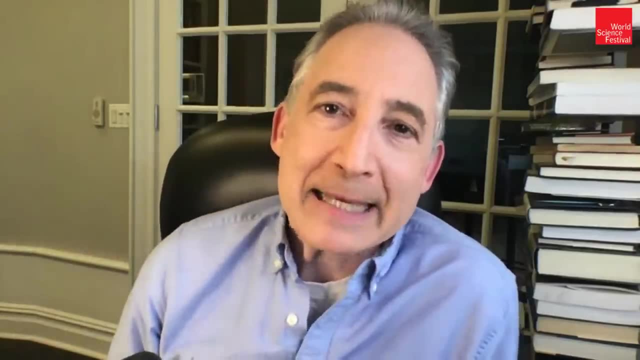 instrumental in the work that we're going to talk about. but their motivation initially- and maybe i'm wrong, maybe brian will correct me, i'm guessing- i think that their motivation was to measure the rate of cosmic slowdown. that was what the project was about: to put some quantitative 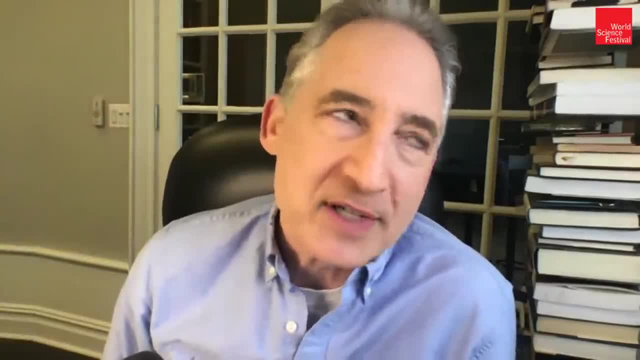 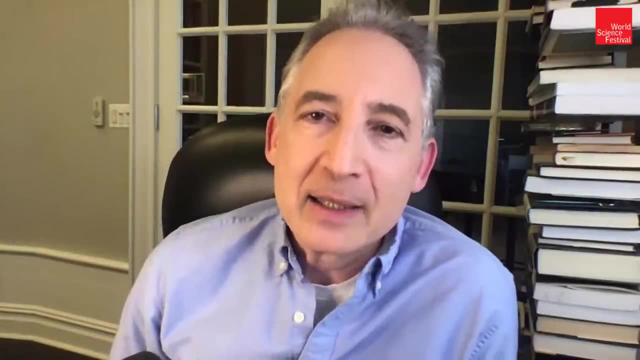 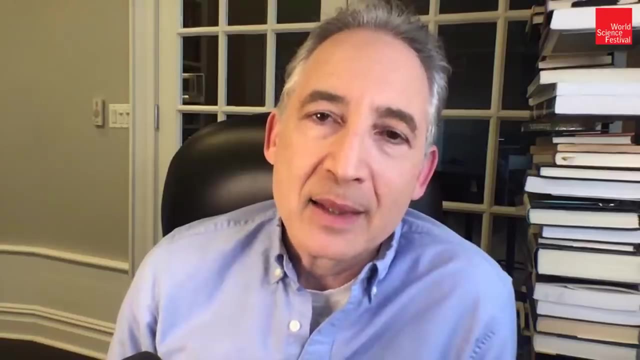 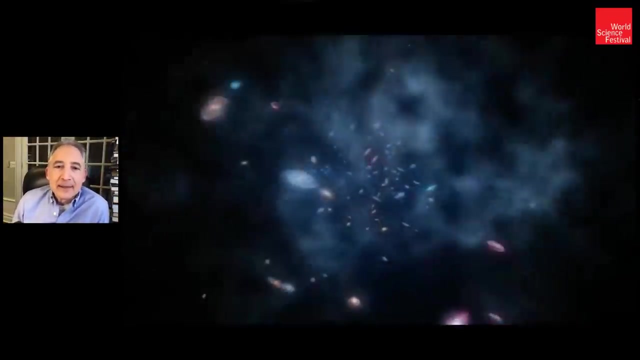 might behind this expectation that the expansion should slow over time. but the remarkable thing, as we will discuss, is that when the data finally came in and was carefully analyzed, they got kind of the shock of a lifetime that the rate of expansion was not slowing down, the rate of expansion was speeding up. so i think we have a little little visual on that they found 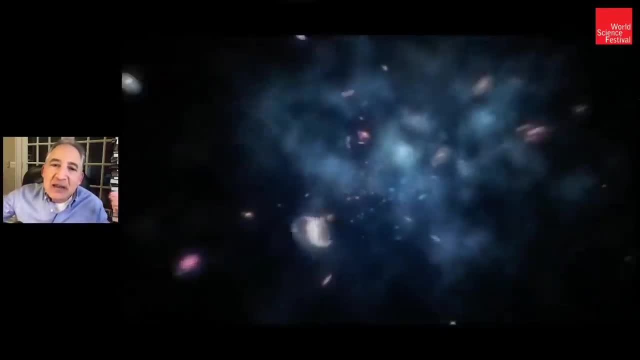 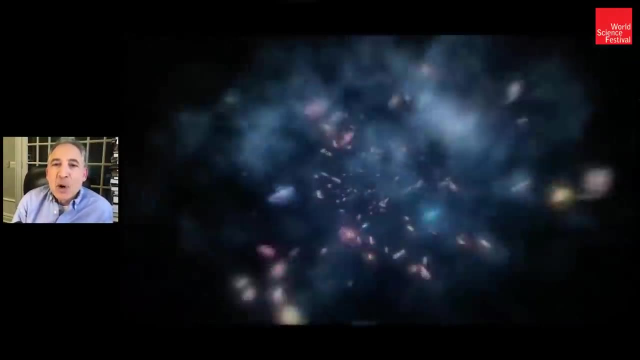 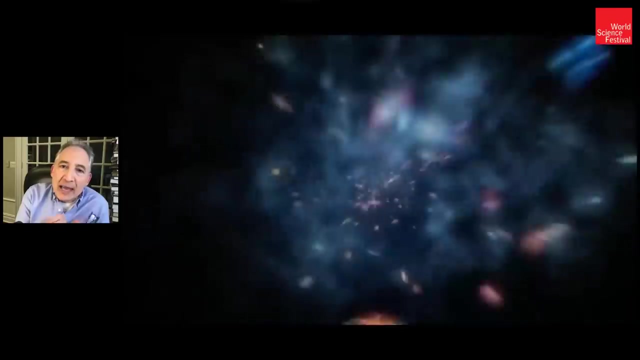 that the rate at which galaxies were moving apart was going faster and faster and faster over time. you see a little smoky white stuff there. that's our schematic, poetic, metaphorical image of what is known as dark energy. as we will see, the belief is that there is this dark energy in space. doesn't look so dark. it was dark you. 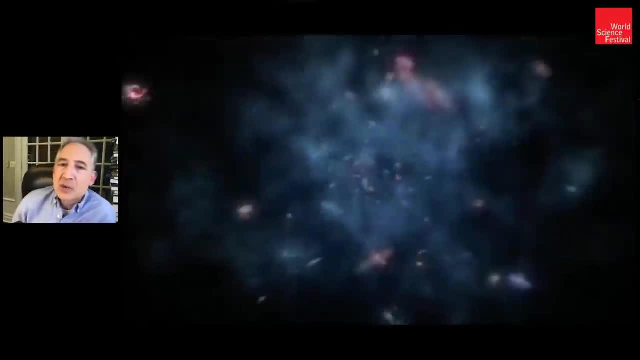 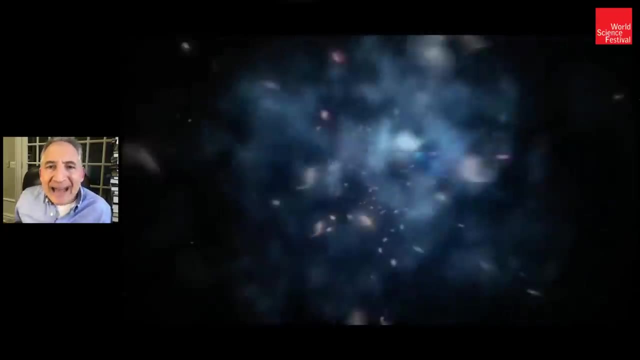 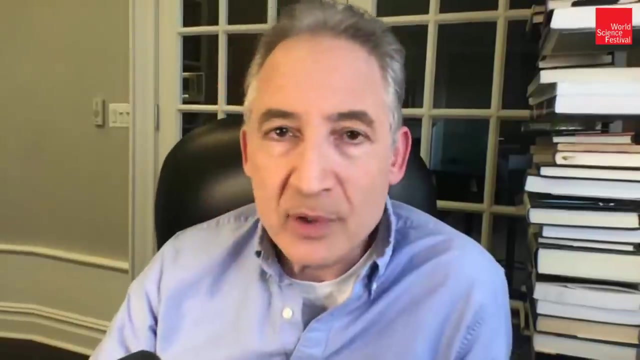 couldn't see it so we made it smoky white. but this dark energy can give rise to a kind of repulsive gravitational push that drives everything apart. not the attractive version of gravity that the expectation was would pull everything back together, so that discovery has kind of revolution. 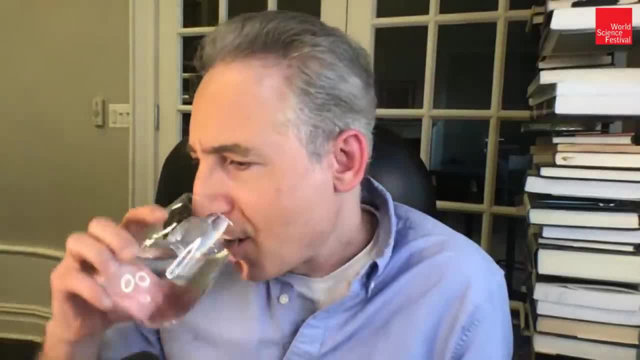 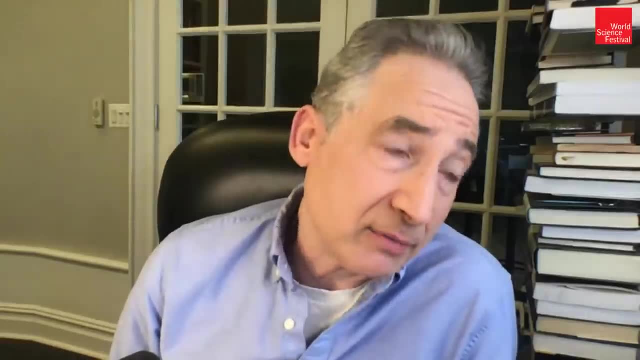 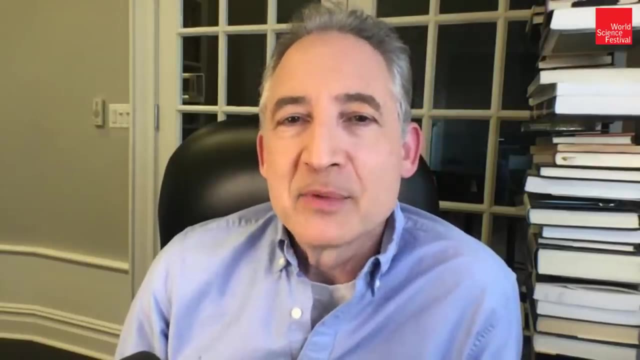 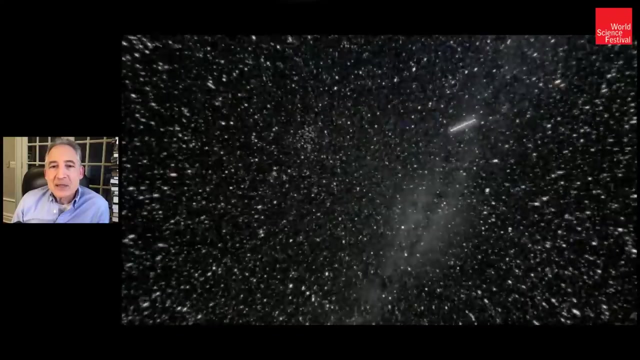 revolutionized our thinking about how the universe is changing over time and it certainly revolutionizes our understanding what the universe will be like in the in the far future. i think we have one final animation before we turn to bring brian into the conversation directly. if this accelerated expansion continues unabated, 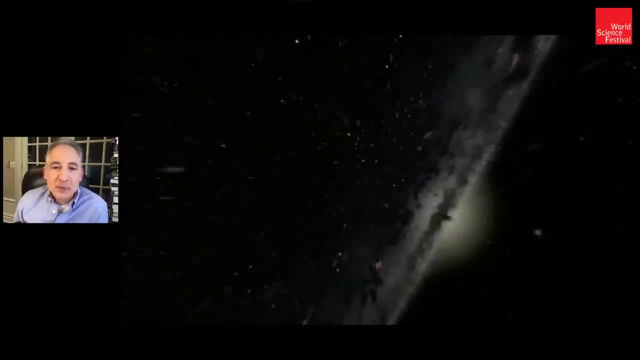 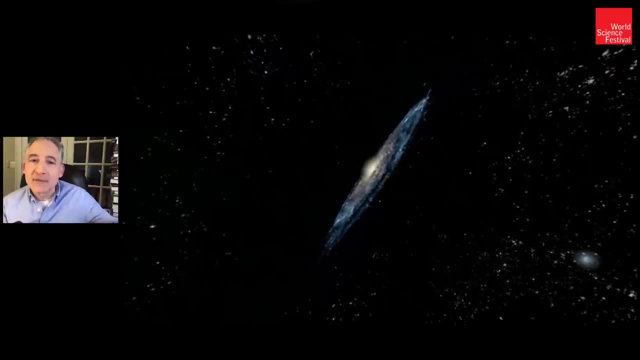 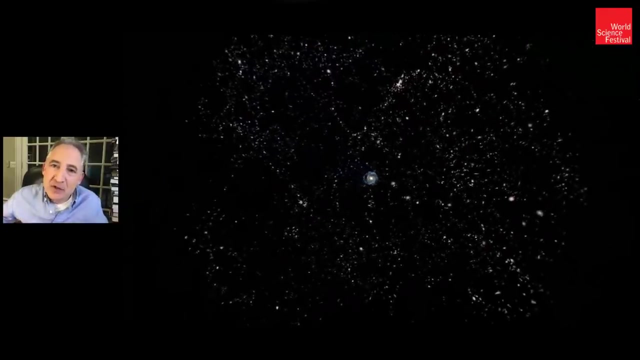 the amazing thing is, in roughly 100 billion trillion years, whatever the distant galaxies will be driven away so fast- faster than the speed of light- that an astronomer in the far future looking into the night sky they won't be able to see those distant galaxies if they're moving away faster. the 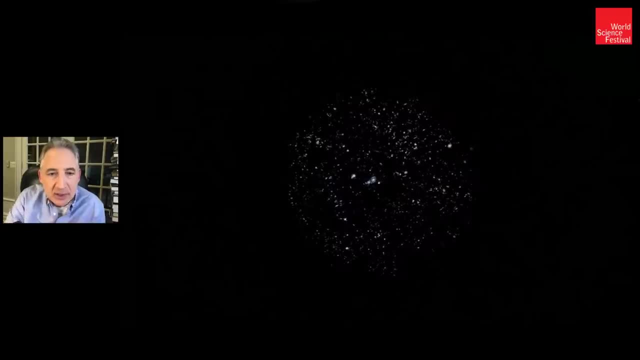 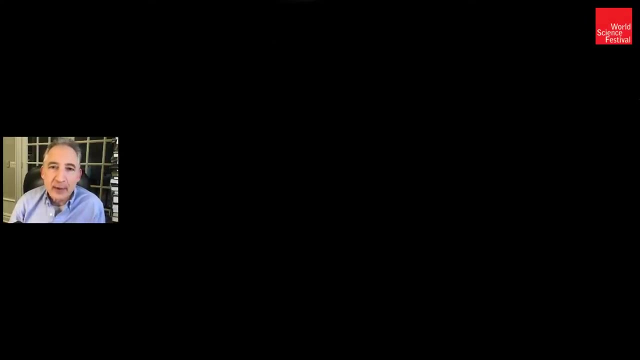 speed of light, the light they emit will not be able to reach us, and so the dark night sky will truly look dark, as we see here. don't, don't take this image away. this isn't a filler image. this isn't a transition image. this blackness represents what the cosmos 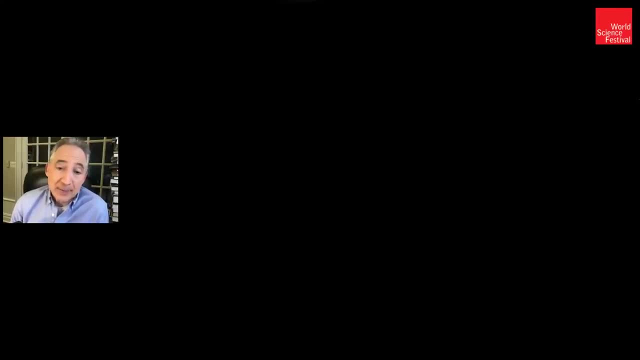 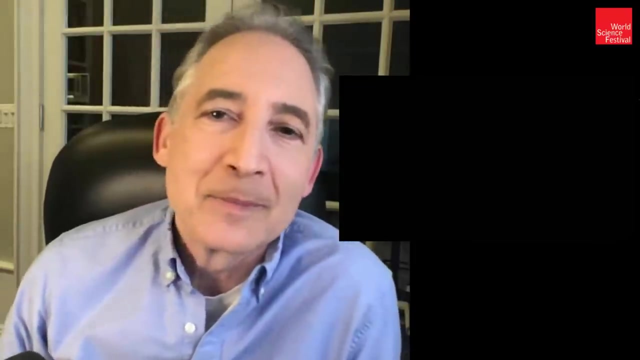 may in fact look like in a trillion years from now. that's kind of an amazing thing, because our understanding that the universe is expanding has come to us by the study of the motion of distant galaxies. if you can't see distant galaxies in the future, how will you even? 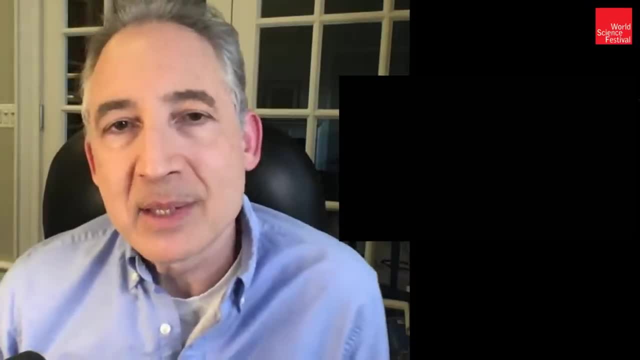 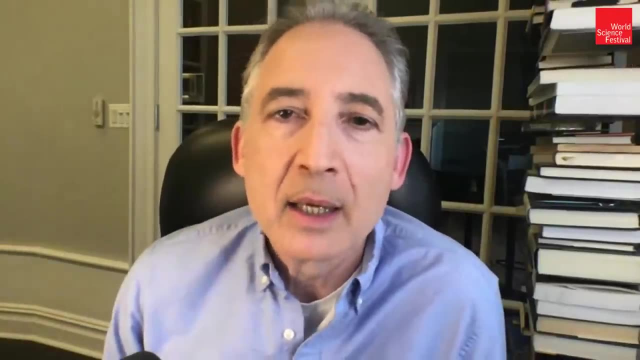 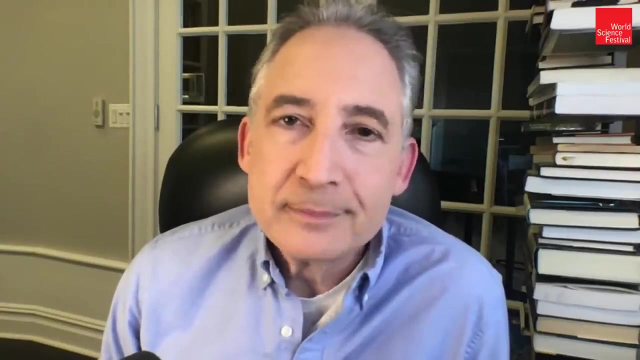 know that the universe is expanding, right? i mean, sometimes people say: well, you'll know it, because earlier generations will have passed on that knowledge, that understanding. but i'm fond of asking the question which i'll ask you all right now, which is: you know, if you have a powerful telescope, 100, you know, a trillion years from now, right, 100 billion. 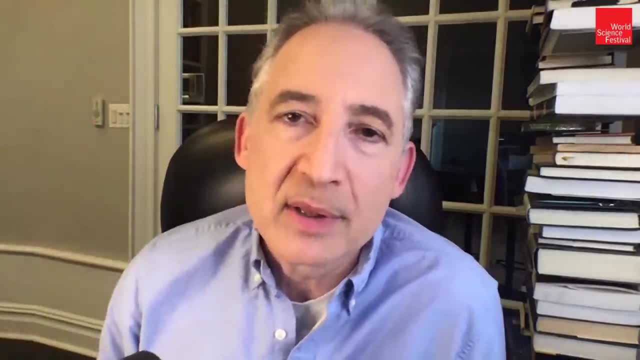 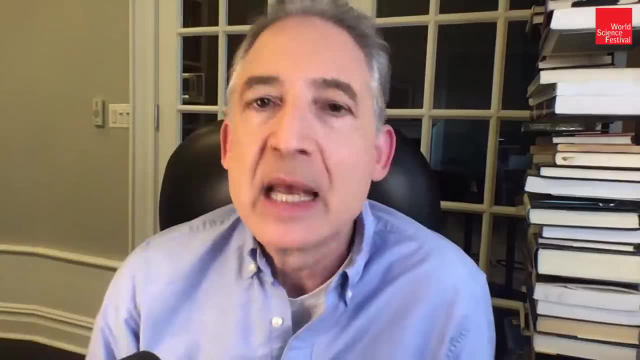 trillion years, whatever, and you use that powerful telescope to look in the night sky and you only see darkness and you think that we're just an island oasis floating in a sea of blackness. and then someone comes to you with this textbook from like a trillion years earlier. 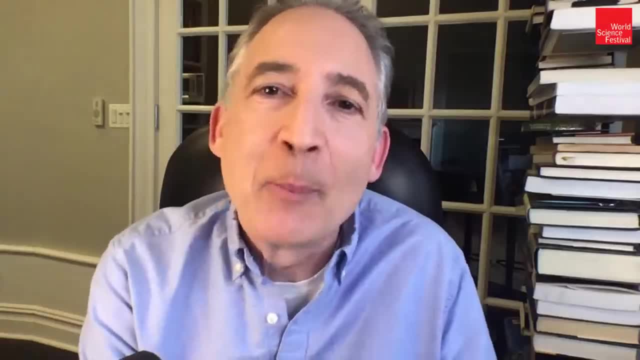 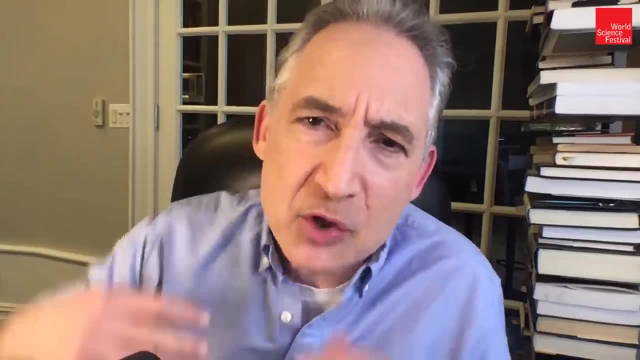 right and they hand you this dusty textbook and you open it up- you know careful not to have the pages crumble- and this textbook talks about a universe chock full of galaxies all moving apart from each other. and if they try to convince you that the universe was like that in the past? 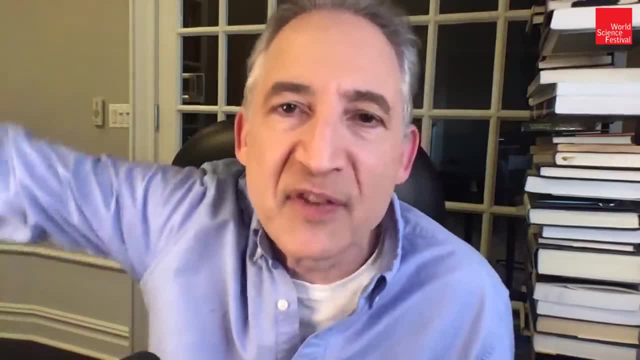 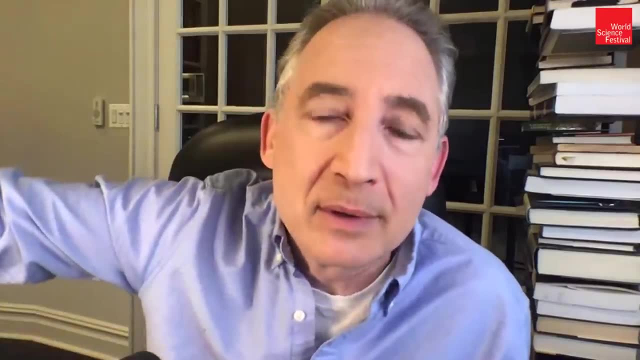 and that all those galaxies have disappeared over a kind of cliff at the edge of space. are you going to believe them? are you going to believe this ancient knowledge? you're going to believe your own state of the art observations which suggest that there's nothing else out there? 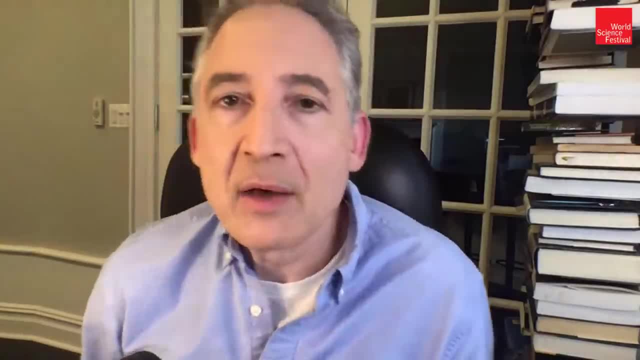 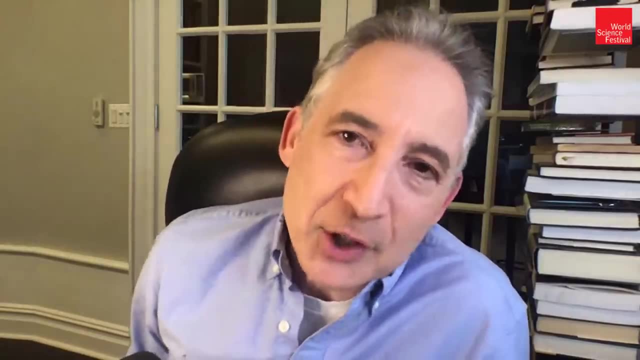 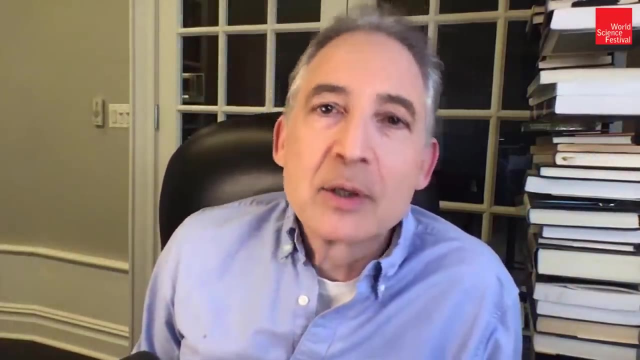 but blackness? you know, i don't know. you can answer for yourself, but i think most of us would be inclined to not trust trillion-year-old mythology about how the universe was and rather believe what we actually see. anyway, we'll ask brian schmidt that question in due course, but with that, let me. 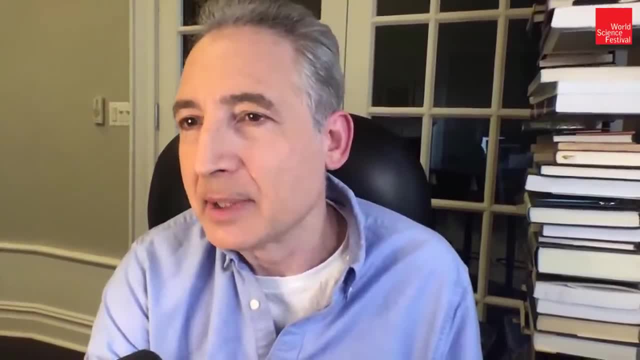 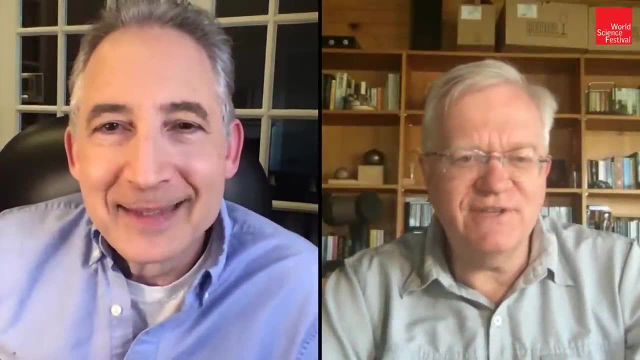 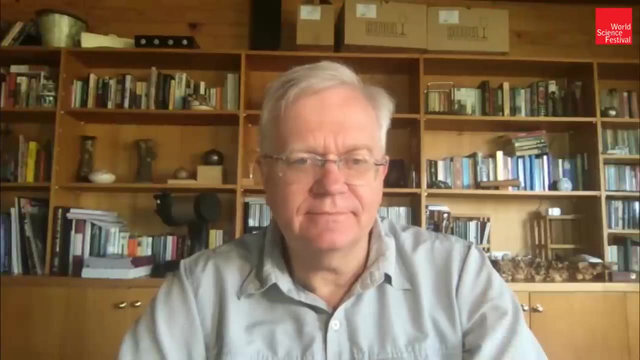 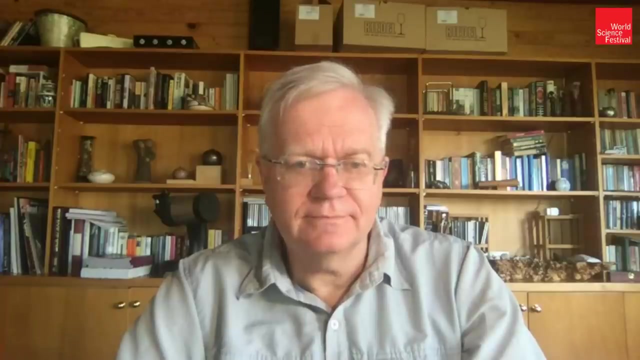 let me bring brian in to the conversation and i'll see you later. bye-bye, you are going to bring brian in at the end of the conversation. i believe that he is with us and as he's brought on, hey, brian, how are you? good morning evening. yeah, exactly, let me just remind everybody who's with us. here that brian schmidt is a distinguished professor of astronomy and the 12th vice chancellor and president of the australian national university. he completed his astronomy master's degree in 92 and phd from harvard in 93 and for his work, as i mentioned, on the accelerating universe, he would 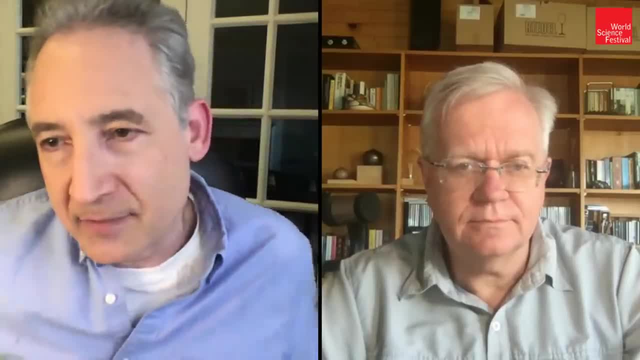 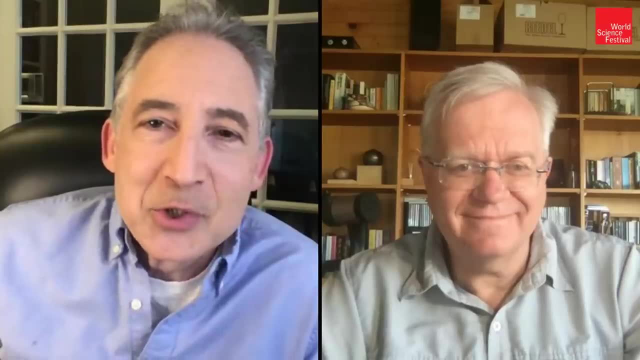 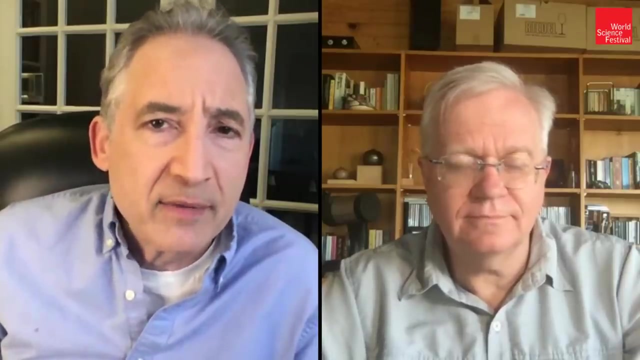 was awarded the 2011 Nobel Prize in Physics jointly with Adam Ries and Saul Perlmutter. So thank you for taking time out to join us. It's good to see you. I think the last time I saw you was when I was in Australia for a World Science Festival event some years ago. I don't remember. 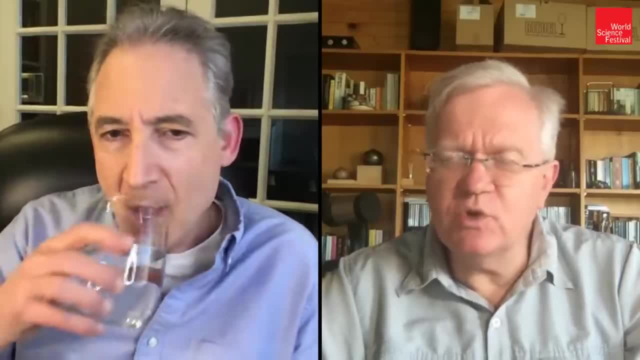 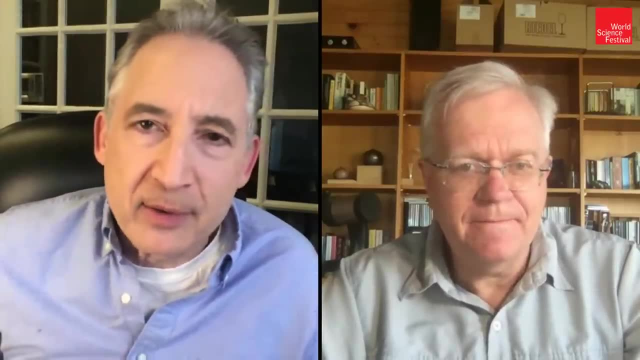 which one? that was You. I think it was two or three years ago. Seems like a lifetime ago now, I'm afraid. Yeah, right, Exactly. How have you guys? well, you guys are doing much better than we are, right? Well, yeah, So we've been COVID free here in Canberra since June. So life in. 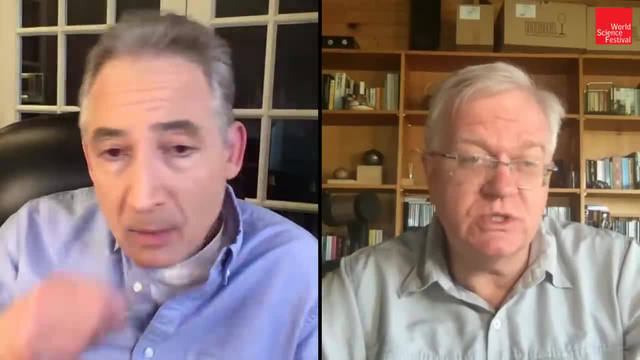 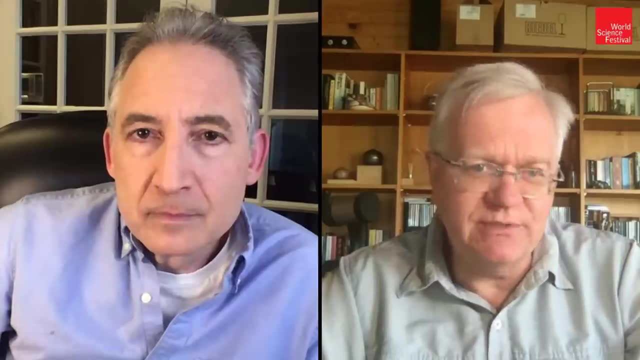 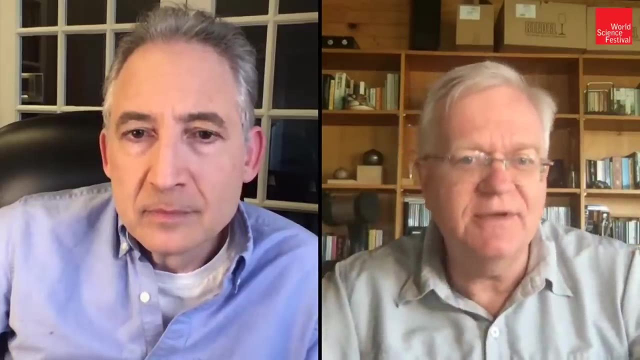 Canberra is very normal, as in pretty much since June. So we're, you know, our classes and everything are normal. but the COVID-19 is now out in Brisbane And you know it's quite interesting because we DNA trace every single COVID case now So they can tell. 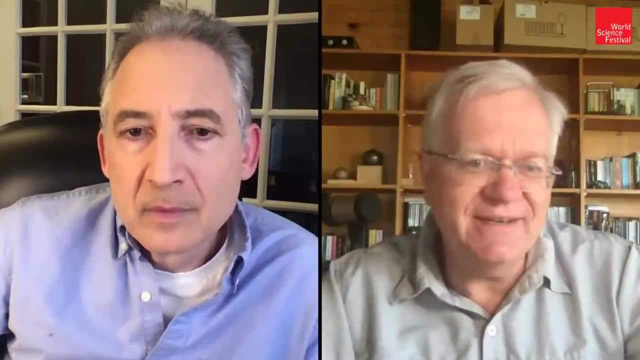 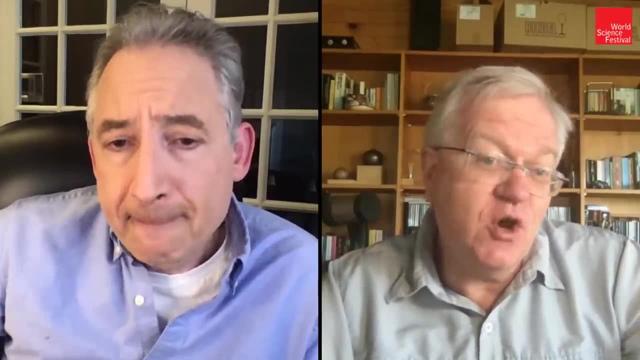 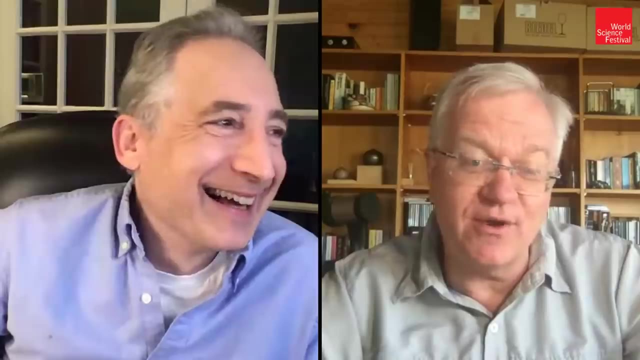 exactly where it came from, And they know there's an intermediary which is unknown, And so we'll see. I have a feeling Brisbane's going to have to shut down because, as you know, exponentials which we use in cosmology, there's one stable number which is zero. Otherwise we're growing. 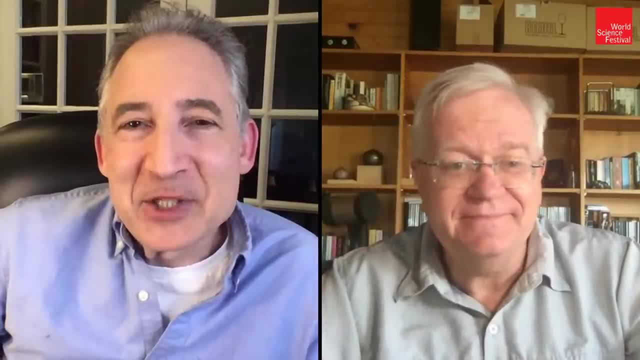 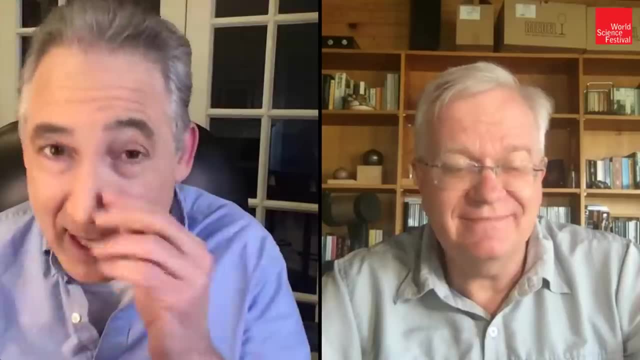 or decaying. Yeah, It's an amazing thing how people's intuition about exponentials is so modest compared to the intuition that we need. I mean, by the time you realize that something's exponential, you're not going to be able to do anything about it. You're not going to be able to. 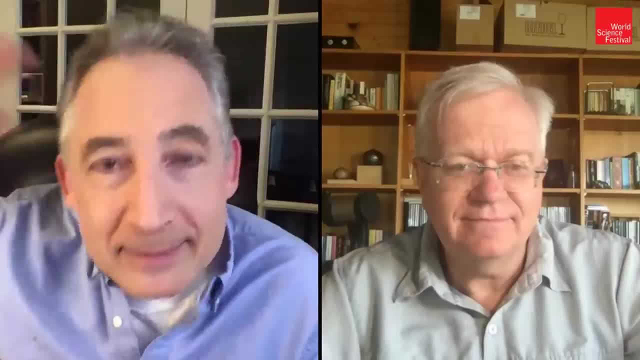 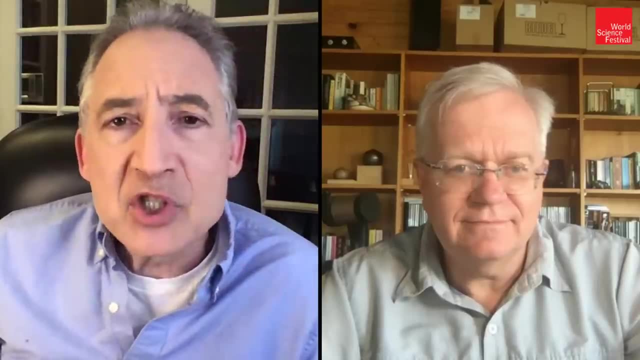 do anything about it. You're going to be able to do anything about it Because we have the ability to see what's actually growing. It's too late? Yeah, You know. you have to be thinking. you know many e-folds ahead of where you currently are. if there's any chance of stemming. 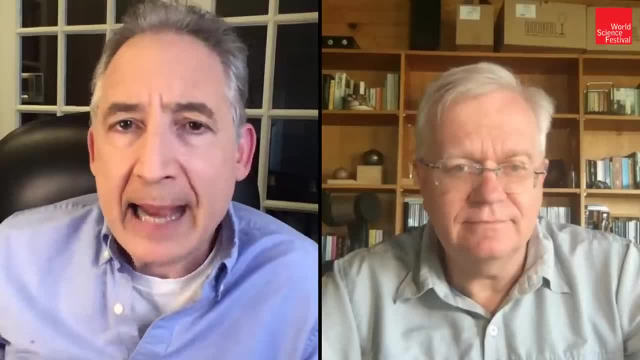 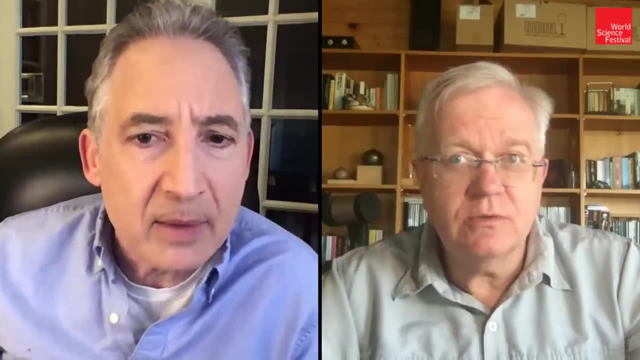 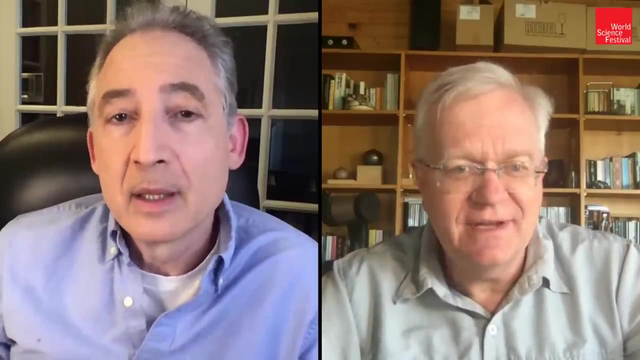 the tide. But I was told that at world science festival Brisbane people were packed into the, the concert hall without masks. Is that I mean? is that craziness? or I mean, It was absolutely fine until yesterday. As soon as you have it, So when you have nothing, 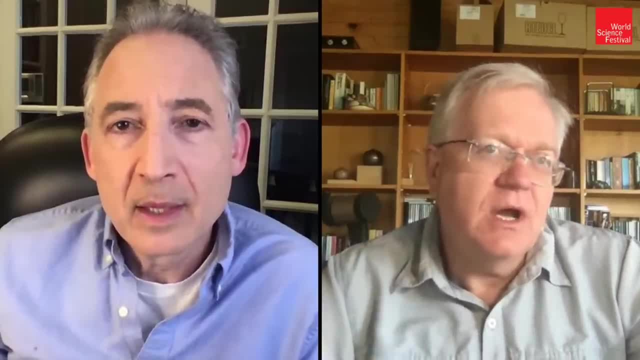 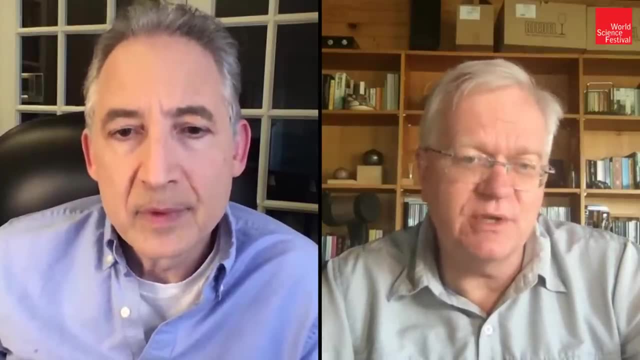 you have nothing, you have nothing to fear, and so, uh, the problem is now we know there's a case out, and that means there's probably 10 cases out, and so i'm i fear that brisbane is going to have to shut down hard. wow, uh, because, uh, i think we've decided, after getting all this way without killing, 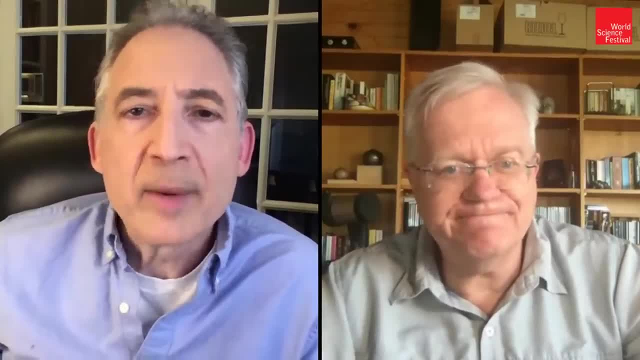 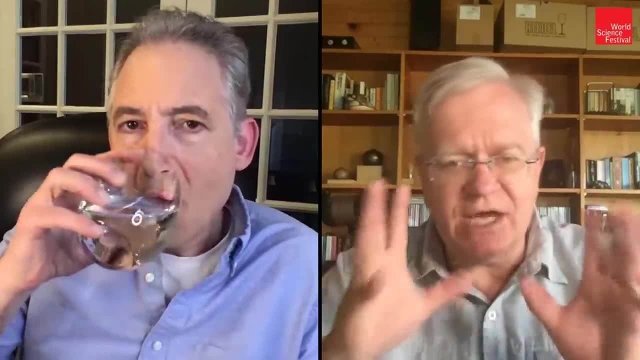 uh, millions of people. it's probably good to stay that way. and what about the rest of australia? similar situation, or yeah? so, uh, it's been. you know there's been these little flash lockdowns where we shut down to get it back down to zero again. but, uh, most of australia right now? uh, melbourne. 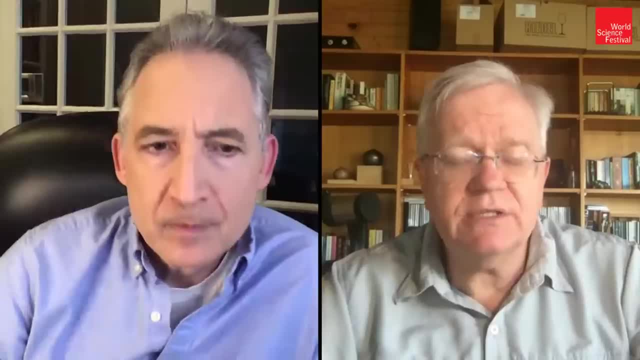 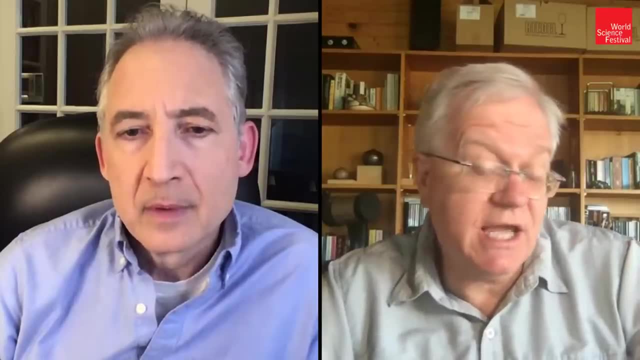 had a big breakout and was shut down for 112 days. but, uh, most of australia is like canberra- canberra's just been the longest period of time, right? so, uh, we've been very lucky and can i say canberra's been quite interesting. it's been very open and we've just had very good contact tracing and very 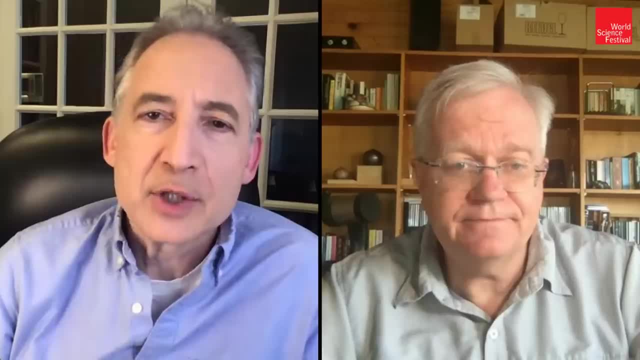 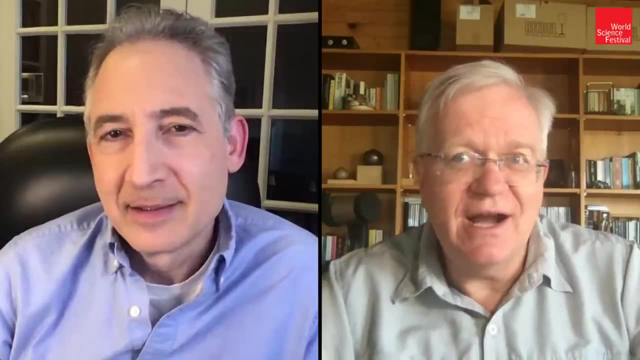 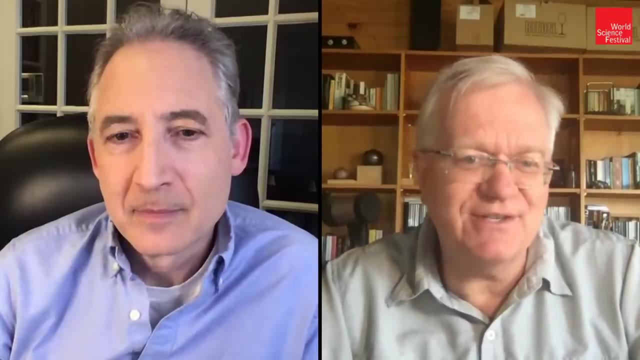 sensible public health policy here. yeah, that's what leadership does: right, compared, evidence, informed, and in our case, our, our government is not any particular different than yours, but it, uh, it panicked and it panicked and actually decided to better listen to the scientists, which was quite refreshing. but you just want to say that that's a, that's a modest difference from the administration. 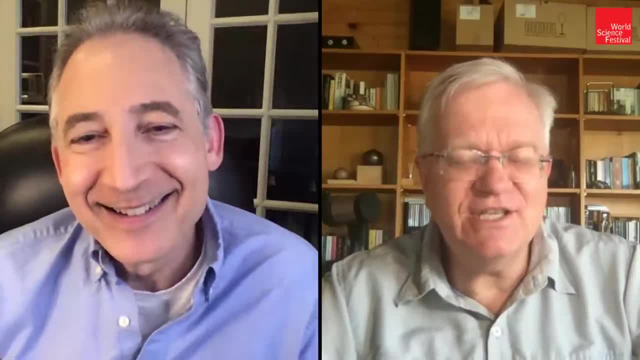 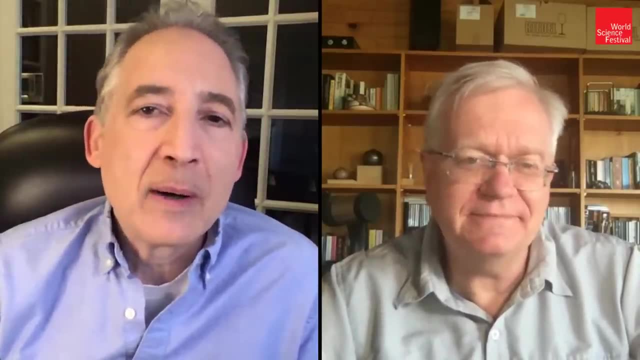 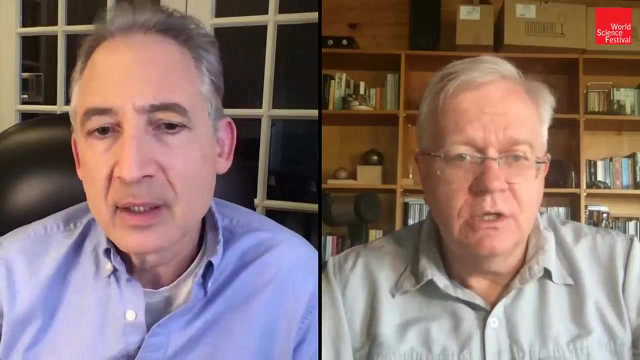 that we had here. that feels pretty significant. it doesn't normally panic and ask scientists for help, but it did in this case and we're all very grateful. yeah, absolutely so. are you now planning um remote classes or are you not at that stage yet? no, well, we are. our classes on campus are happening right. 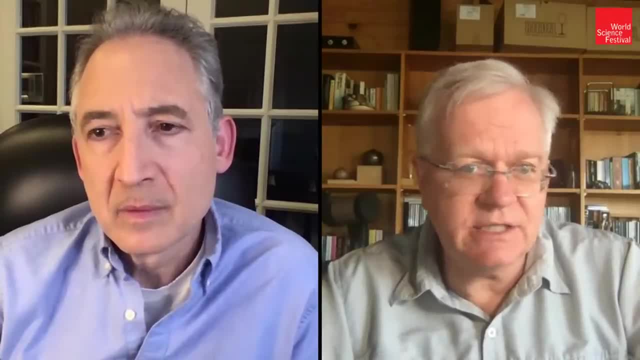 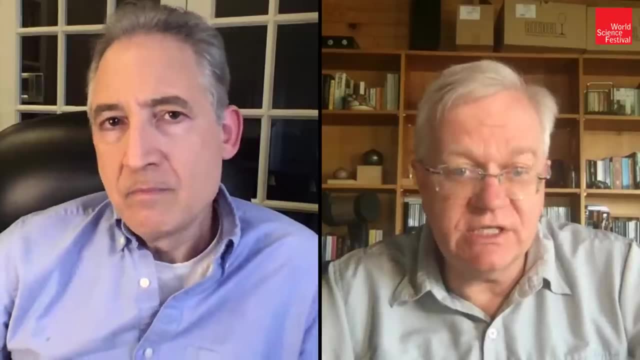 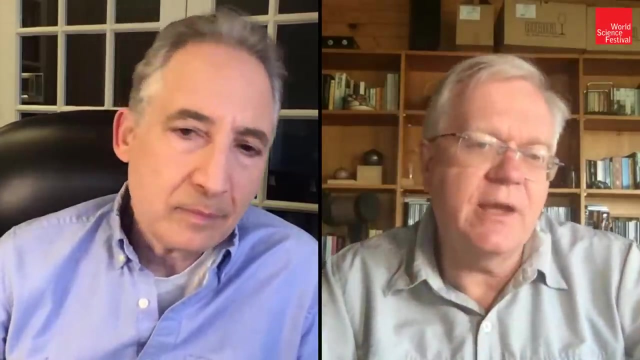 now we are open in in class classes as per normal. uh, we do have a large number of students who are stranded overseas because our borders are closed, and so we are sort of having to run two streams. so we have the online stream and we have the on-campus stream, but the on-campus stream right now. 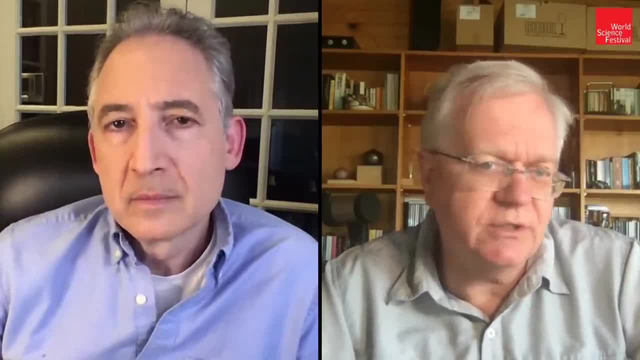 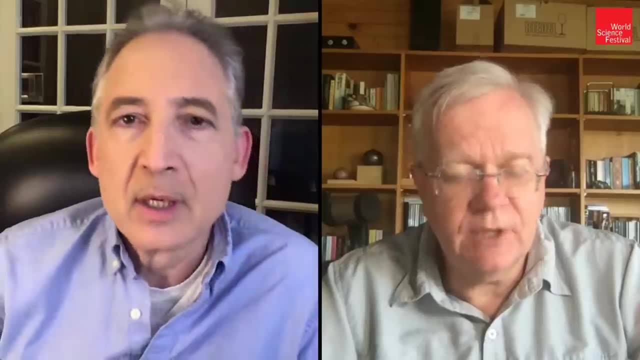 doesn't have as many students as we have every year, and so we've moved over to the online stream, and here we are in our first one streaming on campus, and it's a different experience. we have a lot of the same people as we do on campus today, so that's a very unique experience. 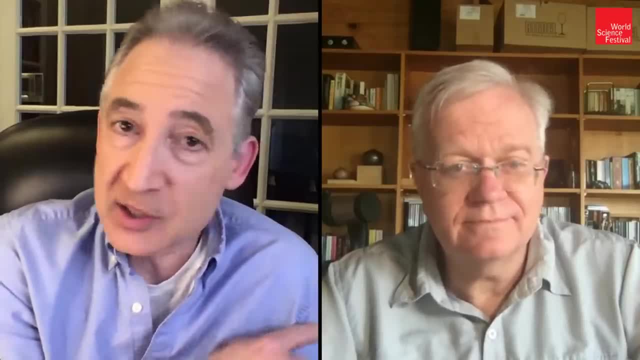 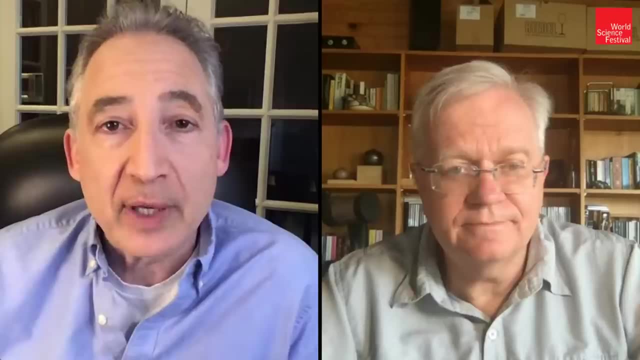 but we've been in the same chat room with many of the universities in our uh country and i think that that's a little bit unique, also in the fact that, as you said in the last recording, the next thing we heard was that there was no masks. no masks: there are restrictions of numbers of people. 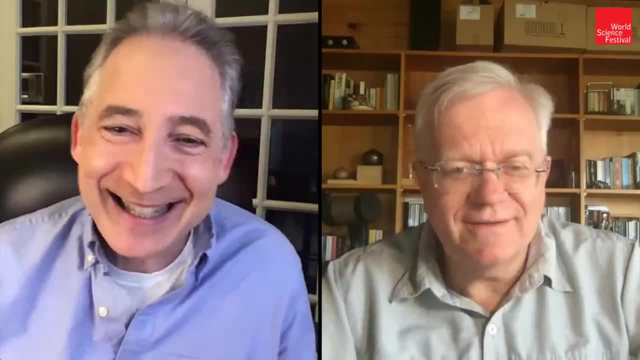 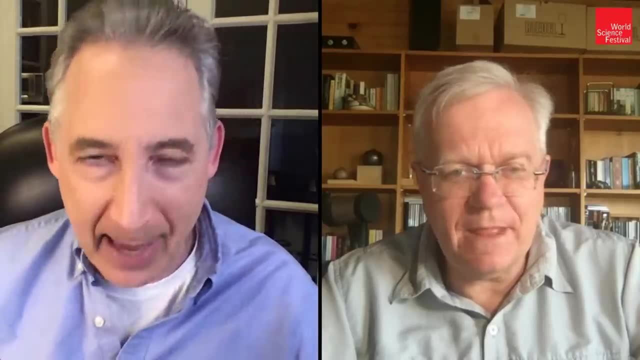 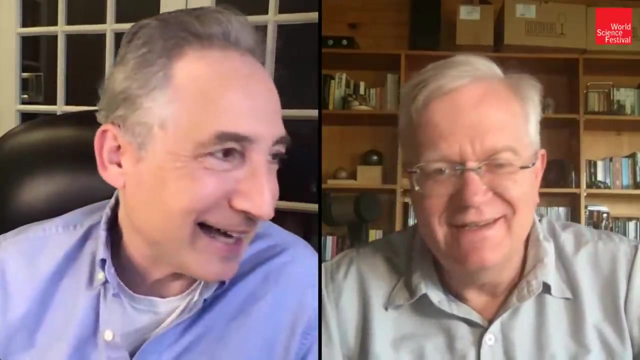 he said for 364 days. he only recently, uh, left, uh, so, uh, that could have been our situation, just by a couple. not that it would have been bad to be, i promise you, australia is very good at having people leave the country, not so good at letting me. yeah, right, right, exactly, um, but look we're. 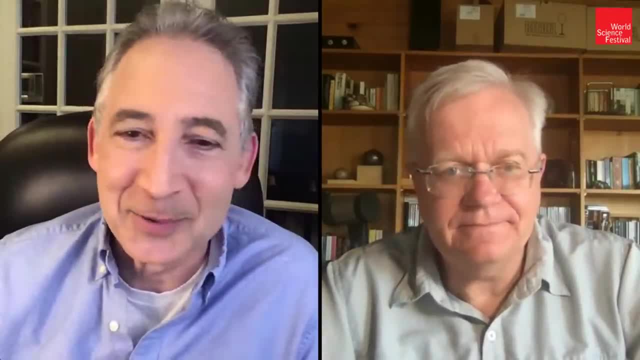 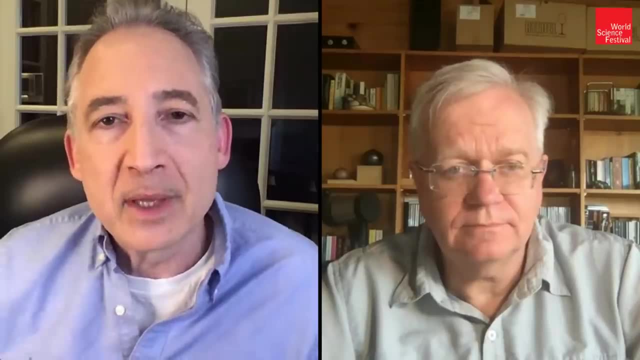 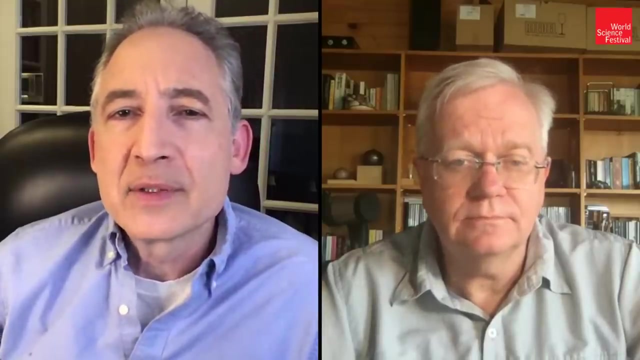 looking forward to coming back- uh, next year, assuming the world will be at that place- but i thought that we'd do here, if it's okay with you. i obviously would like to talk about some of the vital work that you and your colleagues have achieved, but we often spend a 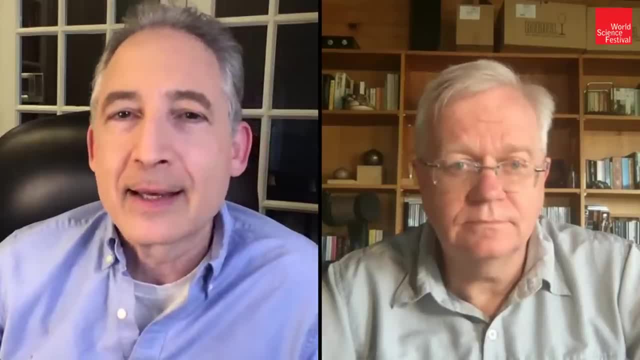 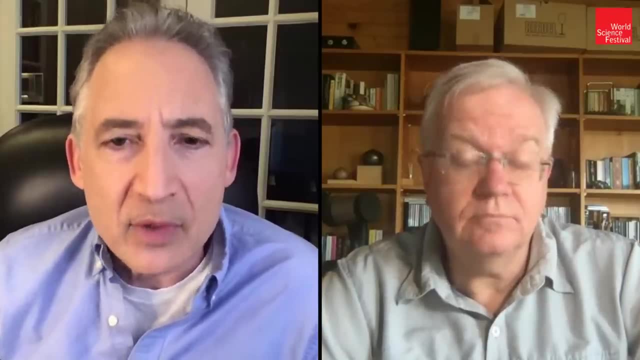 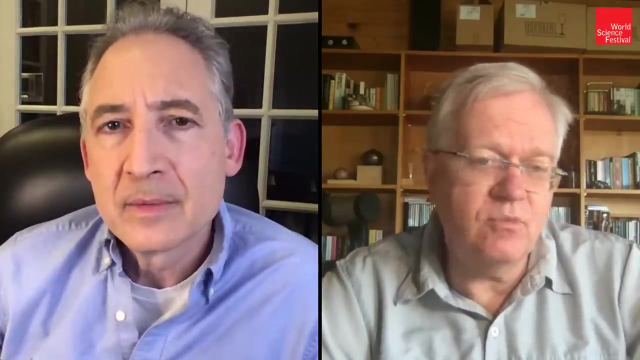 little time on the journey that got you to the place that allowed you to do that work. and you know i, you know, i know that you, you grew up in america, obviously, even though you're in australia. it was montana, is that montana and alaska. so i lived until i was 13 in montana and then moved. 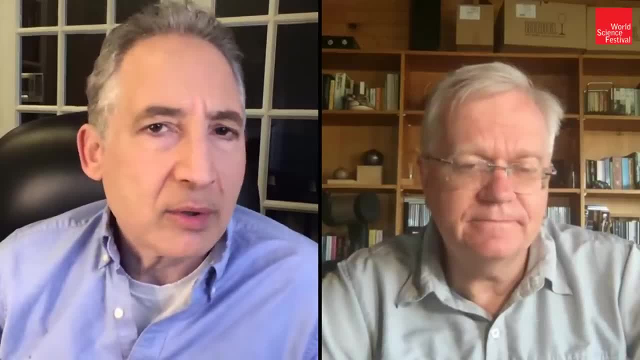 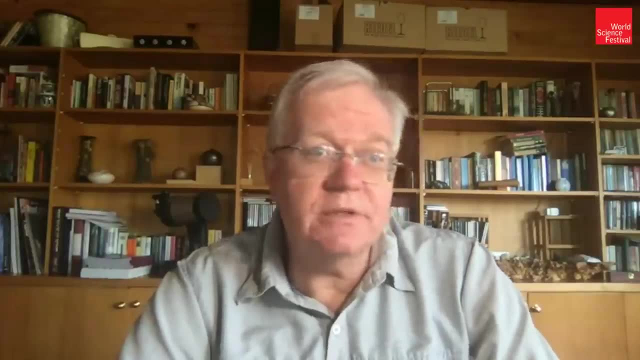 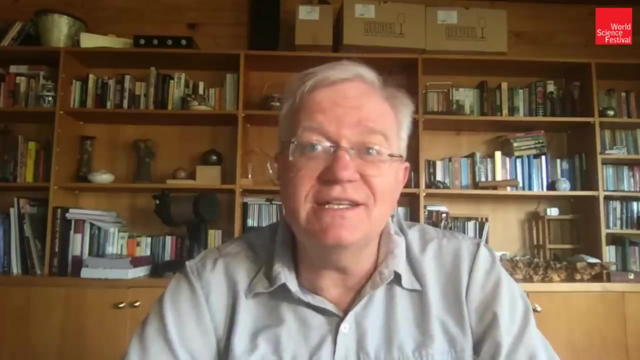 up to alaska. and was that? your parents work or what? what drew you to alaska? uh, yeah, so, uh, my dad grew up in, my mom grew up in eastern montana. they met- i was what they call a sophomore surprise- uh, at the university of montana in 1967. 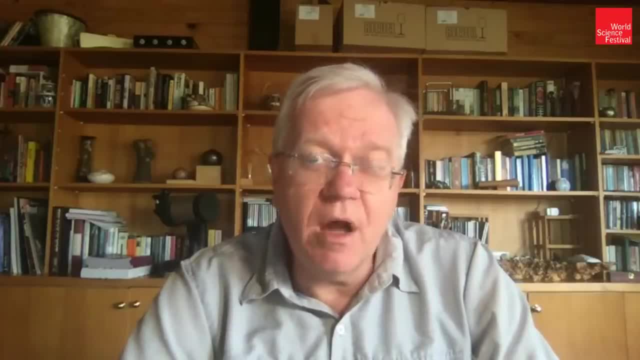 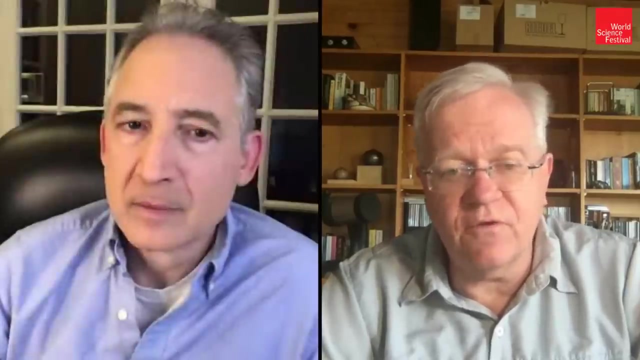 uh, and then my father was a biologist. my mother, uh, did a number of things. you know, had a master's degree, and so we lived with my father doing various biology work, uh, until we moved up to alaska and my father ended up, uh, working first on a big project up there with respect to a dam. 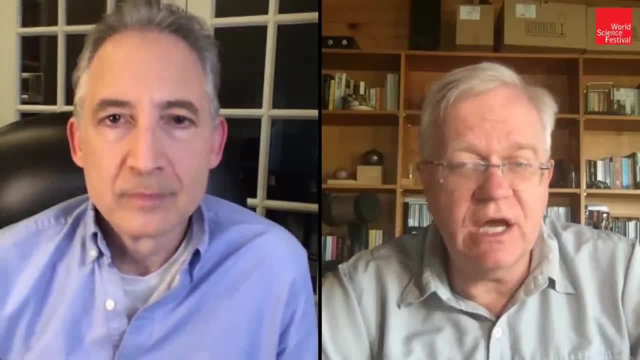 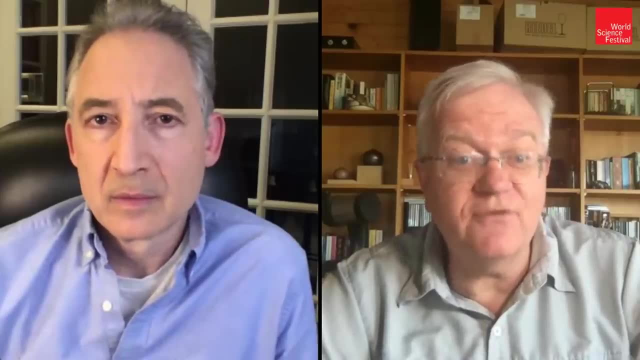 that never happened, but then he went on to become effectively the uh state fisheries biologist for the state of alaska, ended up leaving the state when he uh upset the governor by shutting down the salmon fishery, which is you know? that is i don't know. there's nothing worse. you can do it's. 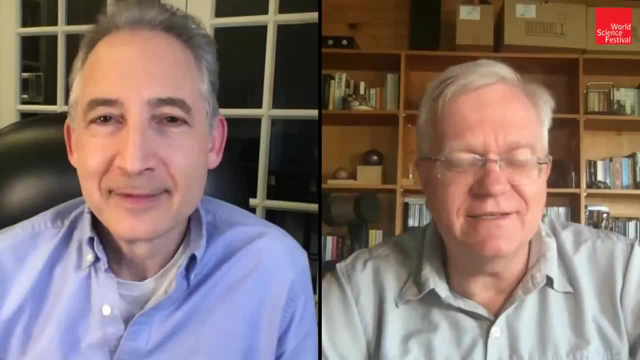 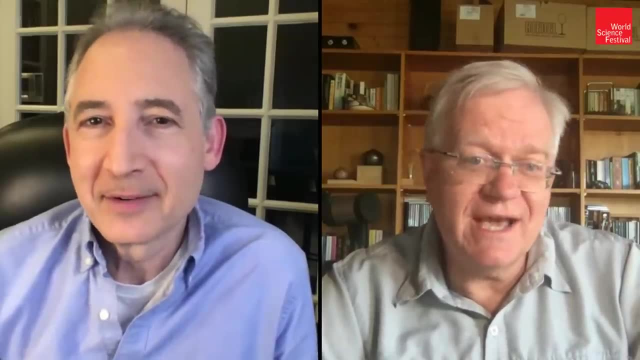 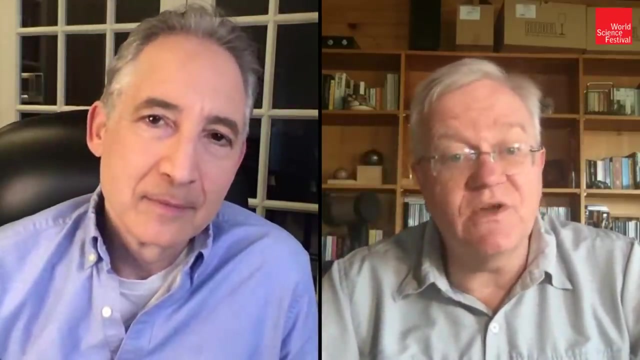 like you know, trying to have an uh in indiana to shut down the basketball team. it's. why did he do it that? what was the motivation? well, the motivation is is that, uh, you know, salmon come in and have variations each year and they have returns. it was very clear it was a very poor return. 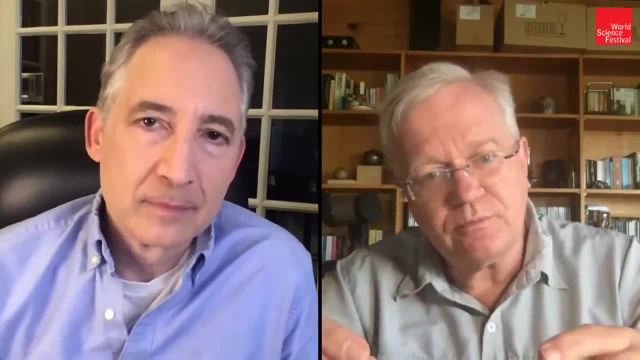 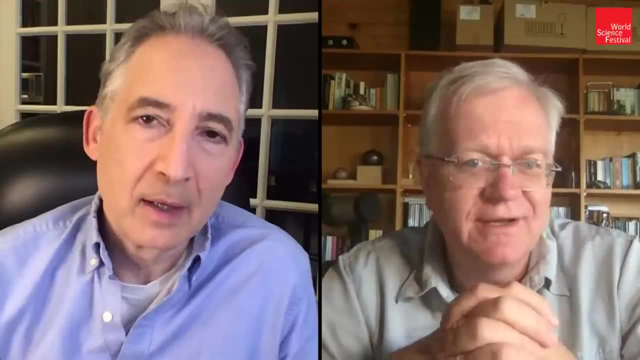 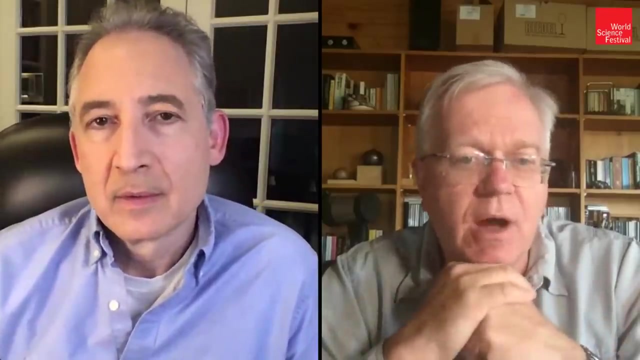 and so that if you don't let the salmon through, then, uh, you end up killing the run later on. and so there is, you're trying to his. his job is to optimize, yeah, uh, for the number of salmon in in castles, and he finds, uh, at least one, uh, as some of the ones that have arrived at costa valencia. 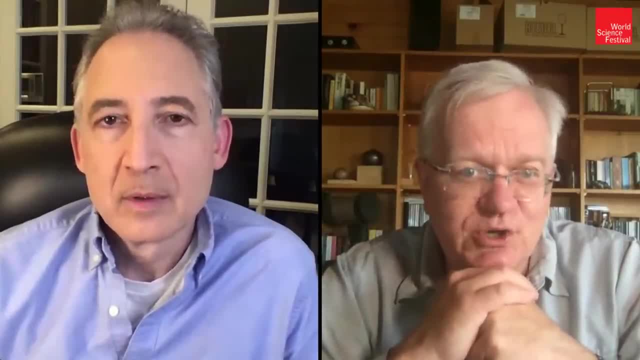 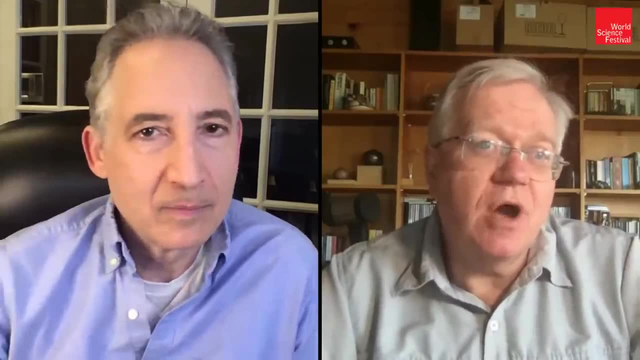 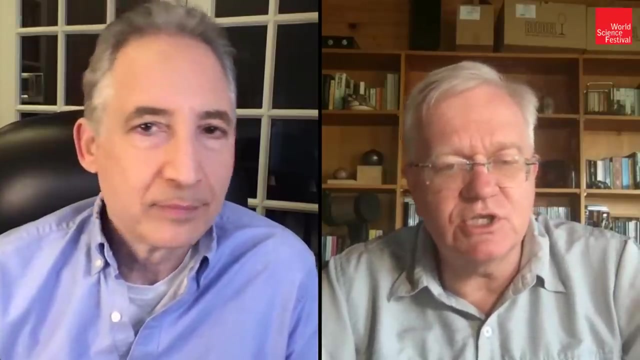 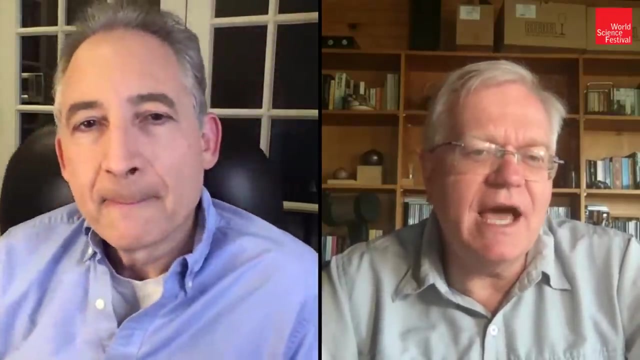 africa. but uh, you support, you support the scales and uh, for the benefit of the general population, what, um, what totally saw on a commercial fisheries who get it? but it was the, the fishermen on the shore, you know the, the, the non-commercialuch. yeah, were they like: do they try to run you out of town or anything? i mean, was it uncomfortable? well, i mean, this was after i was already, uh, in, you know, actually finished my phd. so well, they just, you know, they, they do it as politicians, do they shut down his lab and all the other animals. yeah, well, he decided my dad is not a politician. 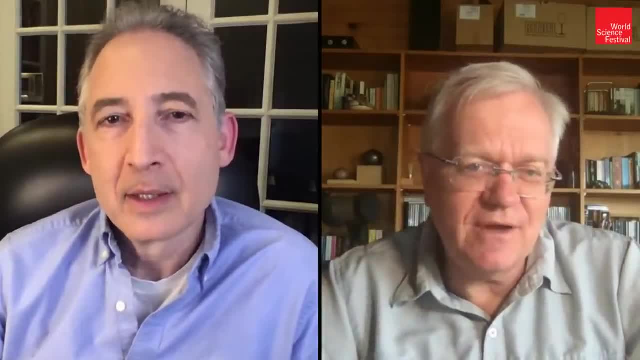 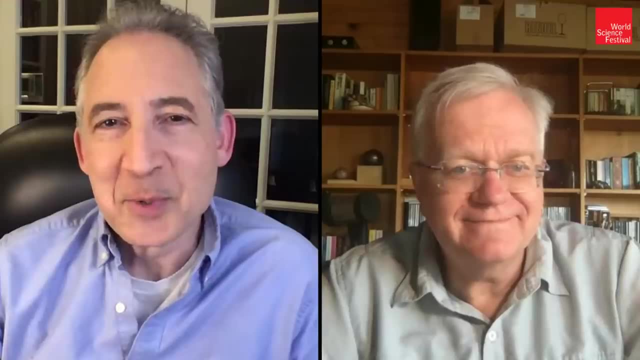 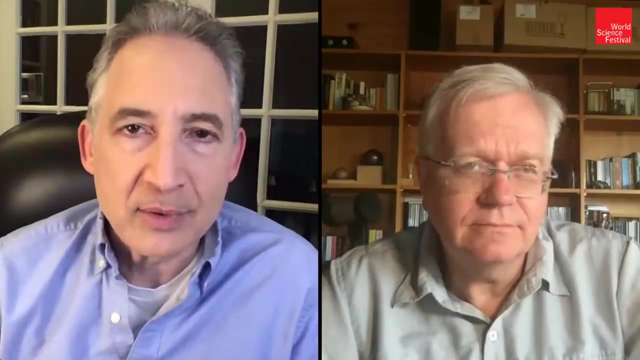 politician. He's just, you know, straight down the line, fisheries, biologist And anyway. so he immigrated to Canada after that. Probably a wise move. So did you have any interest in going into biology? Was that ever in the cards or it was always more in? Yeah well, I always knew I was. 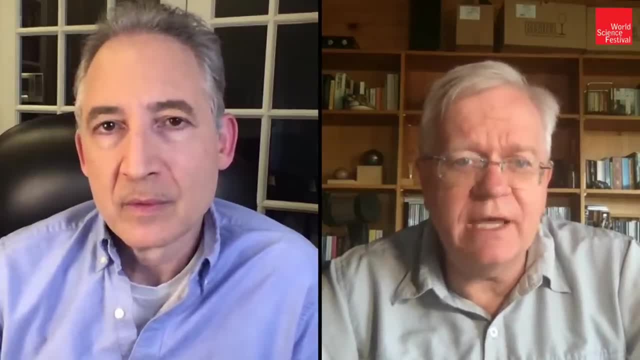 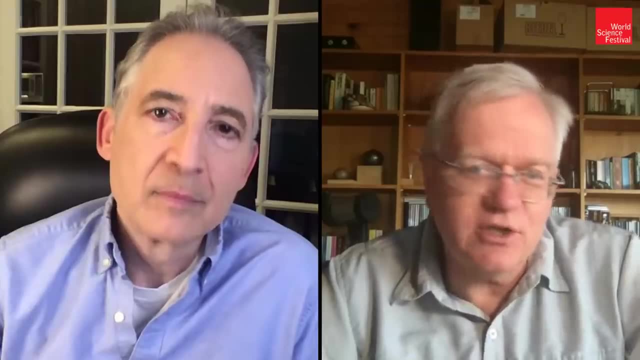 going to do science And you know, I grew up with my dad because I was born when my parents were 19 and 20.. So I, you know my dad, had childcare duties and I used to go into the lab with him. 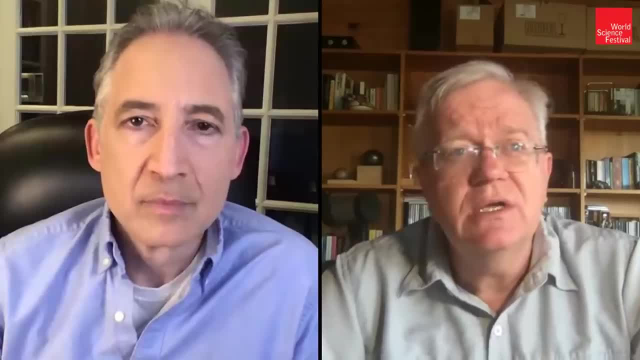 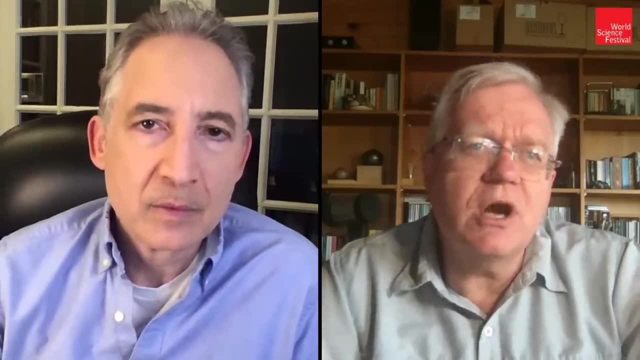 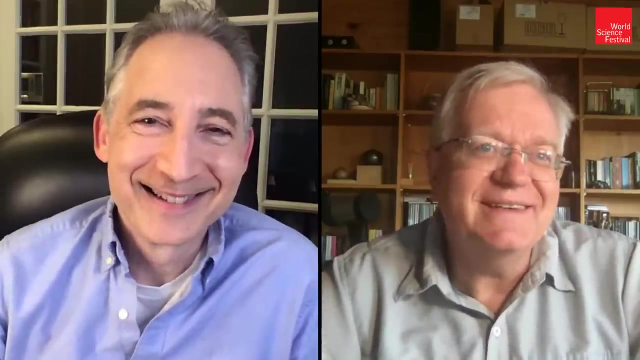 an awful lot when he was doing his PhD. So I was. I was around the science. I always gravitated to physical science, though Even from a young person I was pretty sure I was going to do meteorology. I just love the weather. I still love the weather. I'm just fascinated by it. 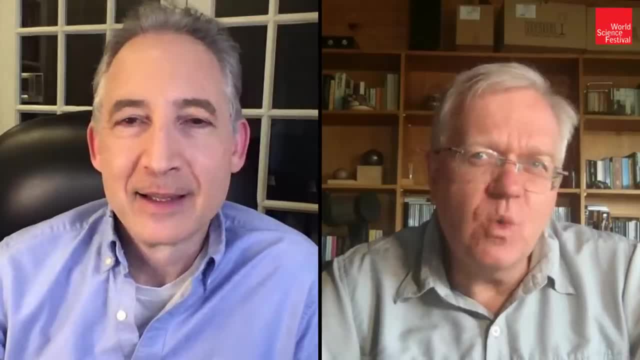 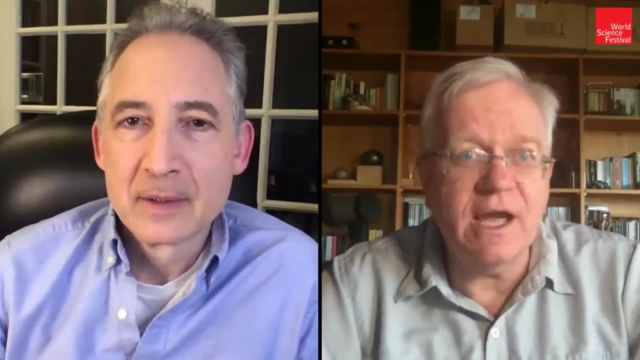 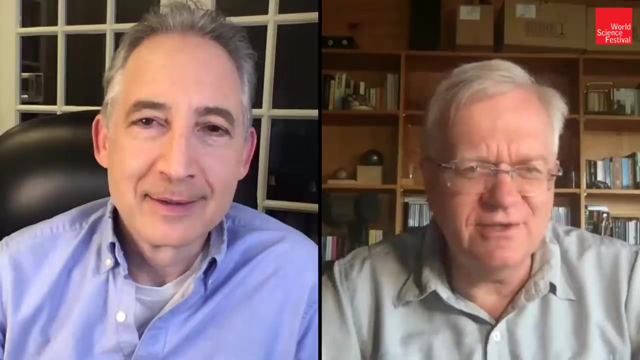 And I'm a weather freak, But I always wanted to do that. And then when I was 16, I volunteered to work a summer at the Anchorage Forecast Center, which was sort of my dream job, But it was all the information and science came down from Oklahoma and you just kind of went and 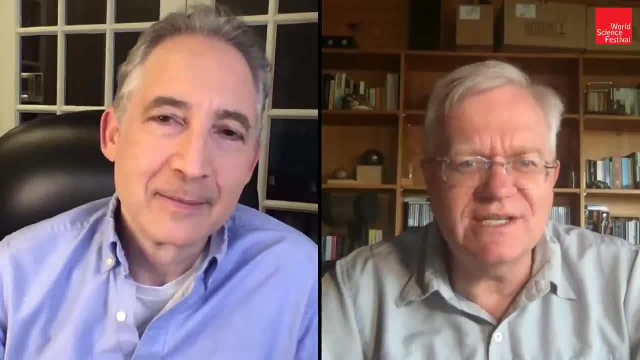 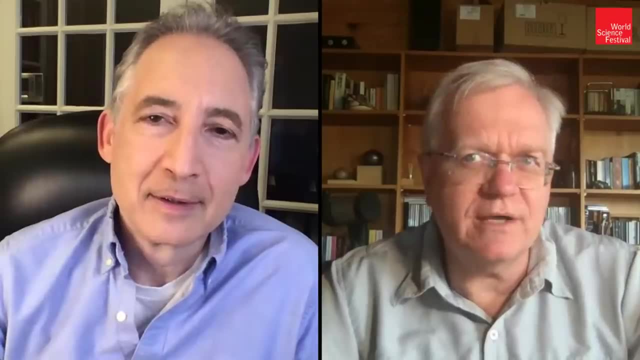 read forecasts and stuff And I didn't find it what I was expecting, And so I was suddenly like my God, what am I going to do? That's not what I was thinking I was going to do. Now, in retrospect, all of the stuff I wanted to do, which is to actually build the models and stuff. 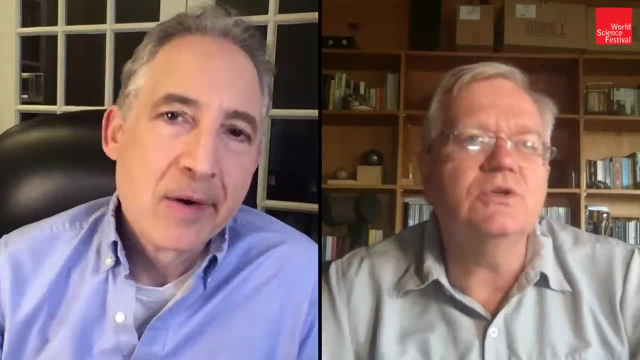 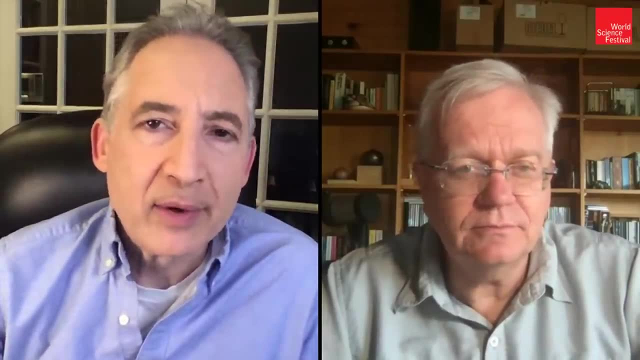 that came out of Oklahoma. that would have been exactly the type of thing I would have done. That's the thing I wanted to do, But rather I went and did astronomy and physics instead. But it's interesting because you know when I think about the weather and meteorology. 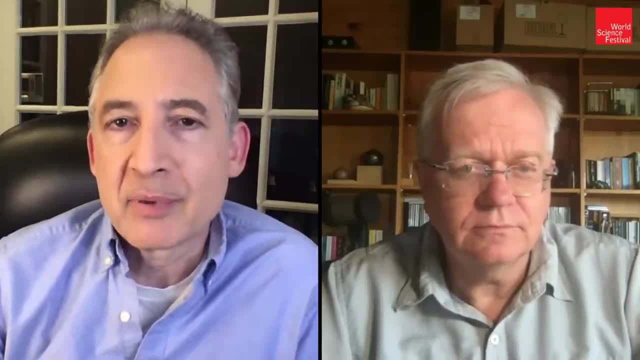 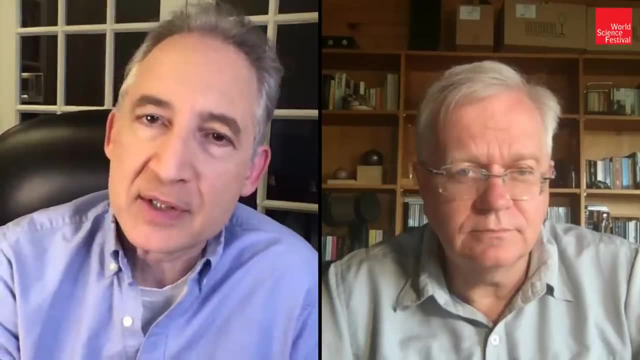 it feels like such an incredibly complex problem that, applying fundamental physics to it, we've made headway on it. But compared to the fundamental physics that's so clean and relatively simple of cosmology and astrophysics- simple astrophysical systems- it seems like 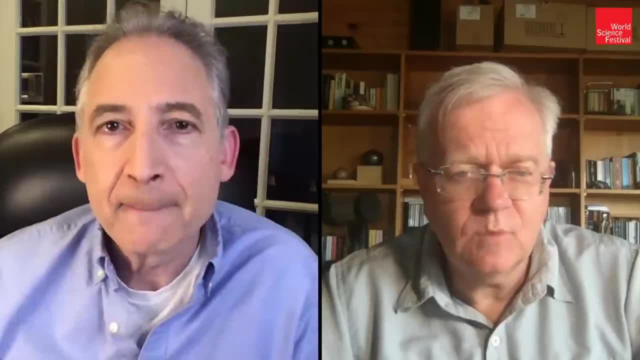 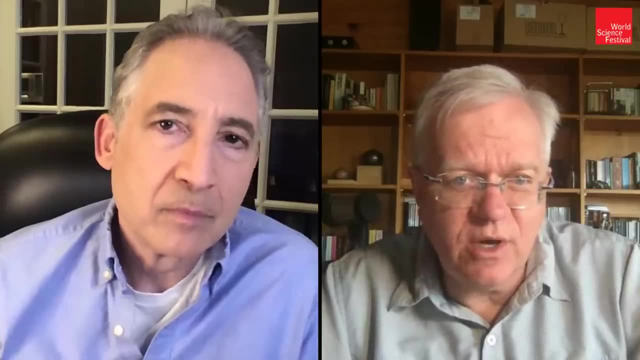 they're almost a universe apart from each other. no Well, I think they're equivalent to people who work on doing giant star formation simulations, where you've got the hydrodynamics mixed in with the simpler bits And you know it's essentially. 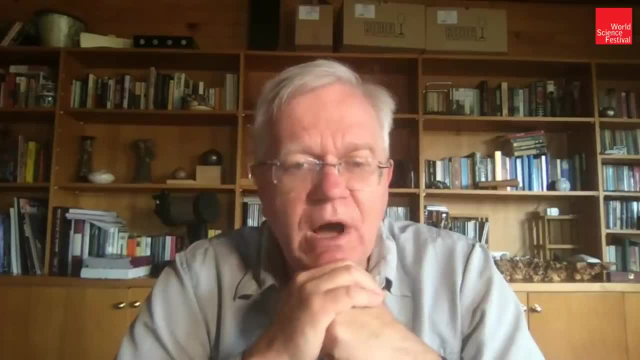 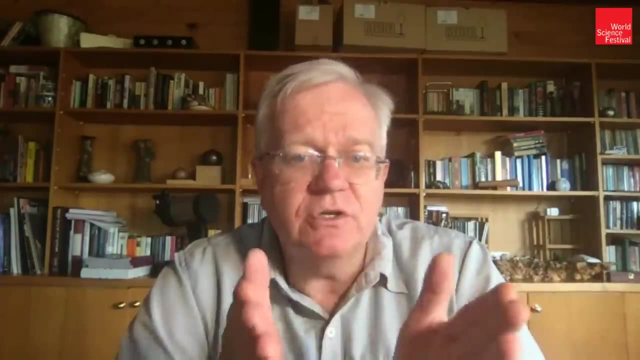 the same physical equations between the two And I don't mind a little bit. And you know, with respect to you know some people will know that I have a vineyard and a winery here. I use now 14-day forecasts for looking at rain. 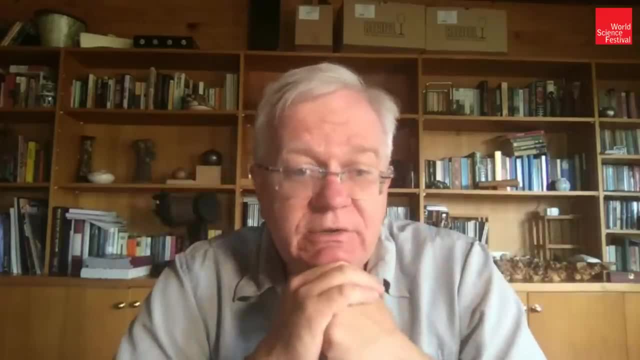 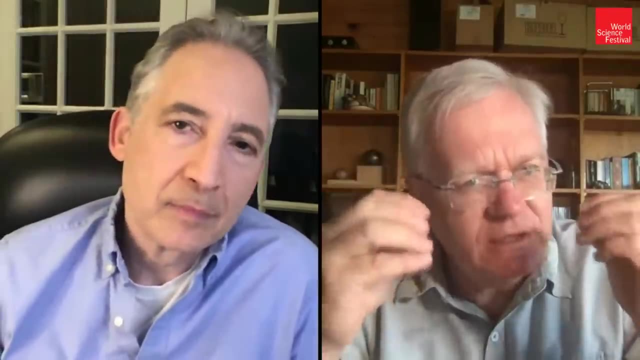 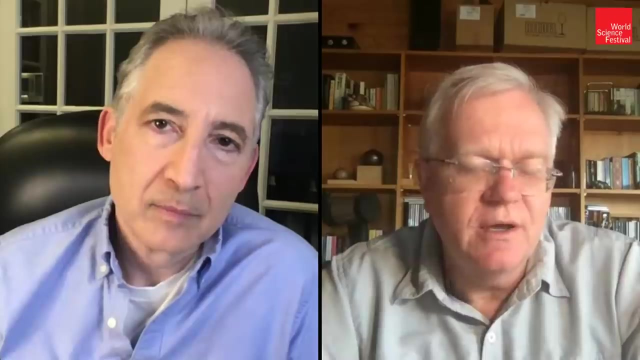 and precipitation, which are 85, 90% accurate. Now, 10 years ago they were useless. They didn't even give them to you. They were useless. So they've made a lot And it's computational grunt. In the same way, you know my guys up at Stromlo who are doing star formation stuff. I mean 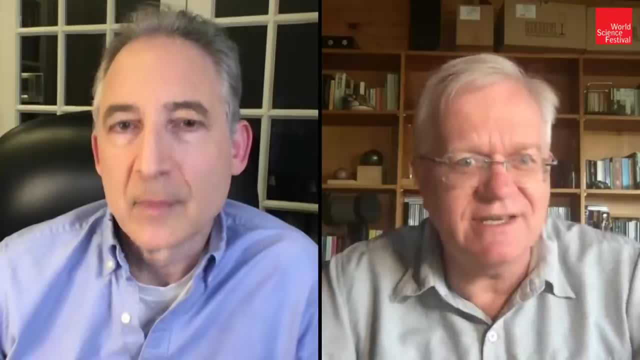 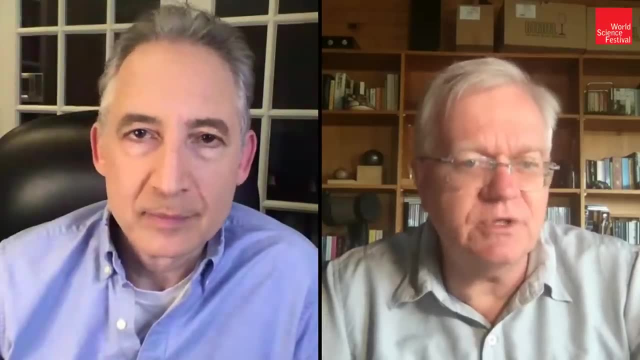 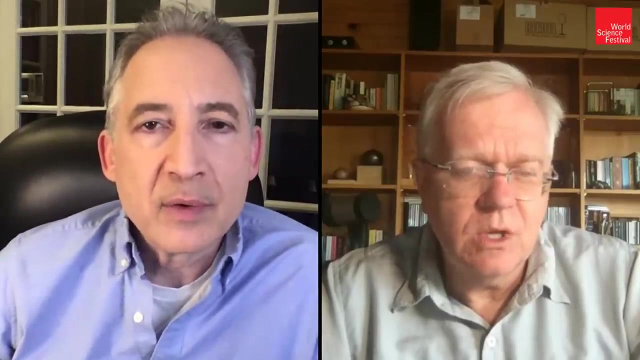 honest to God, when they put together a galaxy now it looks like a galaxy, as opposed to some little toy model. It's pretty frightening, But that physics and lots of computational grunt gives you Yeah, yeah. And so what did you do your PhD on? What was the focus there? 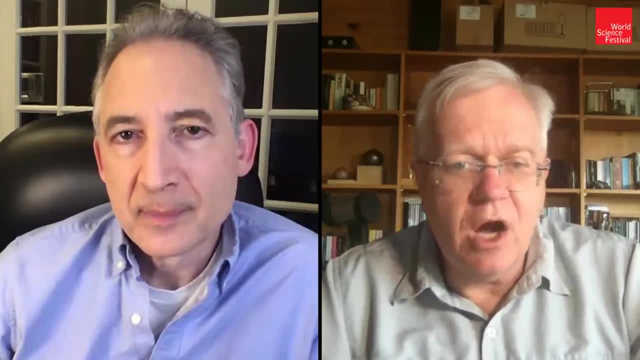 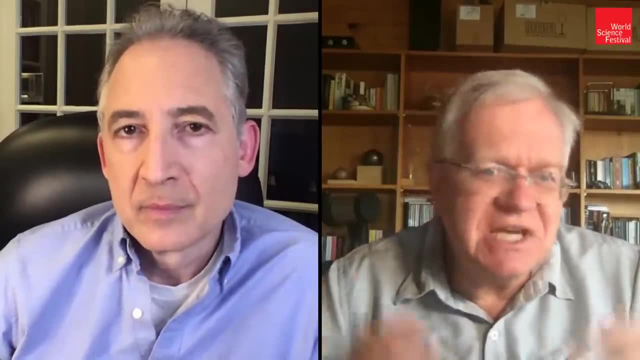 So I did my PhD at Harvard on measuring distances to type 2 supernovae. These are the massive stars that live for, let's say, 10 million years. They're often 10 to 20 times the mass of our sun. 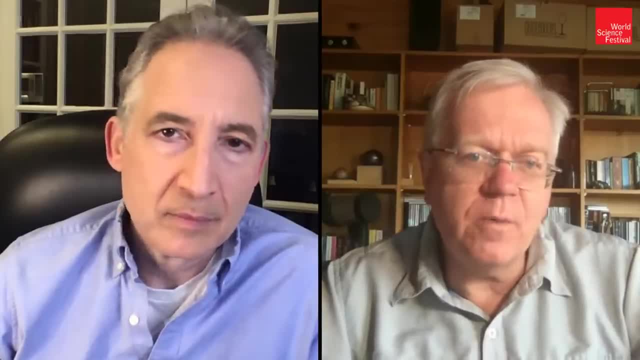 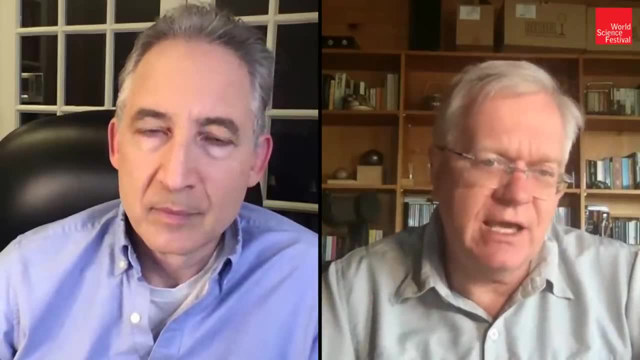 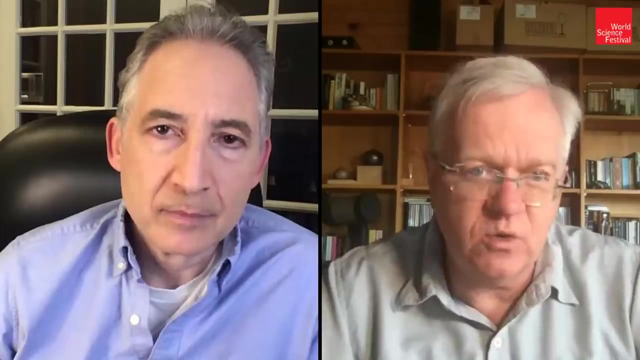 And at the end of their lives they form a neutron star or possibly a black hole, probably Probably both, And as they collapse you get an essentially a shockwave. It's a little bit of bounce, but it's probably a lot of neutrinos, which normally, of course, go right through the Earth. Things are so dense at that neutron star that they- actually, the neutrinos- end up blowing the object apart. Quite remarkable. And you know, these are the things that make most of the interesting elements: oxygen, carbon, iron, Those things. 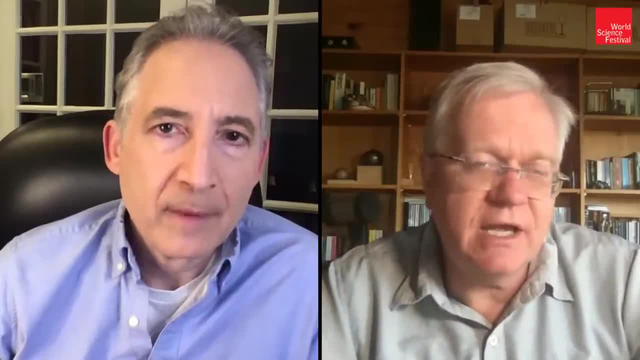 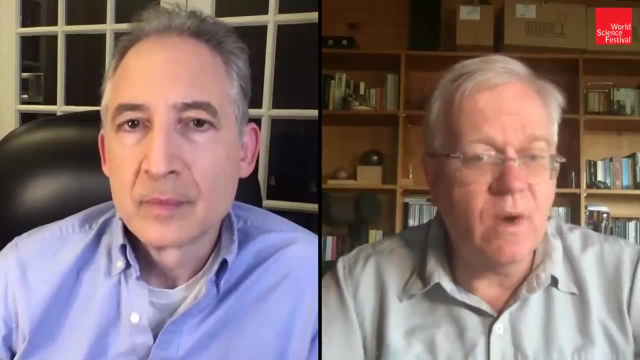 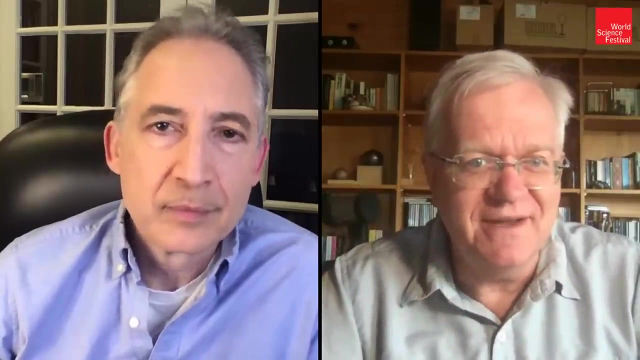 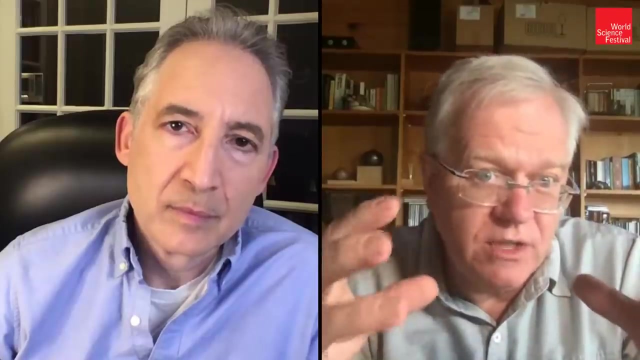 they're all dispersed and created in these explosions And I was able to use them to measure distances in an absolute manner where you actually modeled the exploding star using those weather-like equations- pretty messy, actually, relative to cosmology equations- And we could essentially figure out how many watts they were, how big the light bulb was. 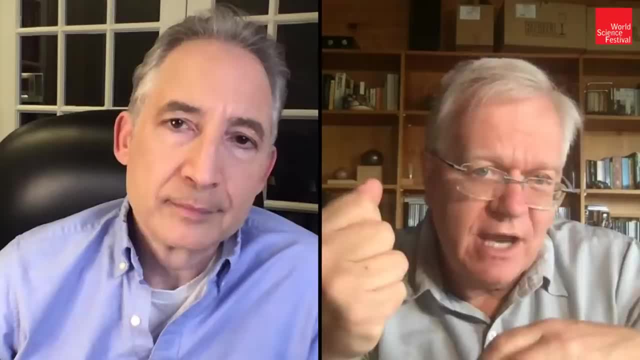 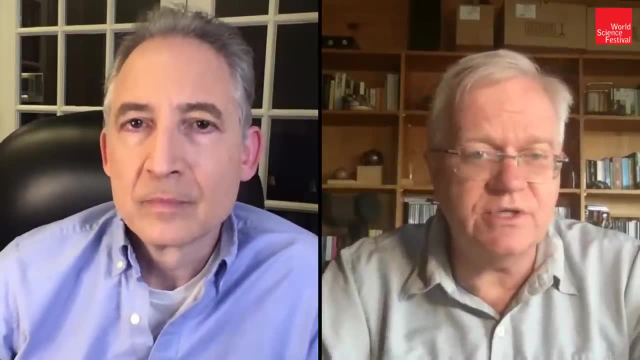 And, of course, if you know how many watts the light bulb is and you know how bright it appears- it gets fainter the further away it is- then I can read off the wattage, measure how bright it appears here and measure the distance. Yeah, And so I was trying to measure the Hubble constant. 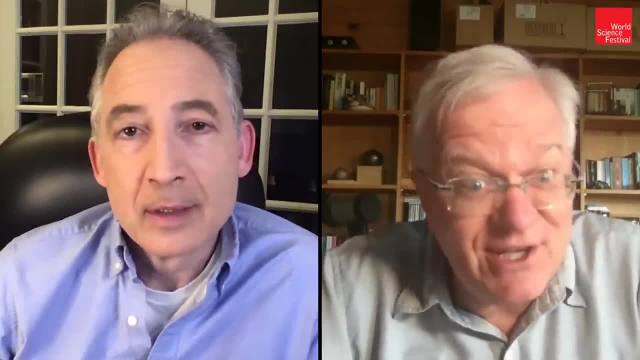 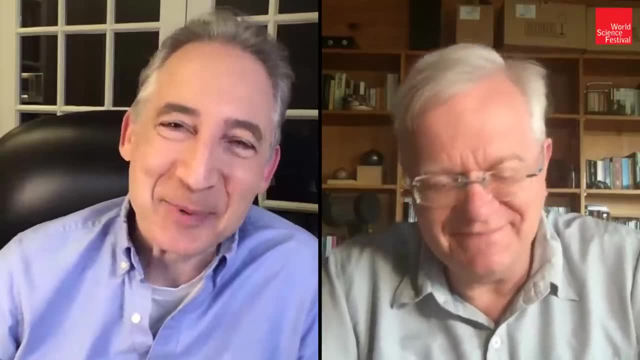 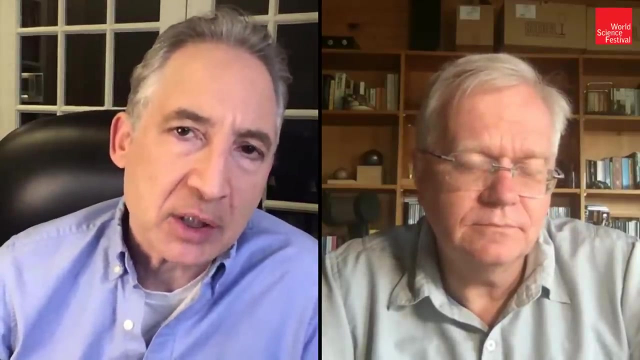 which I did, and I got an interesting number, which was 73 kilometers per second, per megaparsec, which I'm proud to say is exactly what Adam Rees is still getting all these years later. That's pretty good, Absolutely, And so your work then was a blending of observation and 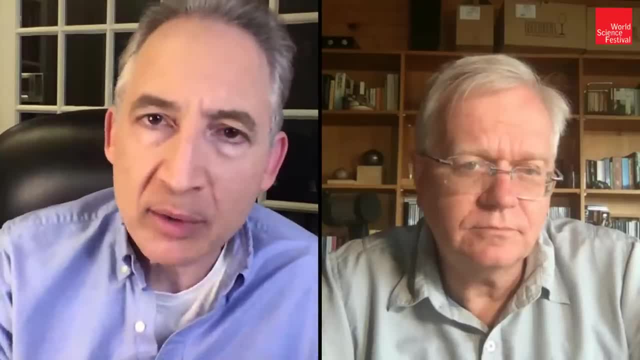 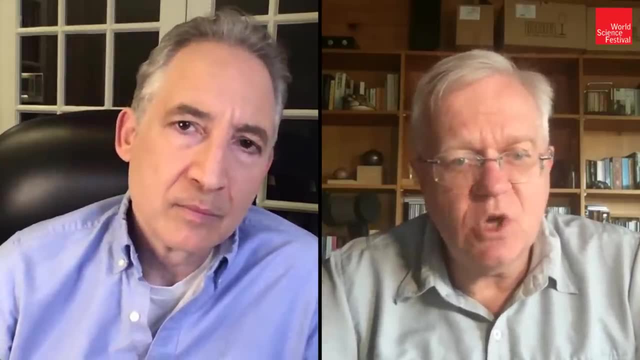 simulation and calculation. Yeah, And so I was trying to measure the Hubble constant calculation, or did it skew one way or the other among those elements? Well, you know a lot of good things in life you do as a team. So, Ron Eastman. 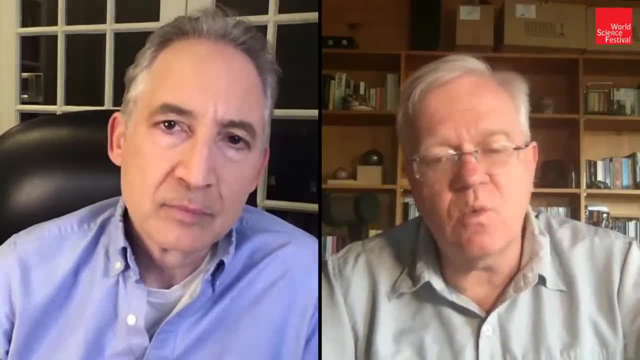 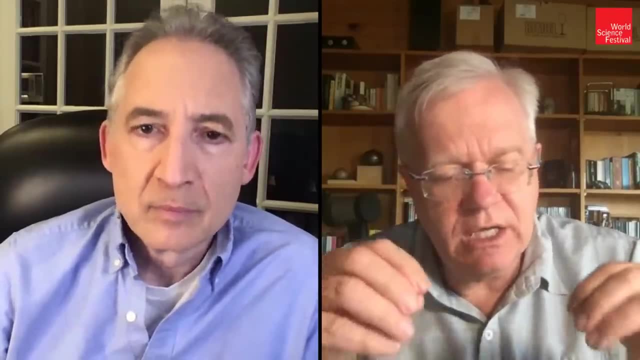 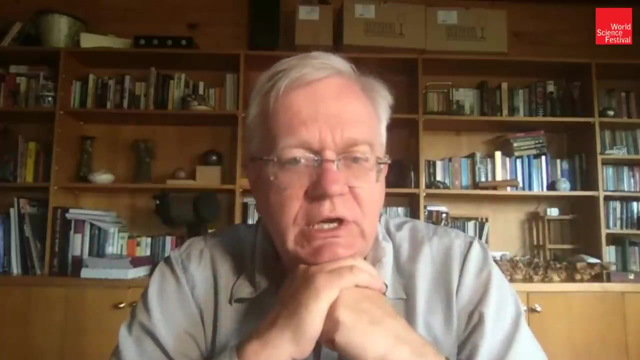 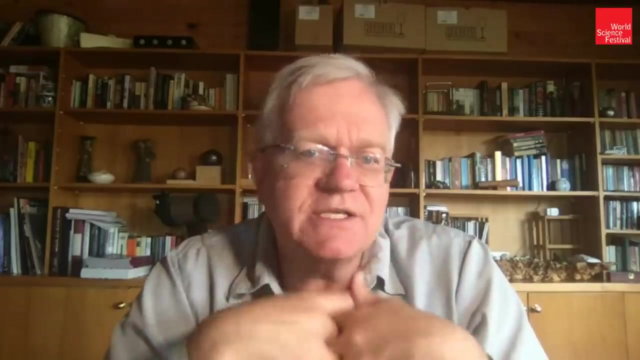 and Bob Kirsten being my PhD supervisor, Ron Eastman, who is Silicon Valley area now he did most of the really detailed calculations. you know, 10 years worth of work to build a model Which had all of the right ingredients to sensibly calculate, And so I was involved. 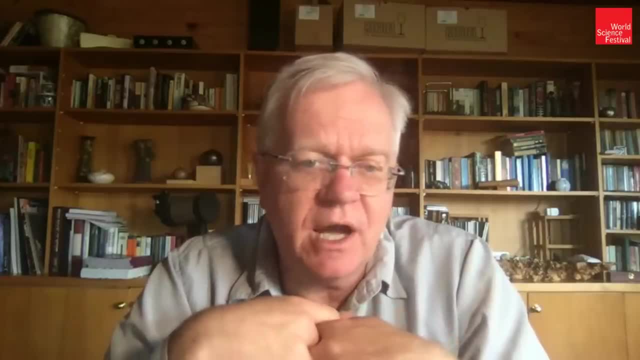 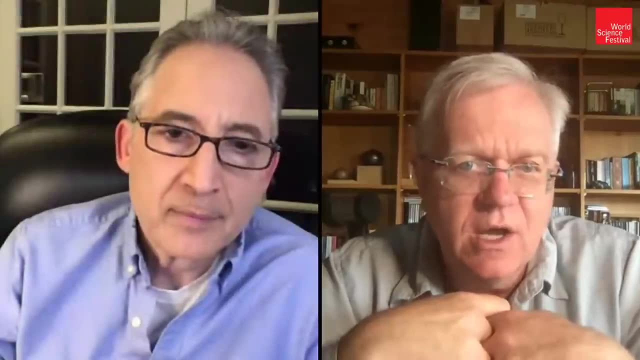 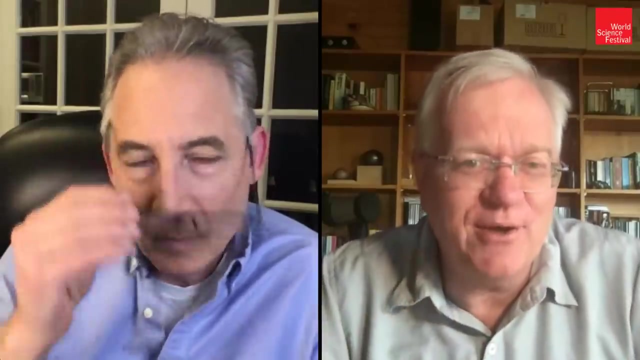 in the periphery of certain aspects of that, but I used that with Ron to do all the calculations we needed to measure the distance. So I actually ended up running more models than Ron ever did because I was so enthusiastic about using them where Ron was always trying to get the little. 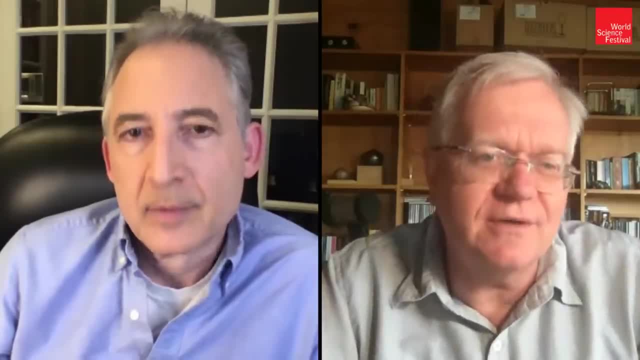 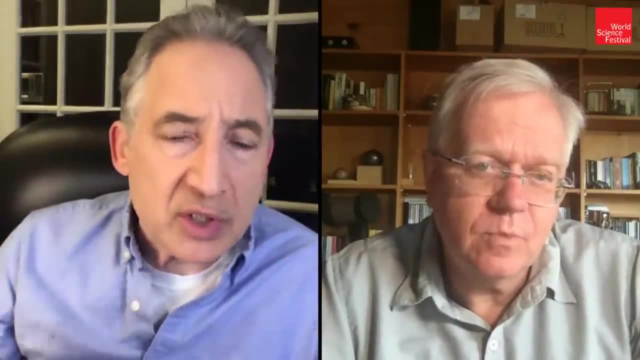 bits and pieces, right. I was like, okay, let's just go, I'm going to go back and forth and see what's going on. So we actually made a pretty good team. And so did you actually go to telescopes to do these observations, or were using data that? 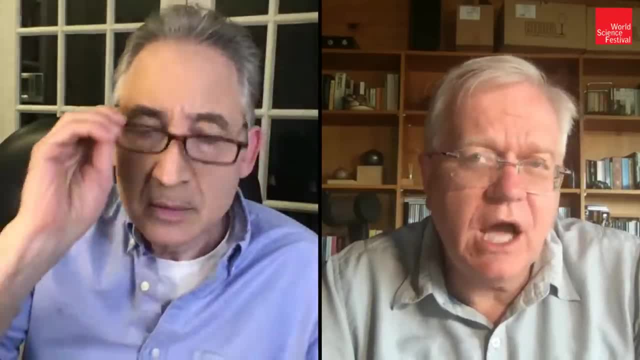 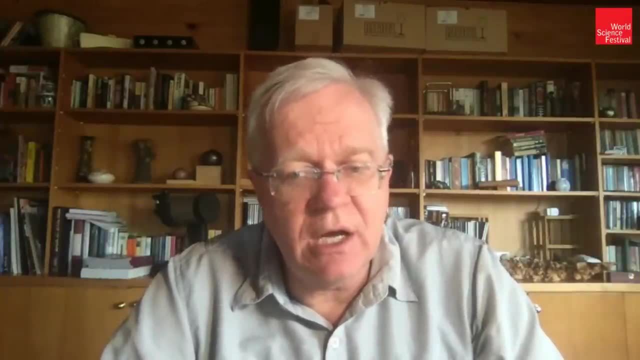 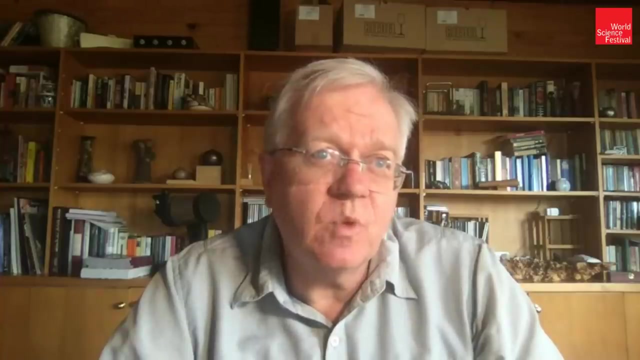 others were acquiring. How did that? how did that work out? Yeah, a little bit of both. So in 1991, so my second year of my PhD- I went and spent about two and a half months down in Chile with the guys at Saratololo, So we had Mark Phillips. 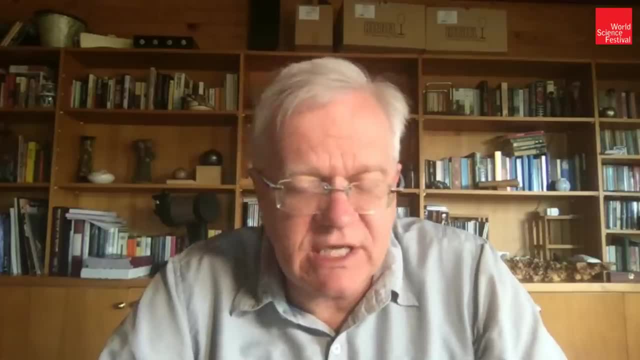 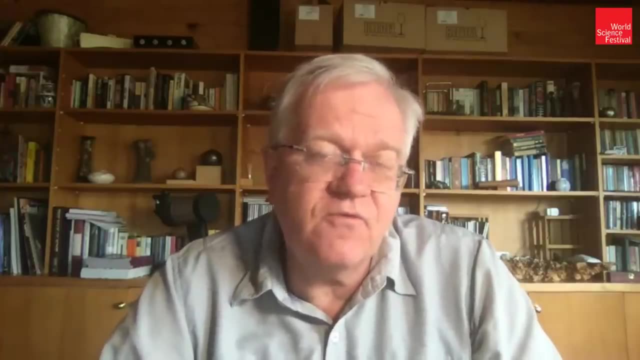 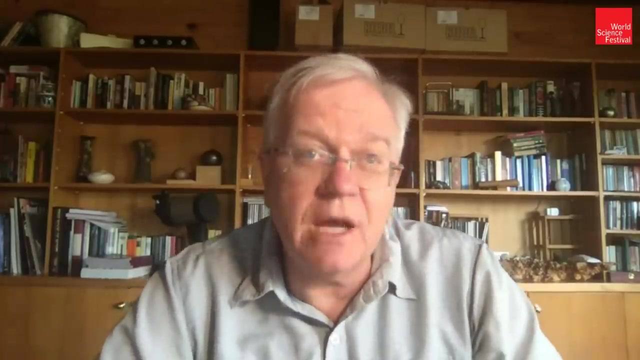 is who I was invited down, So I've been following by, but with Nick Sunseff, and Mario Hamui was there, And so they had gathered a bunch of data for the Kallon-Tololo supernova search, which was really targeting the other type. 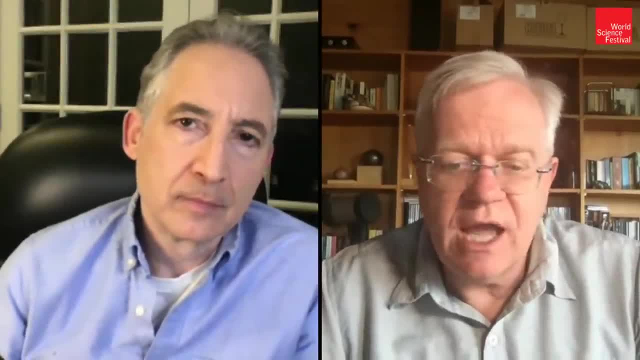 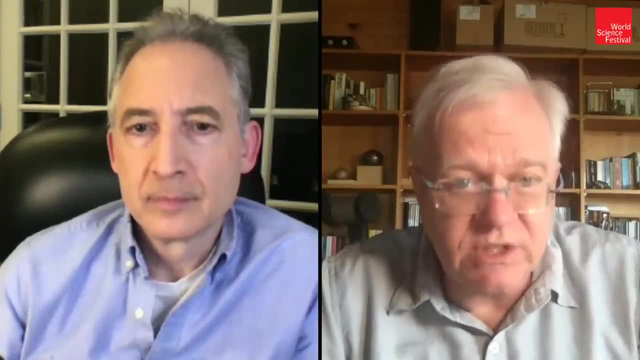 of supernovae type 1a supernovae, which are the explosions of white dwarfs, And so they had these little other things type two supernovae they didn't want to use. So I observed down there. I reduced a lot of data. 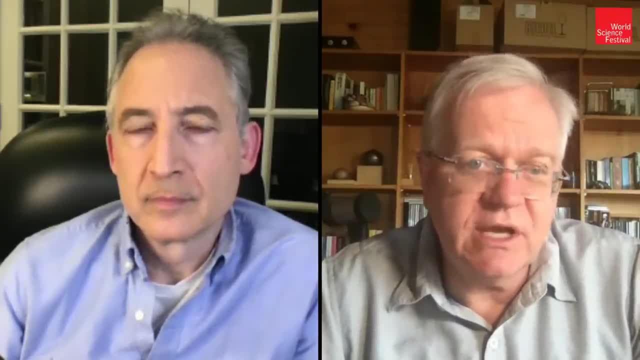 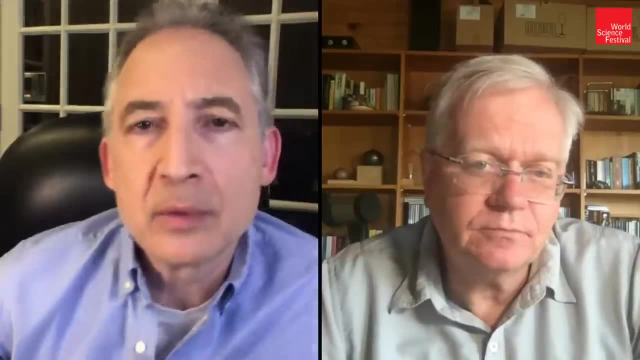 I observed a lot of supernovae up at in arizona using the telescopes that harvard had. so it was a bit of new data, a bit old data, and when did you start then to move more toward a cosmological focus? i mean, obviously, that seems. 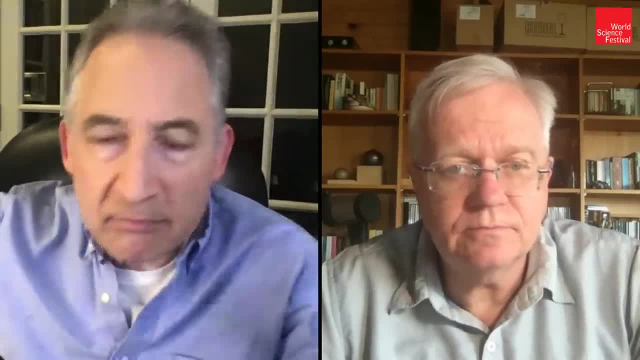 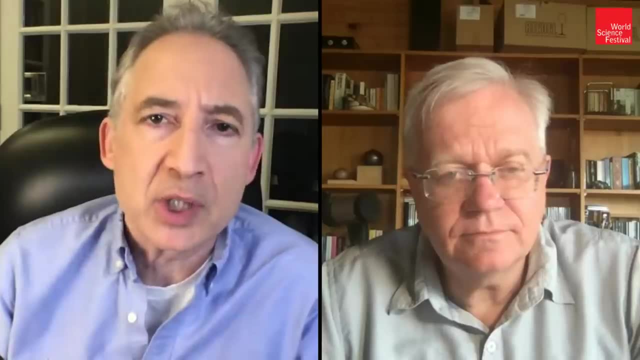 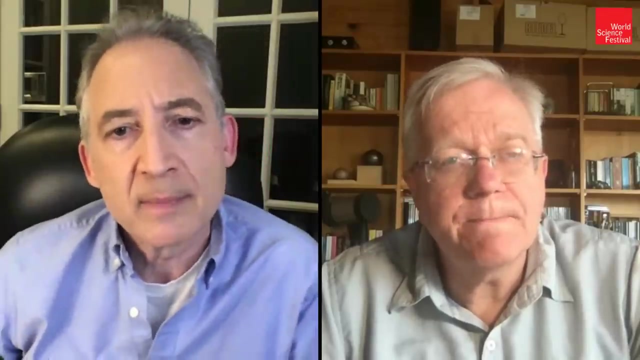 like a natural progression, because you're studying the same kinds of stellar systems. you know from 30 000 feet they're up for the same. but was there a moment when cosmology became your passion, or was it just the sort of natural progression of the- uh, the project i always wanted to do- cosmology? 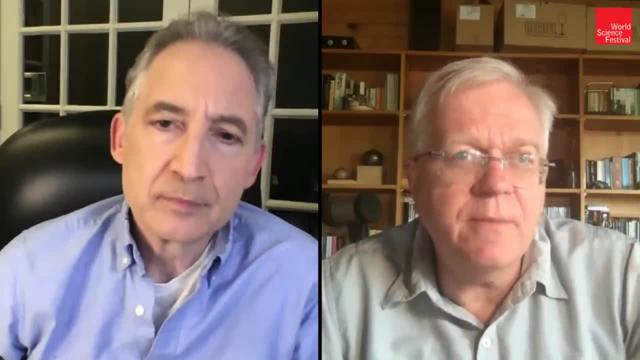 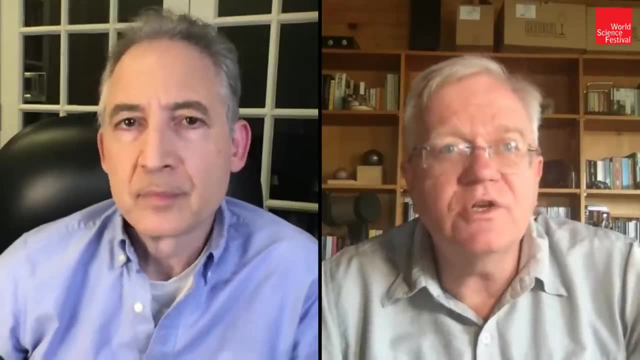 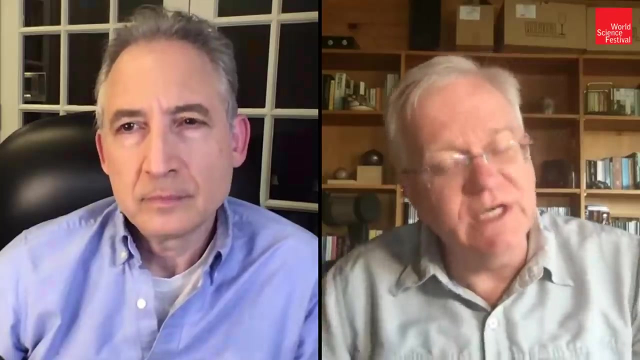 so i was measuring the hubble constant and you know, i remember when i started my phd at harvard, bob was wanting me to do an ultraviolet, bob kirschner wanted wanting me to do an ultraviolet study of supernova 1987a and i was like that's fine, but what i really want to do is this project. 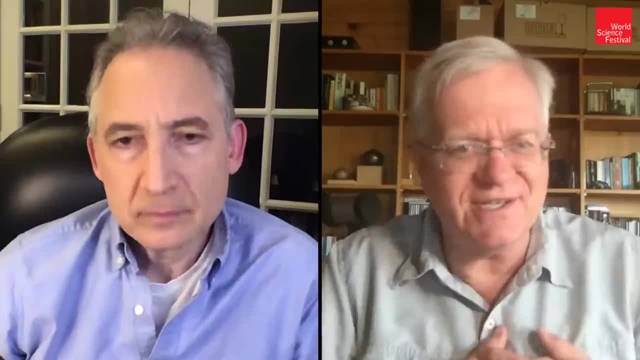 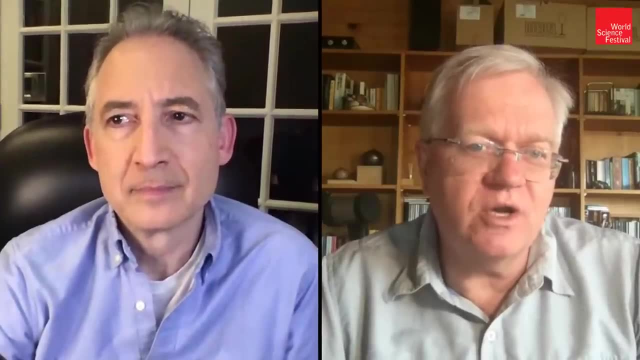 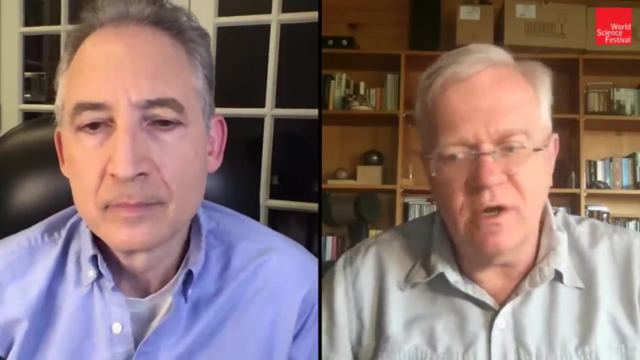 and he said: oh, that's a great project if you want to do it. it's what i did my thesis on is what bob kirschner said. so i wanted to measure the hubble constant. uh, and of course, the reason i wanted to measure the hubble constant is it was easier with the technology at the time than trying to measure. 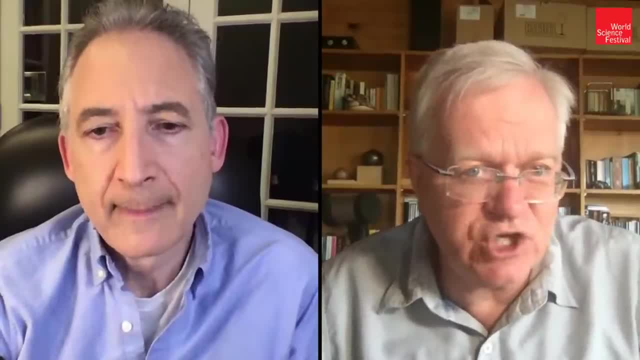 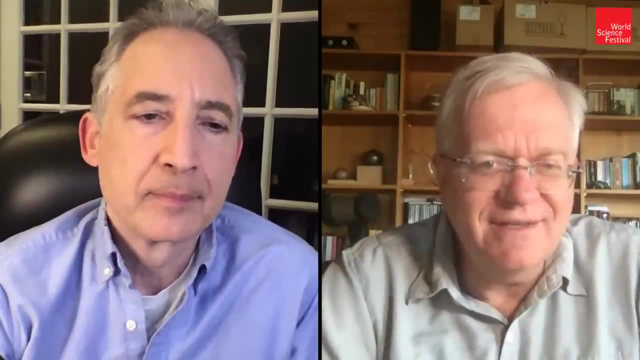 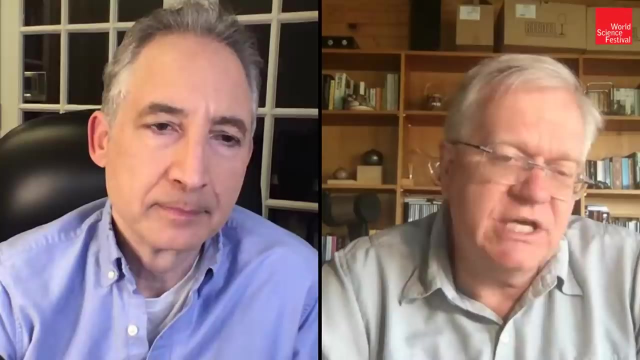 uh. q naught, as we called it, which is the deceleration parameter, uh, and. but i always had an eye to wanting to measure. q naught, uh, as you know, my ultimate goal. and so when i finished my phd, having worked with uh team down in chile, i realized there was an opportunity. uh, saul perlmutter at berkeley. 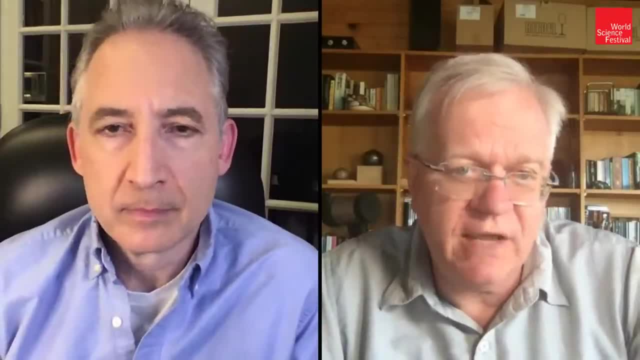 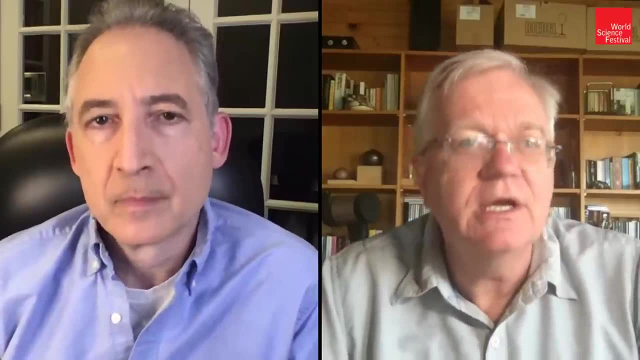 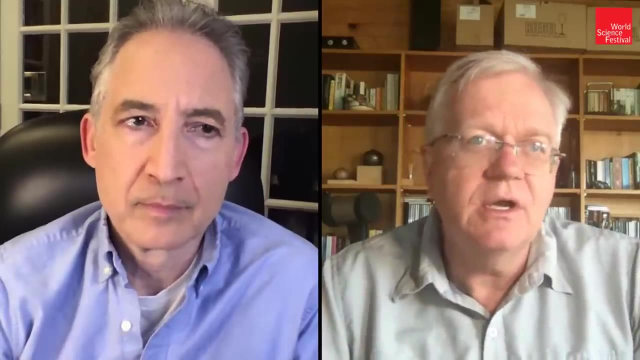 had demonstrated you could find supernovae type 1a very large distances, and my colleagues in chile had demonstrated you could measure distances with them very accurately. and i thought the supernova community should come together. uh, because we- you know, saul and his team were- 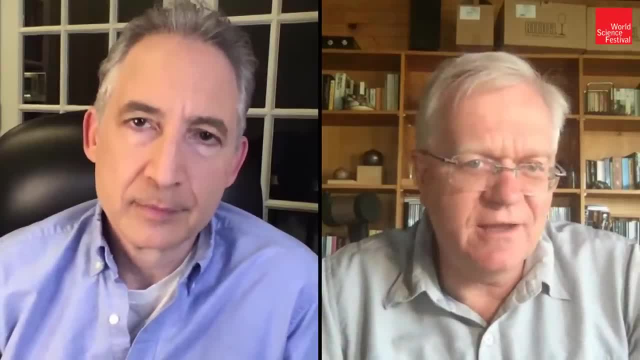 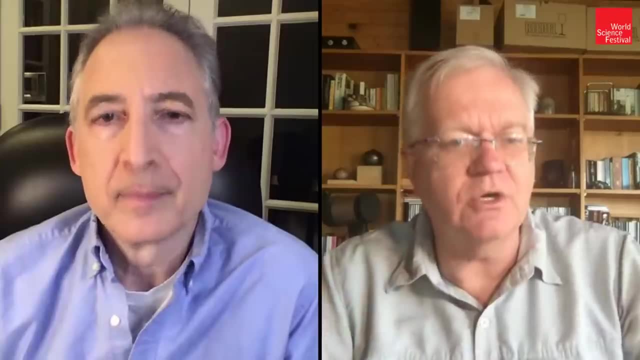 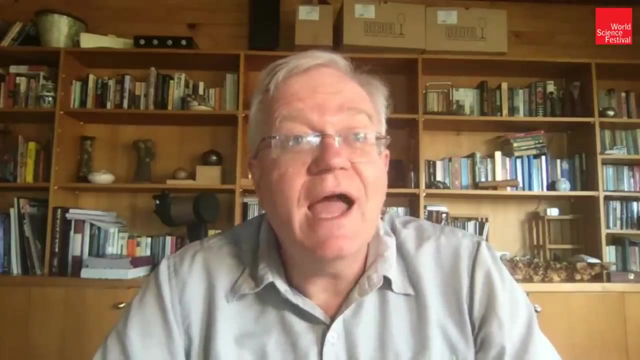 deeply physics culture and uh, there was a huge divide in 1993- 94 between the physics culture and the astronomy culture. uh, we both kind of pointed at each other and made fun of each other- would be, i think, a good way to describe it- and it was clear we weren't going to be able to easily work together. so you know, i when 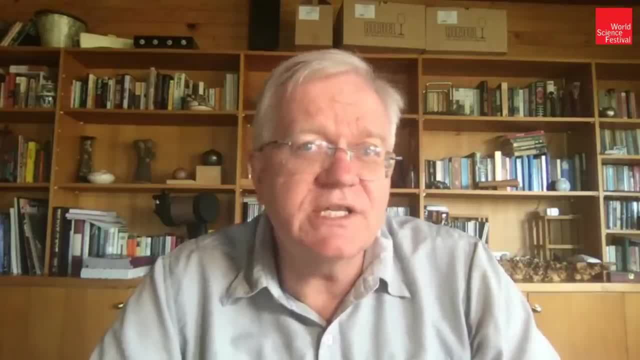 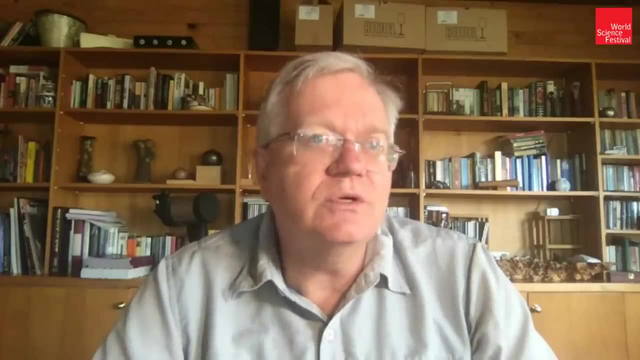 i finished my phd, talked to nick sunset when i was down in chile and said: let's measure q. naught with this, we can do it. uh, I will go through and write the software. we need to do all this stuff because we didn't have any. 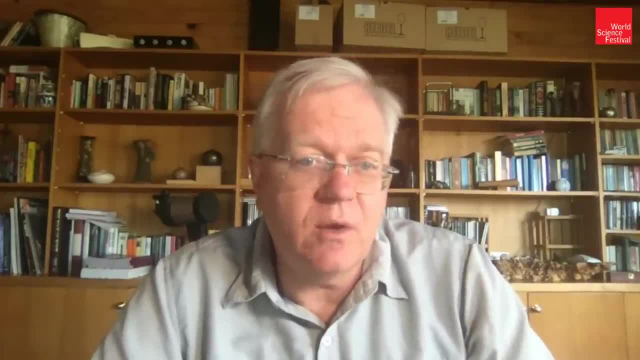 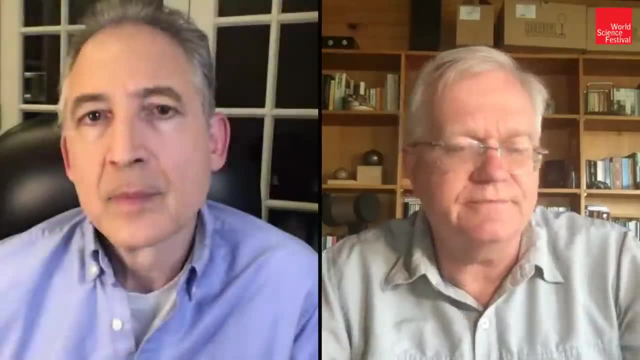 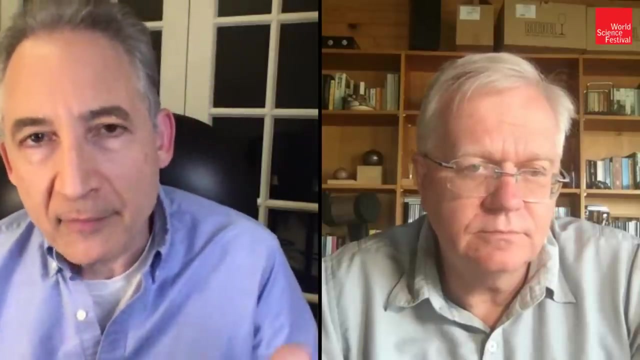 software, And so that's what I did. as my first beginning of my postdoc. I went, focused everything into this project related to my PhD, but quite different. And was I correct in my little introductory remark that you thought that you were going to nail down this deceleration? 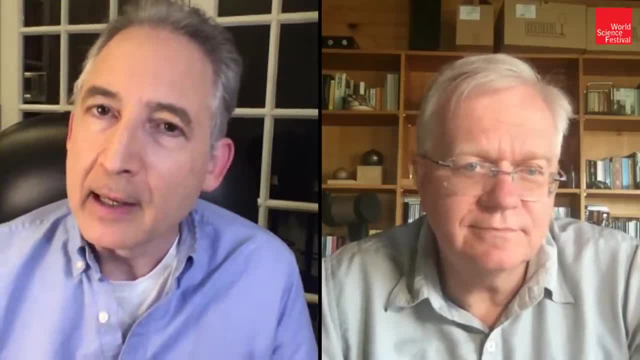 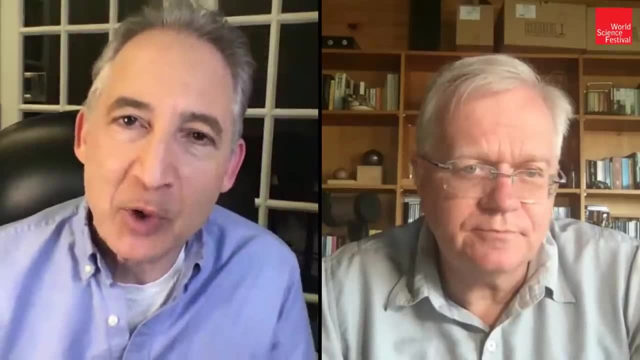 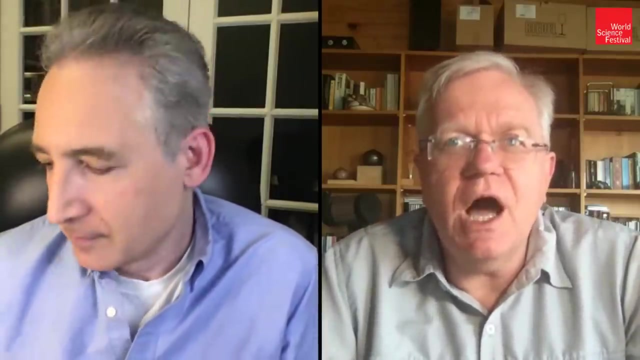 parameter give a quantitative value for it. Did you think that you could be on the cusp of a radically different conclusion from that work, or was that just never part of the thinking? Well, so the idea of a cosmological constant goes back to 1917, and it's sort of been a. 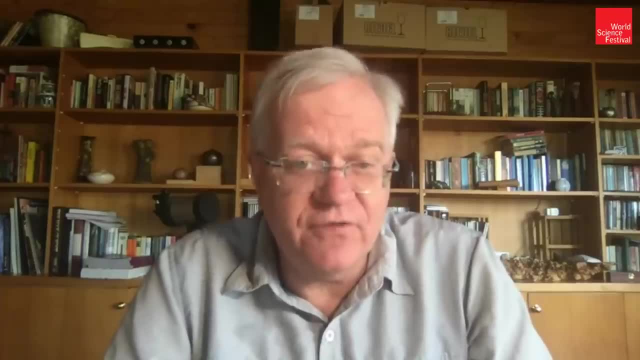 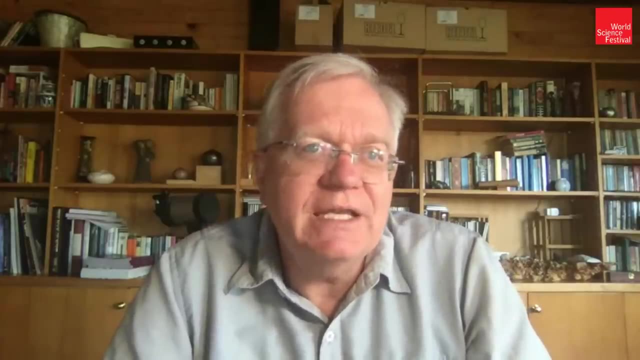 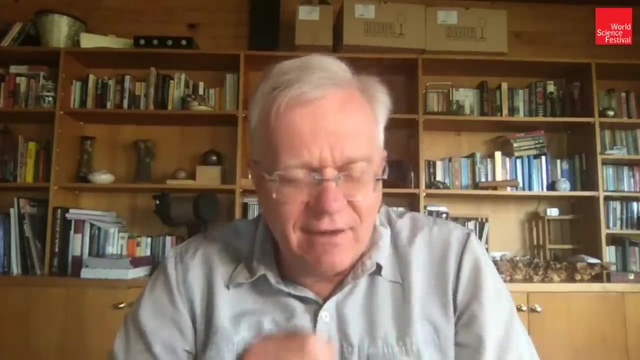 cosmologist's graveyard. So we made fun of the cosmological constant. Sean Carroll, who was my office mate, wrote a review in 1992 for the big astronomy reviews program And I remember him going through- and Alan Sandage had done the review, with little yellow post-its And there were like: 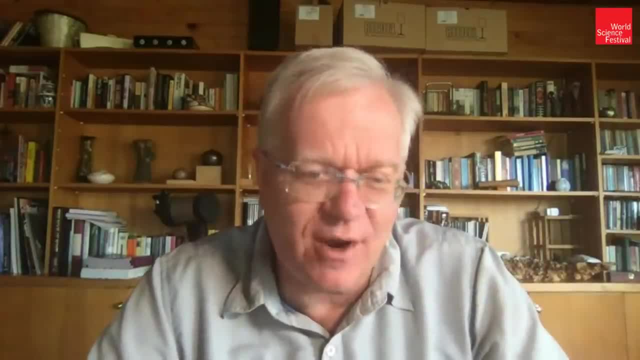 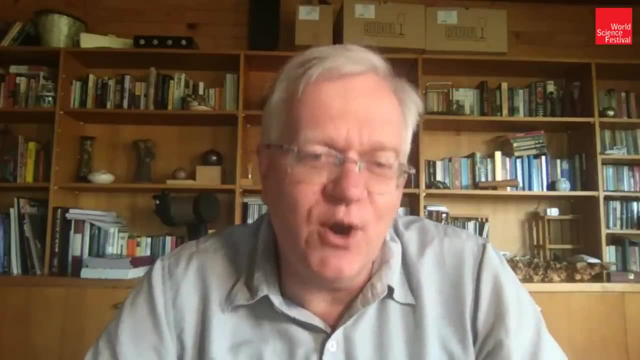 thousands of post-its in this little review. I'm watching him struggle and go through this And I'm like Sean. why are you wasting your time on the cosmological constant when we all know it's a joke? So we knew about it. 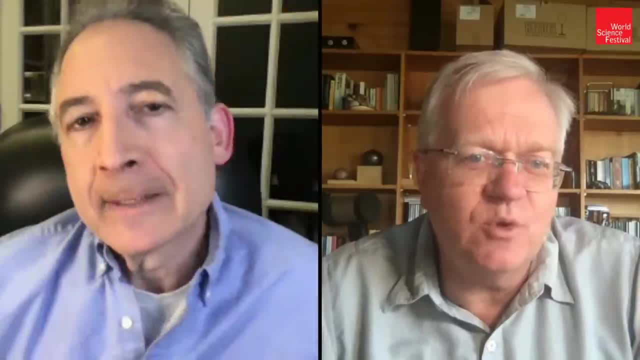 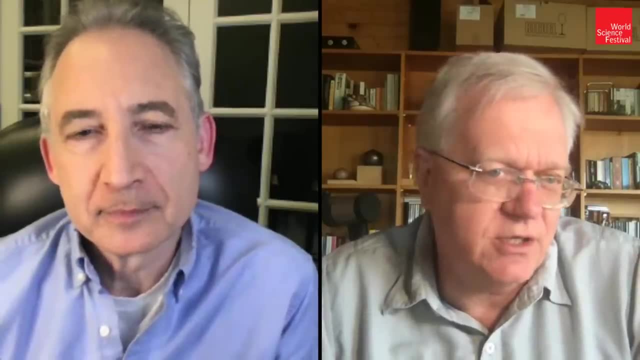 It was a joke. It was the thing that people refer to when they got the wrong answer. That is its history, And so when you suddenly get the wrong answer- as we'll describe later on- you feel like you're part of a bad joke. 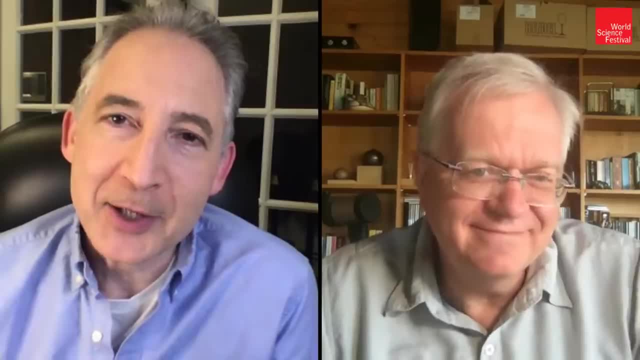 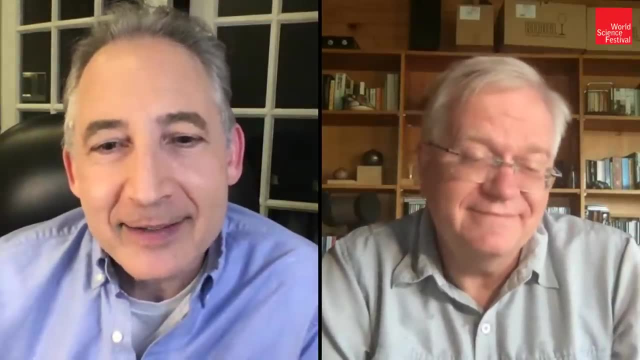 But it is a bad joke that has an illustrious history, right, I mean? the first person to tell this bad joke was Albert Einstein, right, I mean? so I guess that's an example of what you're saying. You know he is looking at the equation. 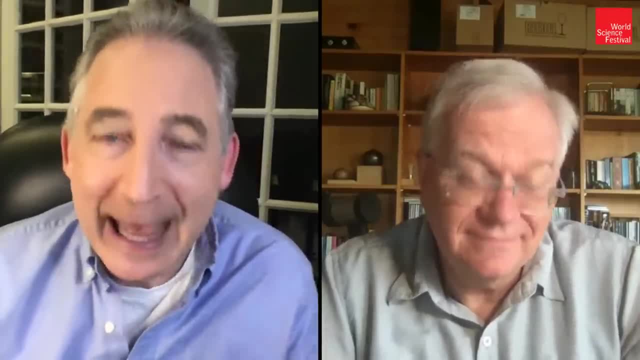 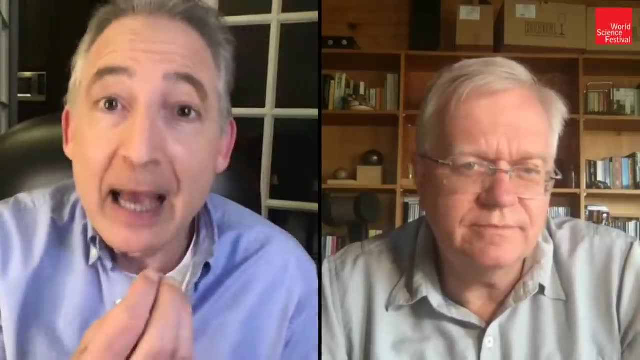 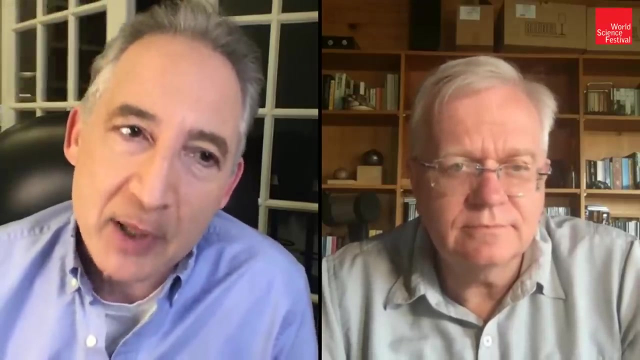 So, But all the contradictions of general relativity can't get a static solution out of the map, as this philosophical prejudice, shared by most everybody in the world who is thinking about these things, that there should be a static solution. And, as you say, he forces one into the math by introducing this: 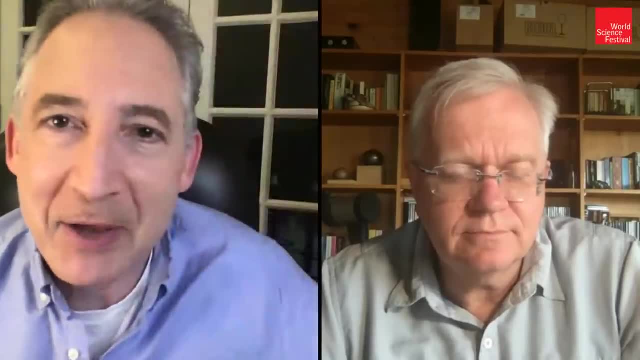 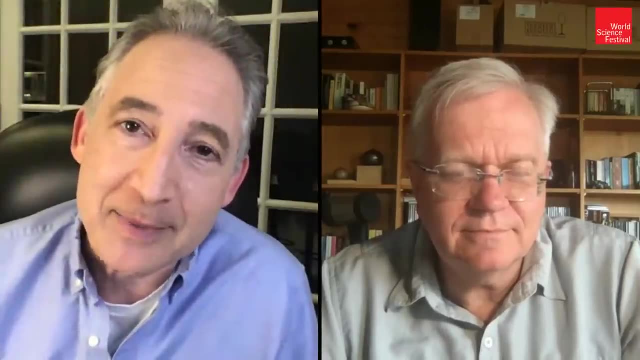 cosmological constant, But he then smacks himself in the head when the observations show that the universe is not static, And I guess that's the first example of where this becomes, perhaps, a joke. right, Yeah, Yeah, Yeah, Right. 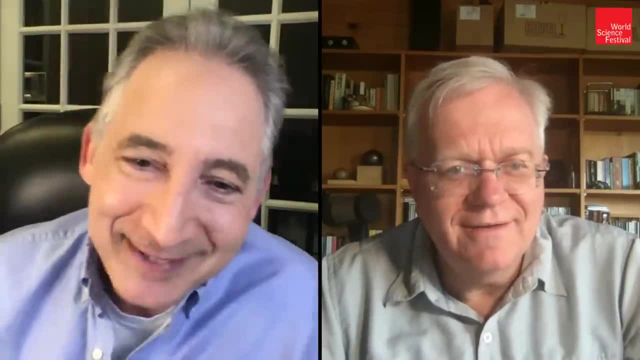 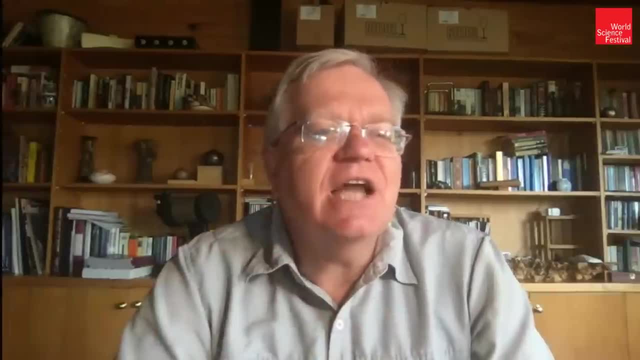 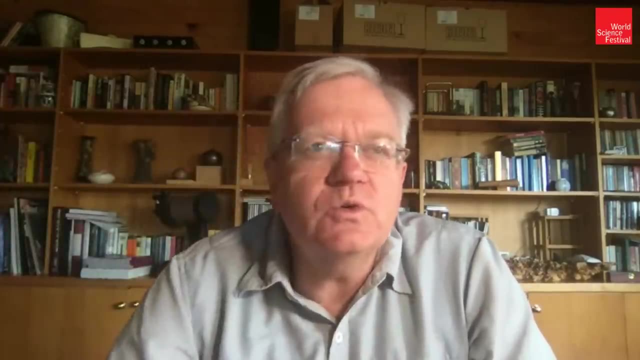 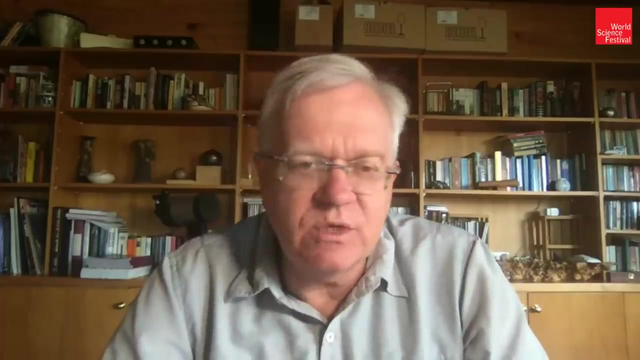 interestingly enough, If you look at his visit in Caltech in 1930, 31,, he still has Landham up on the board And in that very famous interview that was done by Gamow, done in German, often saying it was my greatest mistake, He didn't say it was my greatest mistake. Bruno Leibengut and our team. 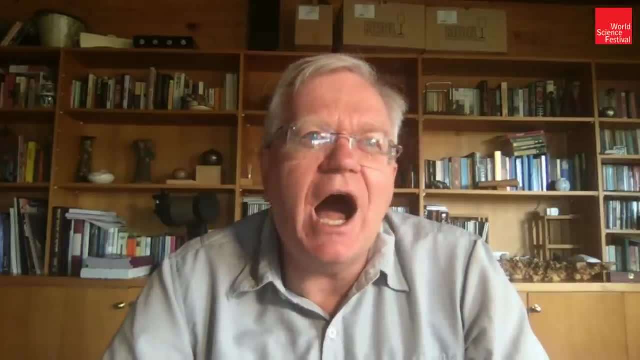 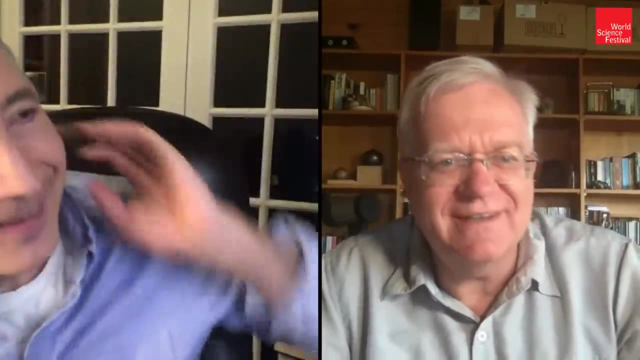 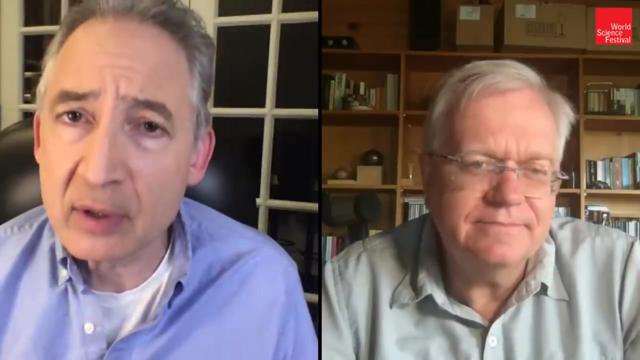 who actually reads German, said. he said I was acting like a donkey with the cosmological constant, Very stubborn to do it. Huh, You know it's interesting because in the 1931-32 period there's another quote of his that I read- I don't know if it's in a paper or if it's in some media. 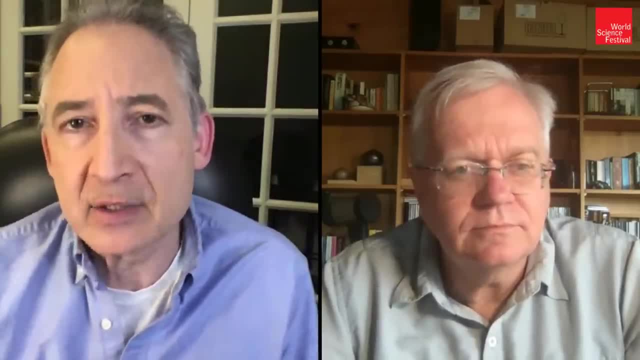 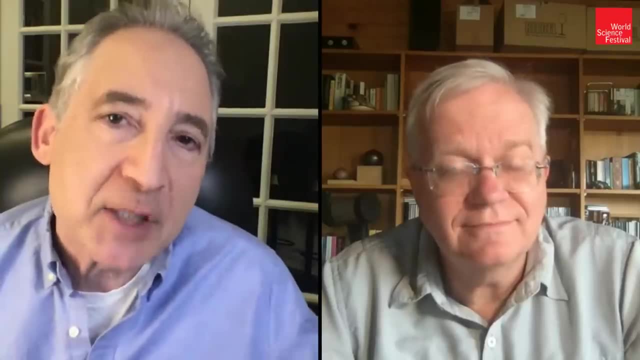 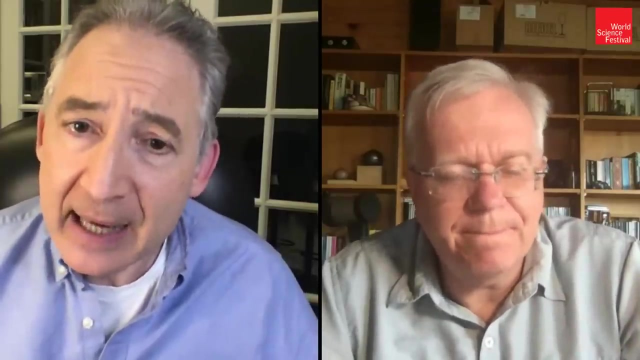 account. But Einstein actually says: I can't get it exactly, but he says something like: only future observations of the expansion of space will determine whether or not there's a cosmological constant. He actually says that back in the 1930s. So you're absolutely right. The 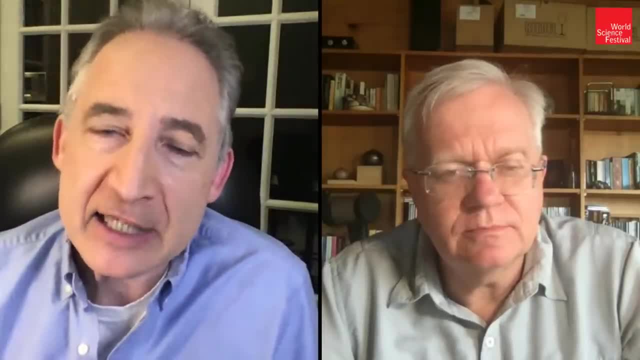 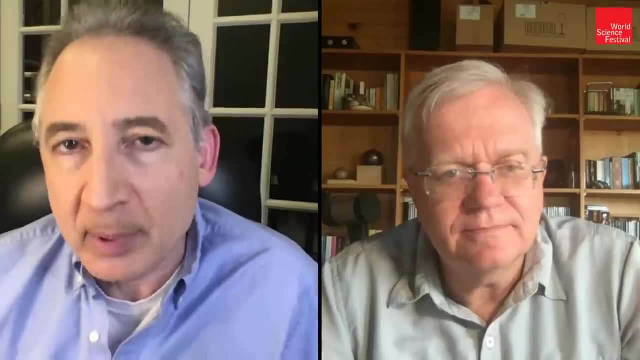 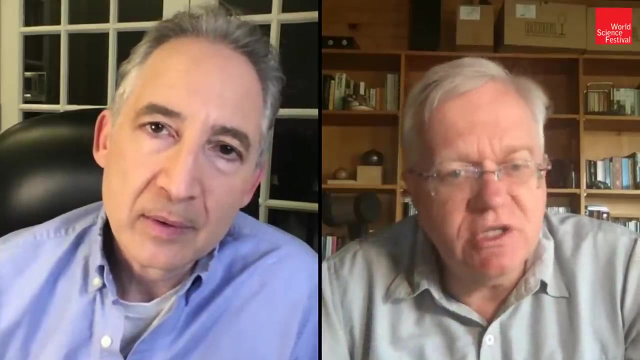 lore that he just immediately discarded it and, you know, rued the day when he introduced it. that's a little overblown, you know, And we need to also remember, in Belgium in 1926, George Lamont, who you talked about earlier And you pronounce his name with such more finesse. 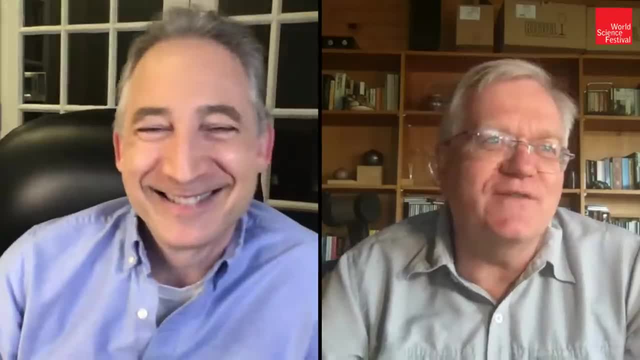 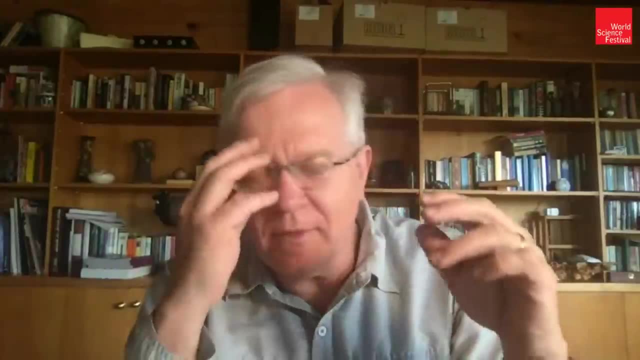 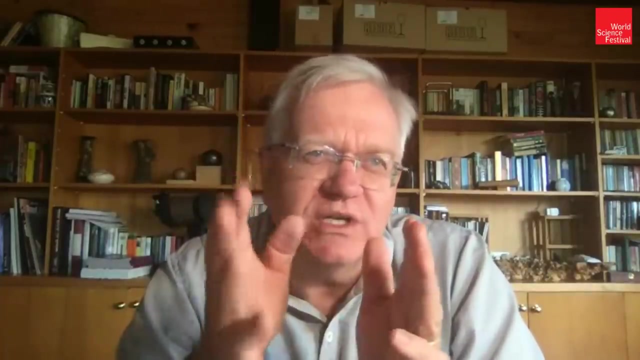 than I do. So the French have just cringed at both of us, But George Lamont showed him his PhD thesis, which he was working on at MIT remotely, And my guess is George Lamont was one of those people who was really annoying, But he basically showed here. look at the data of 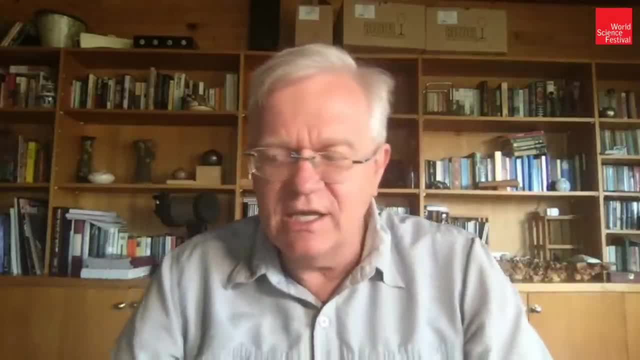 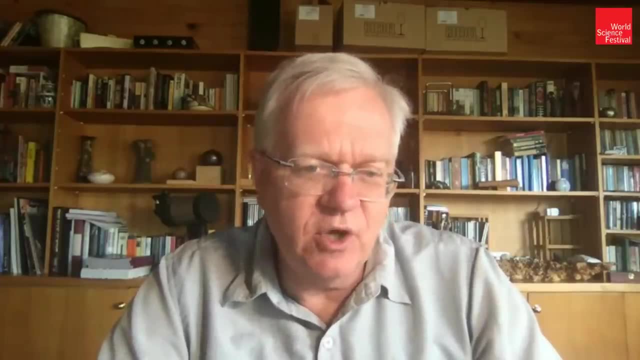 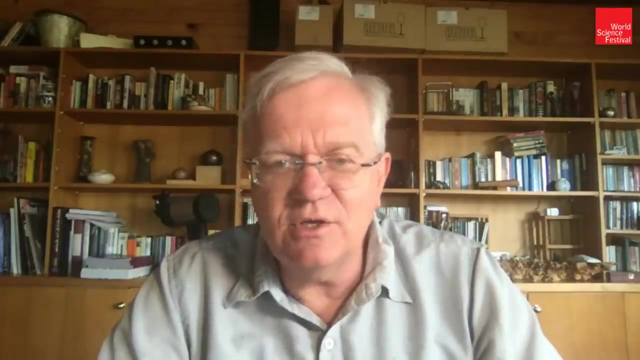 Hubble and Slipher, The universe is expanding. Here's the equations that I have derived, And Einstein reportedly said: well, your equations have already been derived by Friedman And he said something: you are a much better mathematician than a physicist, or something. 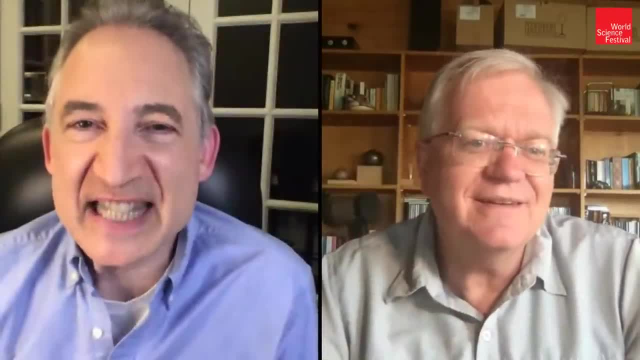 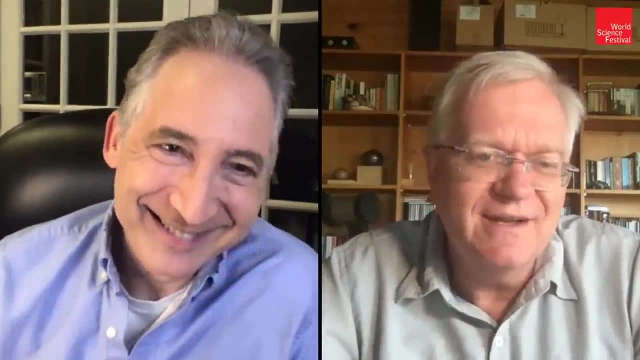 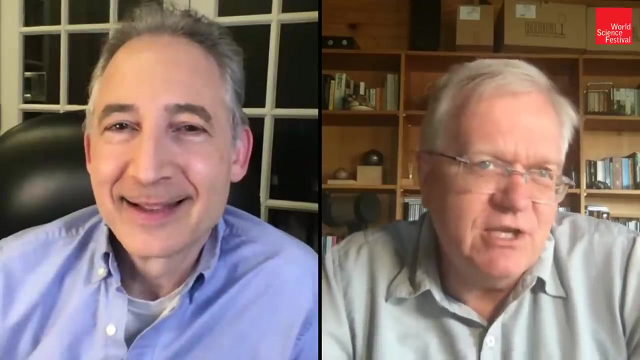 like that. Yeah, I think he said your math is correct, but your physics is abominable. Yeah, that's right, And pretty much just missed him out of hand. So poor George Lamont, who did everything, gets pipped at the post by Hubble two years later, who, I mean, did a lot of the hard. 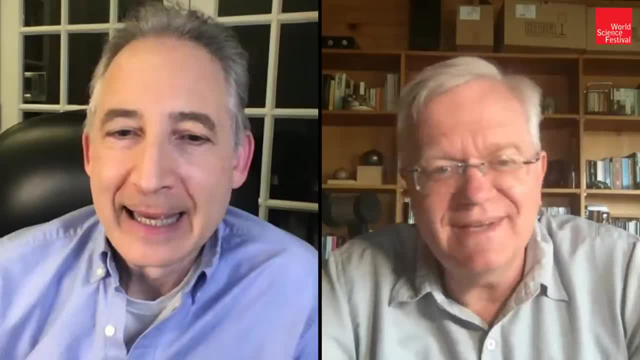 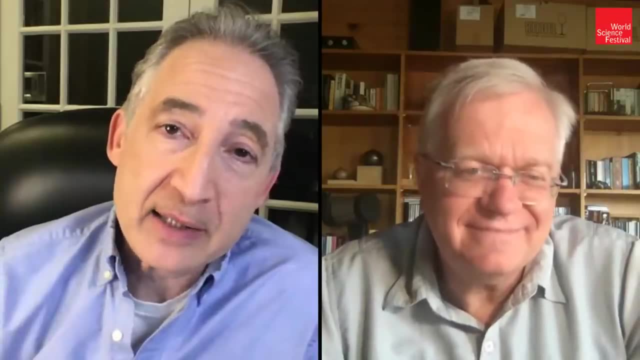 observational work. But yeah, oh well, it's life. Well, you know, it's an amazing example of inner fortitude. I mean, I think if I went to Einstein with an idea and Einstein told me that my physics was abominable, I probably would have changed. 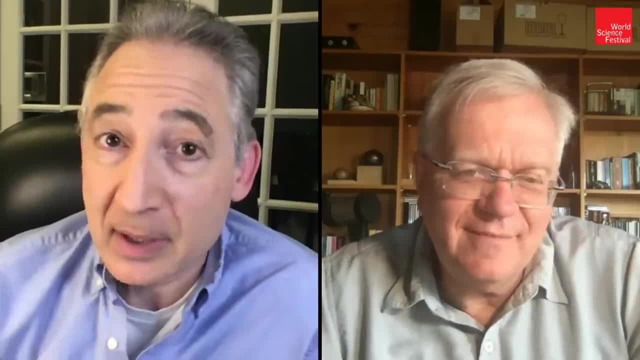 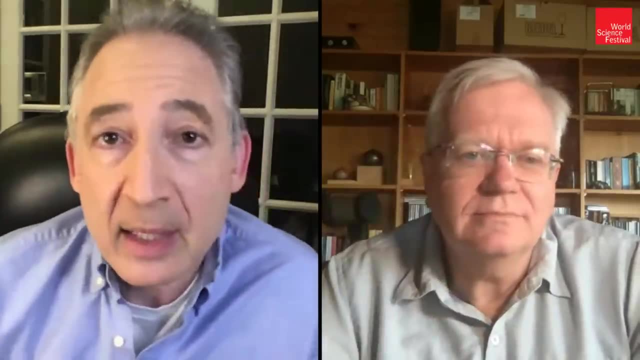 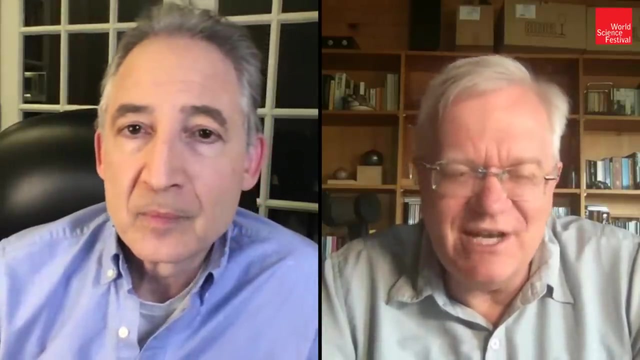 careers Or hidden under a rock or something. But you know that isn't the case with you know, George Lamont, I mean, he actually stays with it and pushes this idea forward. Yeah, And yeah, he was. I said must have been an interesting character. 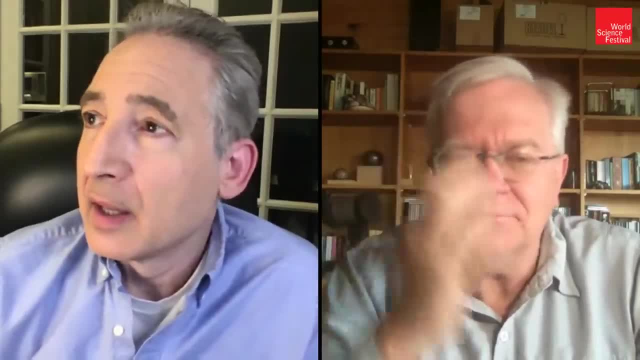 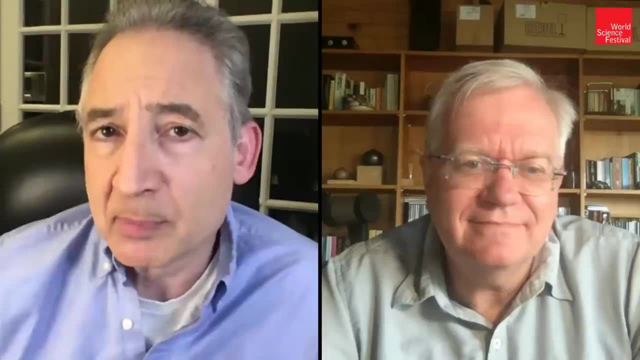 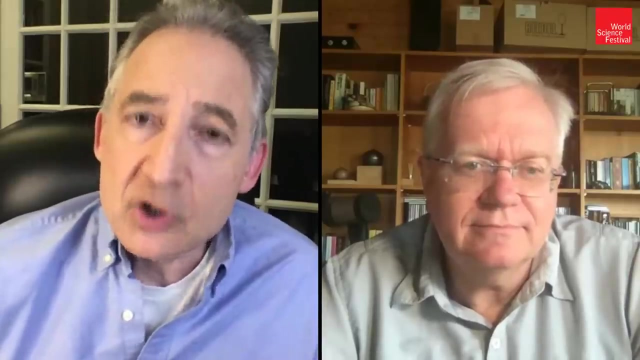 Yeah, yeah, yeah, absolutely. I mean, you know it's unusual to have you know training in physics and to be ordained. You know, the Pope at the time- I forget which Pope it was- Got wind of his work in cosmology and described it as giving a confirmation of the story of. 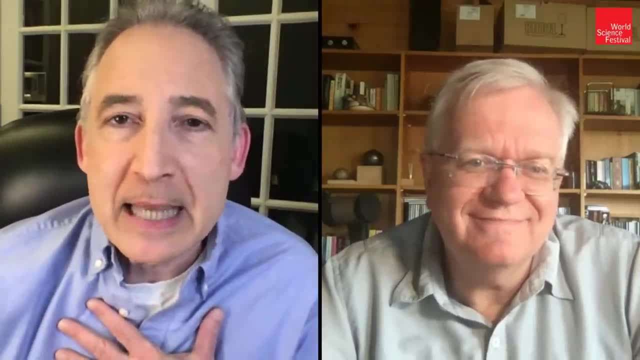 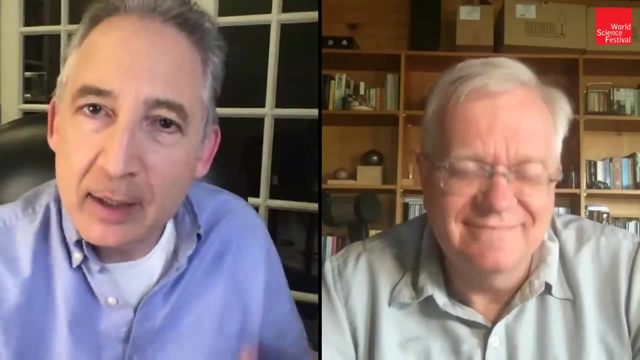 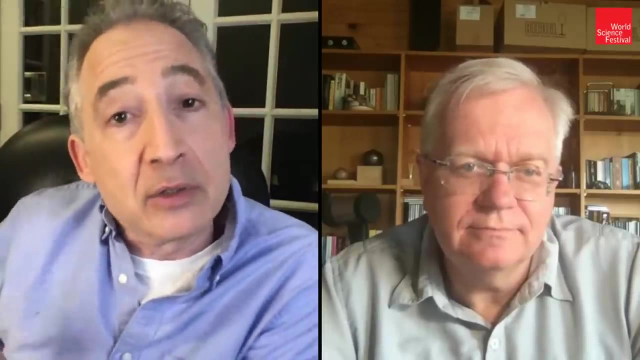 Genesis. And this, to LeMaitre, was absolutely mortifying, because he had diligently and carefully drawn a line between his theological, his religious side of his being and this sort of scientific side. Now, if you're going to do work in science, that has to do with the science. 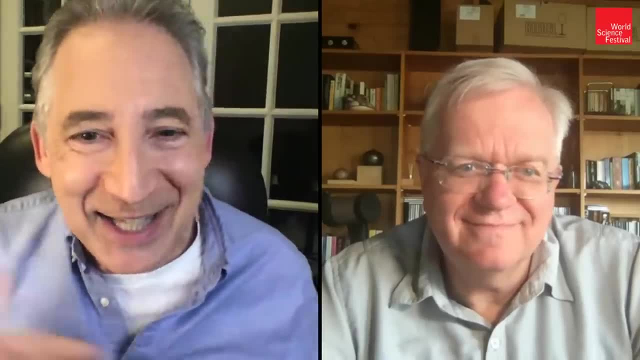 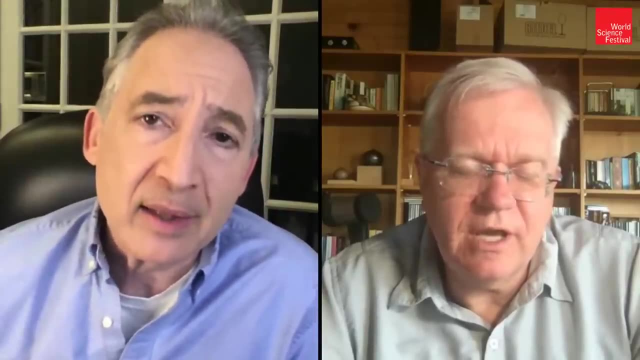 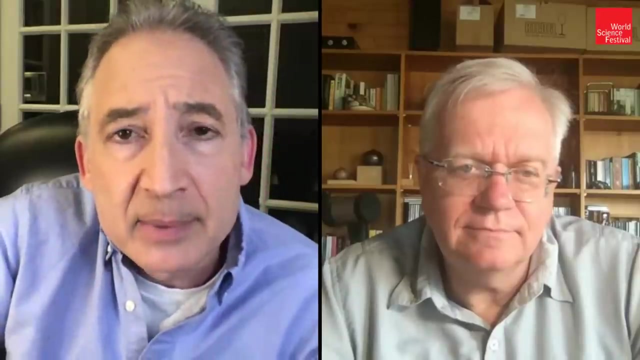 the origin of the universe. you shouldn't be too surprised that it's going to be, you know, crossing over. But it was something that he found very difficult when the religious community kind of glommed on to his work as some kind of confirmation of the ideas in the Bible. So 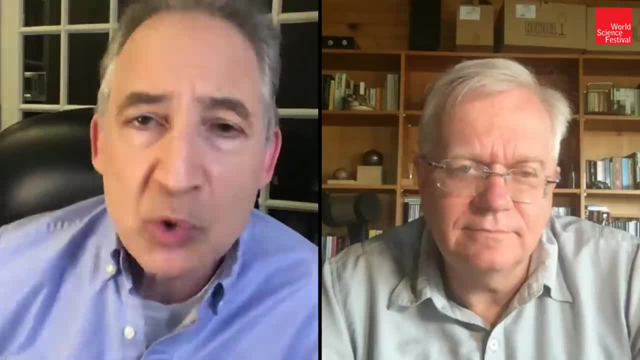 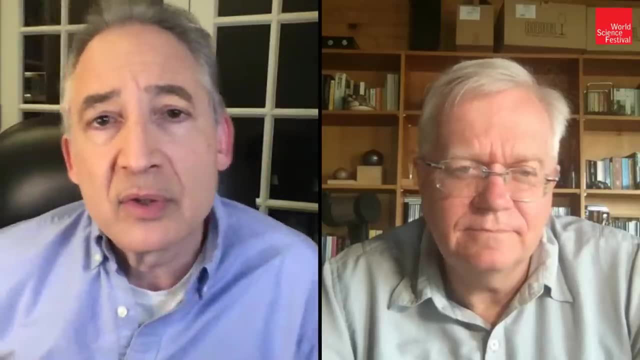 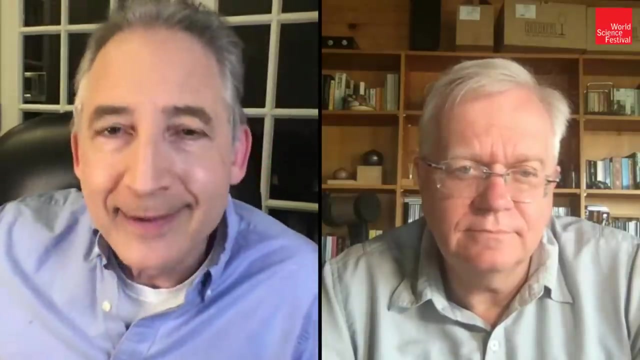 yeah, I imagine. you know. I don't know a lot about his personal story, but I can imagine this must have been a difficult, difficult period for him, But nevertheless. so this is the sort of first introduction of the cosmological constant. then ultimately it does go away from mainstream. 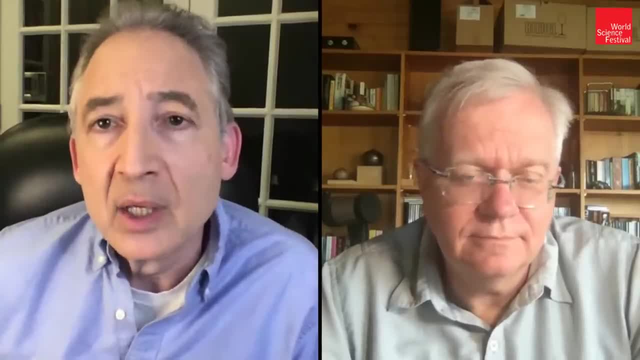 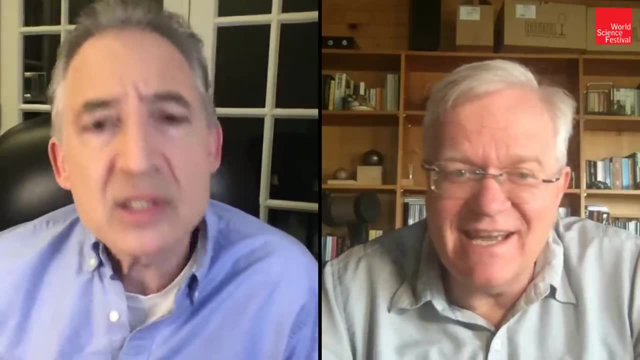 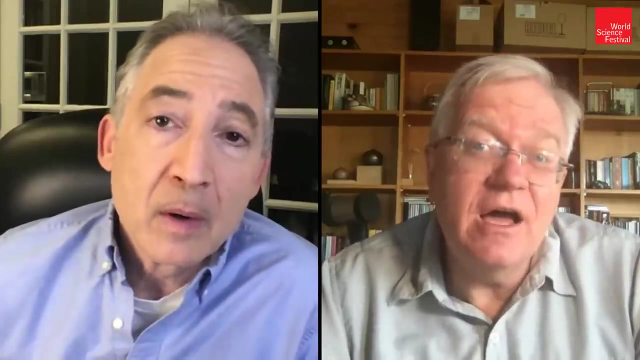 thinking in the cosmological scenario. Really it pops up I guess now and then in the 70s and early 60s. Alan Sandage, first measurement of it, cosmological constant, Beatrice Tinsley, the guys looking at- I'm sorry, I don't know that name, Who is? 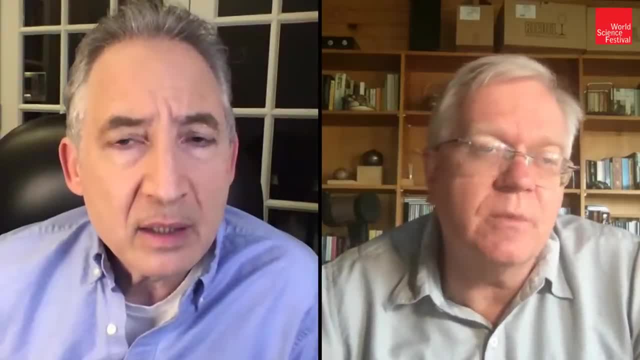 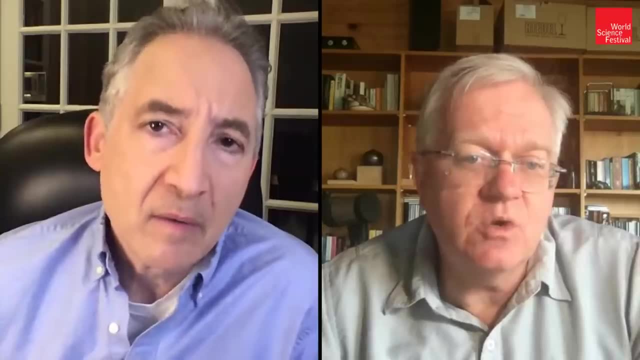 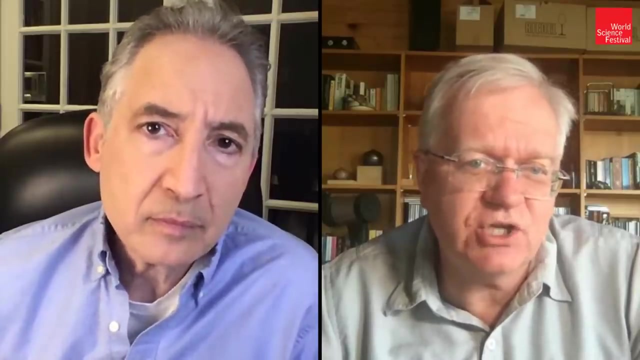 Beatrice Tinsley, great Yale astronomer. She died young but she was one of the great re-emergence of women in astronomy. So New Zealander, but at Yale, did a lot of stuff in stellar astronomy but went through and basically said the K corrections. 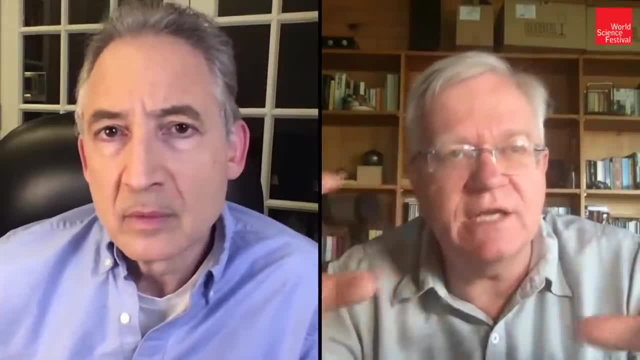 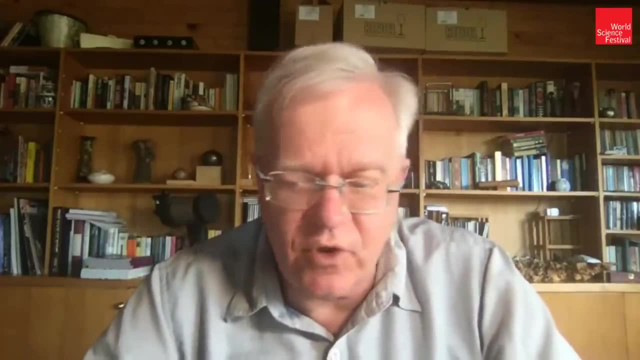 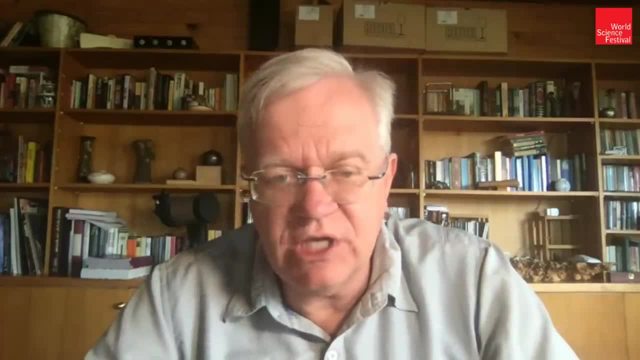 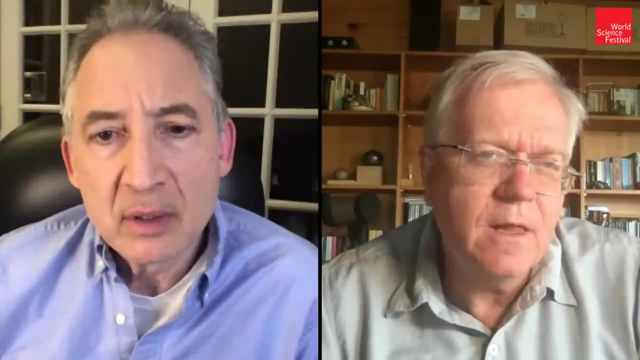 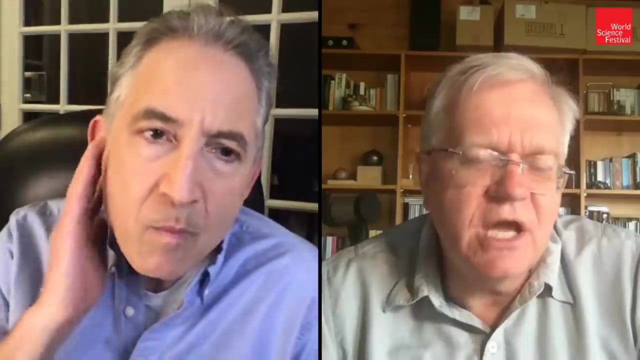 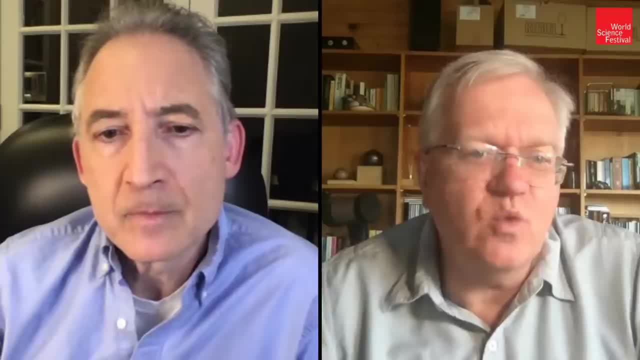 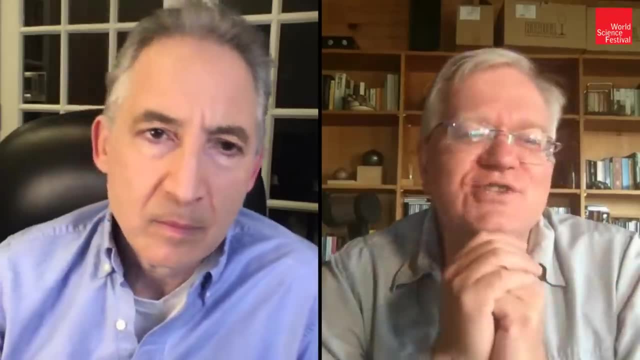 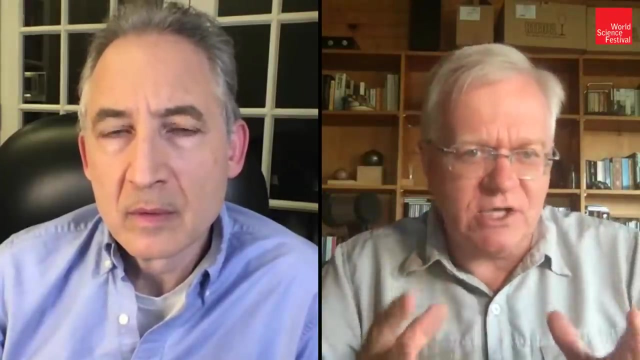 even today are too much. But it was interesting that they weren't even worrying about the evolving stellar populations back then. So big change And then, I think, really the really interesting one, just to show you where people go askew on this: in the late 60s we saw all of these quasars. 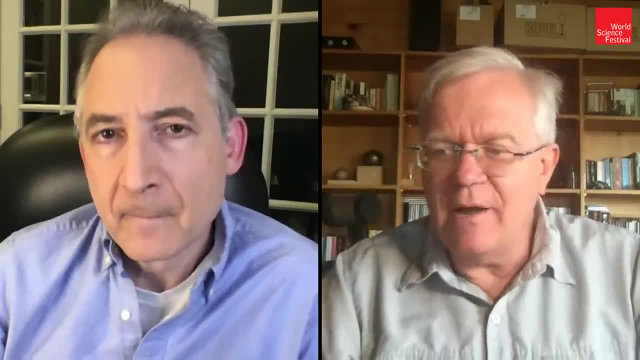 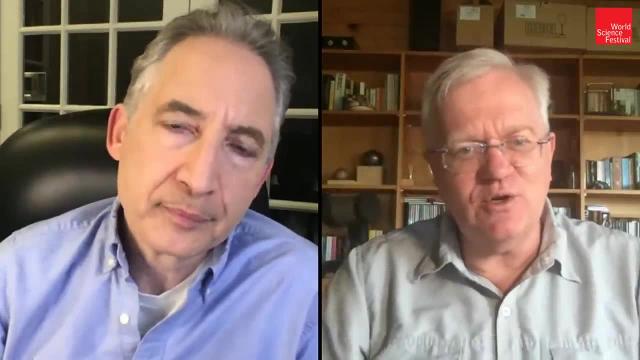 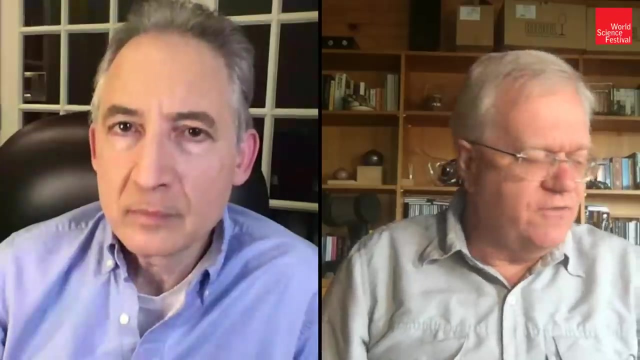 which are these bright black holes? it turns out peaking at a redshift of two, So about 8 billion years in the past, And it turns out that you can create what's called a loitering model where you have just enough cosmological constant that the universe is slowing down due to gravity. 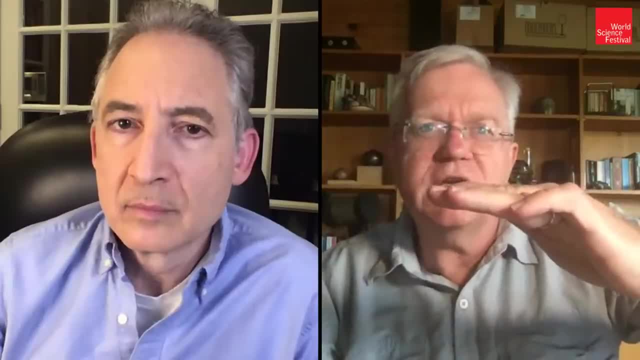 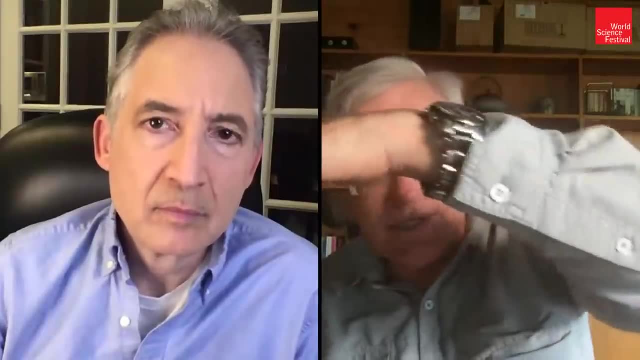 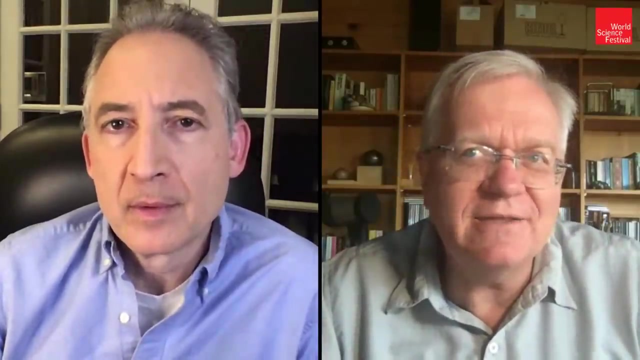 and the cosmological constant, which has that repulsive gravity, kicks in at exactly the right time and the universe kind of stalls. And so the idea was maybe the universe stalled back to 8 billion years ago And that's what we were seeing. That became quite hot for a couple of years Again. absolutely not correct. 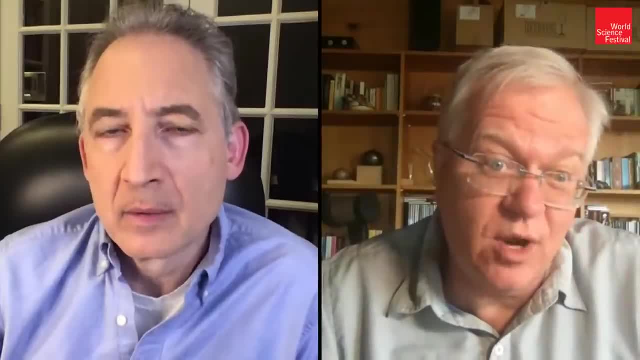 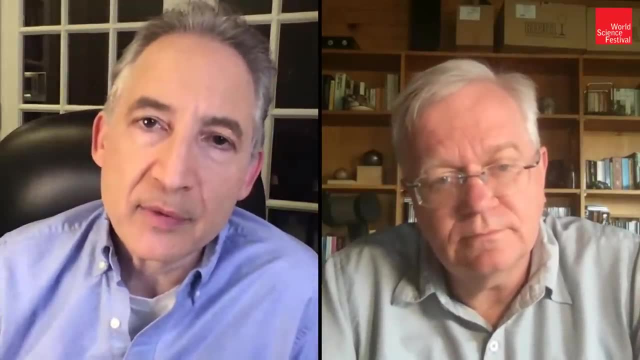 It just turns out, there were a lot of black holes 8 billion years ago that were really bright. Yeah, right, right. And so then this gradually leads us to, of course, the work of you and your colleagues trying to measure the rate of cosmological slowdown. 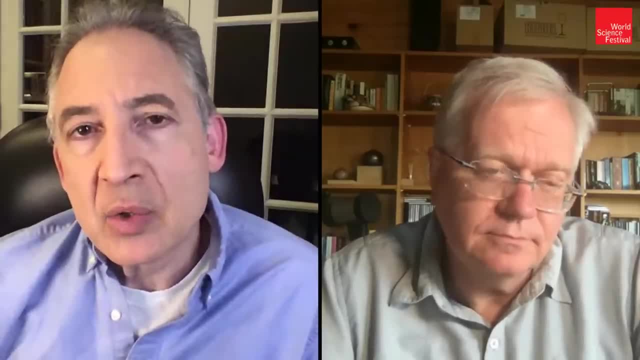 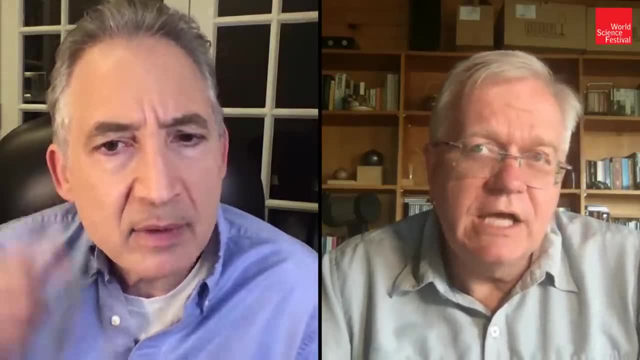 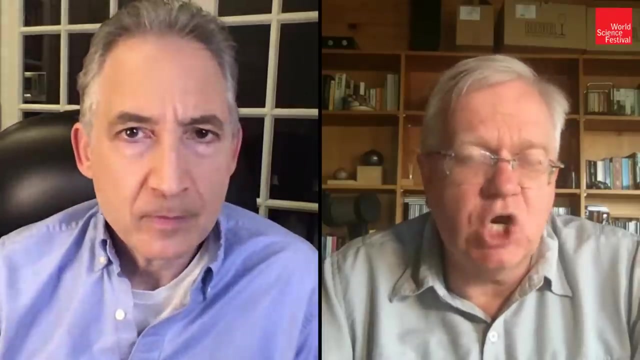 in the outward expansion. And so when did you, when did Did that work begin proper? Was that early 90s? Was that sort of the beginning of? Yeah? so Sol Perlmutter, who I know you've had a chance to talk to, but he and the group at Berkley started in 1990, give or take a year or two. Yeah, so Sol Perlmutter, who I know you've had a chance to talk to, but he and the group at Berkeley started in 1990, give or take a year or two. started in 1990, give or take a year or two. 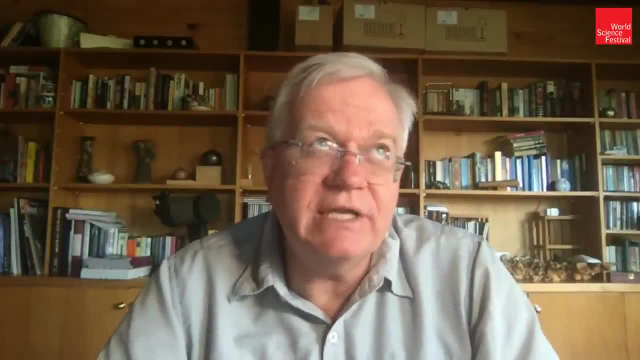 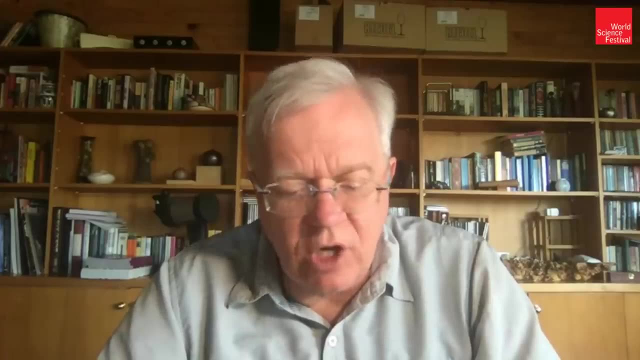 but they didn't discover their first object until 1993.. I think, uh, the technology just wasn't there, Uh, so I started the high Z team with Nick Sunseft in 1994.. I just finished my PhD, Uh, 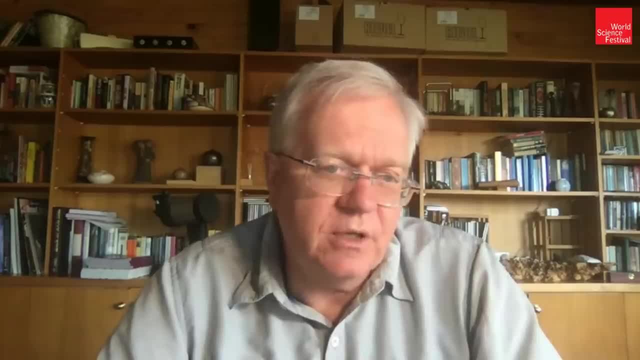 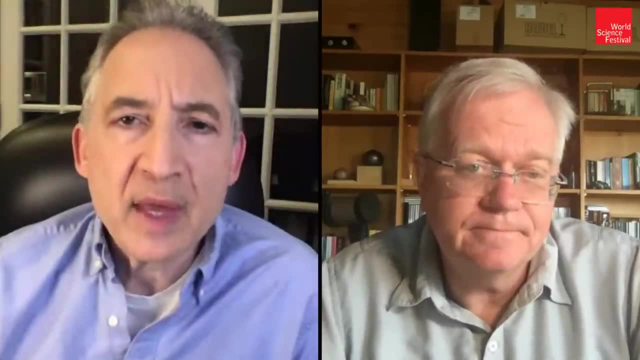 and so we really started in 1994, but uh, Saul and the and co had been working, you know, almost four years on it, So we had a lot to catch up. And where were you at that time when you started? Remind me again. 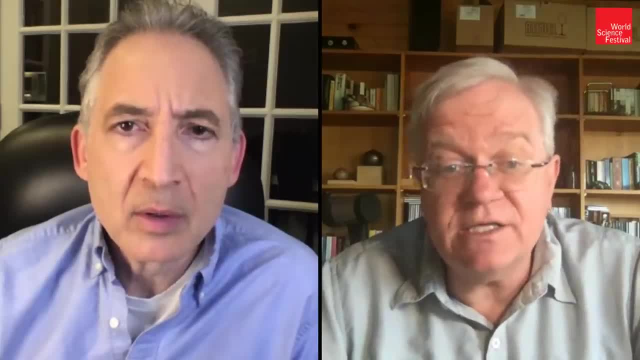 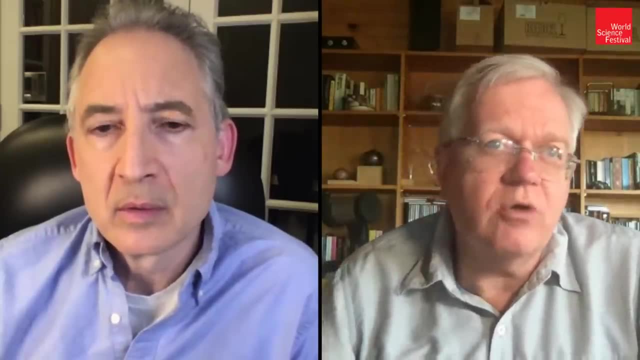 when you were? Oh, I was a- uh, a CFA, a center for astrophysics fellow, where I spent 18 months before moving to Australia. So when I started the work, I was already transitioning to move to Australia, Jeremy Mould. 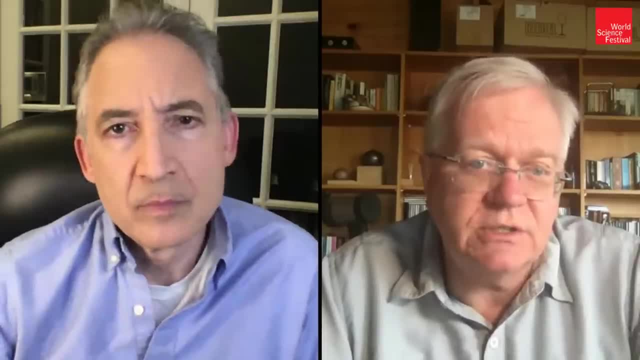 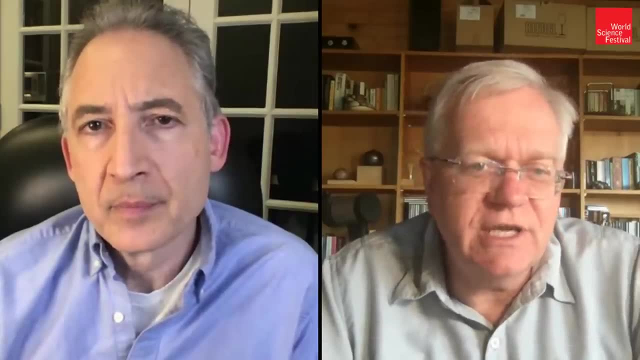 one of the leaders of the Hubble key project to measure the Hubble constant had become moved from Caltech to to ANU, where I'm at now still Uh, and I eventually, after several attempts, managed to get a job here. So so I moved here at the very end And and I was able to get a job here at the very end of 1994.. Got it, And when? when did the data really start to have, you know, sufficient accuracy that you could begin to calculate the deceleration? 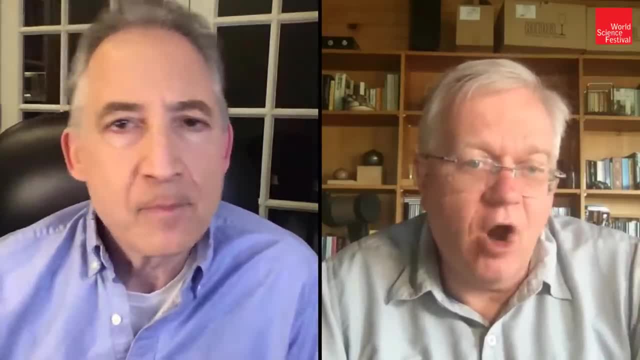 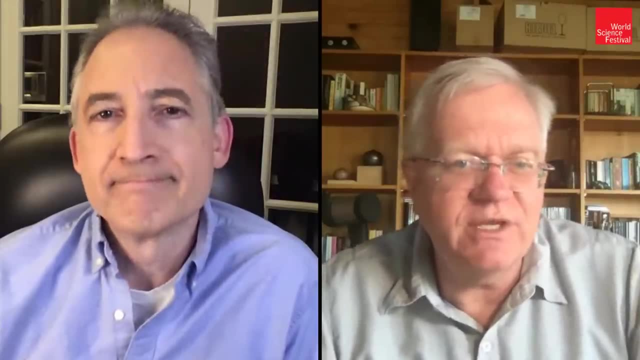 parameter? Was that in the middle? Yeah, So we took our first data in 95 and almost didn't discover anything. It was a disaster. I was trying to run a telescope with a young baby from Australia when the internet was one character per second. Uh, Oh God. 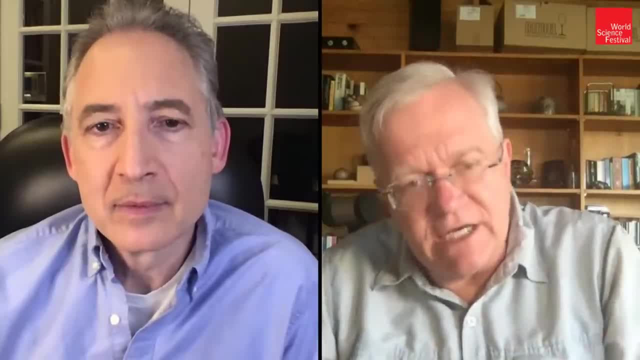 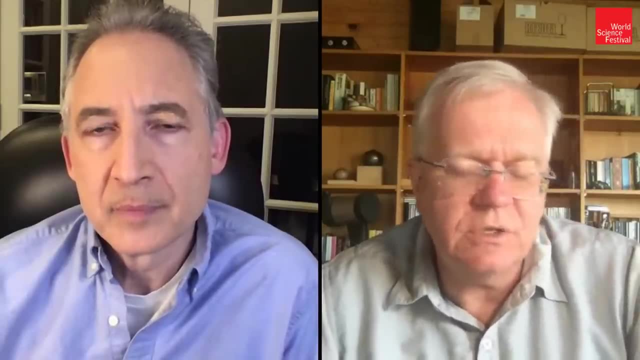 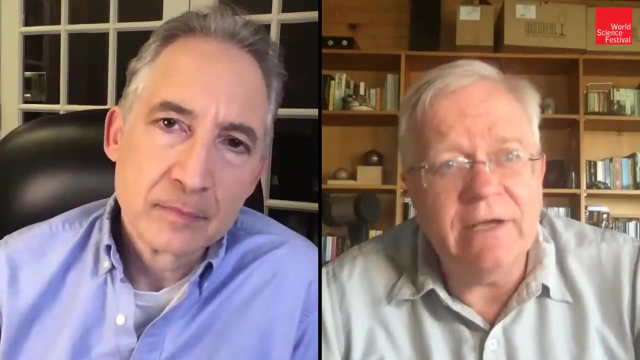 but we did manage to find one, but over 95,, 96,, 97, we then brought together roughly 20 objects, 15 of which were useful. And so at the very end of 97 and from memory, talking to Adam, 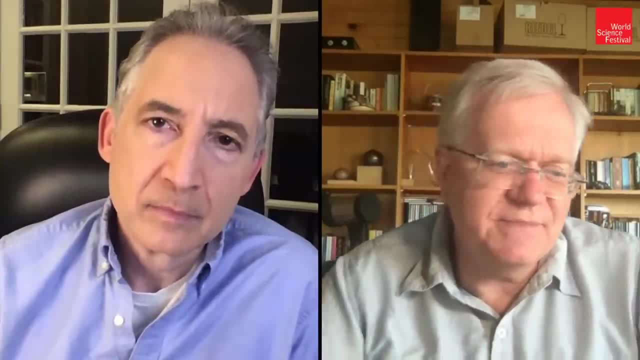 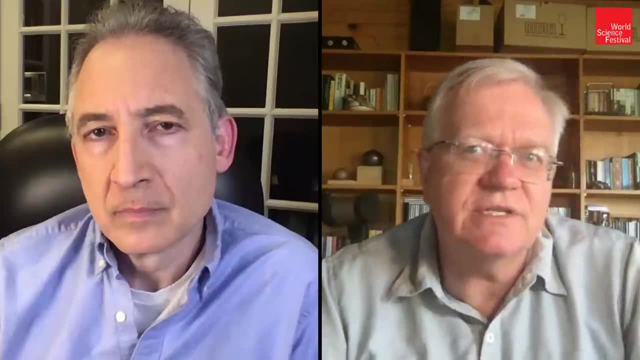 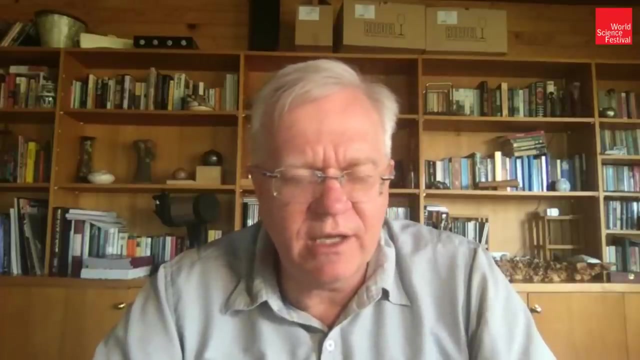 it was in November 97, Adam sent me the final data of the distances and the redshift and said: tell me what you think, And so you know. we had independent codes and I ran it and I'm like uh. 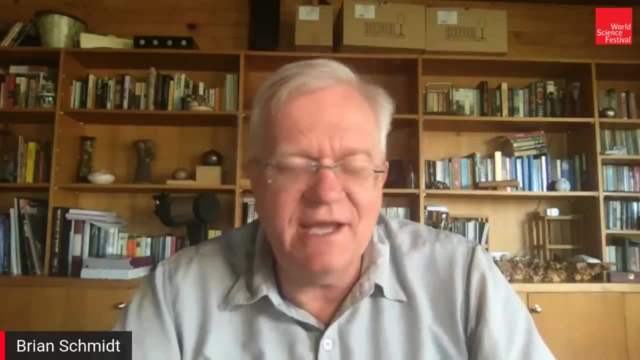 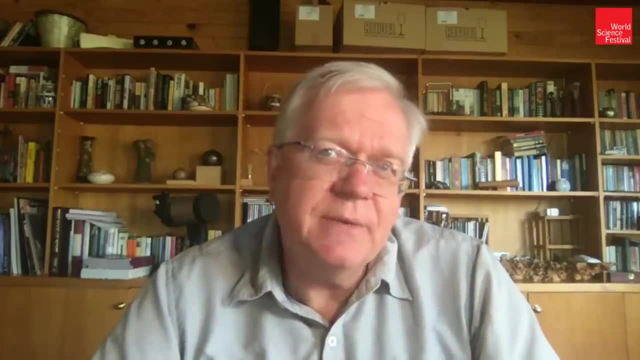 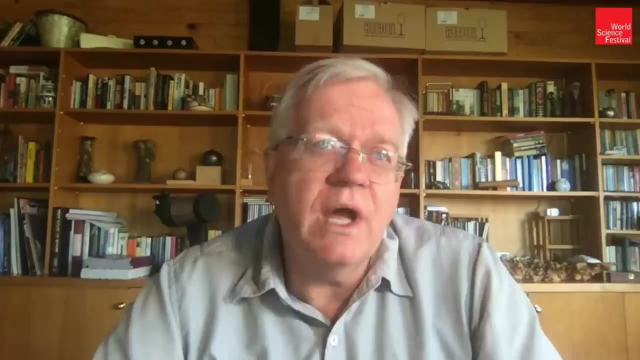 something like Houston. we have a problem because it's very clear It indicated that the universe was speeding up over time. Uh, and so from that time in November, Adam and I worked very closely together just to go through literally everything independently, together, in our own way. 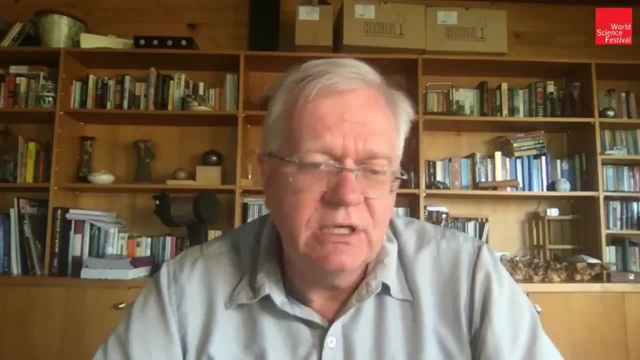 And you know, we found some little mistakes, but in the end, uh, by it was the 8th of January 1998, we had gone through every single thing we agreed we would go through. Uh, and we were. 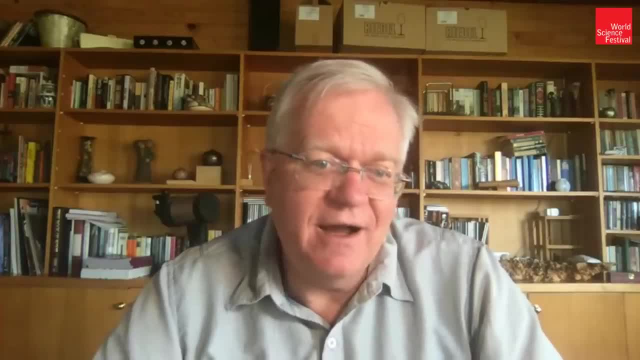 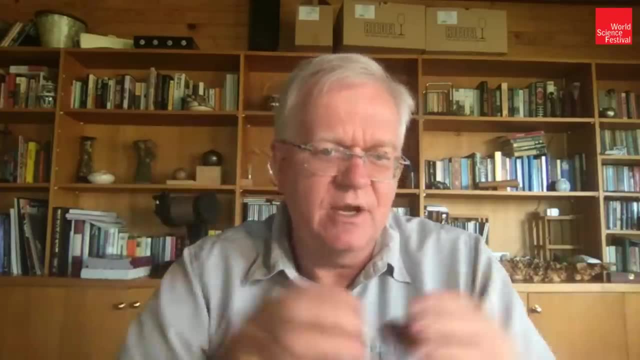 uh, at that point, having to tell our team: uh guys, this is what the analysis looks like. Um, because every person in the team had had a little bits and pieces of it, but we had been doing the final synthesis together out of the resistance. 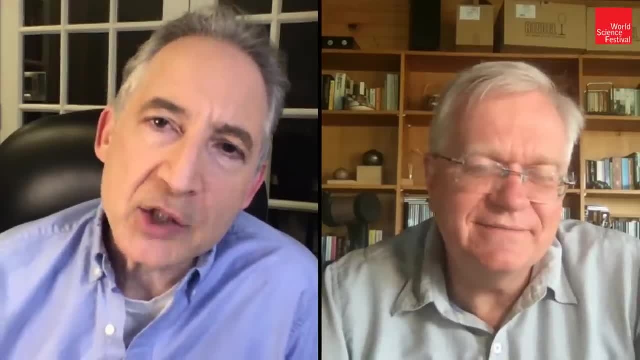 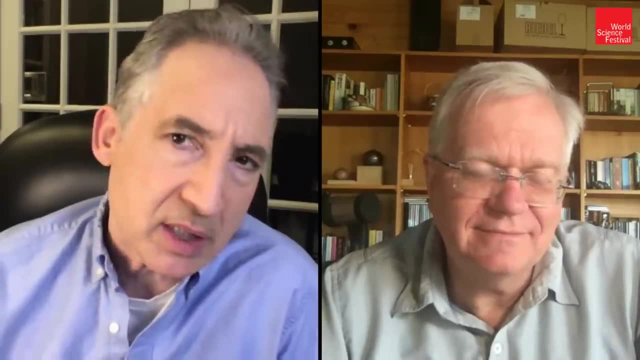 In other words, you can well imagine that you don't want to be the butt of another cosmological- uh, cosmological constant joke, right, You know? 80 years later, or something. So was there resistance in the team to this conclusion, or was it? 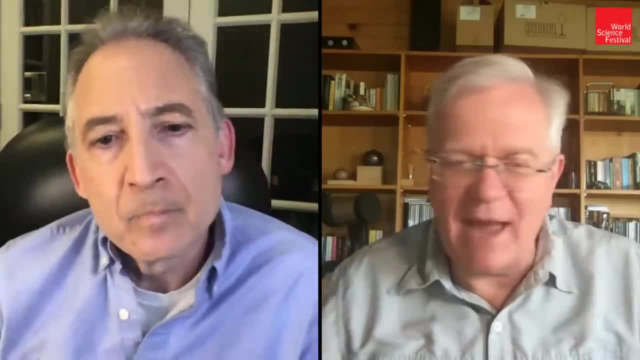 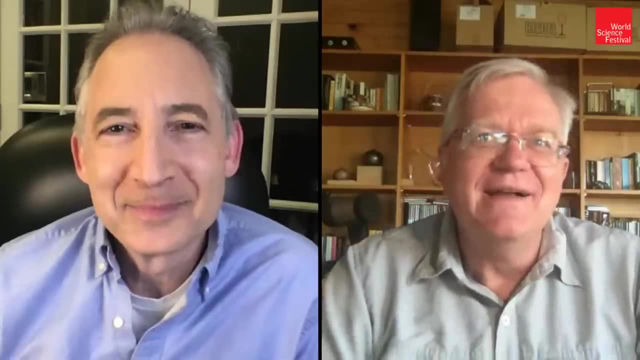 Hey, that's what the data is. That's what the data is. Well, it was complete smattering across the things. Alex go, this is right, We got to go out nature paper tomorrow. Um, Bob Kirschner, uh. 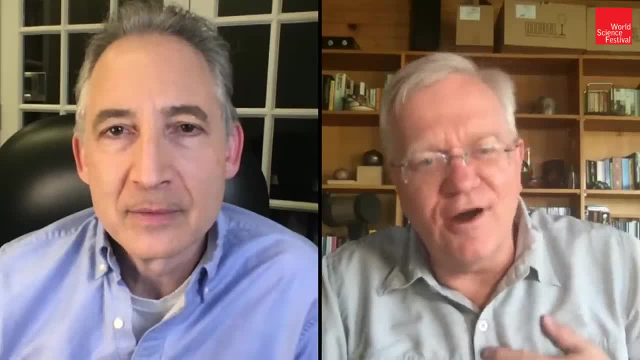 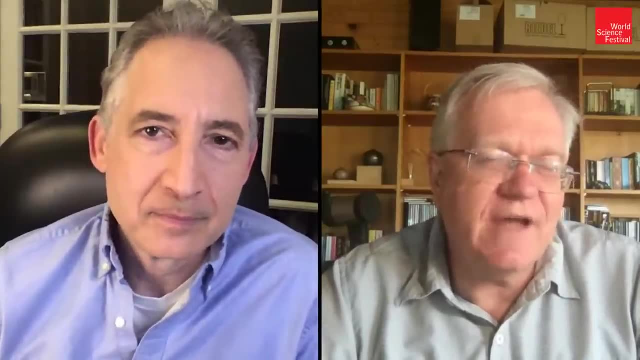 saying: uh, yes, it's the day to data, but our heart of hearts, we know this cannot possibly be right. Uh, you know the very careful uh, Nick, sunset at Bruno live and good, uh and um. 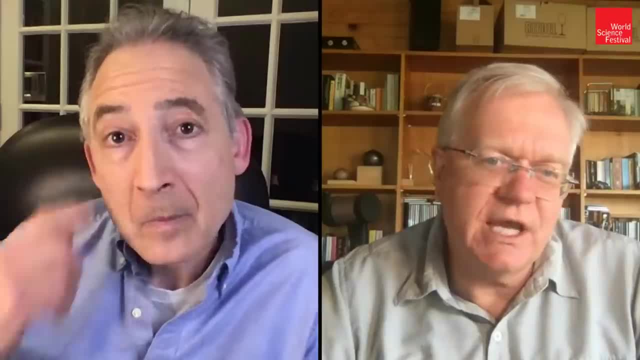 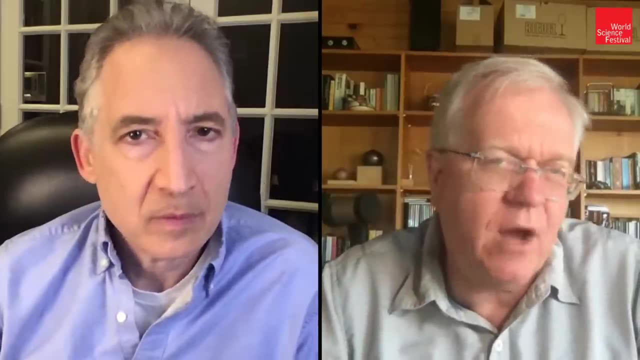 Mark, uh, Phillips, going through and say, Hey, Hey, we need to go through all of this bit by bit. There's, you know, this requires extreme proof. Now, Adam and I had done pretty much all of that ourselves. 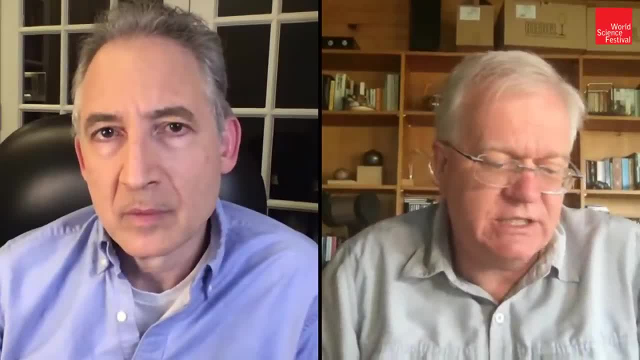 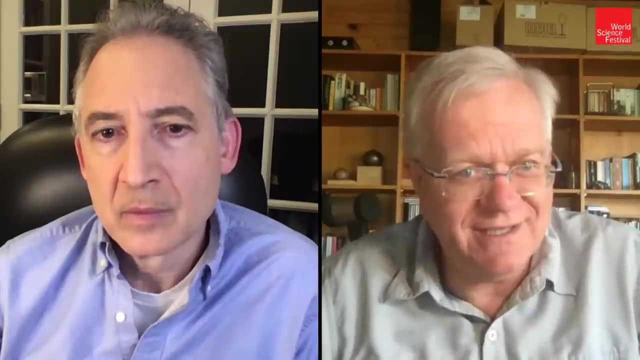 but the whole team and you know. the basic thing I said is, yes, we are scientists, We don't like this answer. It is crazy, but we are gonna. we're gonna have to publish it, even if we don't like it. 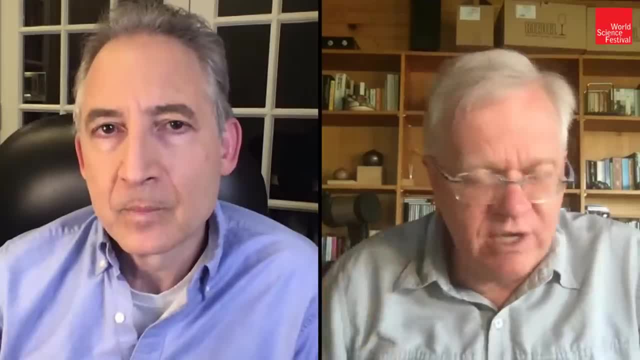 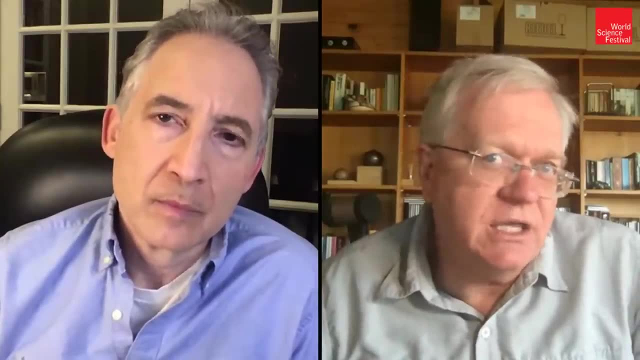 If we are convinced it's correct and we will do every reasonable test that this team can come up with. Adam and I have already done a lot of them. Uh, and the reality is, I think we had more or less done every test that people had asked for. 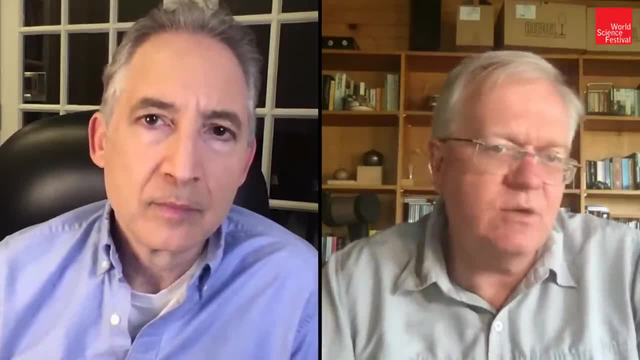 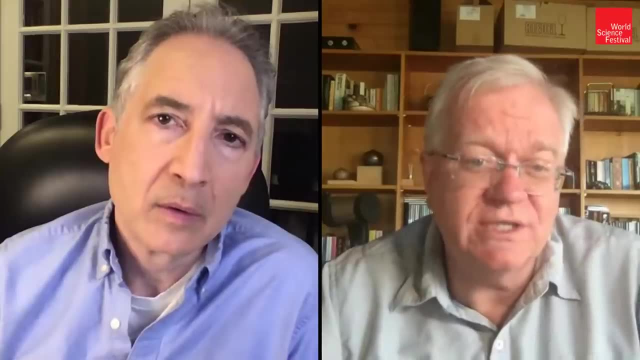 but people wanted to do it their own way, in new ways, And we did that. in the end Everyone was like: all right, we cannot make it go away. It was quite a robust result. in the end, You know, it was a 15 or 20% effect. 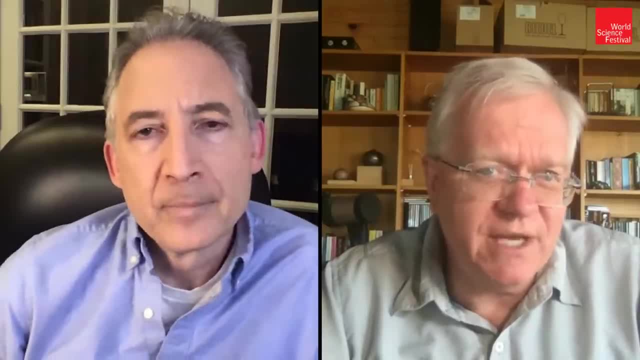 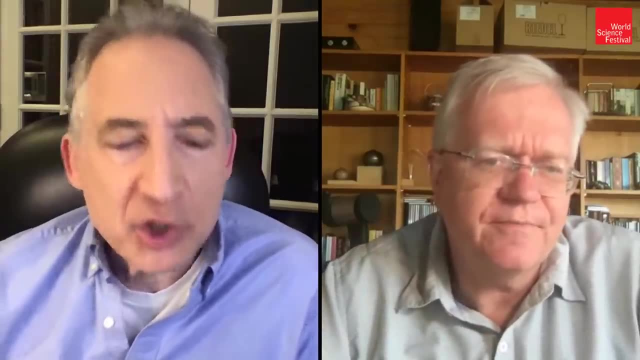 Which you know, uh, for astronomy at the time was pretty precise, but we knew we were, we had things controlled to two or 3% And I should know the answer to this. I don't apologize, but you can tell me immediately. 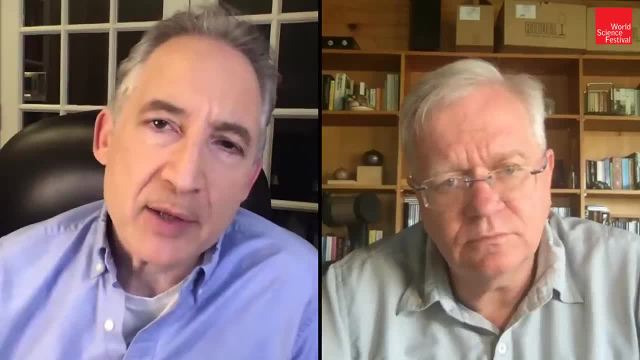 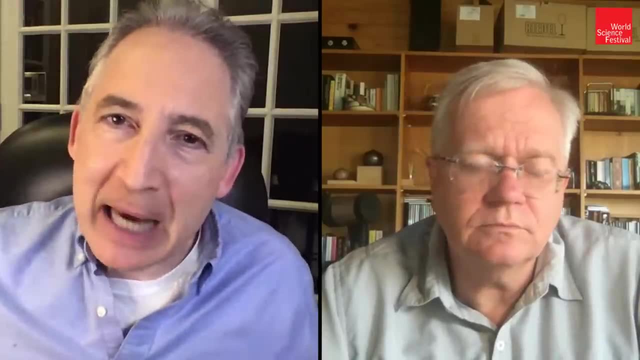 So in your paper, did you commit to the cosmological constant as an explanation or did you focus for the most part on just here's the data? we have some kind of accelerated expansion effect, but we're not going to commit to an explanation For how that could be. 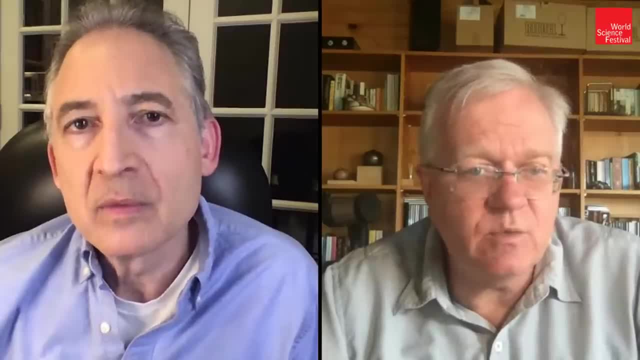 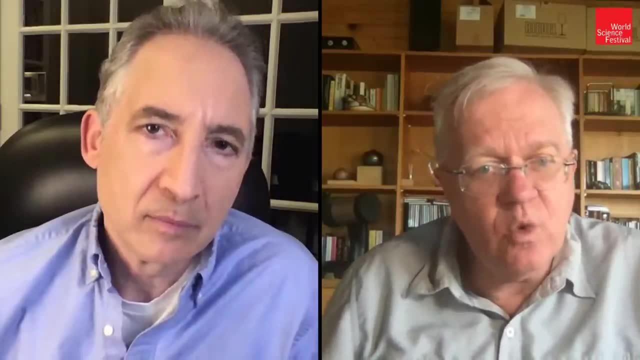 No, no, we. we did the full analysis and we said: the simplest is a cosmological constant. We then ran a paper directly after that where we used- we actually did a full marginalization over the equation of state priors. Uh, 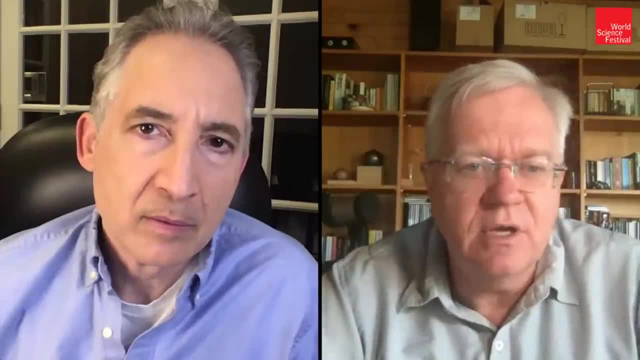 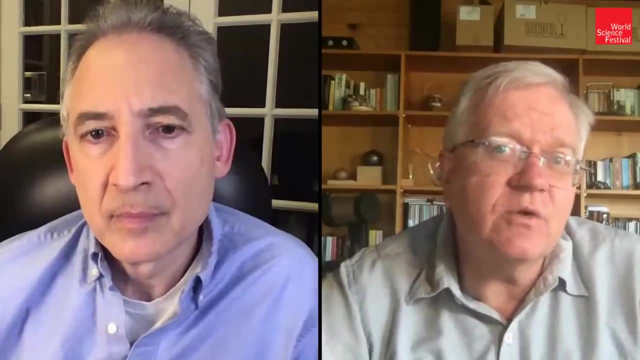 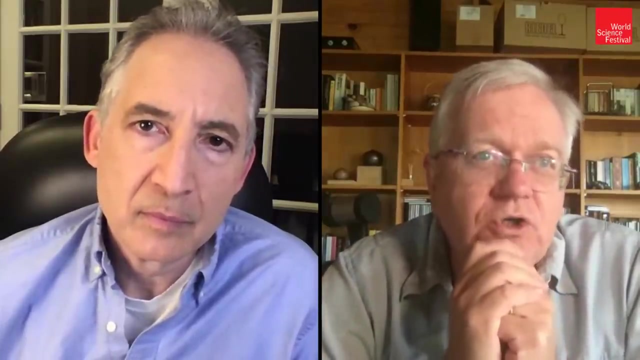 we had the earliest cosmic microwave background flatness priors. You could only do it with the fact, the idea that the universe was flat. Uh, and it's quite interesting things that people maybe you don't realize is that that 1998 paper was a full Bayesian analysis. 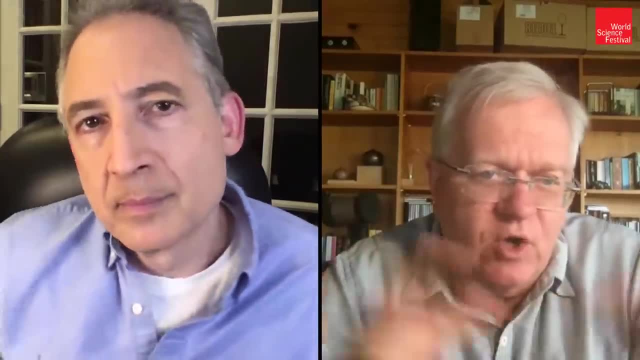 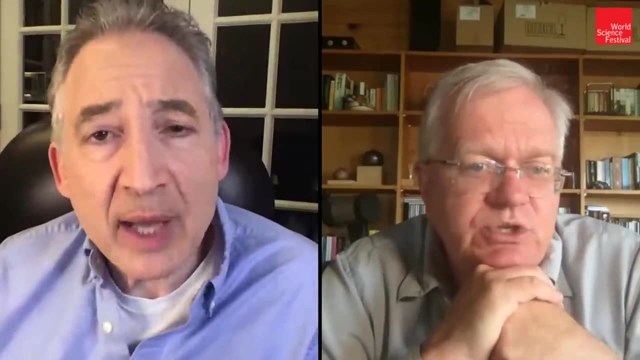 which is a way of doing statistical treatments, that it's the only way you do them now, But that is literally one of the first Bayesian treatments of cosmological data ever. Is that your? I did not realize that. Okay, Yeah, Well. 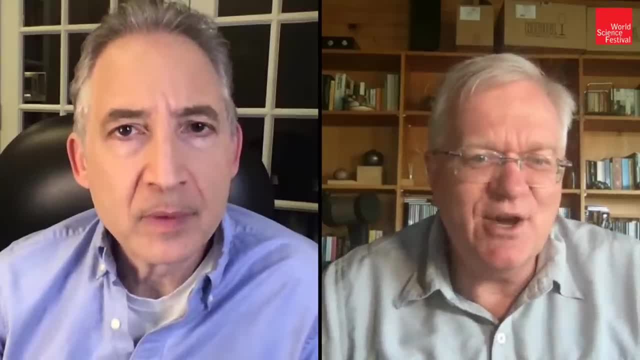 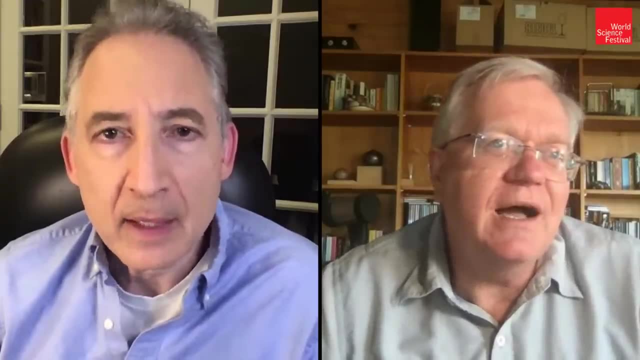 the problem is is I didn't learning of this in graduate school, while Adam uh, being helped by bill press, who was at Harvard and taught both Of us, uh, and my graduate advisor actually. So, uh, all right. 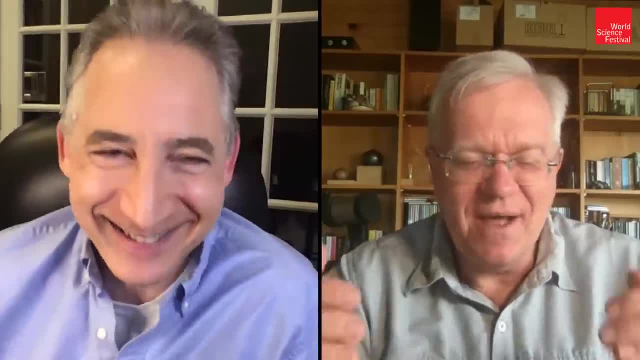 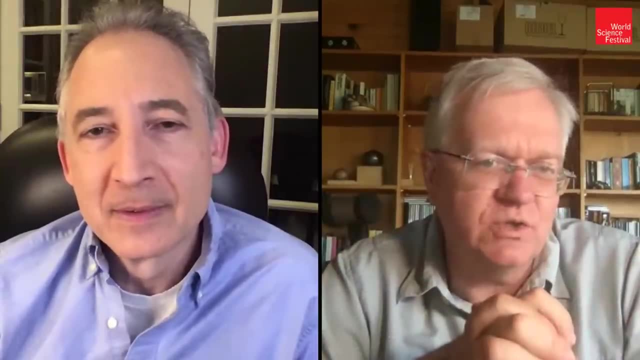 Okay, Well, there you can work in in some way. So we were learning Bayesian statistics as part of this, because it was almost impossible to analyze it using the normal methods of the day, because there's parts of the diagram You're not allowed to go. 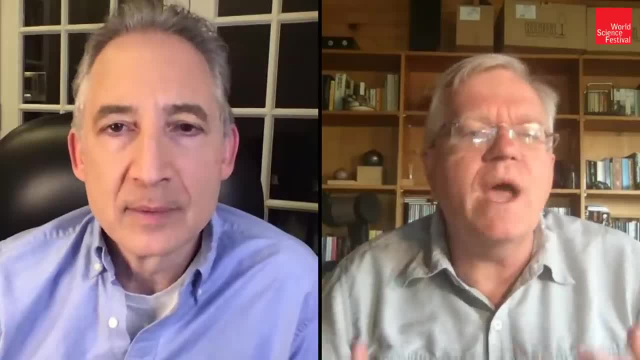 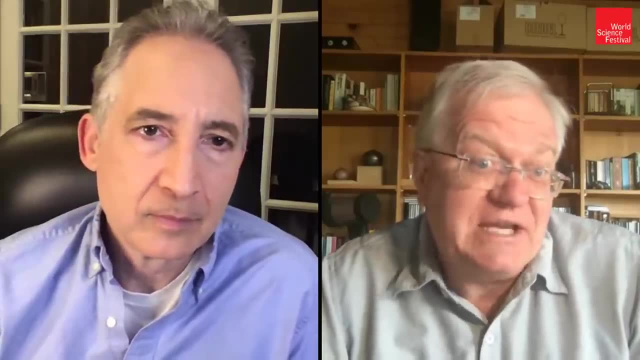 And with frequent is statistics. You just there's just no way to analyze to me like that. So, uh, it was quite an interesting journey, uh learning, uh all sorts of new things as we were doing it, Right. 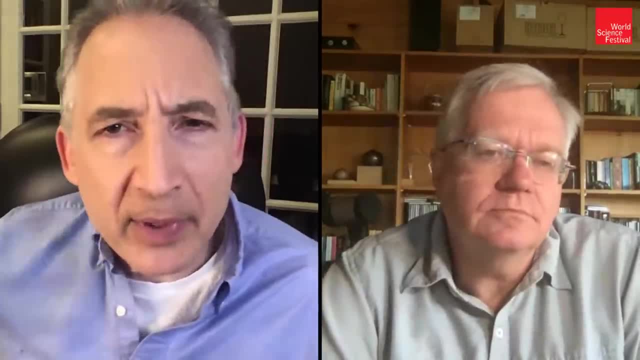 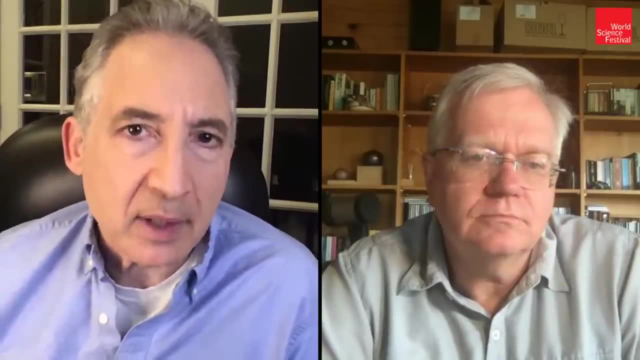 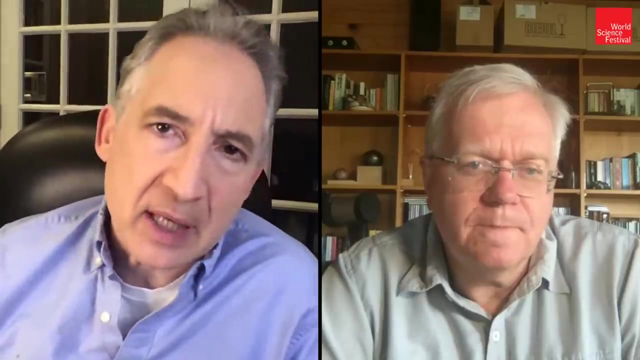 And and so, uh, by January, February, ish of 98,, the team is convinced that you've got a shocker of a result that the universe is speeding up in its expansion. Did you, did you, coordinate at all with the other team? 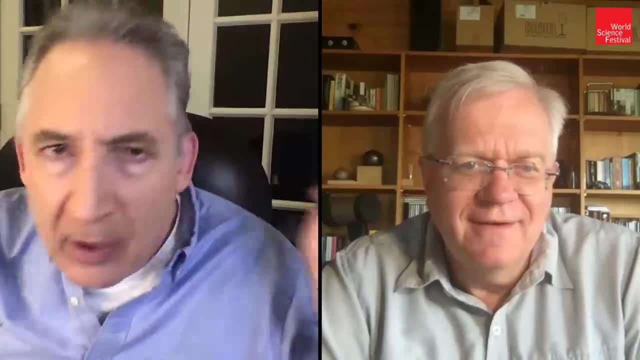 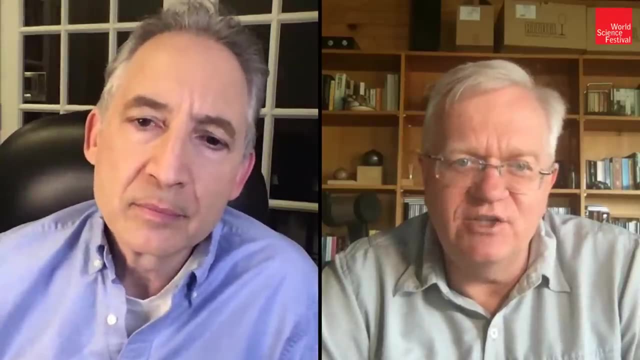 this all promo, or did you guys just? you know, let's just all go out and and make our announcement and just see what happens. Yeah, So it was, it was. Hey, it was very competitive at the time. You have to remind the two teams. 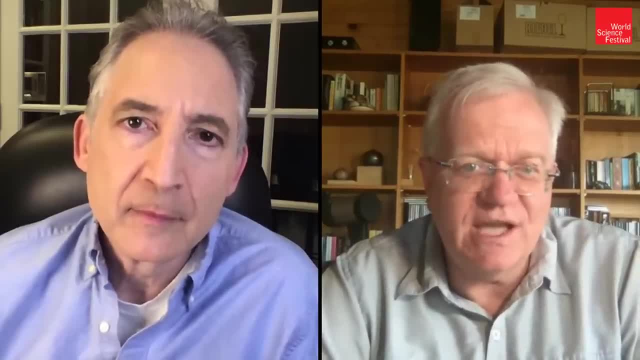 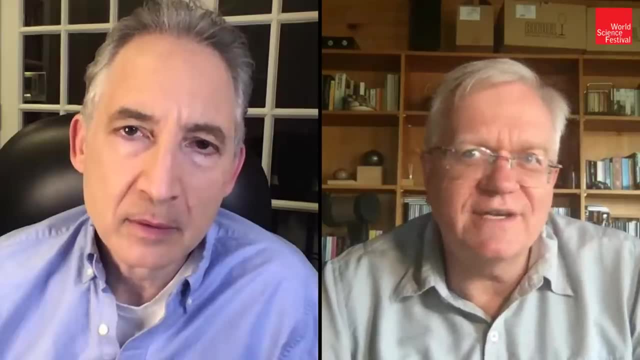 uh, I got along quite well with Saul, but I would say there was a lot of hot competition. Alex Philip Pankow had switched teams. uh, Saul and Bob Kirschner were having spats with Gerson Goldhaber and people in between. 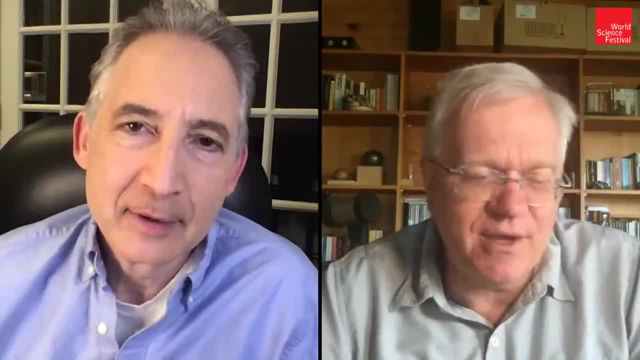 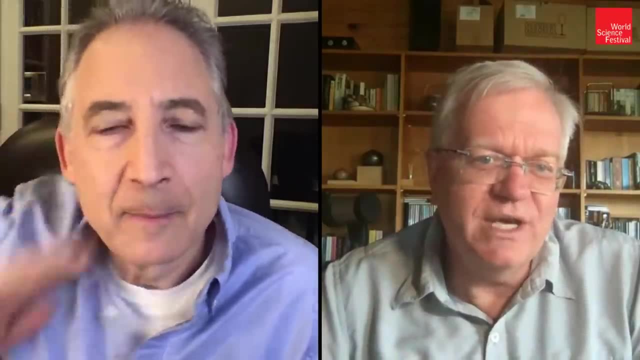 uh, Richard Ellis on their side, uh, throwing Spears as well, Uh, and we're all pretty good friends now, but I was pretty, pretty hot. I mean, I was pretty good at the competition. So no, we uh. 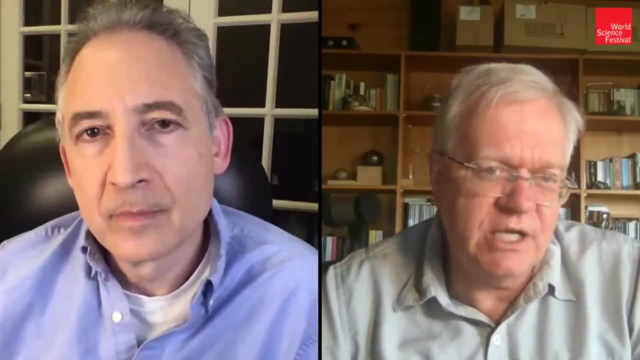 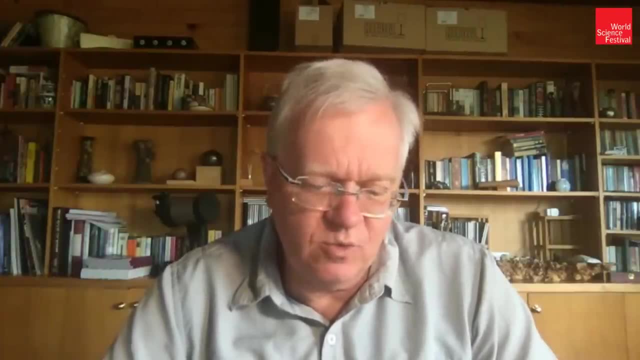 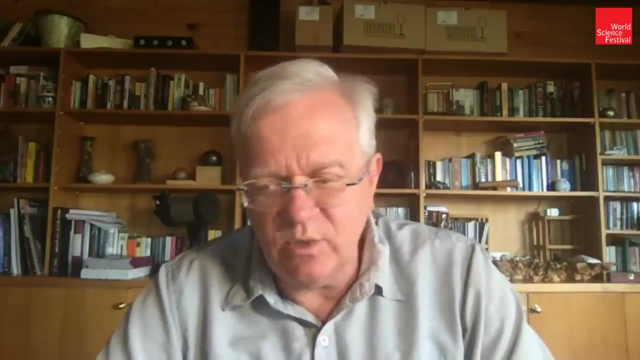 we did not, uh, share what each other P each people were doing. One of the interesting things that had happened is: on the 8th of January, We told our team: my God, the universe appears to be accelerating. on the 9th of January, 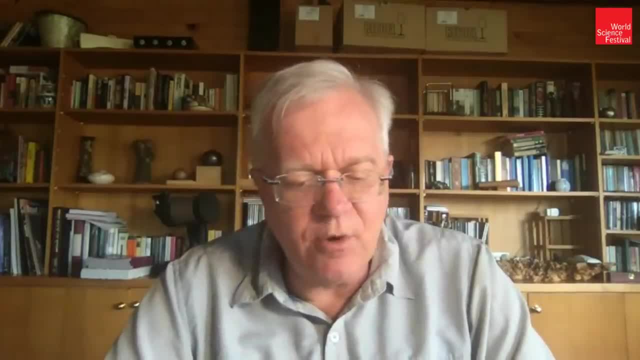 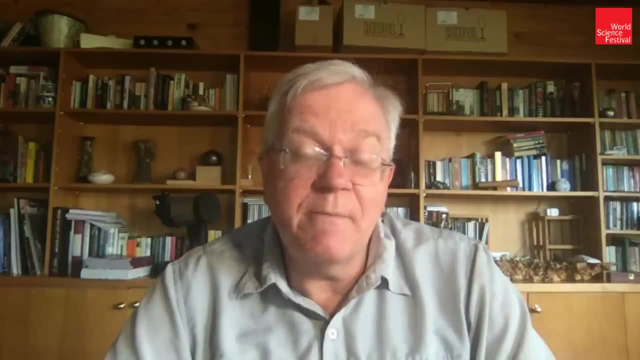 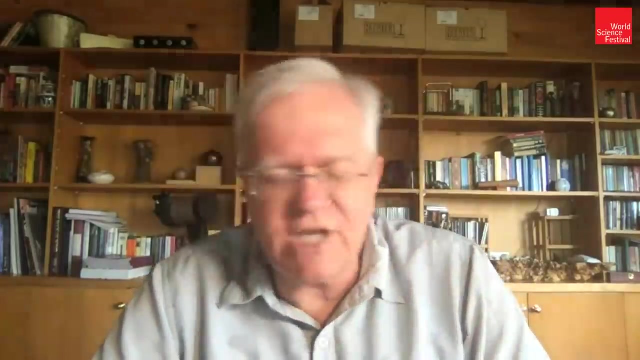 At least my time, This is Australian time. Saul Perlmutter showed preliminary results at the American Astronomical Conference which basically showed an accelerating universe, But they hadn't. you know, there was only in one color, They hadn't corrected for dust and all these things that we had already done. 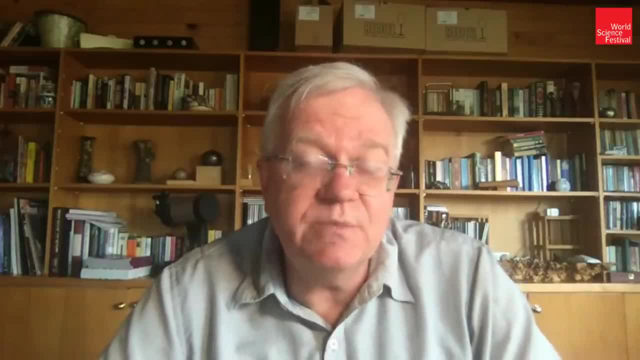 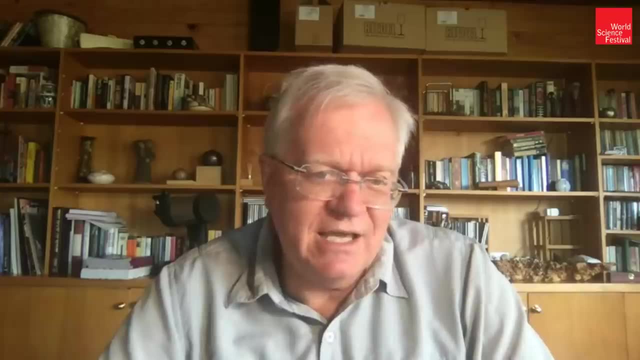 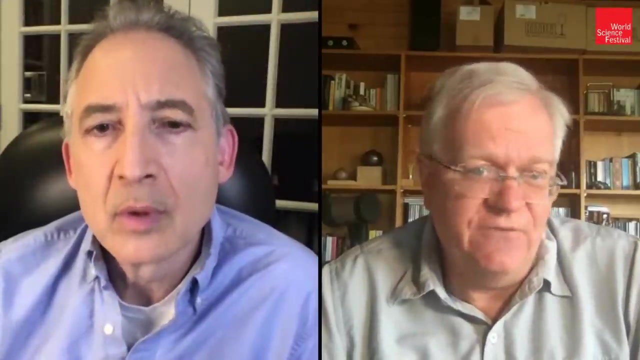 And so that was a big shock to us, because three months earlier they had essentially published a result that said the universe was slowing down quite quickly, So we thought we were getting this answer that was completely different to them, which I was going to say worrying me. 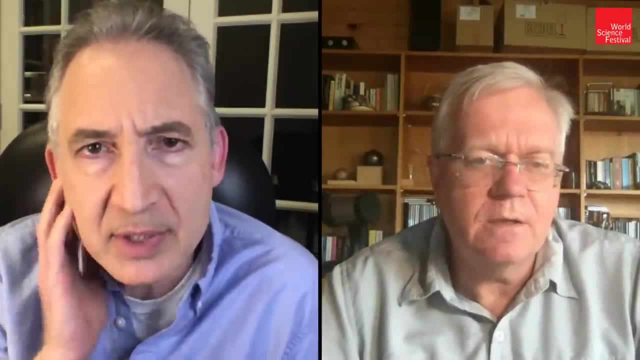 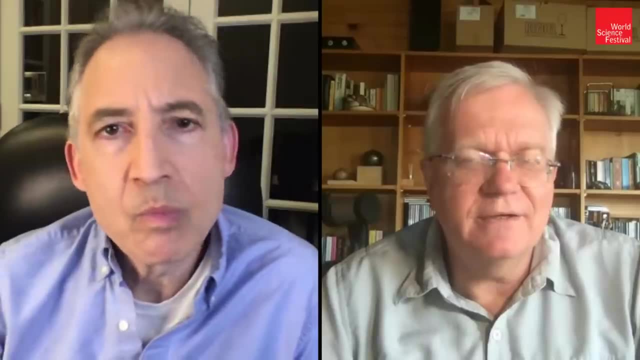 So how did that happen on Saul's team? Was there reanalysis of the data or I? they had a lot more data. Uh, I will just note I don't know It. I'll be honest, it still doesn't make sense to me. 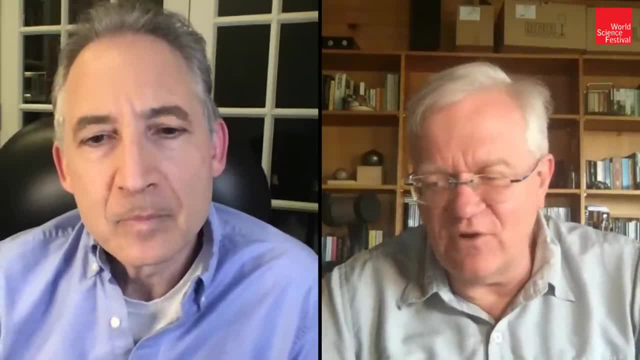 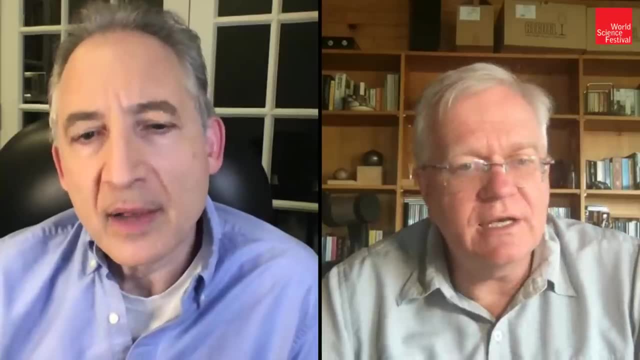 The uh, the consistency of those first seven objects that they published. they're just not consistent with the rest of the data- Man, I can't put it any other way- and they're not. They were not easily figured out in in their paper. 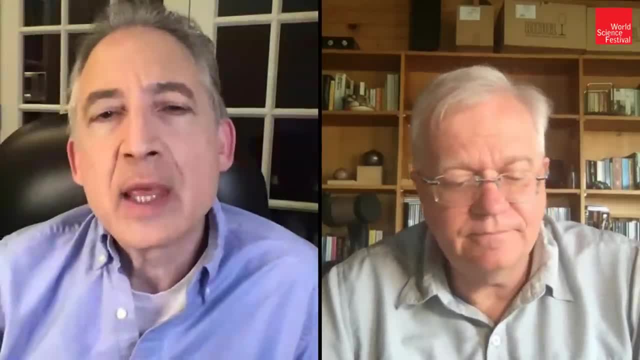 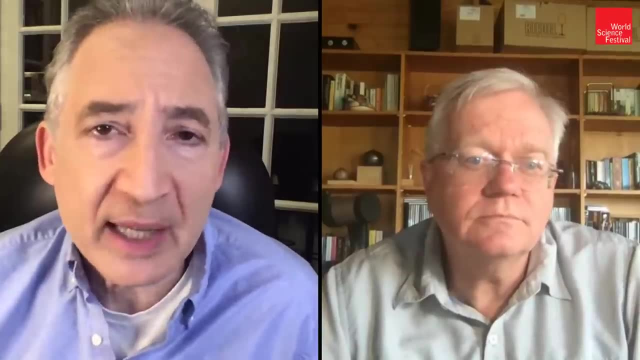 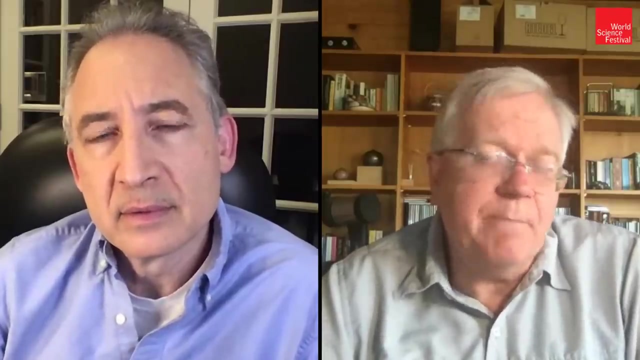 Um, I'm afraid. Uh, and so in the end of the day, would you say the competition was good for science or irrelevant? You were going to get there anyway. What role did it play? Uh, it was. it was good for science and bad for science. 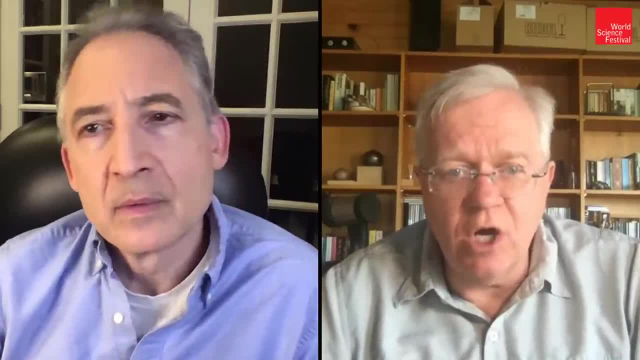 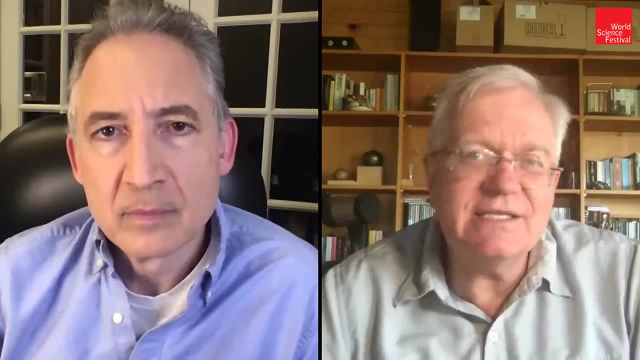 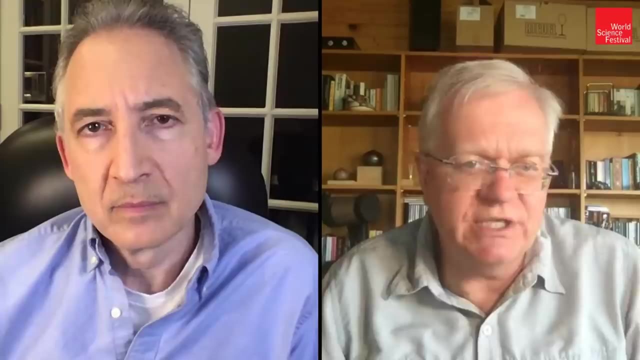 So how was it good for science? Um, we worked hard. We were careful, We knew we had another team That was going to spring us if we did any mistakes. We knew that we had to use the telescope time absolutely to highest advantage, because if we didn't, 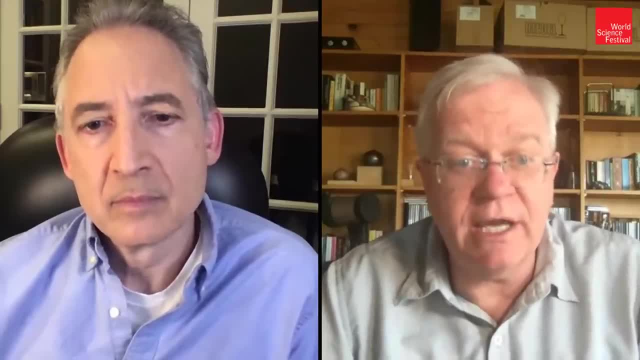 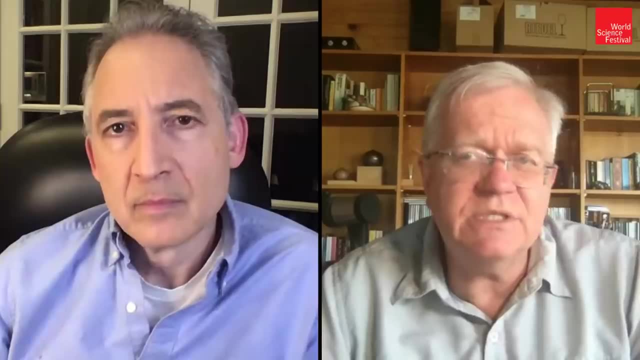 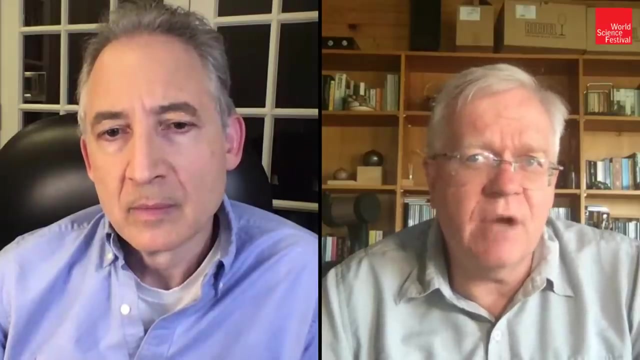 they were going to get it. So it really made us sharp on our game. That was good, But I would say the rather toxic atmosphere between the two teams would have been would have put young people off. Um it, it's not anything that I'm I'm proud of. 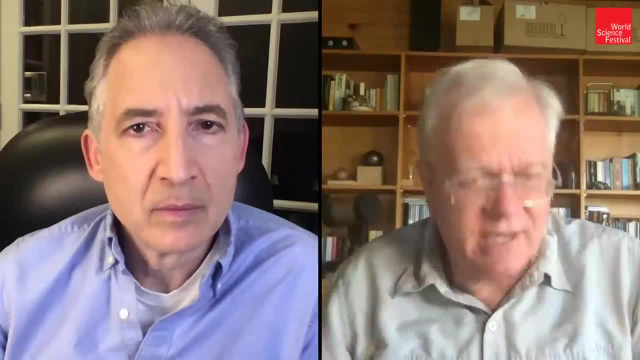 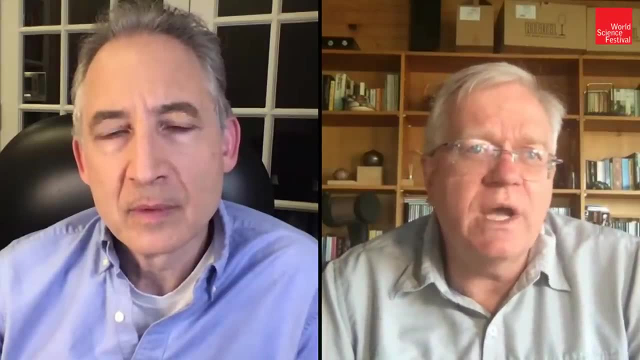 Quite The opposite. Um, and I will say here in Australia, I kind of kept my head down, avoided a lot of it, But no, I I'm not, Um, I don't, I don't think that's the way it. I think it's good to have competition. 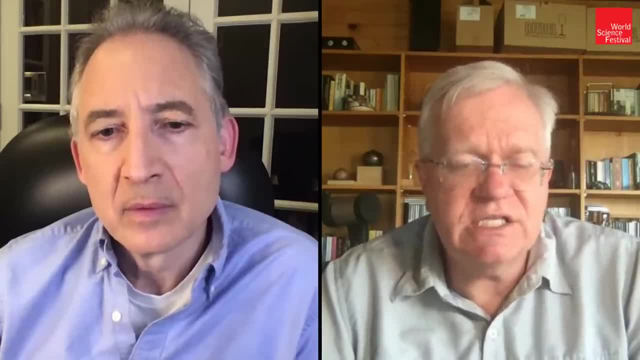 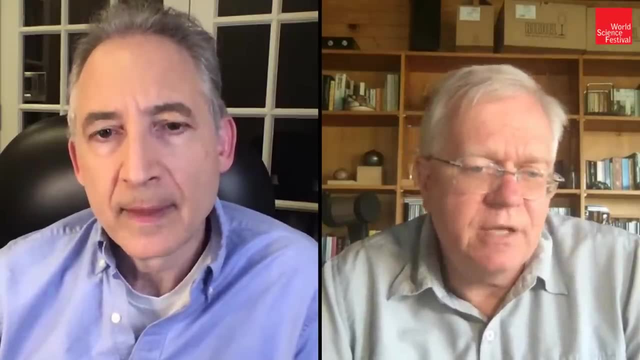 but it should be done in a collegial us, the best for science matter, And so I I think we were just a little too hot, to be honest, at the time. But you know when you're competing for finite resources and you feel like at any given time. 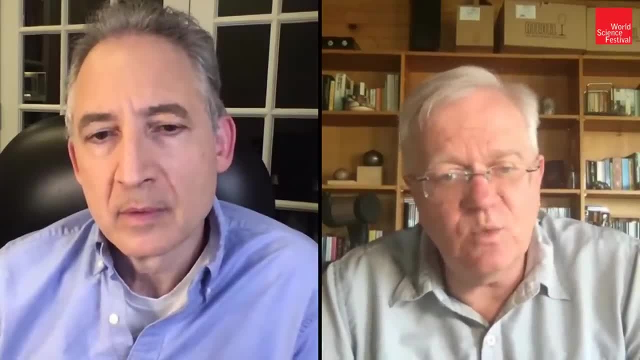 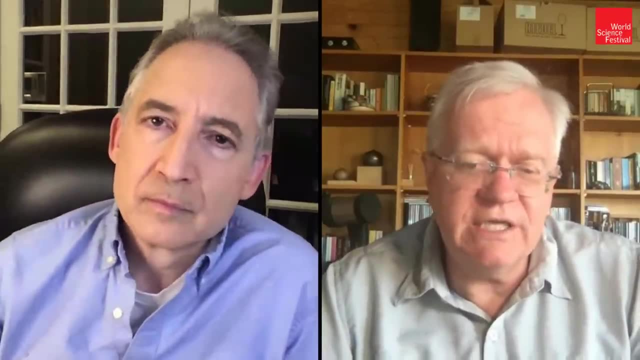 the rug is going to be pulled out From underneath you. you act in ways that is highly competitive, So it help us. And what it did help us really importantly is in 1998, when both teams basically came out with the answer at the same time and we were known for not getting along with each. 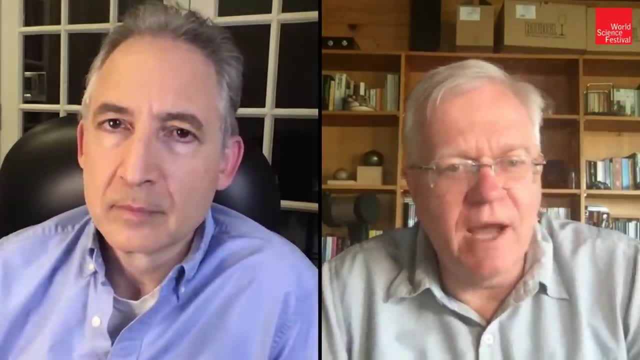 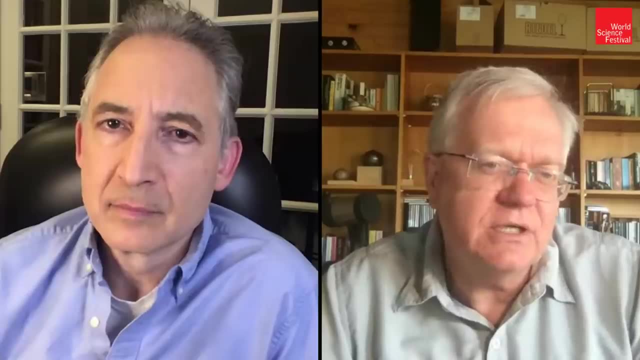 other people like yourself or Mike Turner got the megaphone out and said: this is real folks And so, rather than being laughed out of the stadium sort of like I thought we might be, uh, people took it very, very seriously. 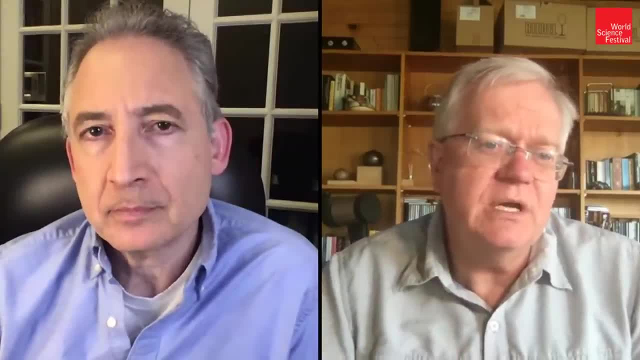 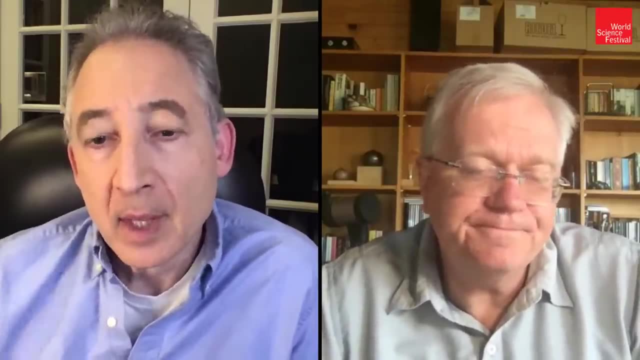 very quickly. So I think, having we would only had one team, I think it would have taken until the cosmic microwave background results got quite good to resolve. Right, right, No I, I remember being- I happen to be- at a talk that Saul gave around that time. 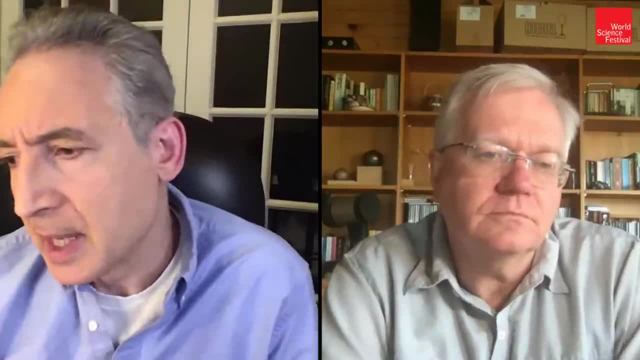 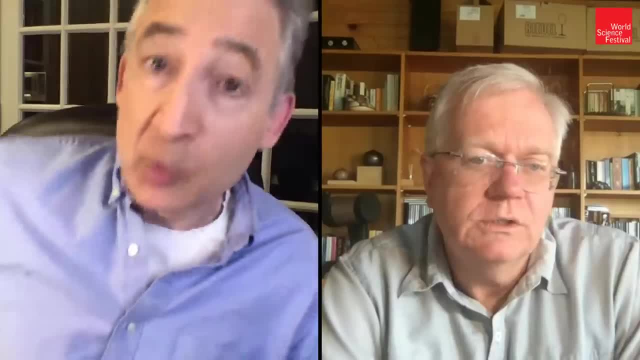 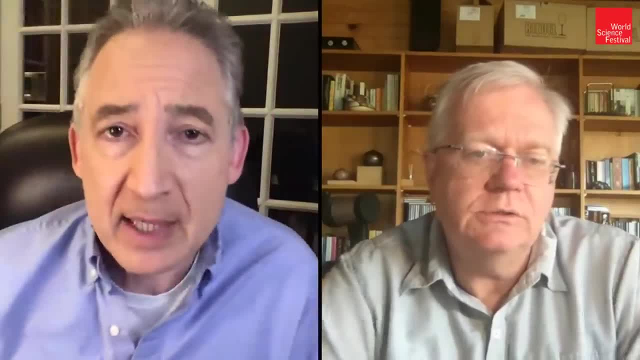 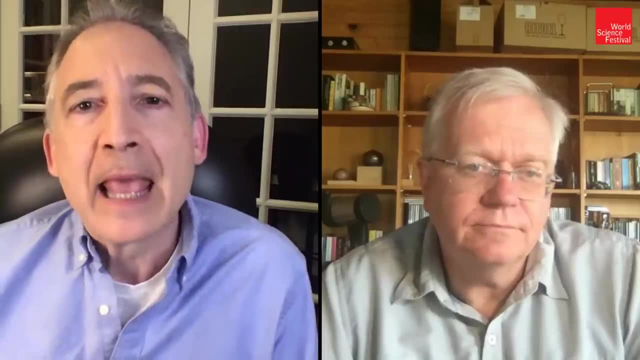 Because, As you're saying, Was Knowledge. that Too, independent teams. Were not Chummy, We're, we're coming, you know, to the same same result. How long did it take For the the heat to cool? 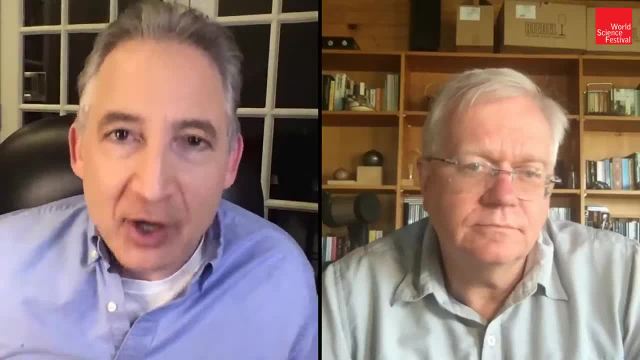 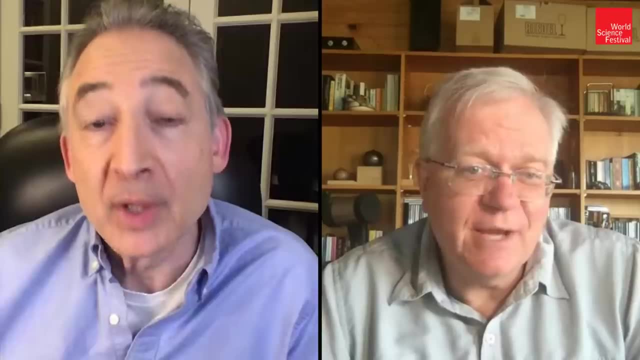 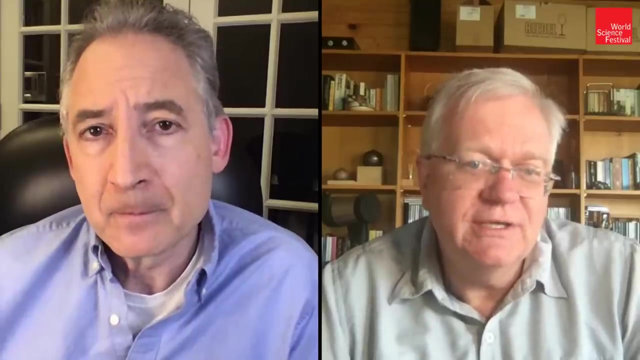 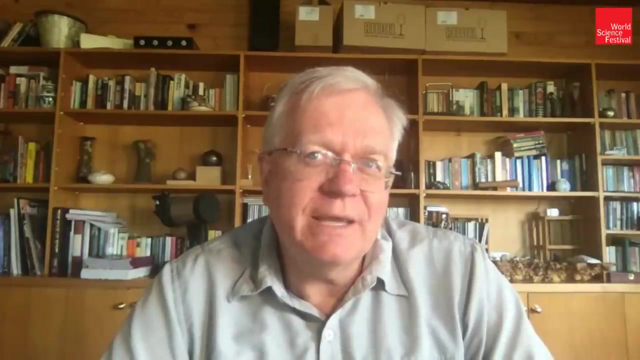 And turn into, You know, the camaraderie of discovery as opposed to the competition Of trying to get there First. I think it took to the Nobel prize. I mean, yeah, I think again I had a pretty good- you know pretty good- relationship with Saul, because I've been isolated. 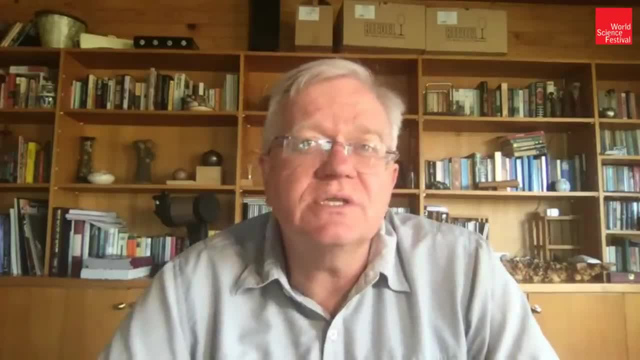 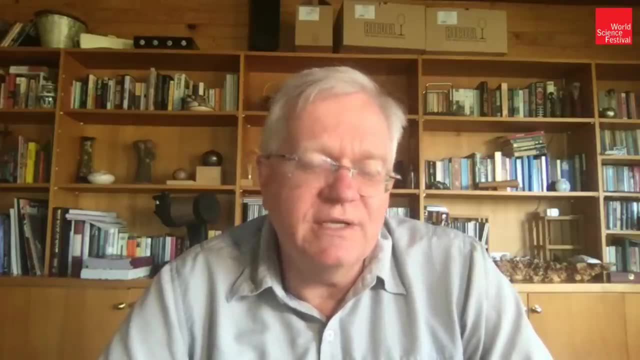 I'm not fighting over the same US resources as everyone else, So it it made it a little easier for me, But I things things remained pretty hot until 2011.. And then, when that happened, I think people made a decision that there was nothing to fight over anymore. 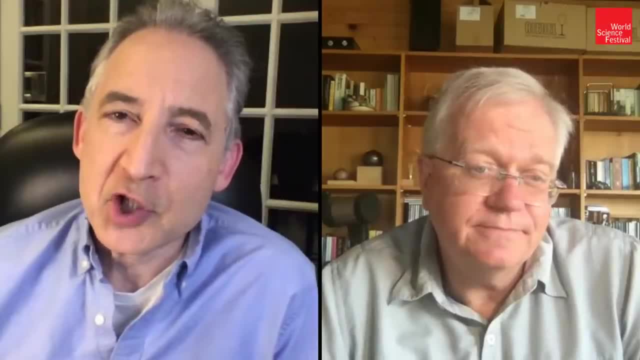 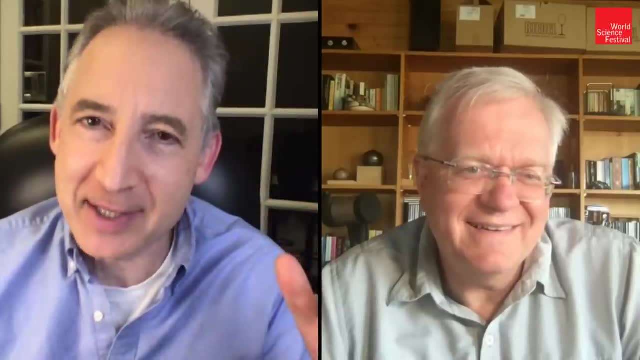 So I think that's how long. So the, the, the, the jocular photograph of you and Saul kind of duking it out. that was around the Nobel Prize time, I guess. Well, no, that was much earlier. That was in an Aspen meeting. 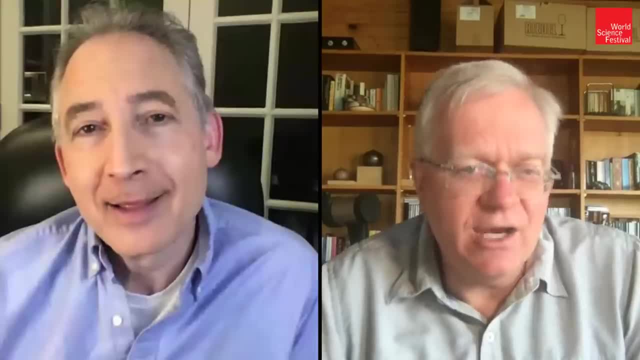 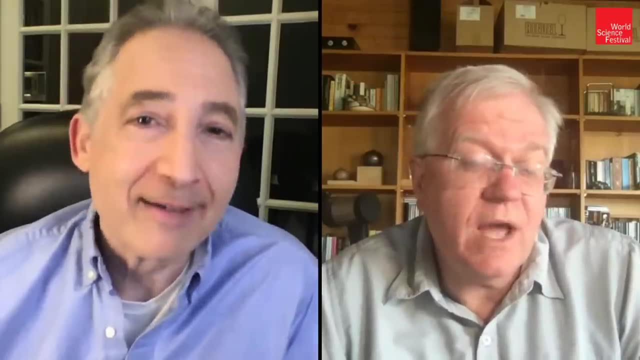 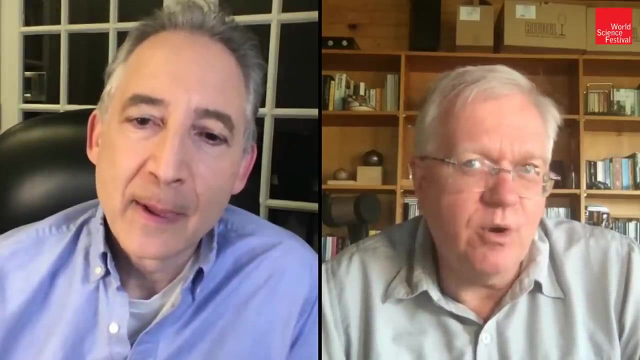 Oh and again, again. I had quite a good relationship with Saul, So that that would have been like a 2004 Aspen meeting, maybe around that time. But there still was a lot of animosity between the different power brokers, largely in the United States, because we're still doing competing projects for time. 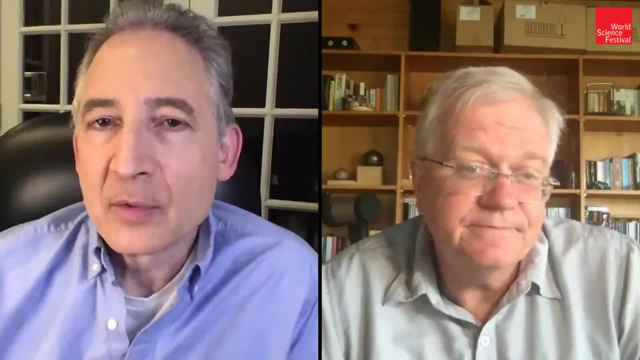 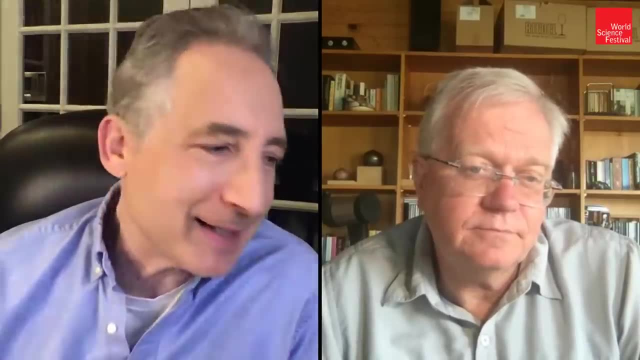 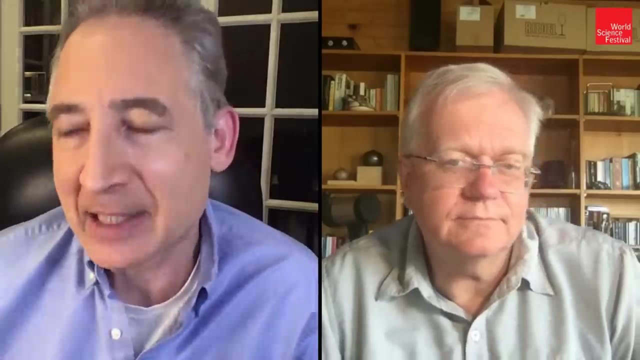 And, yeah, it was pretty competitive. So so the Nobel Prize is announced 2011.. You know that in many ways is the pinnacle achievement- At least that's how the public sort of views it- in terms of achievement, say in the sciences, physics in particular. 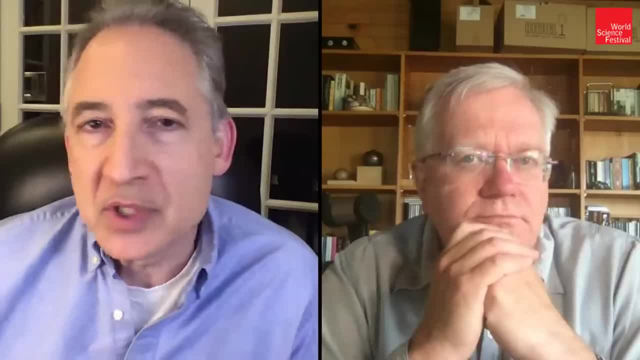 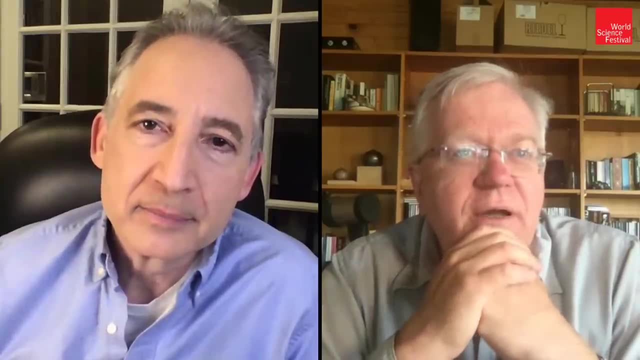 Was that a radical life changing moment or is it just: hey, this is cool, And you just kind of went on with what you would have been doing anyway? No, it's life changing And you know, Feynman described it as the worst thing that ever happened to him in his life. 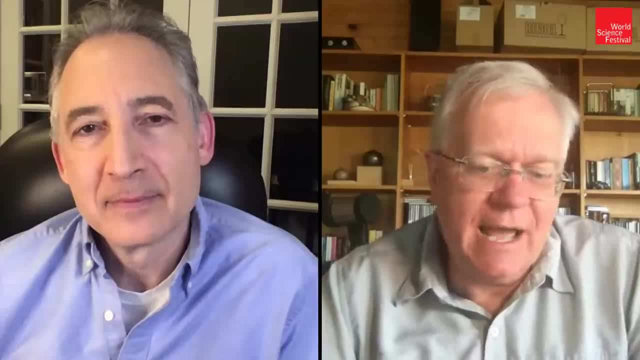 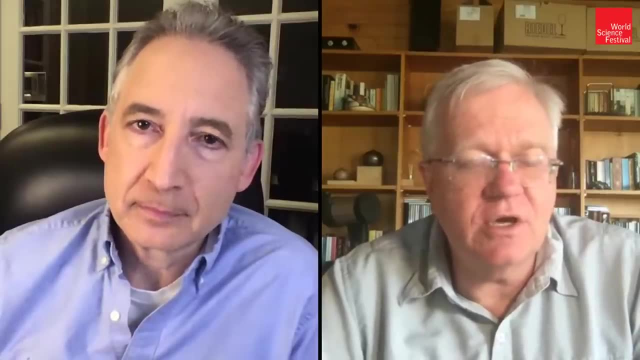 For me, you go with the flow and you're right. It is an absolute, especially in a country like Australia, where there's very A small number of them. it it changes your opportunities, but it also changes the demands on your time. 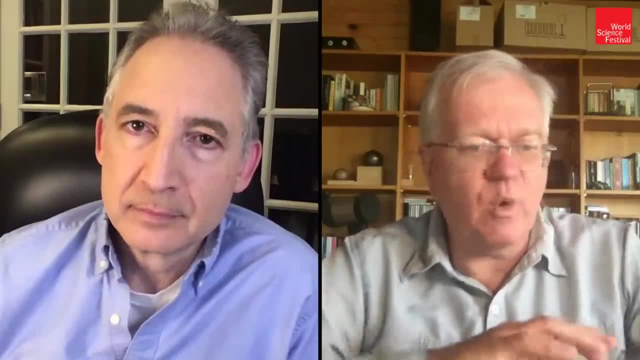 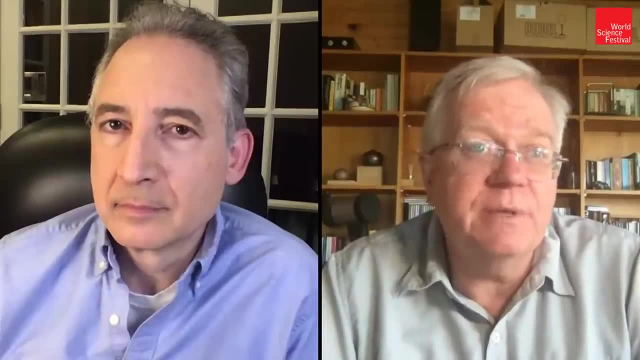 And you can. you can just put your head down and say I'm going to ignore all of the requests for my time and keep doing things, And that is a perfectly reasonable way for people to do things, But it makes you very unpopular, if I can be honest, amongst groups. 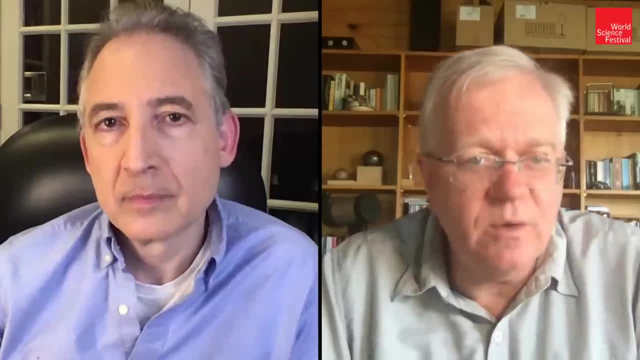 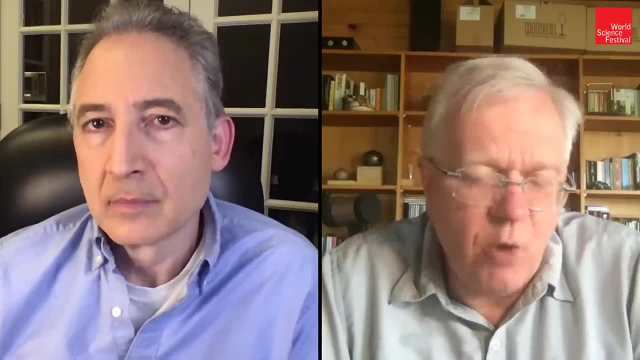 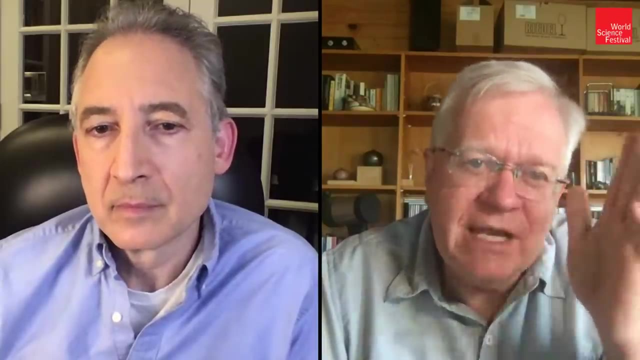 In my case I made the decision to go with the flow And you know I don't use it as a way of promoting science, but it does kind of eat you alive if you become a show pony and it is very difficult to to to maintain that focus that you need to really do your science. 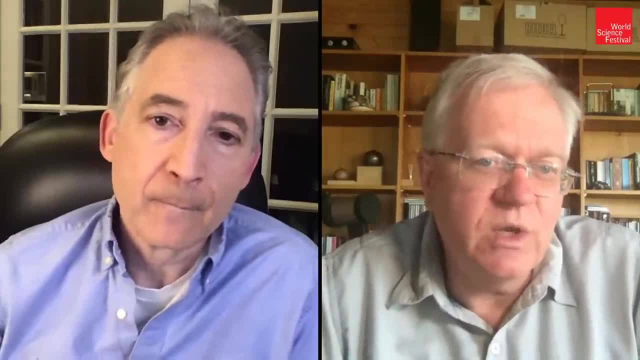 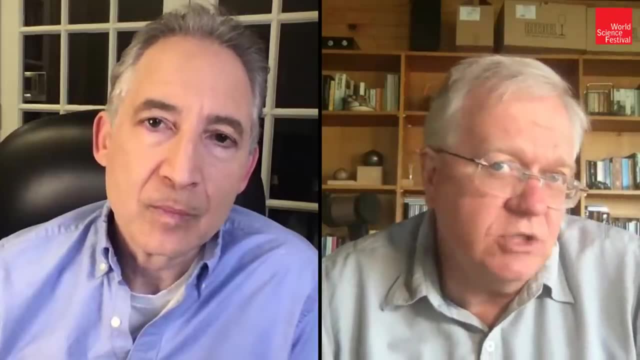 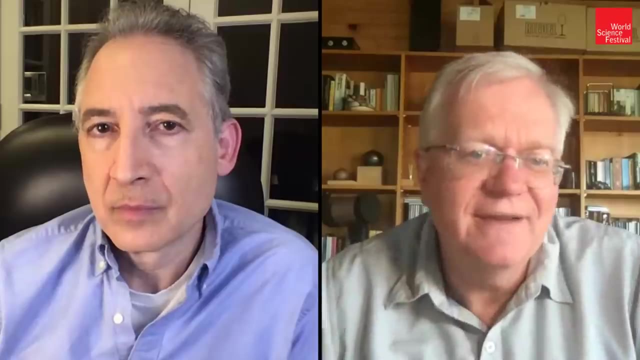 You know you don't do science 10 hours a week between meetings. You do it by focusing your efforts to answer things. So it was challenging And ultimately, the reason I am running a university right now is for me to grab my life back and to focus on something. 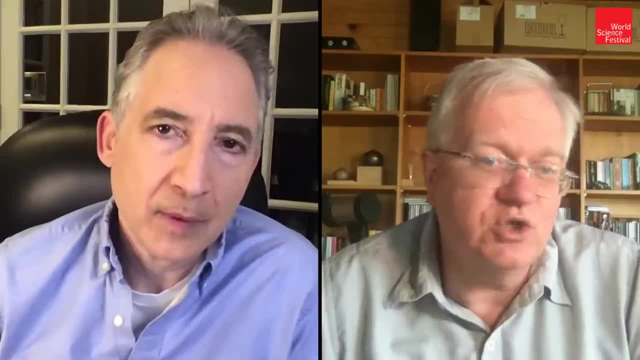 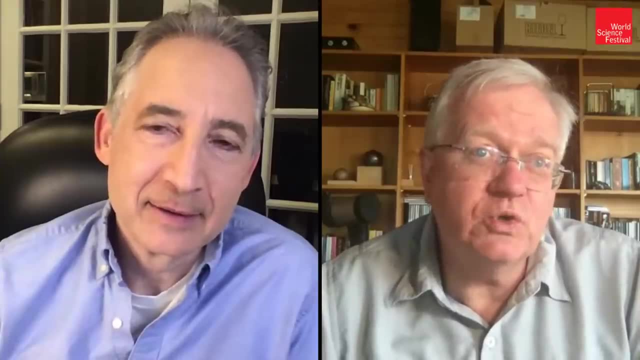 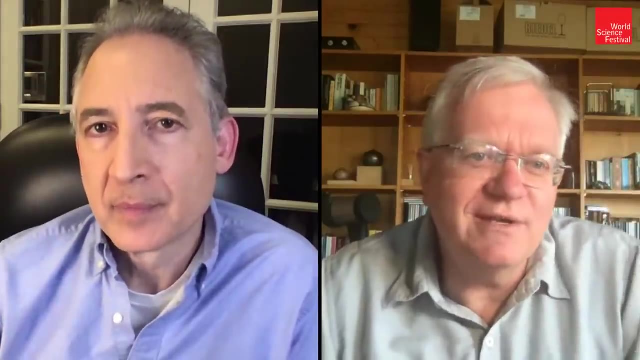 Now, running a university is not anything I ever thought I would do, completely antithetical to my interest 10 years ago, But it's been. it's been a place to- to recapture my, my focus, It's- yeah, it's. I wouldn't recommend it for most people, to be honest. 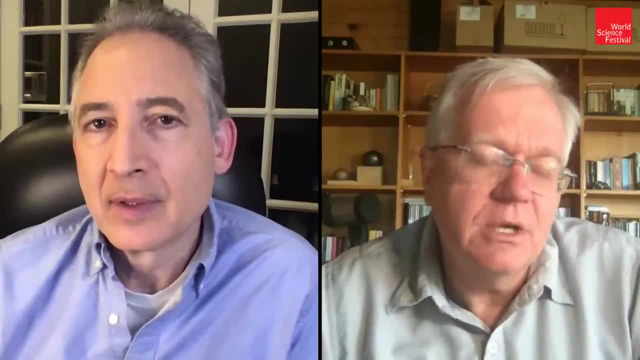 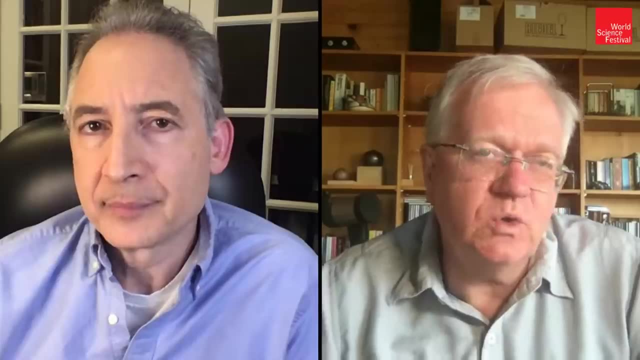 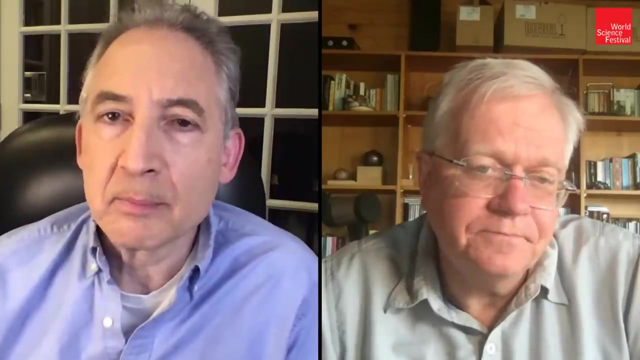 It's. it's an incredibly challenging Job, but it does allow you to do things with the. I guess that the Nobel Prize opens doors and it gives you the opportunity to do good that you just didn't have before. Have you been able to mold the physics, astronomy programs in a way that you feel has had impact? 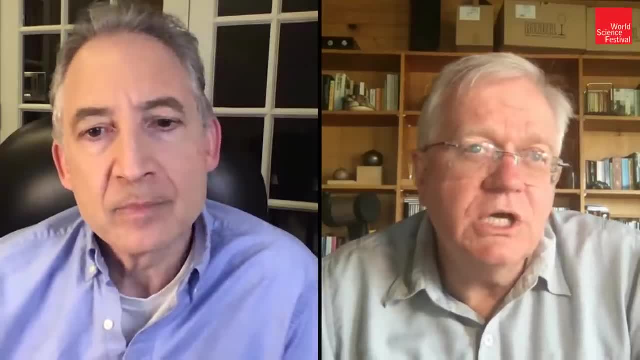 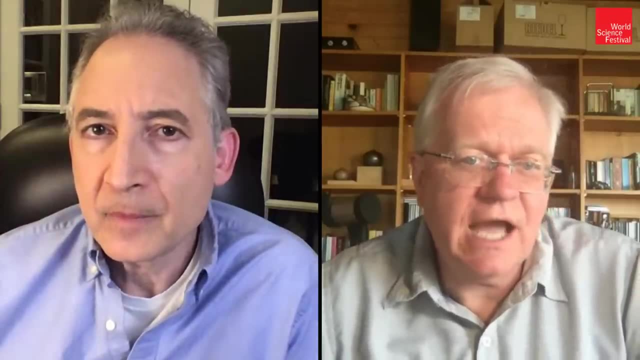 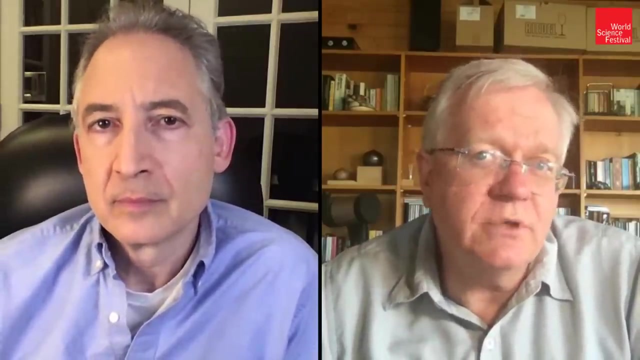 Is that? is that a part of the focus? Certainly in before becoming vice chancellor, Astronomy in Australia is very Much a whole of country activity. We, we hang together, because if we don't, we won't survive. So we were able- and I was able to help a fair bit- ensure that we had a vibrant astronomy program. 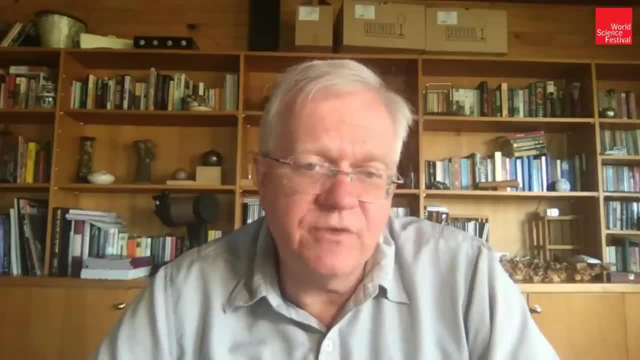 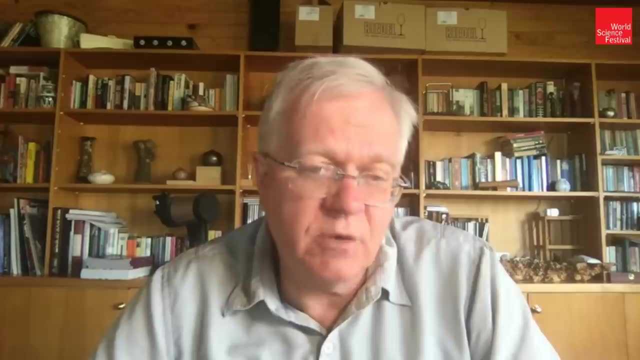 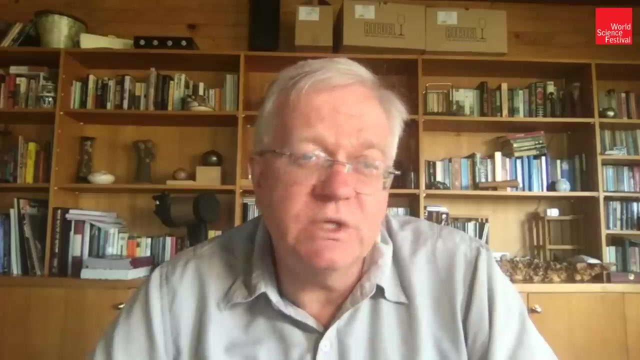 And so that means that Australia is part of the giant Magellan telescope, We're part of ESO, part of SKA, So we have a very vibrant, strong astronomy program that I was not alone but helped to grow Now as vice chancellor of ANU. it's not just physics. 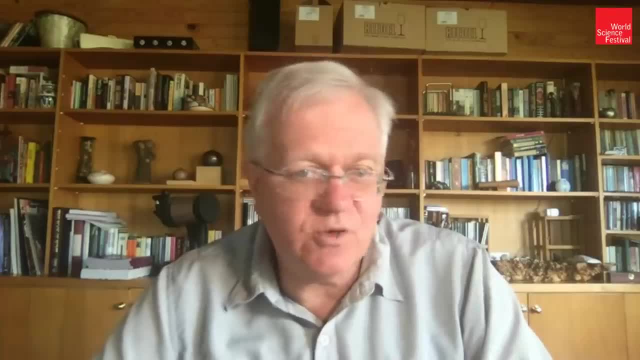 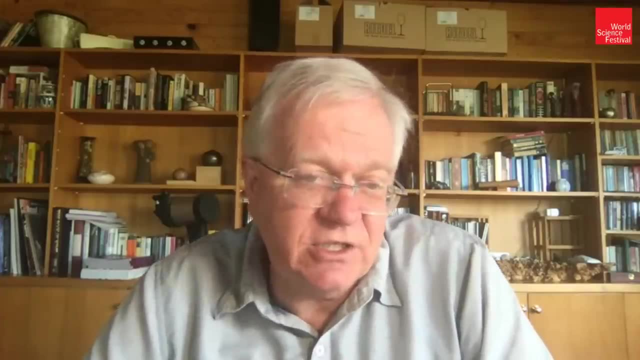 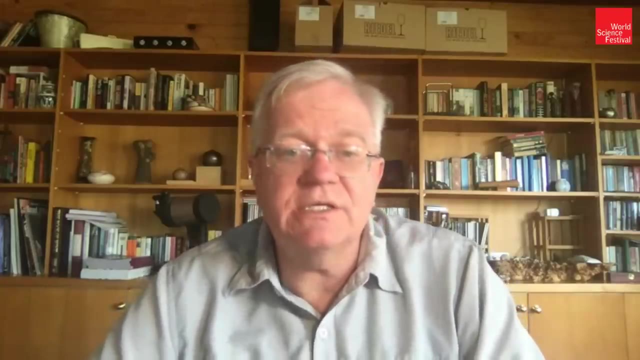 Of course it's. it's everything, including questions around our democracy. How is science done? How do we translate science into things and stay connected to the community? How do we ensure that right now, you know, 75 percent of Australians still see universities as a highly trusted institution? 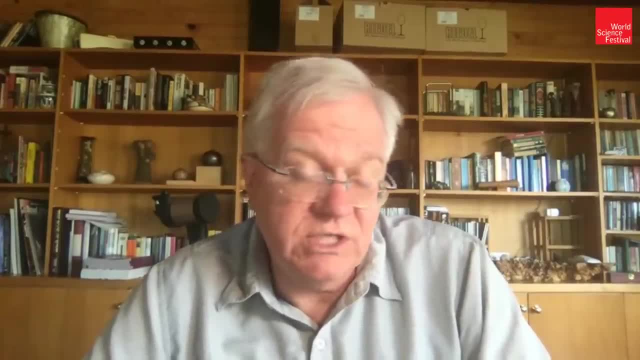 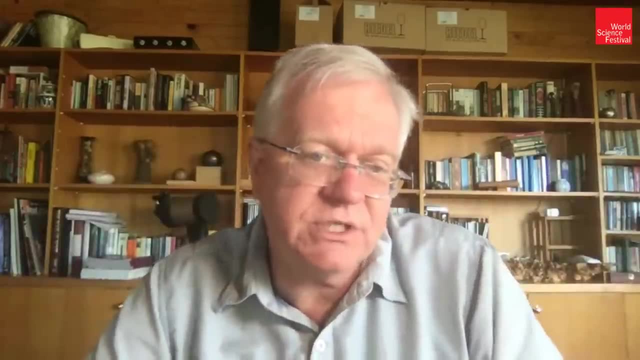 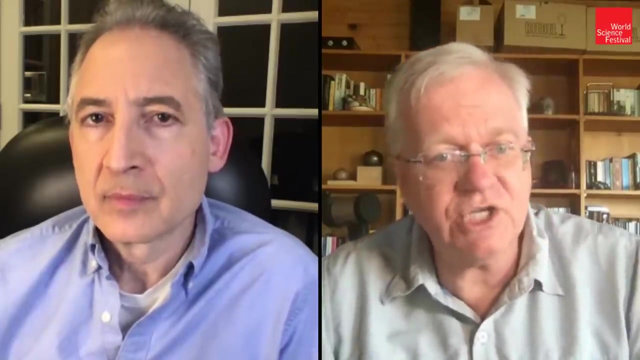 the highest, most trusted institution in Australia, where you will see, of course, in the United States universities, trust has plummeted. So you're really playing at the very highest level of the democracy when you run the National University, And that's you know. I would have never thought that would be something I would do, but it's something I'm passionate about. 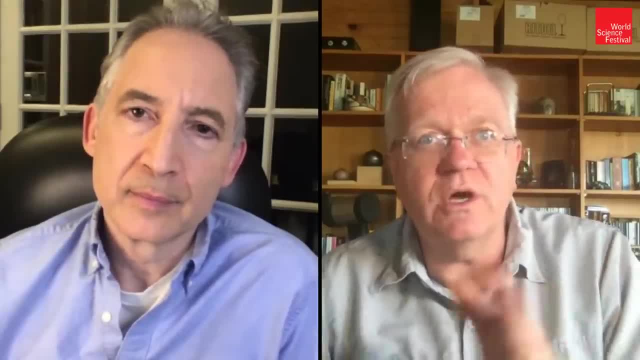 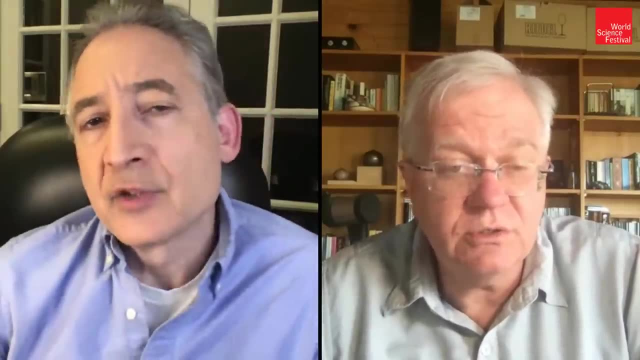 And it is something where I want to ensure that Australia doesn't go down certain paths that I've seen the US go down, because it's been tough to watch. So, based on that experience, especially as you've lived in both countries and, I assume, still have a 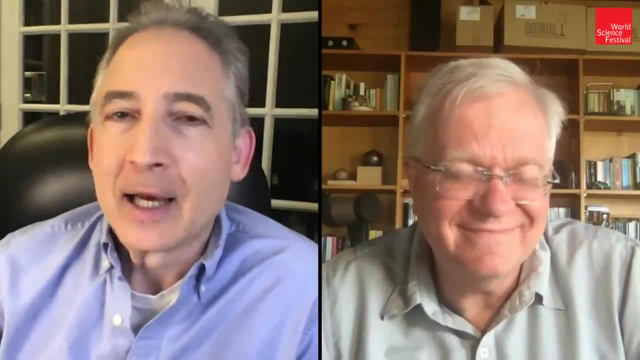 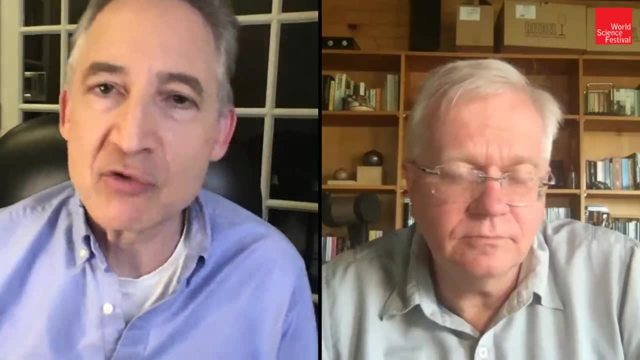 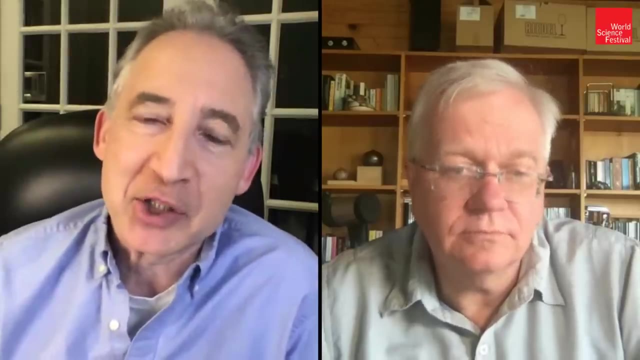 Certain affection for your country of origin. what, what advice do you give us over here? Because, look, obviously the transition from the previous administration to the current one is a step in the right direction, But there is a significant fraction of the general population here, as you're saying, who distrusts expertize. 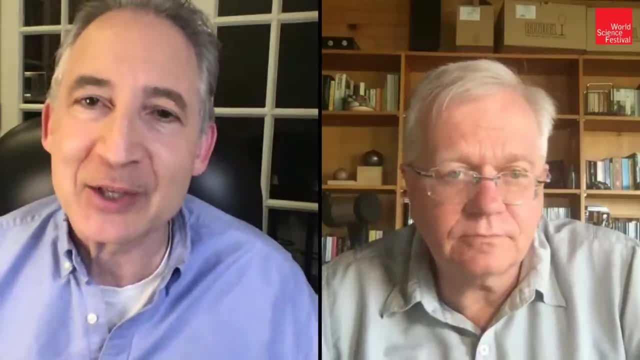 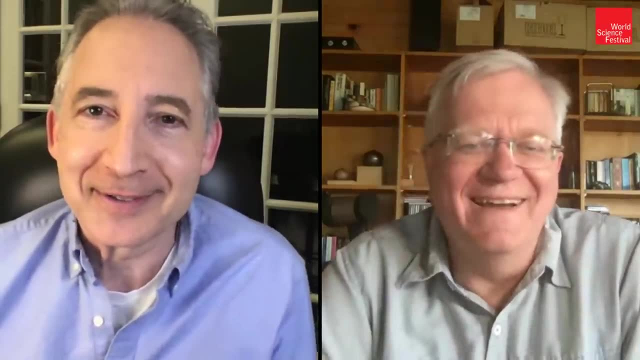 who distrust anybody that has anything to do with a university? And I'm asked this question all the time: What do we do? Thankfully, I can now ask You that question. you know well, the Dutch have an expression that I think is, I think, very telling. 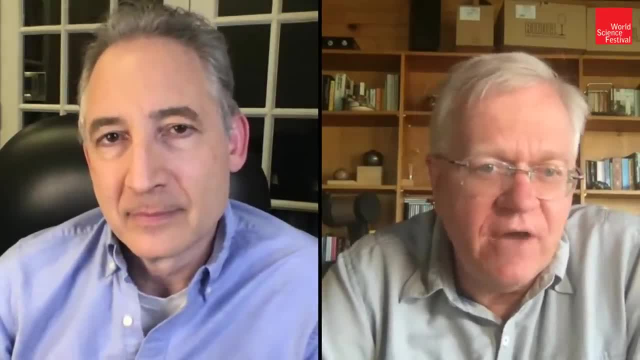 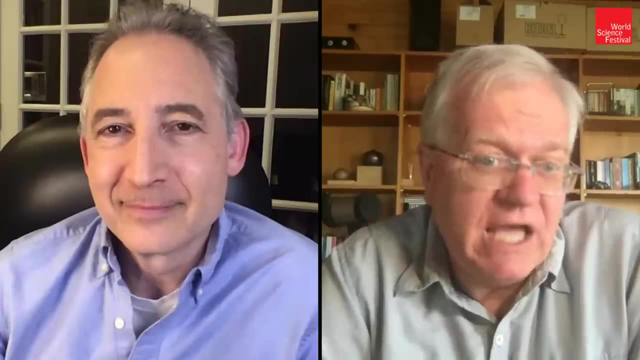 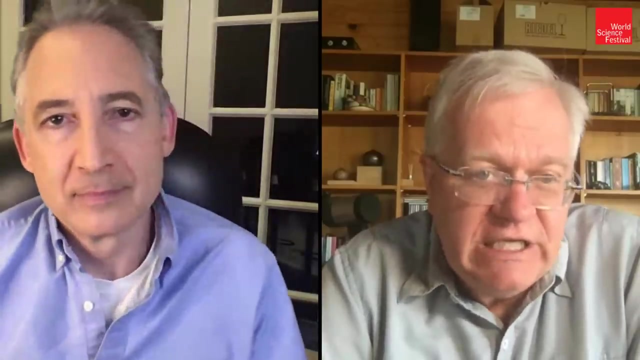 which says that trust comes in by foot and leaves on horseback. So the reality is a lot of that trust has gone and it is going to take a long time to build back. You would think COVID-19, which has done a lot to rebuild trust in Australia. 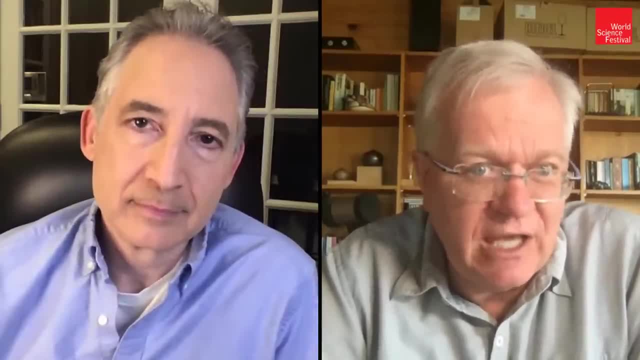 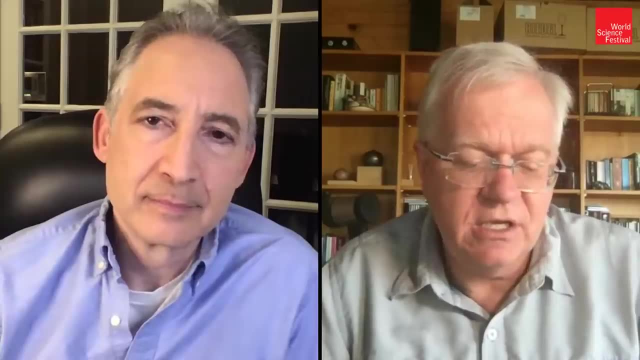 is not going to do anything And we have seen over time that that has a very positive effect on the local economy. But I think- at least in my opinion- we are now seeing a little bit less of a positive impact on national relationships. I think it is a little less preaching because we're all talking about the kind of trust that we have. 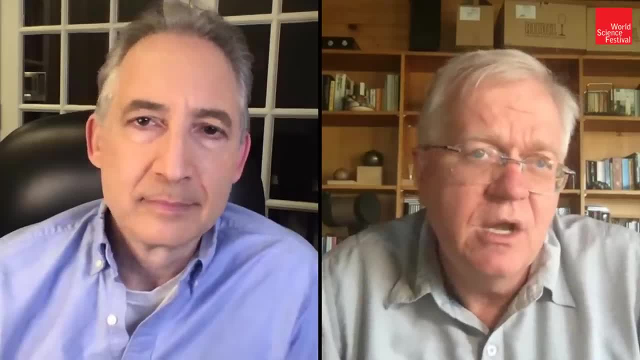 And you know the state of emergency that we're talking about is so strongly focused We have had for a long time. There's a huge shift in the government movement and the public policy that we've been doing, And there's a huge shift, of course, in the government, I don't think in the international community. 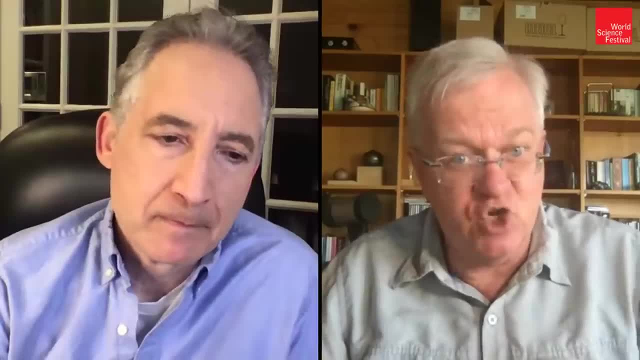 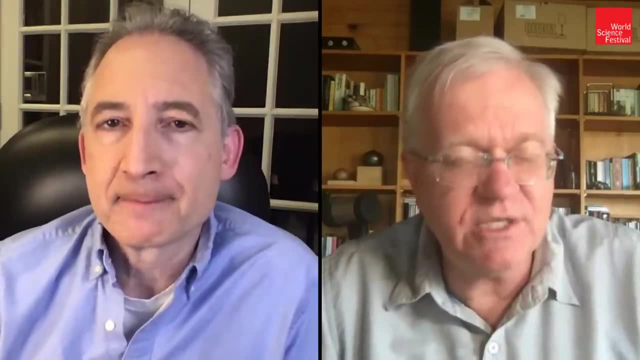 But there's an increasing interest among some skeptical because it has literally been life or death. That clearly has had some effect in the United States. But I think it is a little less preaching. It is noticing and understanding polarization. People need to understand that US enemies have used polarization to break the US apart. 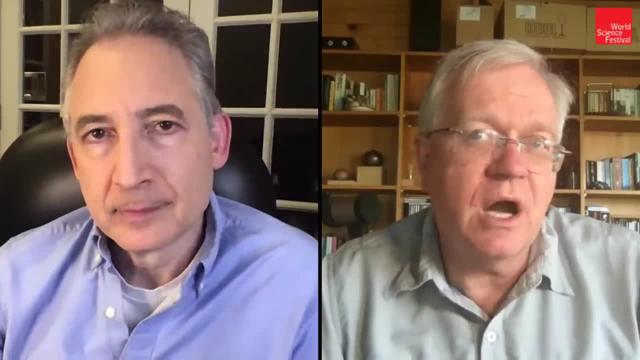 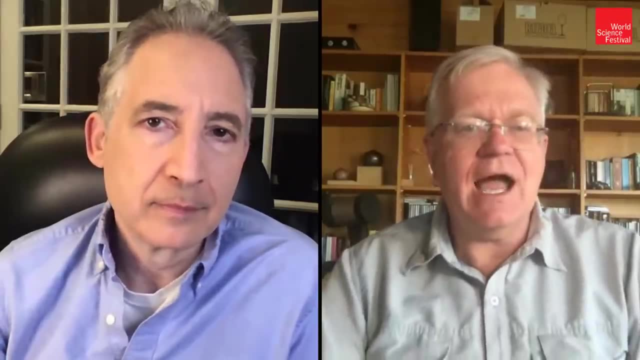 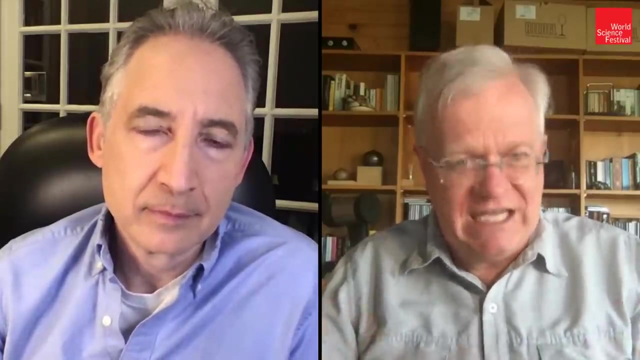 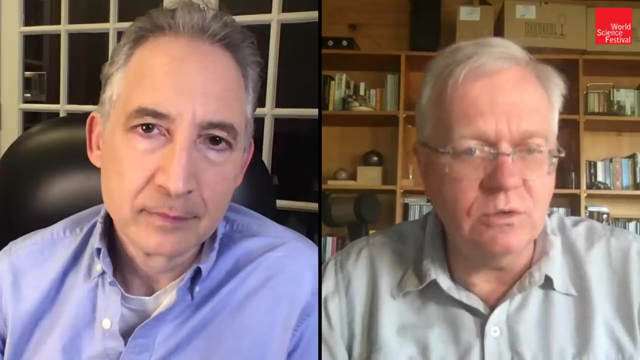 And I think universities need to step back and, rather than saying, but we are right, you are wrong, even when that is true, to say: how are we going to bring social cohesion- And that is, reaching out, listening and bringing in the people slowly, bit by bit, person by person, into our fold of prosperity? 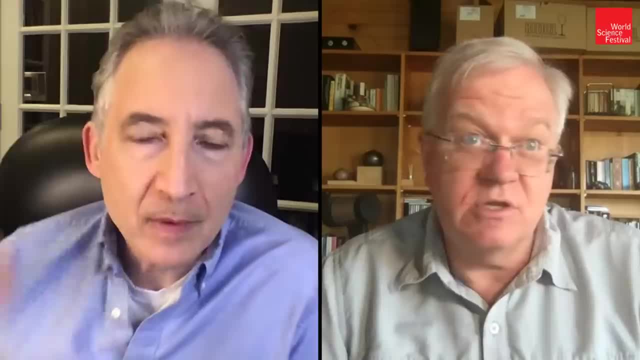 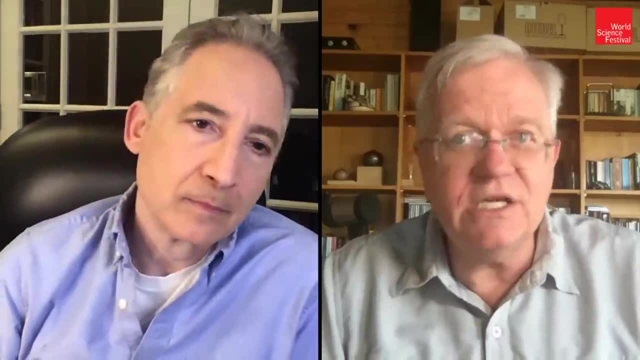 I mean, the reality is In the years to come, if you want to be prosperous, you want to be connected to that university scene and we need to go into the little towns of, you know, of the south of the Midwest where I grew up. 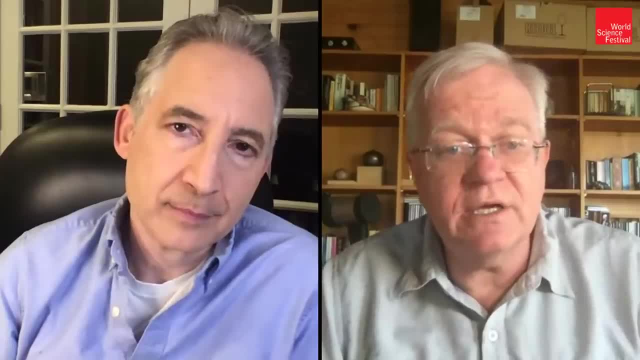 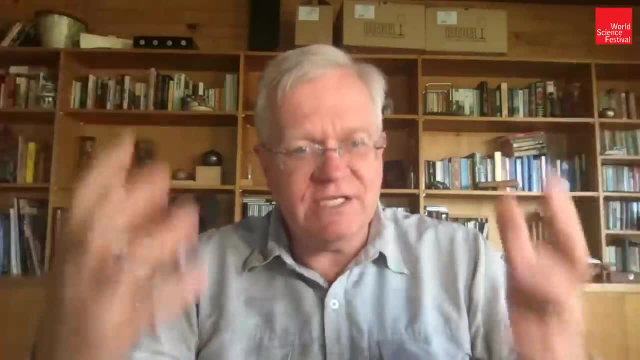 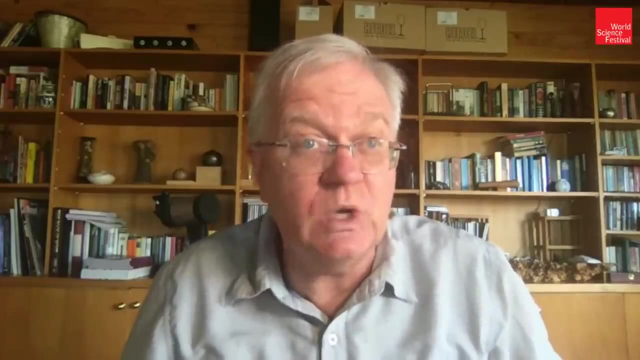 My family are from those places and we need to reach back in there, make sure our alumni and people who have gone out go back there, tell the stories, make sure the sons and daughters of those parts of the country are welcomed and have a place and listened to, even if you don't like what you hear. 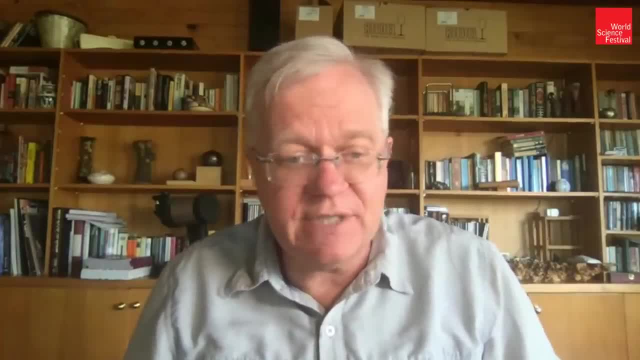 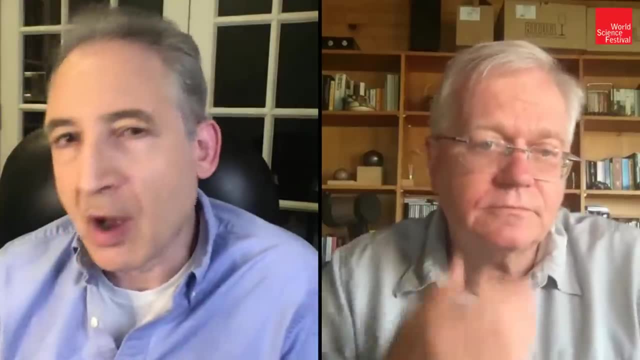 So I think it has to be a big project. But just getting up and telling people they're idiots turns out not a very good way. No, it's hugely refreshing for me to hear you say that. Yeah, Yeah, Yeah, Yeah. 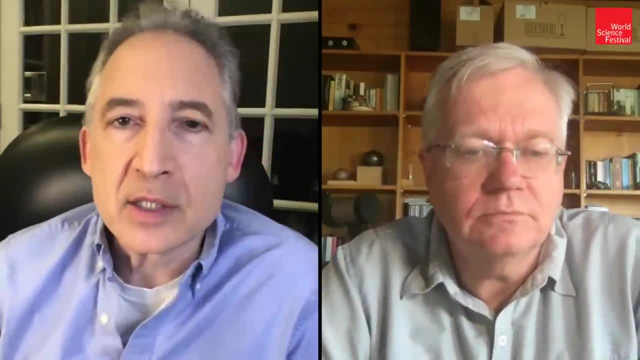 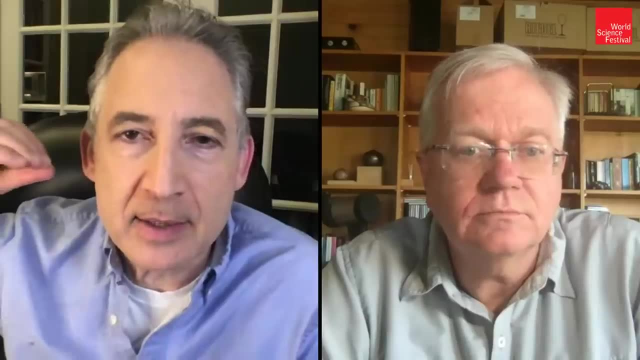 Yeah, Yeah. Oftentimes the conversation over here assumes that people come to their beliefs about the world through some kind of very systematic sequence of rational judgments. You look out at the world, you judge the data, you come to a conclusion and nothing could be further from the truth. 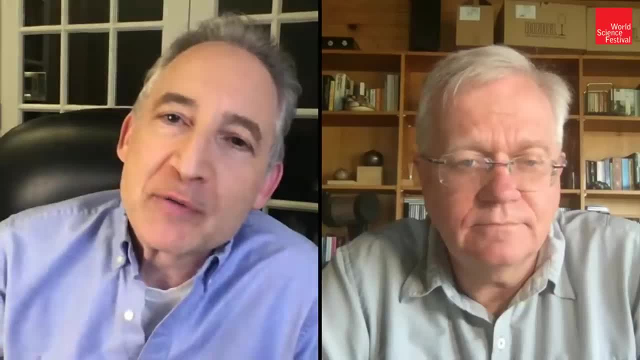 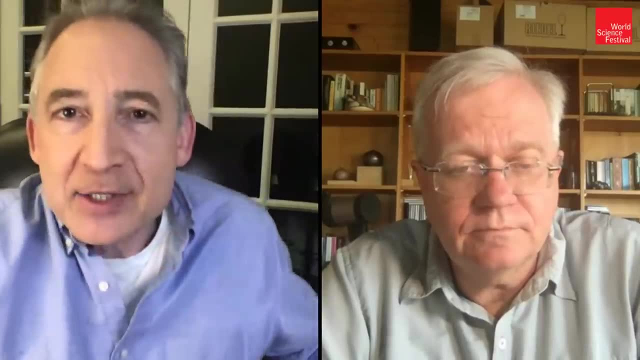 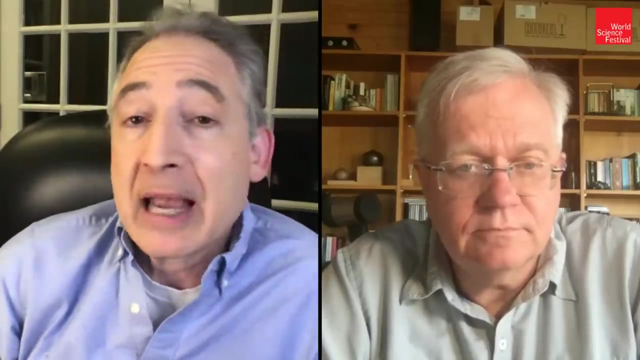 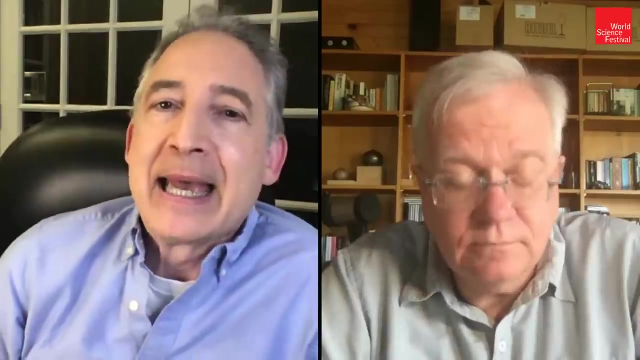 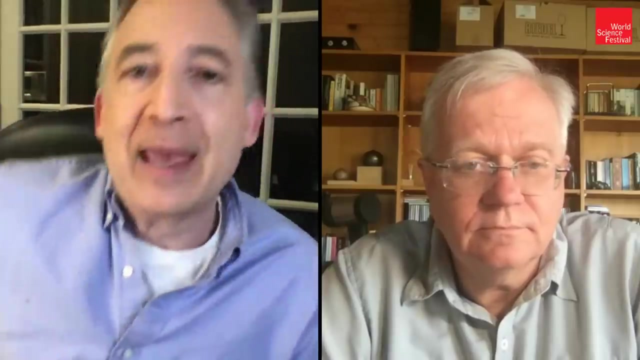 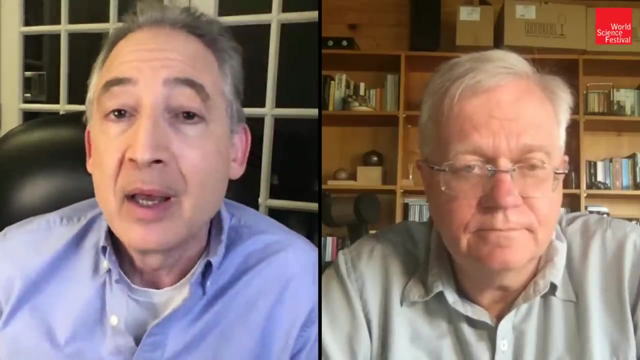 The vast majority of people come to their beliefs by virtue of the group that they belong to, And their identity is so bound up with that group that if the group believes X, you believe X because that is, And so you're absolutely right. We have to reach out to those groups, listen to the grievances, listen to the perspectives, and not slam it with a hammer of rational discourse, but rather reach out with a, with a warmth and an empathetic perspective, in order to bring everybody ultimately to a place that I think will be better for us all. 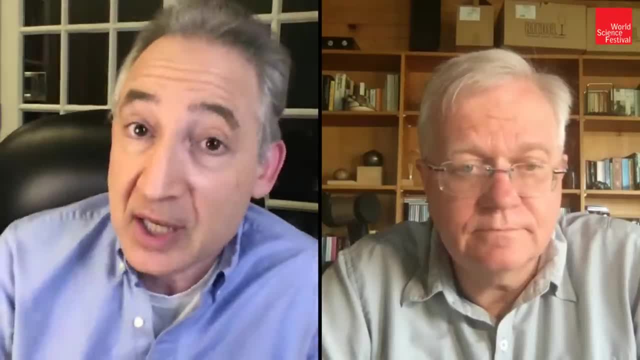 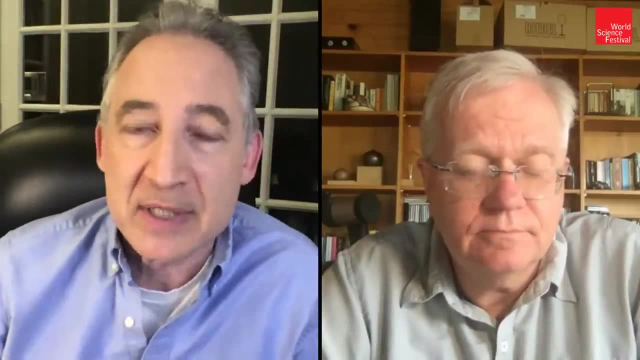 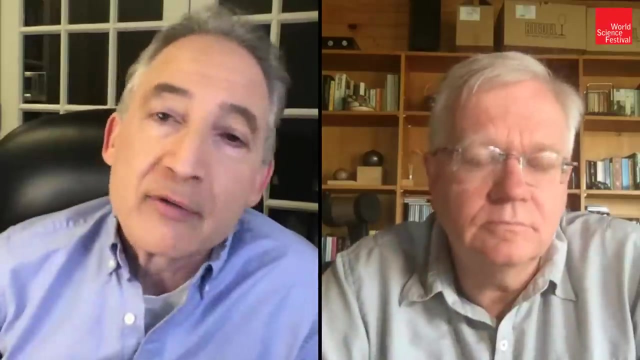 And look, I mean the World Science Festival with one of the wonderful things In World Science Festival of Brisbane, just to bring it home to. I mean, this event is part of that celebration of science. World Science Festival of Brisbane goes out to communities that are not directly in the heart of major cities. 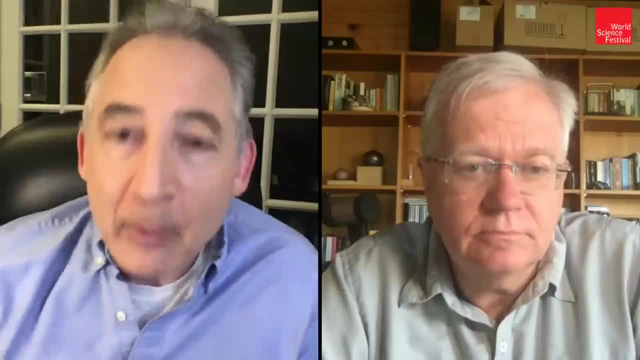 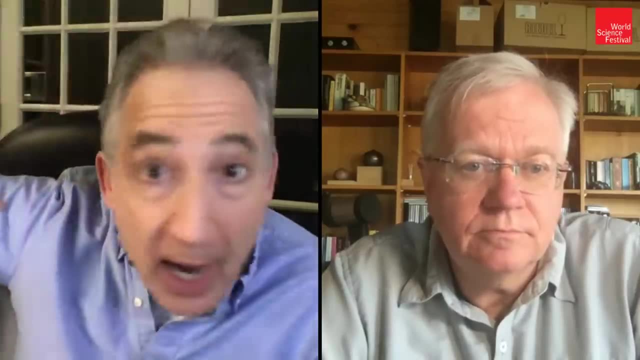 And so we view that as a wonderful model, And our intention in the United States is to do the same thing, to begin to see these World Science Festival events in a variety of cities and countries, World Science Festival of Brisbane, just to bring it home to, I mean, the world. 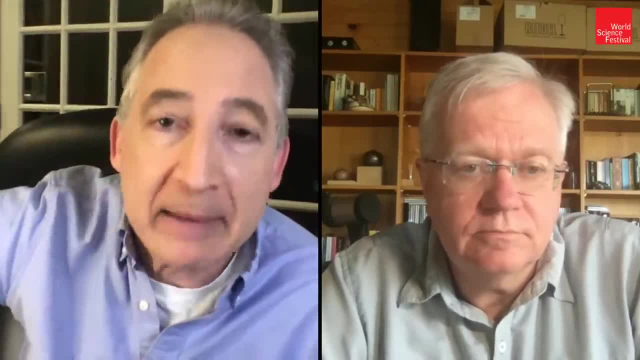 And look, I mean the World Science Festival of Brisbane, just to bring it home to, I mean the world. And we need to have a way to reach out to people who are not necessarily in extra city environments, where you don't necessarily have great population centers, but that is where you're going to reach people where they're at. 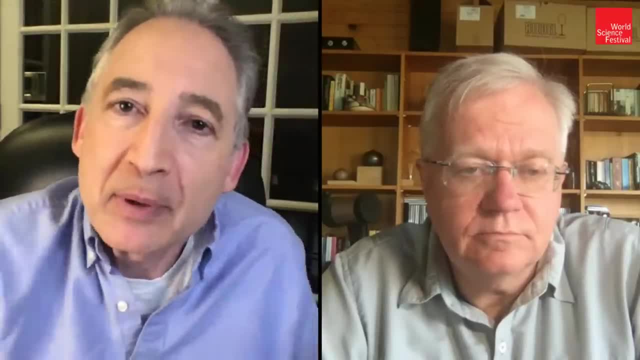 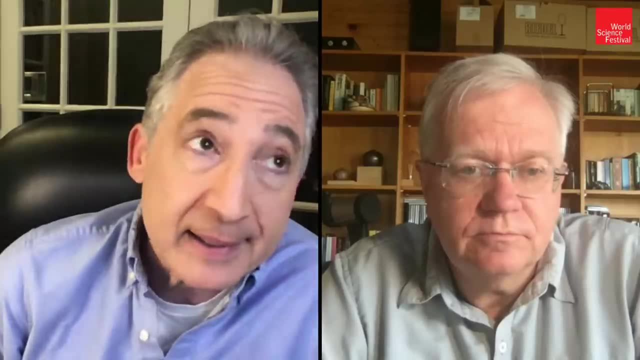 And so I think you're absolutely right. And so I think you're absolutely right. That kind of reaching out is the vital thing that needs to be done. And astronomy and physics is great because it's not- it's not political. And astronomy and physics is great because it's not- it's not political. 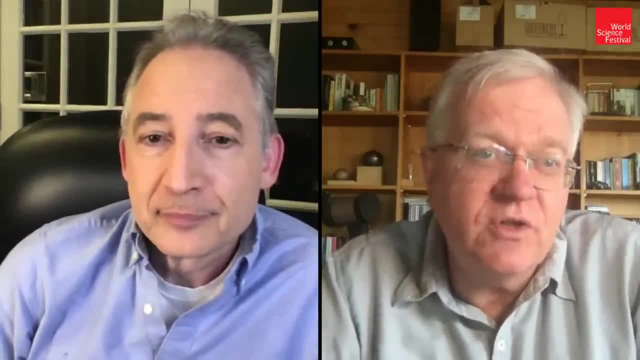 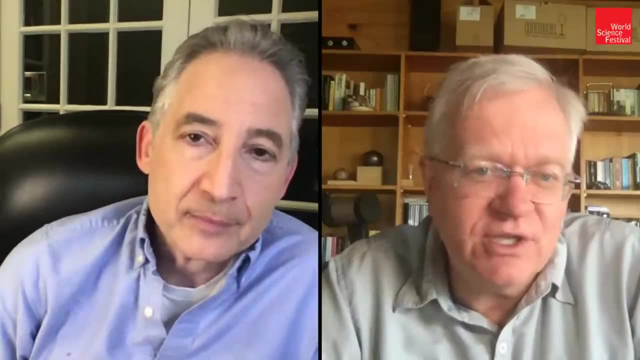 There is no, It is. It is just the wonder that the world shares. world shares. And you know, when I go to Namibia and I talk to kids there and look at the sky and tell the story, it's just like going to Cunabara brand, where the observatory is. here. It is a. 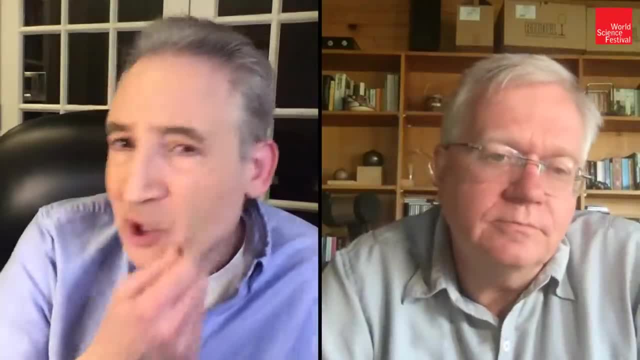 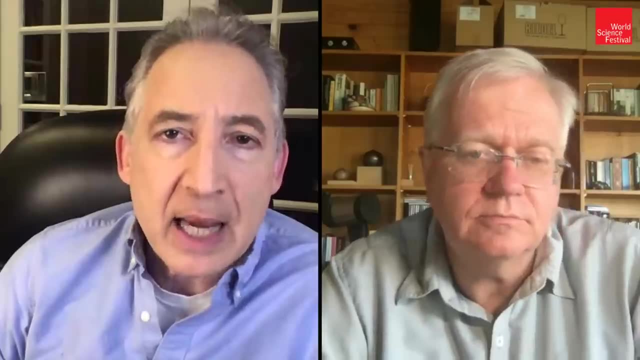 real universal language? Yeah, no, absolutely. And so, looking to the future, both from the political standpoint and from the scientific standpoint, where, do you think, the great excitement? what are we going to be talking about in this kind of event 50 years from now? 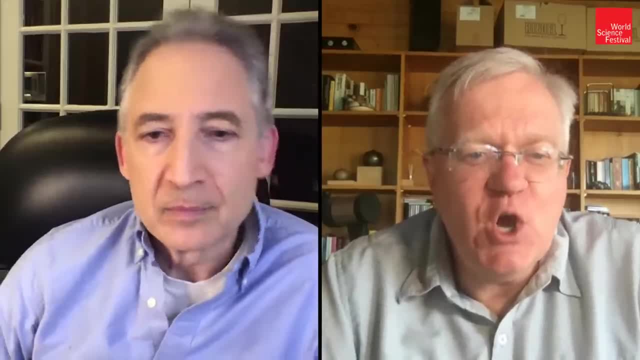 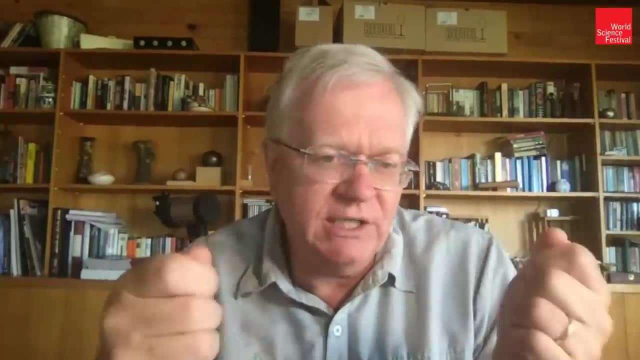 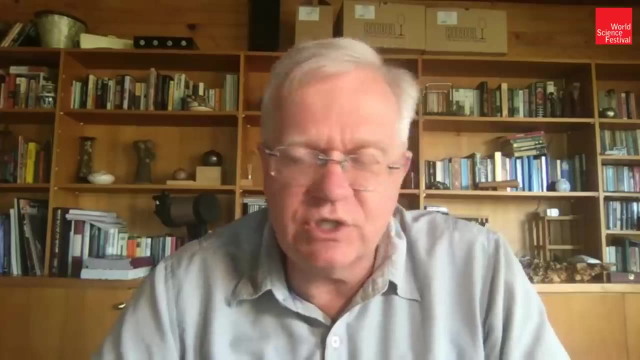 Boy, it's so hard to know. you know, because the way I think people think of science being quite linear, and it often is. but when it's linear it's not very interesting. It's when you get the big, sudden revolution. So you were talking earlier about this little crack in the door. 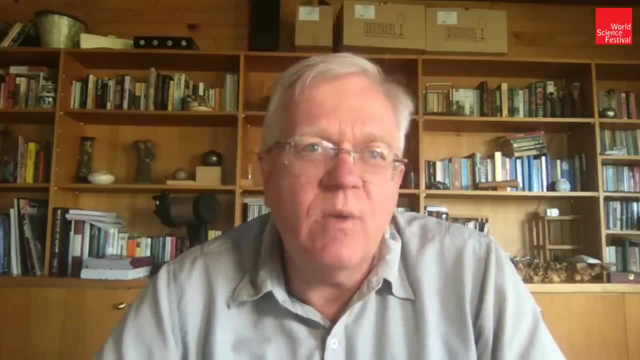 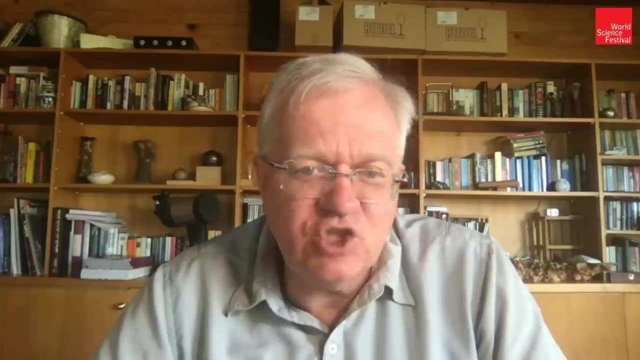 that is emerging potentially at CERN around the standard model because, as you're aware, right now the standard model is a little bit more advanced than the standard model. standard model is, uh, it's in trouble because it's just been so good at predicting things and there's. 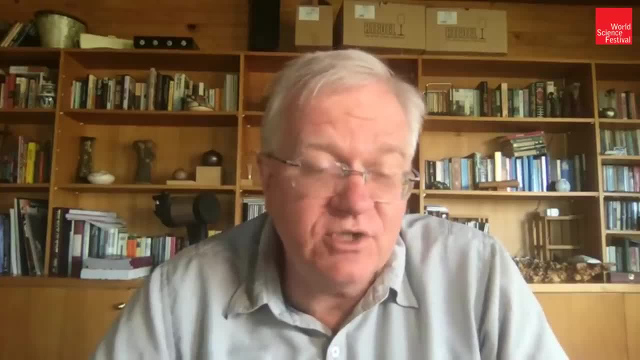 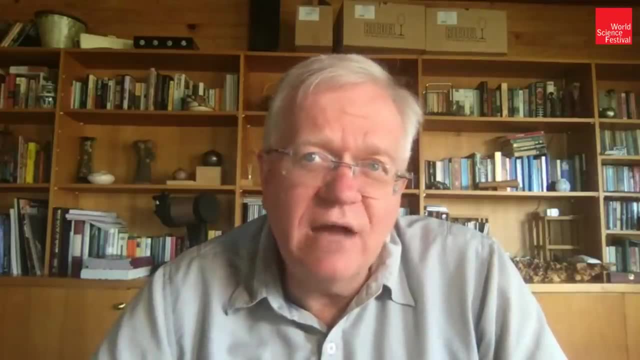 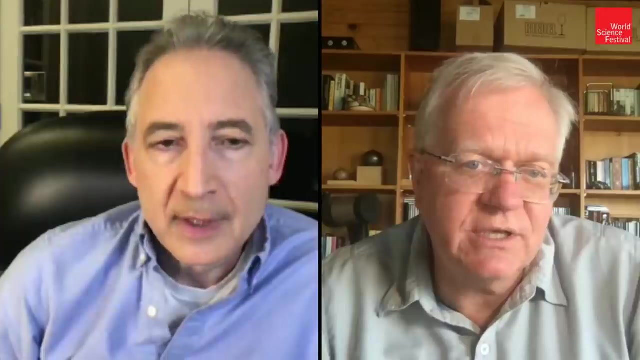 just nothing else to do, although it'd be nice to understand the mass of the neutrino and what dark matter is, uh, among other things. but, um, the, the reality is, uh, you know, that might be a little crack in the door that suddenly opens up a new world in particle physics, and and how can i know? 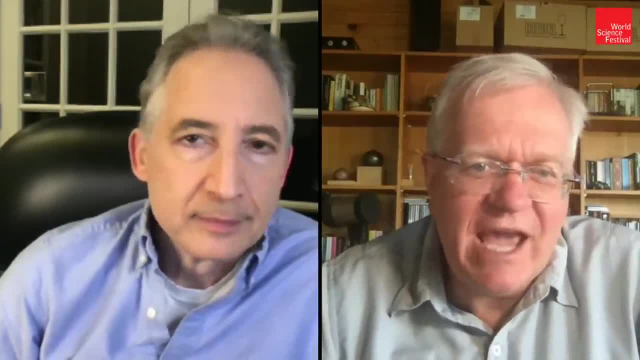 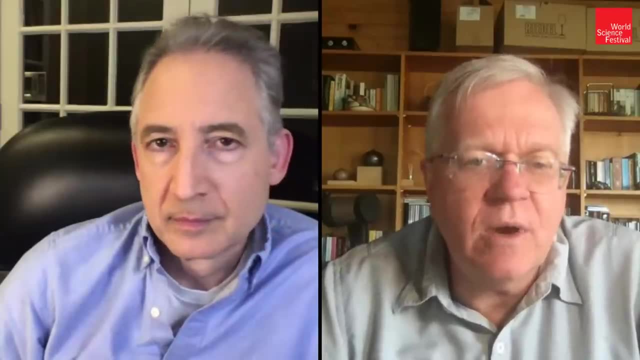 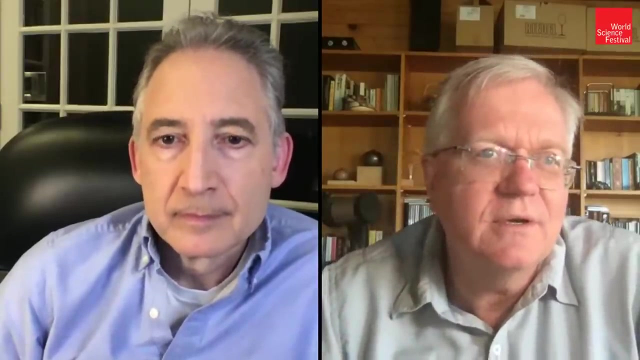 that. but if that door turns out to be a dead end and we can't figure out, you know why neutrinos have mass, what dark matter is? so let's just say dark matter only interacts via gravity, it is. it's a new type of particle that does not interact by the other three forces. what kind of screw i just 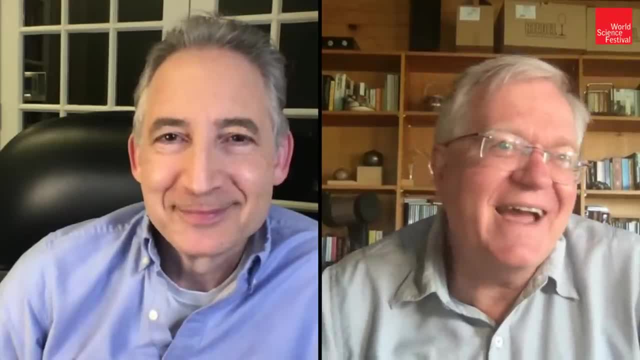 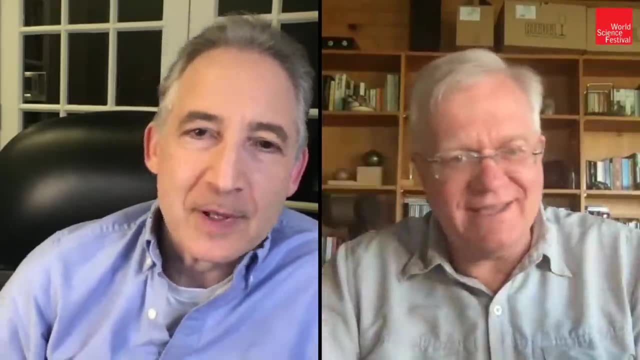 don't know how we're going to make progress on that, uh, and unless someone like you can come up with well, actually, it naturally emerges from this flavor of string theory and etc. um, but what i do know, so the things that i feel confident that we're going to have linear 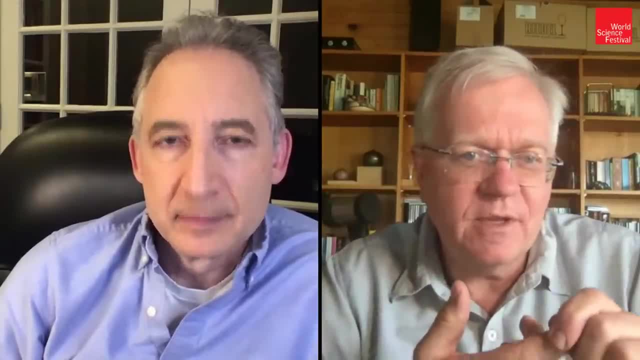 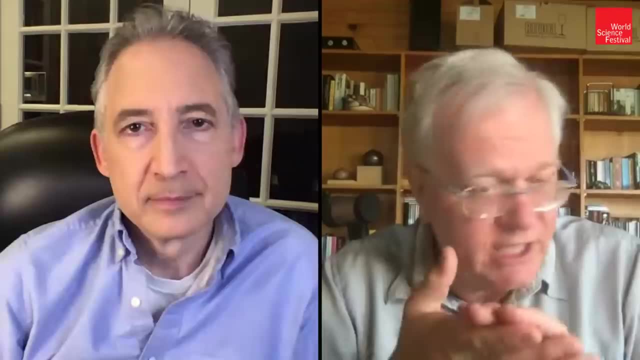 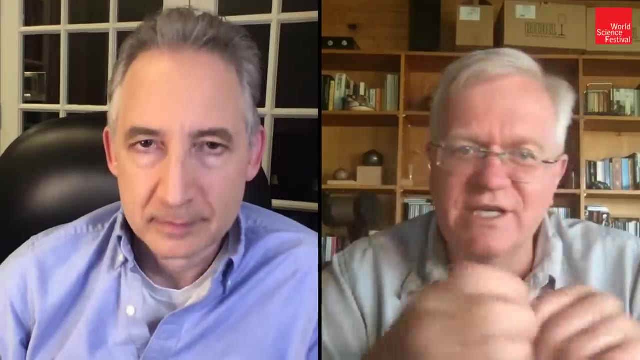 progression on uh planets it is. there's just a clear path for the next 50 years to go through and start finding habitable planets, looking at their atmospheres and potentially even as we get bigger and bigger telescopes looking at, you know, the rotation revealing continents. 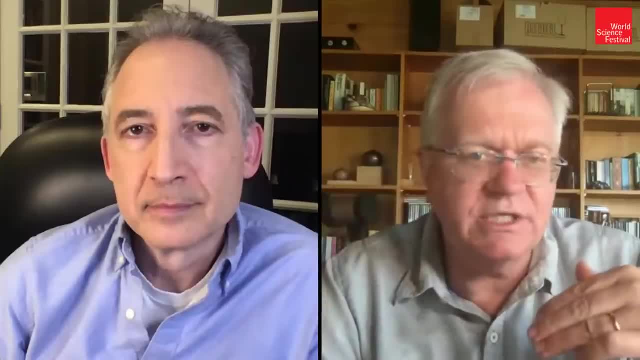 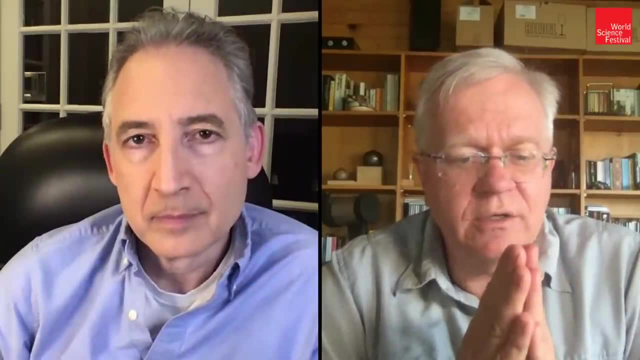 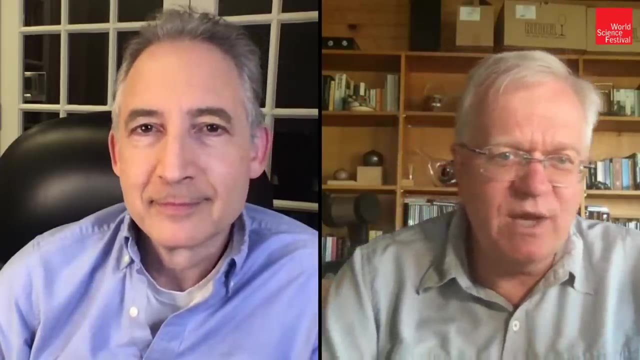 oceans, things like that, that that is almost guaranteed to happen and that is going to be exciting. yeah, uh, we have the ability. you know, right now, if you look at our, our, our map of the universe, we've got the ultrasound photos, the cosmic microwave background and we have the teenage. 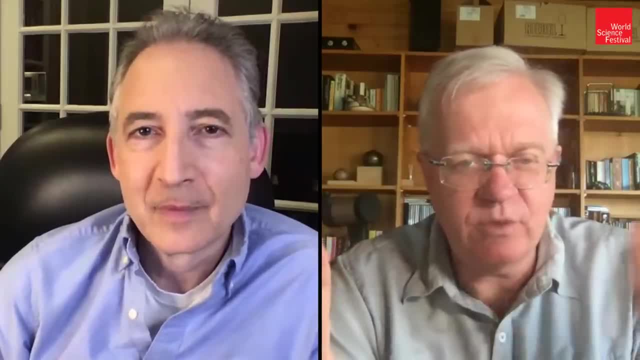 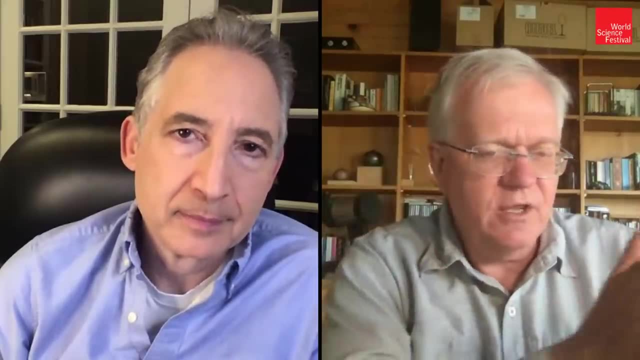 years, which are how far back we can look, and with the james webb space telescope, square kilometer ray and things like that, we're going to be able to get the baby photos. so we're going to be able to piece together the life story of the universe pretty much from beginning to end, and that's going. 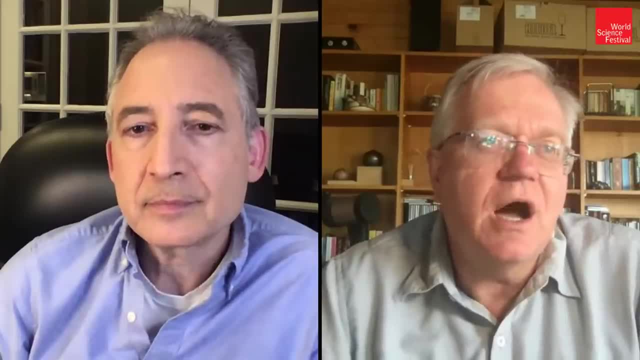 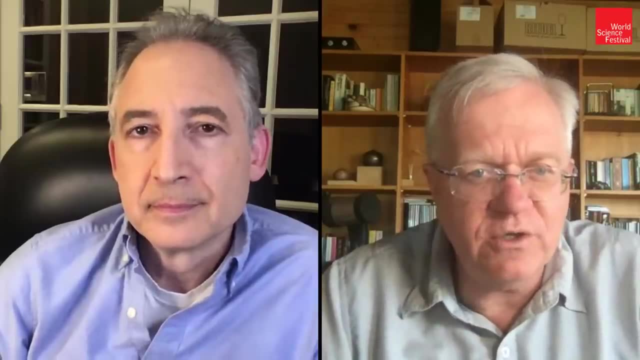 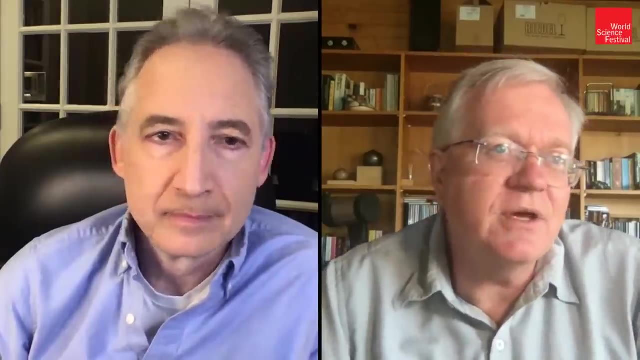 to happen over the next 30 years as well. so those are two things i'm really sure of. we have the whole notion of gravitational wave astronomy, which is four years old. um, there may be a whole level of richness in there. uh, you were showing the, uh, the. 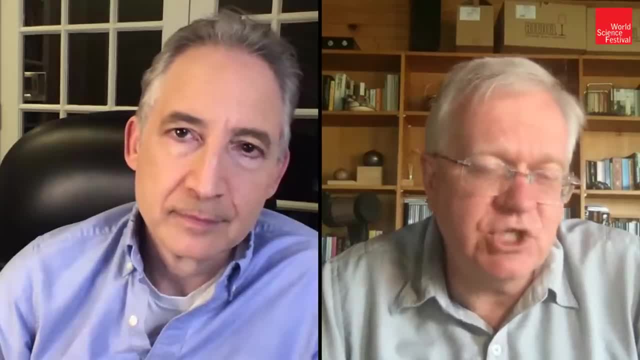 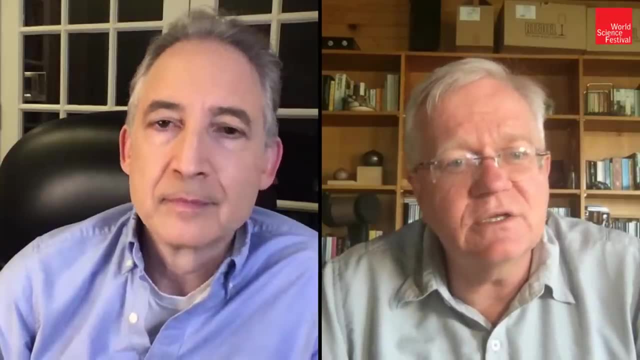 uh, the amazing images with polarization coming out of the m87, things at the beginning, and you know that there's just a whole new world there and you should say: you start being able to do dynamic movies and you start doing dynamic movies. and you start doing dynamic movies and you start. 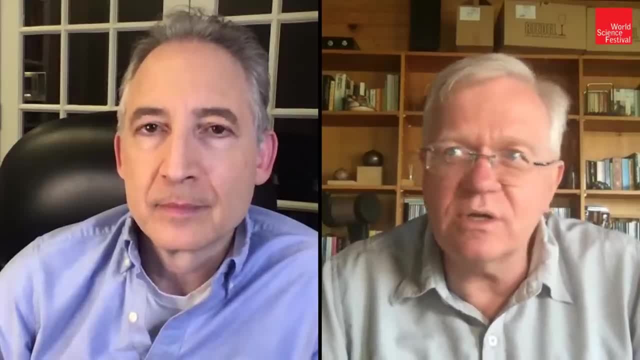 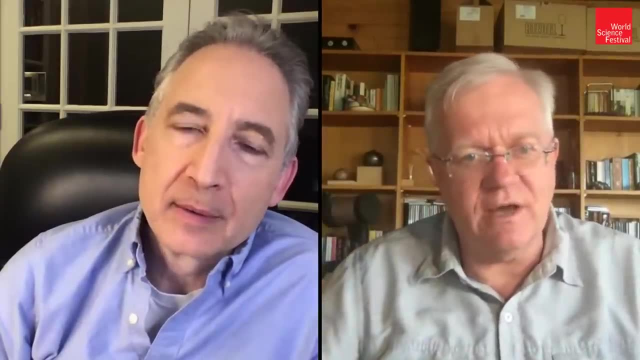 being able to see how a black hole works. those are things 50 years from now. who knows the next level? we're going to be up, maybe we're going to. instead of having that whole earth telescope, we're going to have an array on the moon and here and you're going to be able to really get. 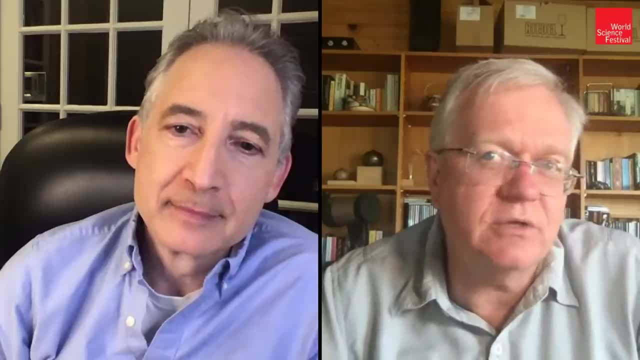 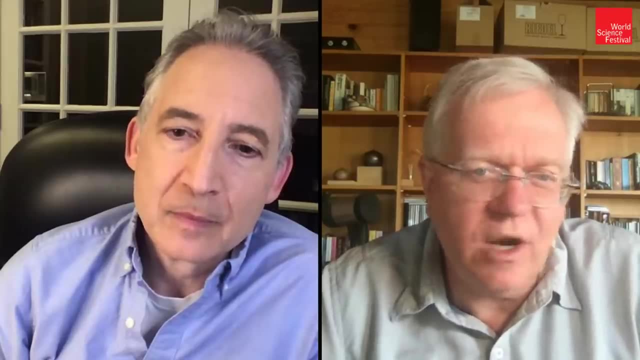 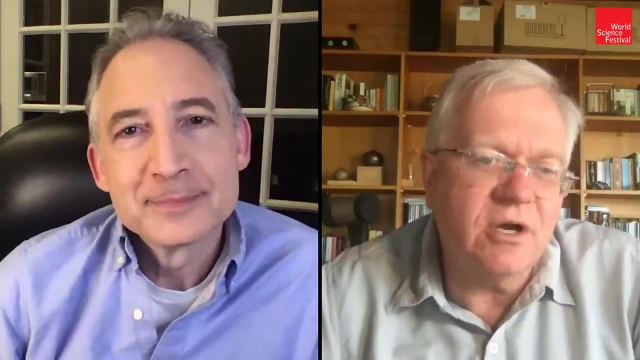 uh, look at the horizon incredibly accurately. so i i, but what i think we'll be talking about is something you and i can't contemplate now. which is the most exciting thing. yeah, i mean we'll probably between you and me. we're still going to be talking about dark energy and have no idea what it is. 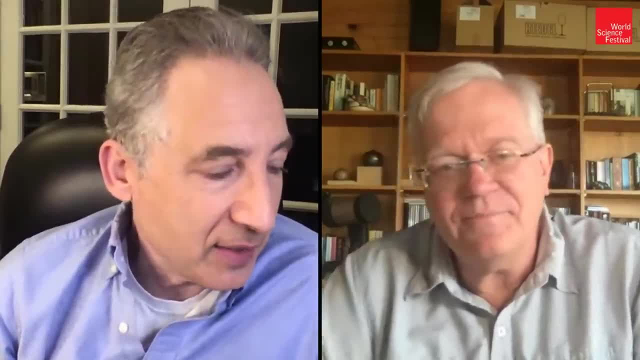 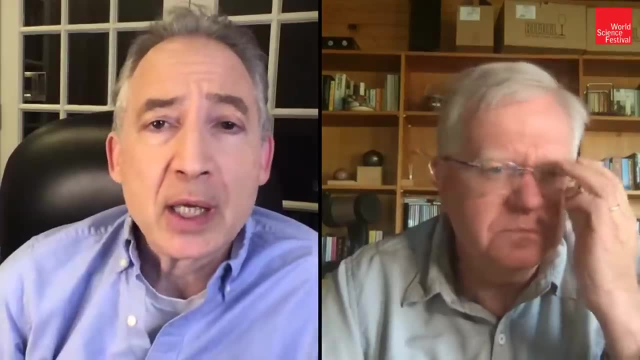 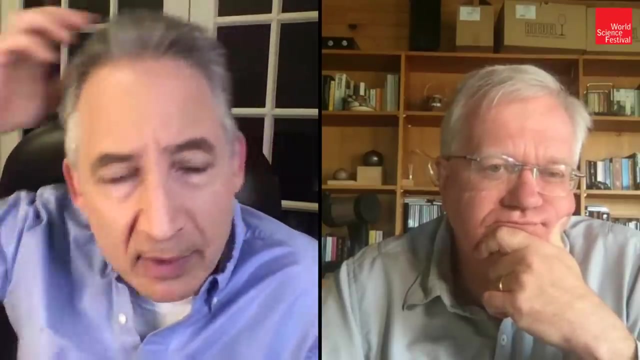 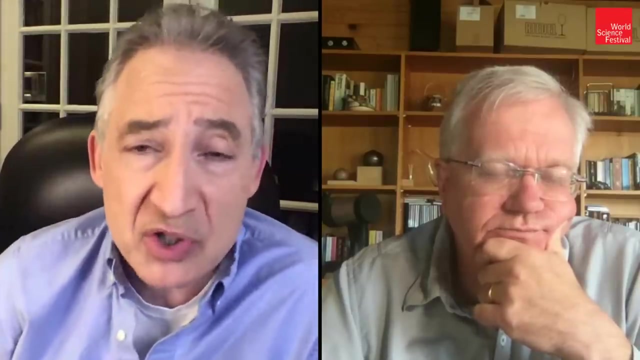 that's what i think. well, along those lines i got a question there. you know, every so often there's a paper, sometimes by serious people, questioning your result, right, questioning whether the you know, accelerated expansion is real, whether the dark energy evidence is real. do you take those papers at all seriously? do you look at them? do you concern yourself with them? 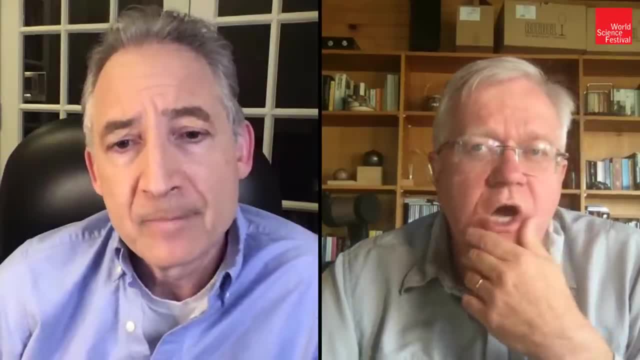 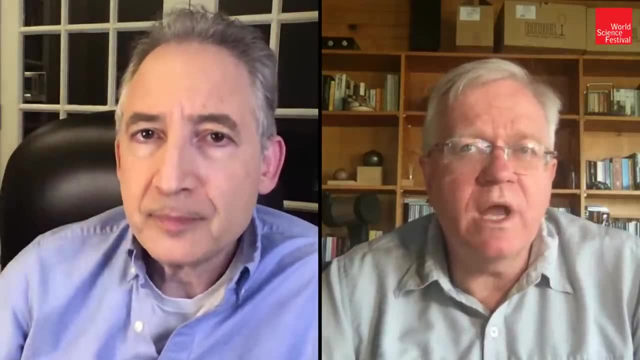 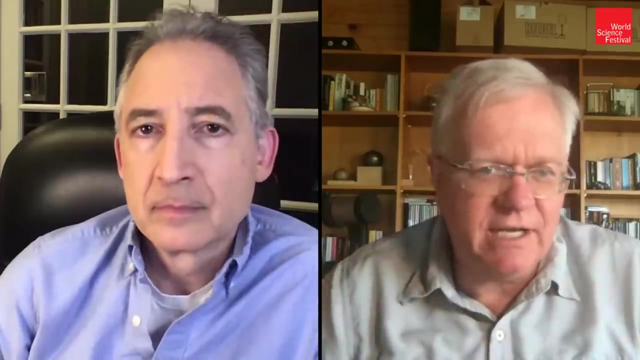 or or how. what's your response to those papers? so i take them seriously, uh, as they deserve to be taken. if i can be honest, um, when i see someone just taking weird, i've decided to run my new bayesian tree blah, blah, blah on your data and i find that it's only four sigma rather than seven. 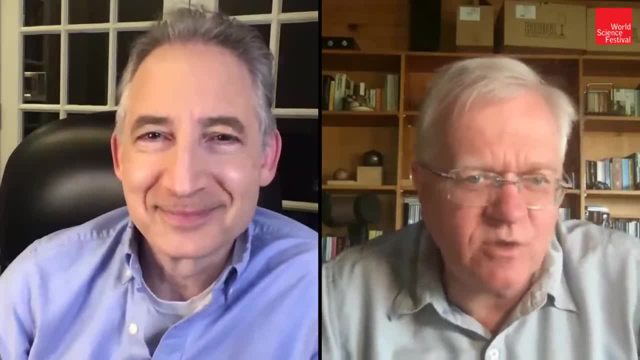 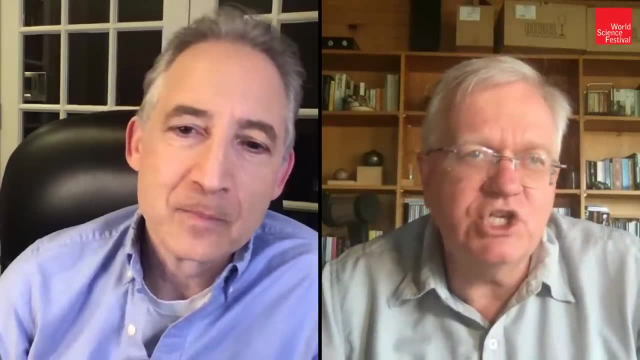 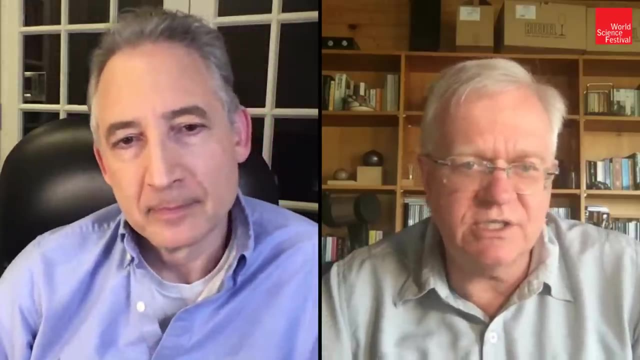 sigma, i'm not interested. i'm sorry. that's, that's fine. go talk to. that's a status statistician thing. i'm going to do something. i understand better. dark energy and acceleration is way bigger than supernovae. right, it has things we call baryon acoustic oscillation, so the bumps and wiggles from the cosmic microwave. 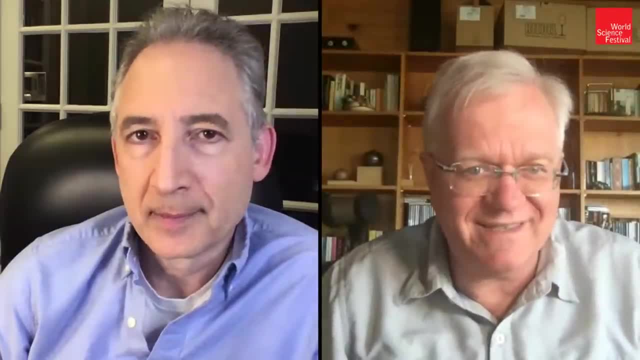 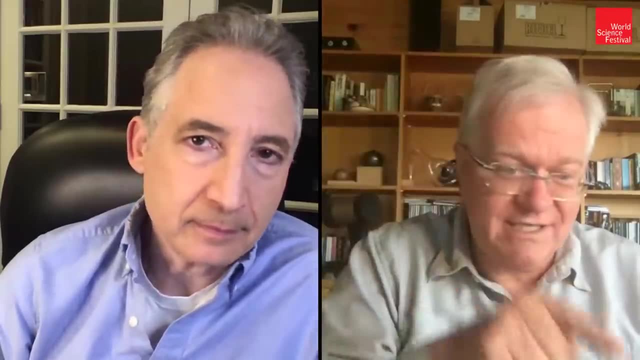 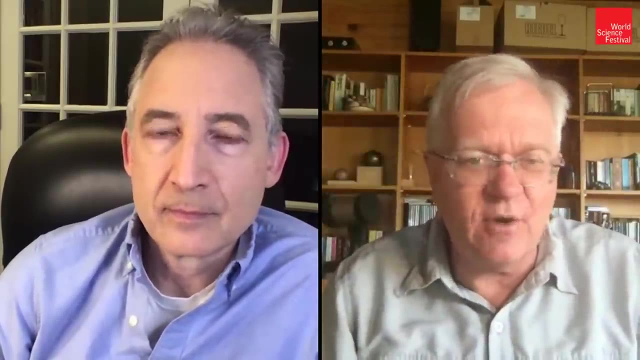 background. they, on their own, tell us because of how big they are now that acceleration is occurring. then you get to use those same bumps and wiggles in the galaxies over time and they give the same answer now, yes, there's a little disconnect between at the seven or eight percent between. 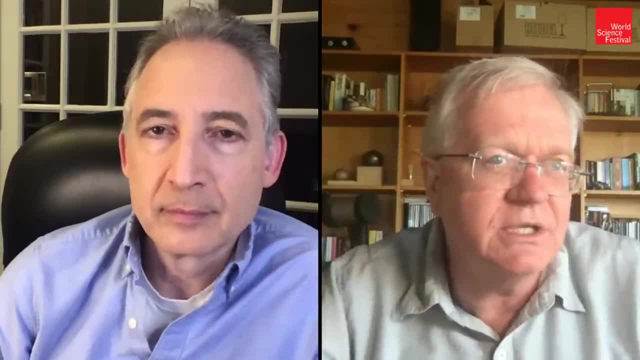 the upper and the lowerligion and the lowerlignum. but i think that's a brilliant question and we'll the distant and the nearby version of the Hubble constant, but you just can't. it's not gonna make it go away. So it's like people who want dark matter to go away. 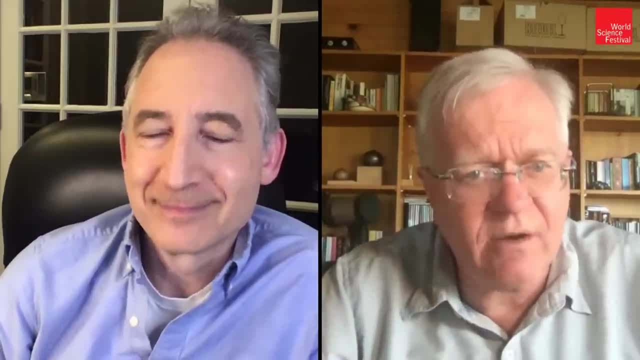 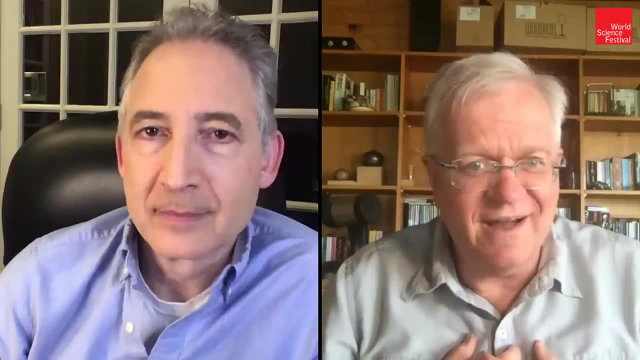 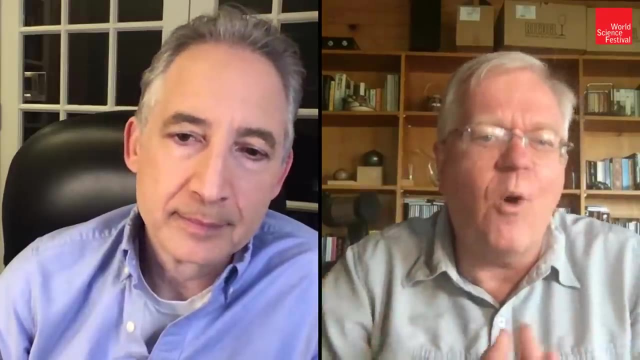 And the first thing they do is we will not cover the cosmic microwave background. The baryon acoustic oscillations, the cosmic microwave background are why I believe dark matter, not the rotations of galaxies, which I think add lots of evidence. But you can't avoid the whole of evidence. 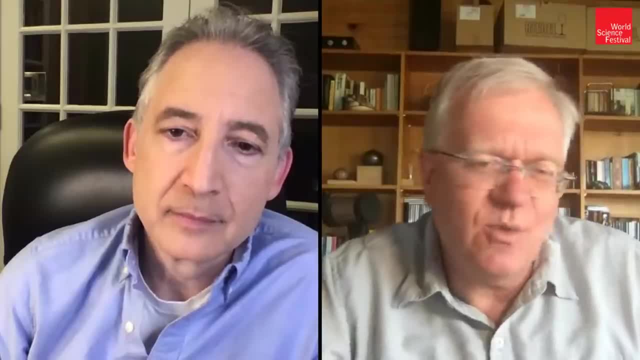 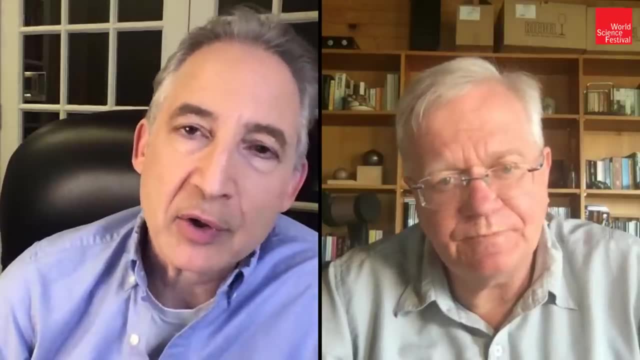 when you just cherry, pick little bits and try to pop holes in it. That's not the way science works. Yep, So there's a famous parameter that people use to characterize the dark energy, the so-called W-parameter equation of state parameter. For those that know, 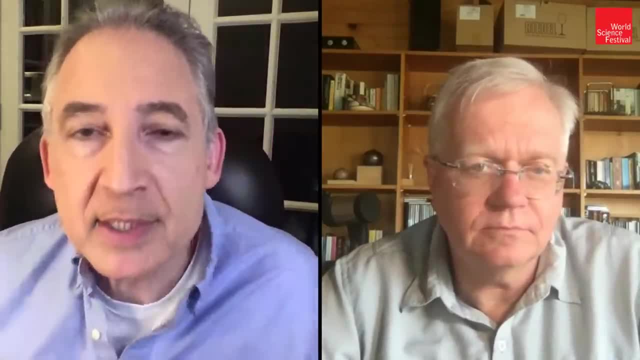 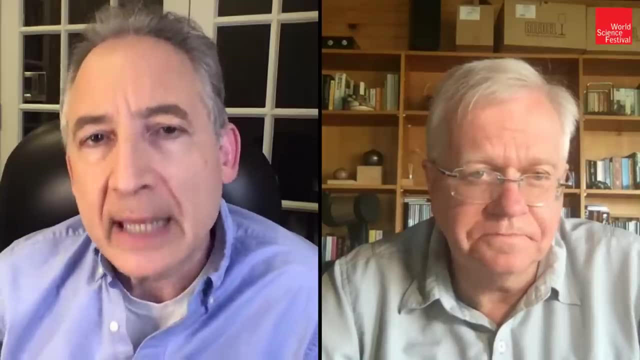 those of you who are listening who know about this. W equals minus one is the equation of state parameter for a true cosmological constant. Do you think that we will nail down a value of W that perhaps is different from minus one through subsequent observations? 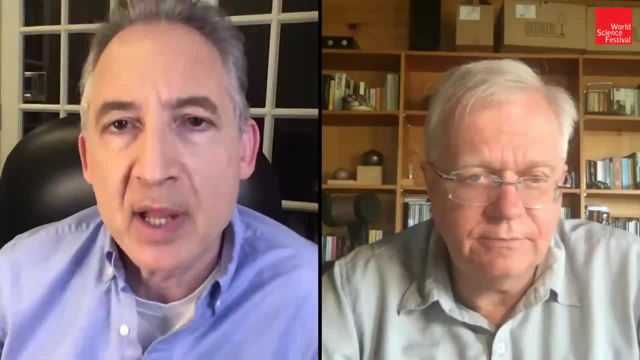 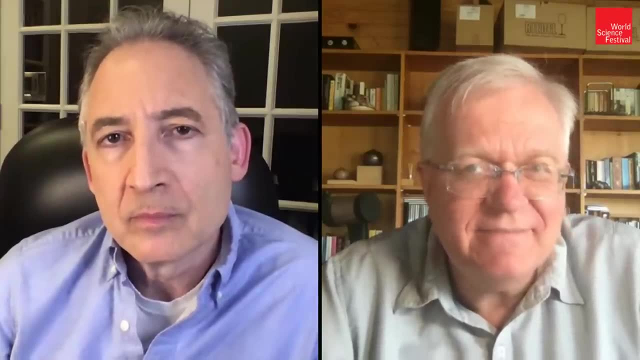 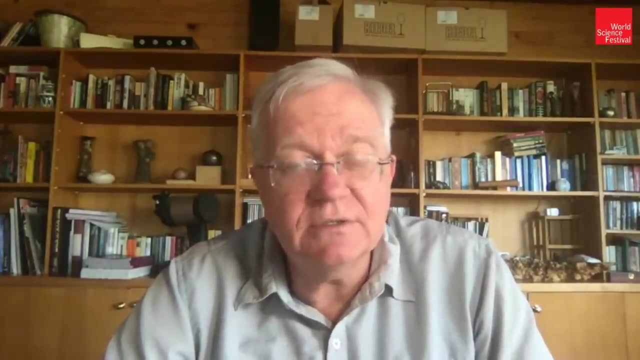 Are you confident that it's all gonna just be the vanilla version of the cosmological constant going forward? I'm certainly not confident, but if I had to bet I would be prepared to take 10 to one odds that it's gonna be just vanilla. 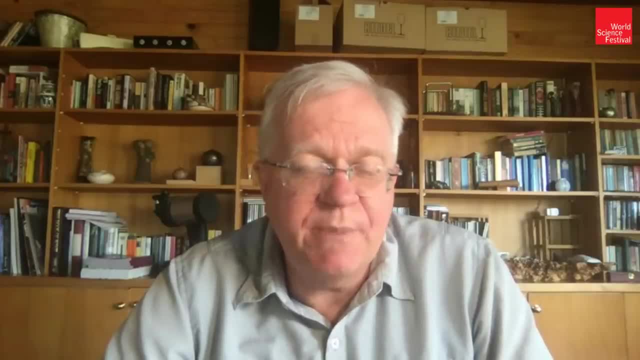 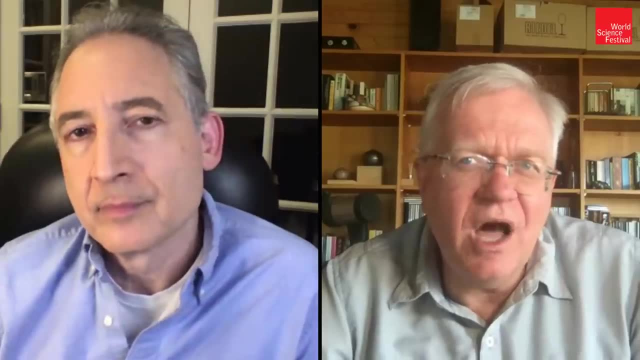 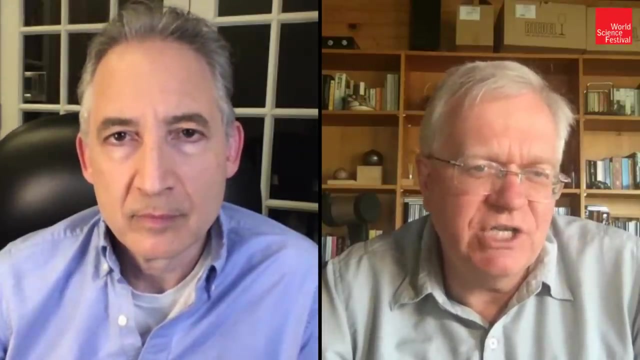 But you don't know until you do the experiment. The question is: how many are you prepared to spend on The experiment, especially when a lot of, if you would say. what is a natural value for W in a dark energy, sort of an inflation type? 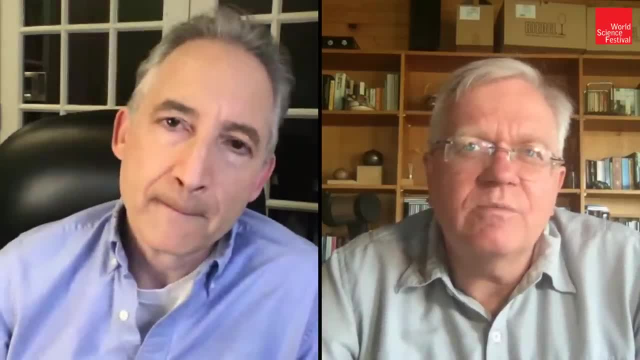 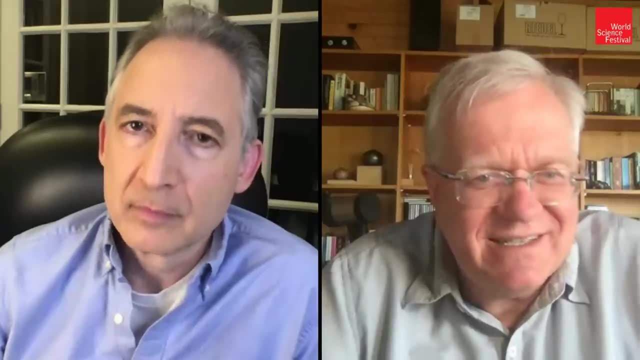 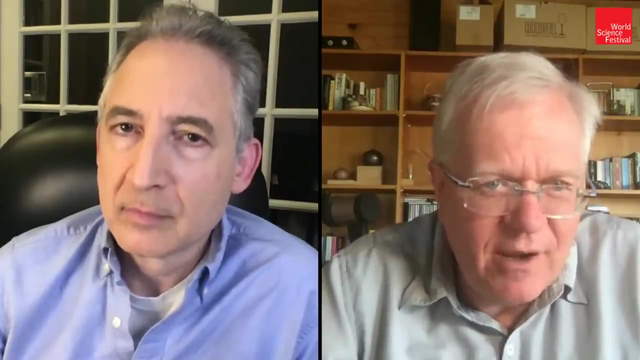 in some sort of particle based version of what's going on, you would expect four or five, nines or maybe six Minus 0.95 is not a natural number. It's not a natural number. It's not a natural number for most theories. 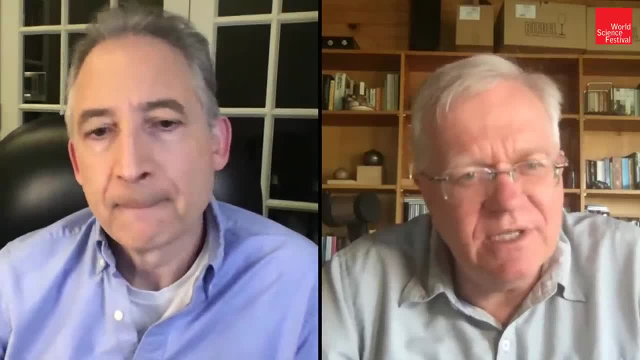 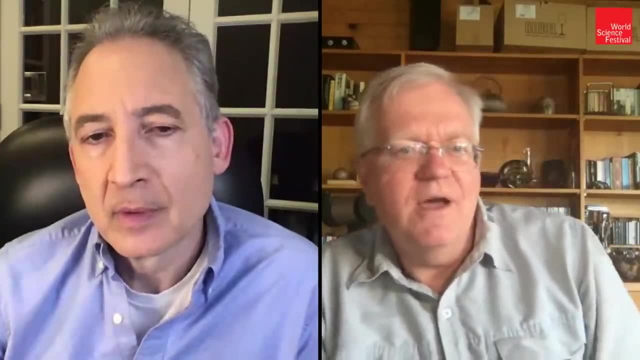 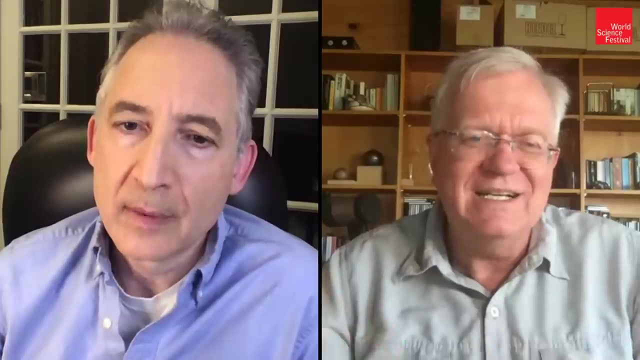 And so it's kind of hard to go out and spend billions upon billions of dollars when you literally don't have a theory that says the blah, blah blah predicts this number at the right bit. And we think that's really a beautifully aesthetically strong theory. 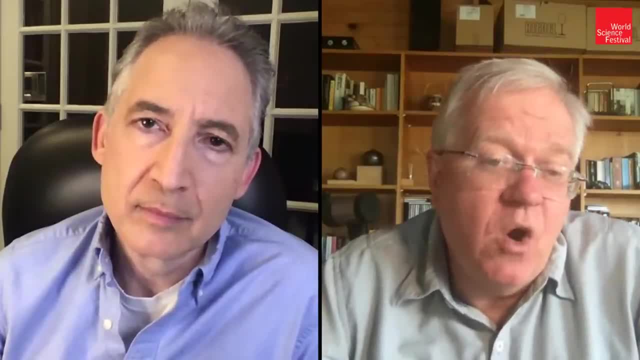 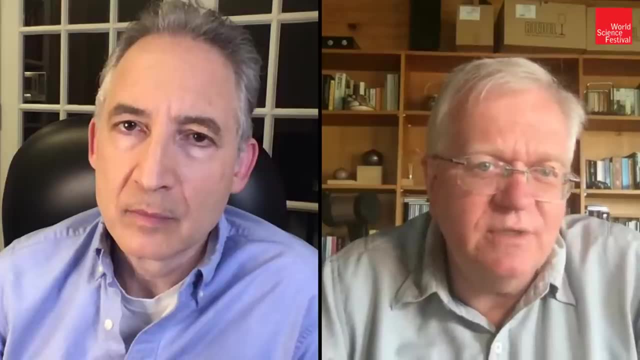 So I don't know. I mean, my guess is it probably is very close to minus one. It may be exactly minus one, but do I think it's going to be different enough from minus one for us to see it? My guess is unlikely. 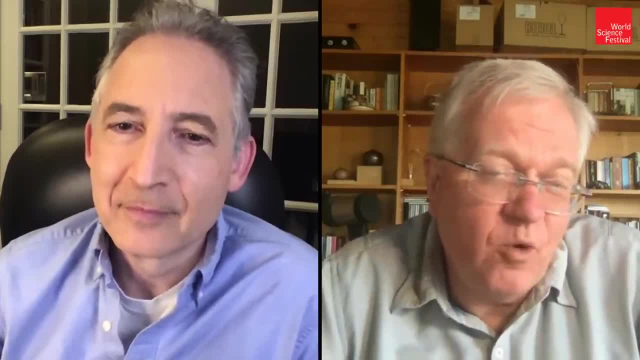 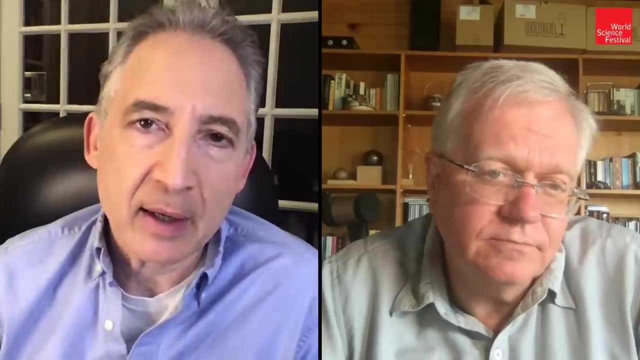 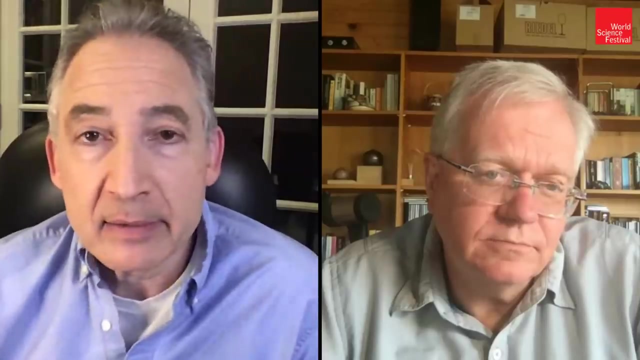 I think we're going to run out of money, quite frankly, before we can do it. So how do you view the mathematical description, say, of cosmology, as it currently stands? Do you view it as a clever encapsulation of the data? 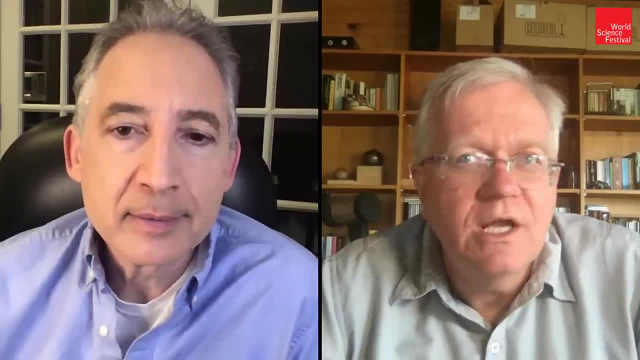 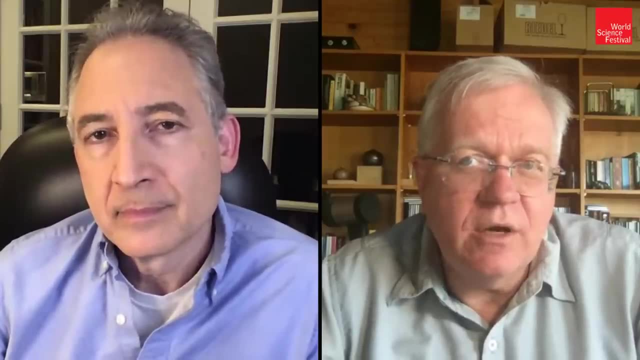 or do you view it as truth? Oh, definitely don't see it as truth. I see it as well. and the reason I. well, let me explain why I don't say it as truth. And this is a place where I've moved a lot. 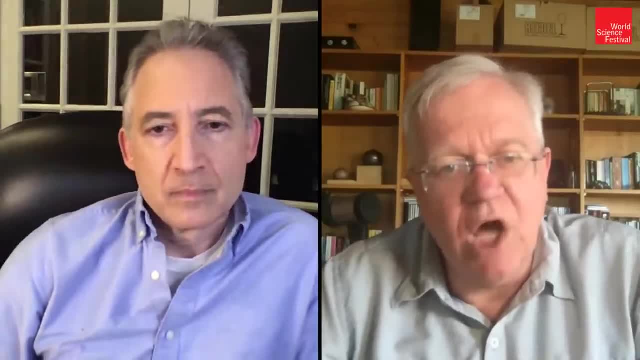 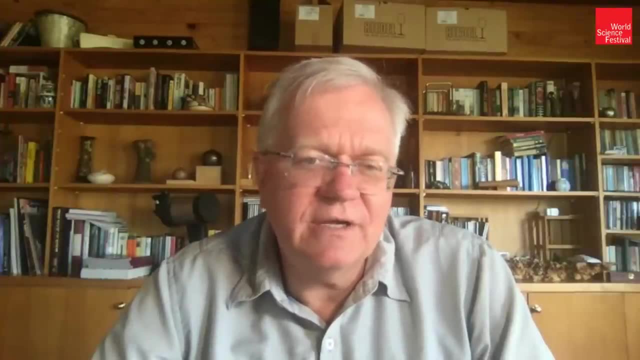 in the last 10 years. It is very clear that to me that gravity has to be connected to the other three forces in a quantum regime And I think it is quite likely that it's going to be connected to the other three forces in a quantum regime. 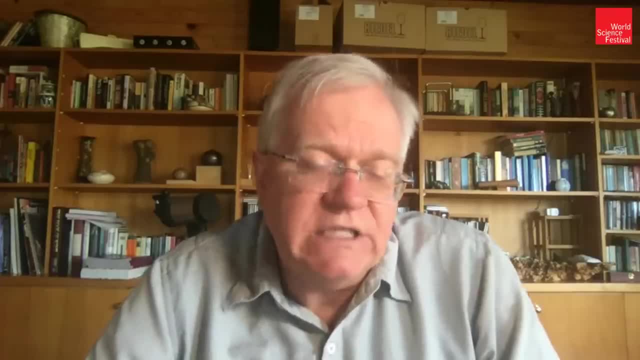 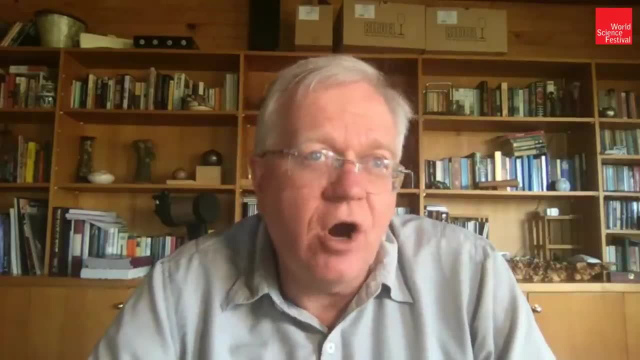 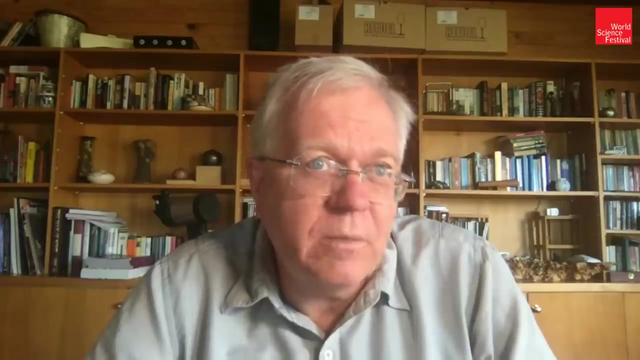 And I think it is quite likely that and that gravity, as we know it is some sort of emergent phenomenon. GR is an emergent phenomenon rather than the truth. Now, it's a very accurate truth and it's certainly good enough for me. 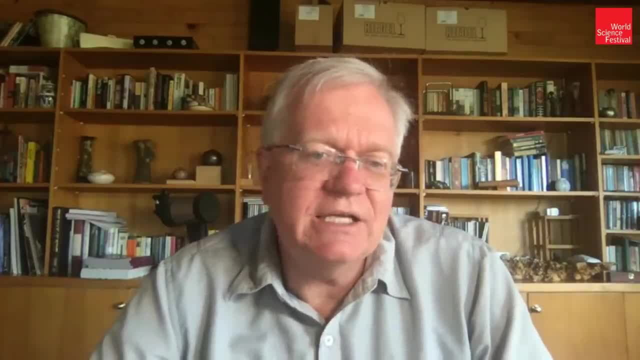 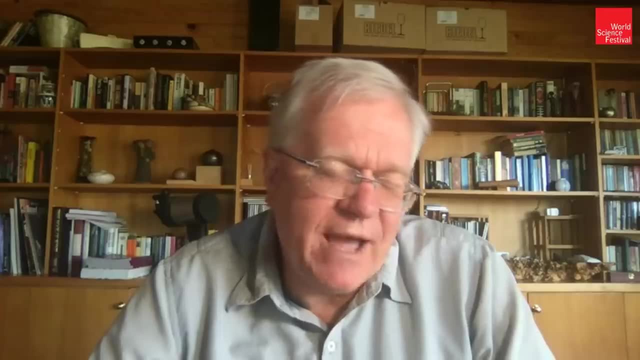 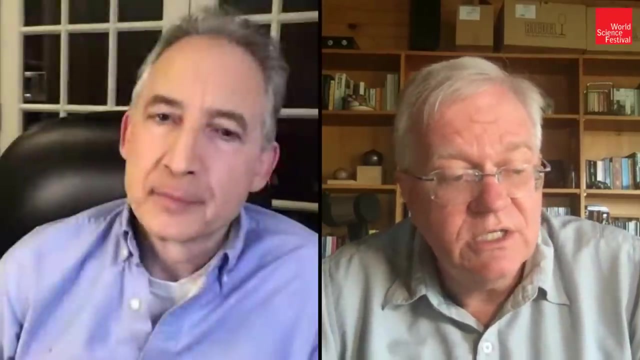 But my concern is that it is hiding a bigger theory that probably is, you know, back to when the universe was 10 to the minus 35,, 10 to the minus 35th of a second or something. So it is, I see it as being a really good approximation. 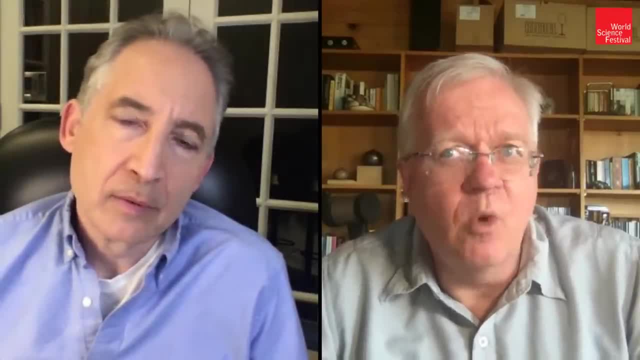 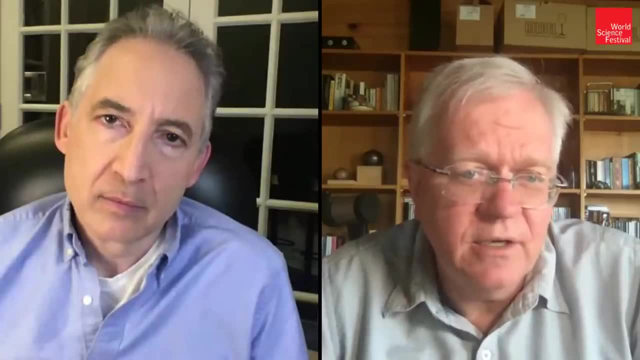 but my sense is that almost certainly it is not the defining truth And that's why, when people talk about the singularity of the Big Bang, I'm completely unconvinced there's a singularity, because I just don't think general relativity goes back to the singularity. 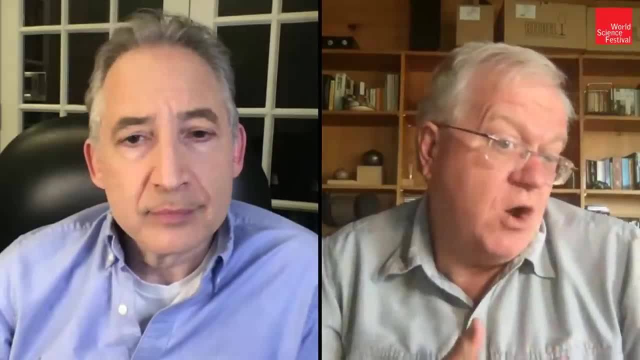 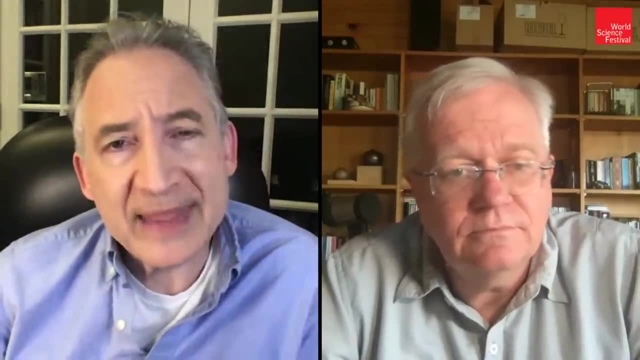 I think it breaks down at some point Now. do I know that? Don't know, But you know that would make sense to me. Yeah, You know that's my perspective too, as I think you know. But what that leads me to also wonder about is the following: 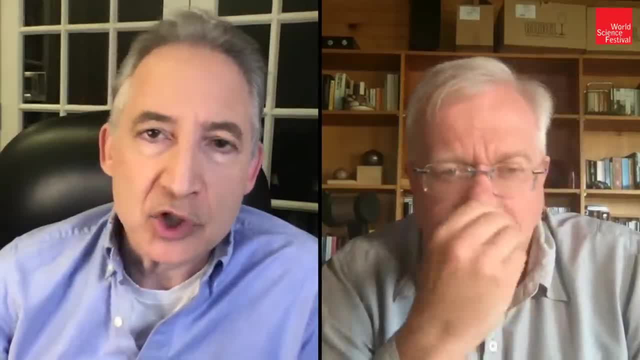 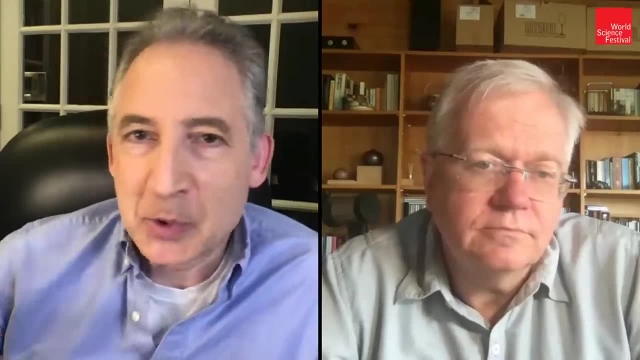 When we use naturalness arguments in judging, say, W the equation of state for dark energy and say, look, minus 1, very natural, but you know, minus 0.95,, minus 1.05, kind of unnatural. it always makes me wonder. 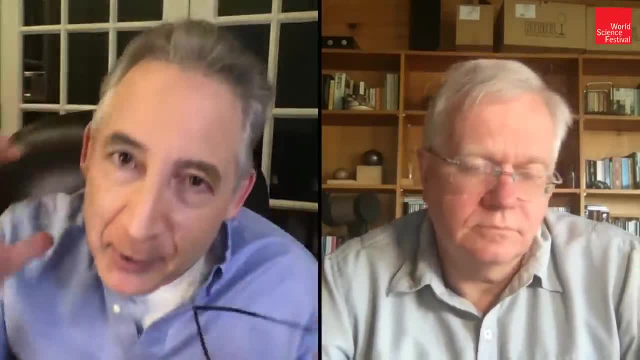 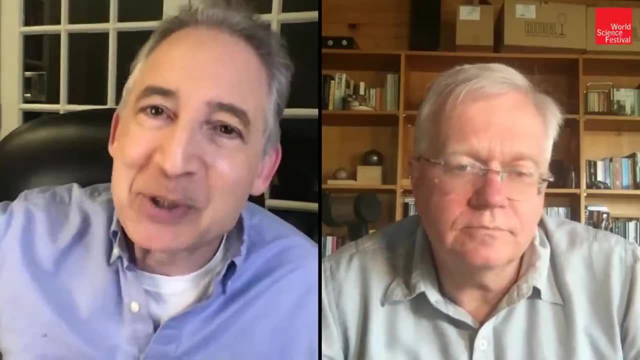 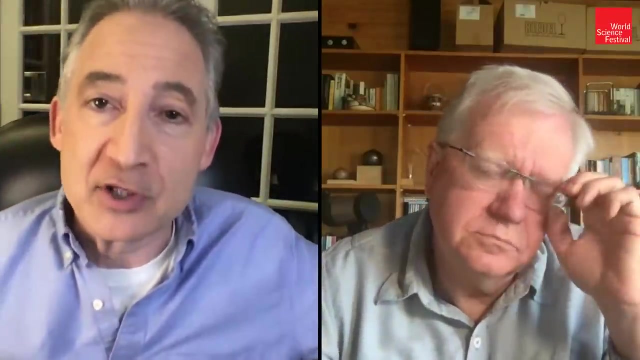 yeah, it's unnatural in that particular mathematical description, but perhaps, as you say, that's not the truth. Maybe there is another mathematical description in which the unnatural number, say 0.95, is totally natural in that other description that we just haven't found yet. 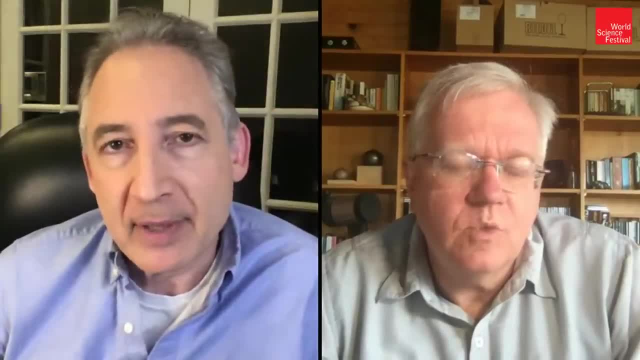 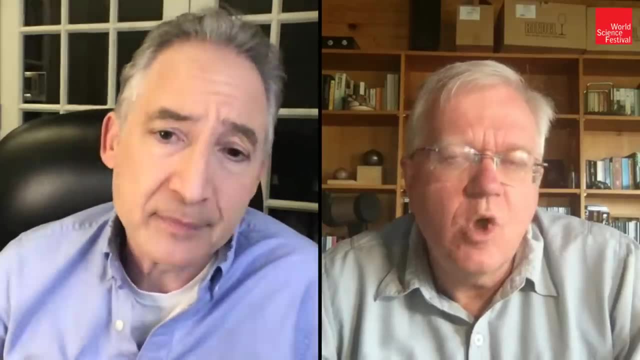 So I'm always skeptical. I mean, I use these arguments too, naturalness arguments, but I always, in the back of my mind, wonder if we're just fooling ourselves. Well, the answer is: when you don't know what's going on. 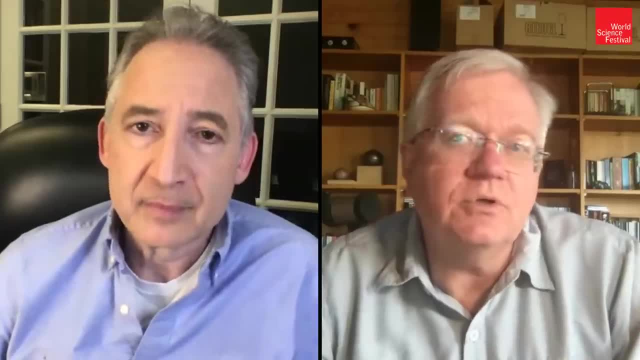 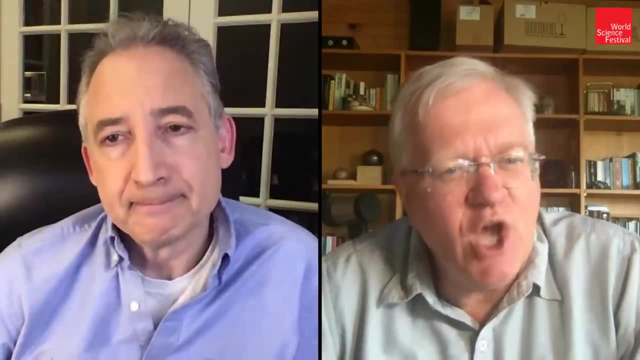 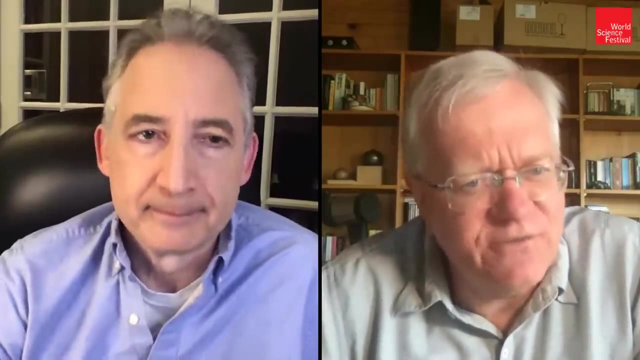 it's easy to fool yourself. But let's take, for example, curvature of the universe. So we know the universe is very close to being flat And we know that that is by. you know. I was always told that's kind of the natural place for it to be very 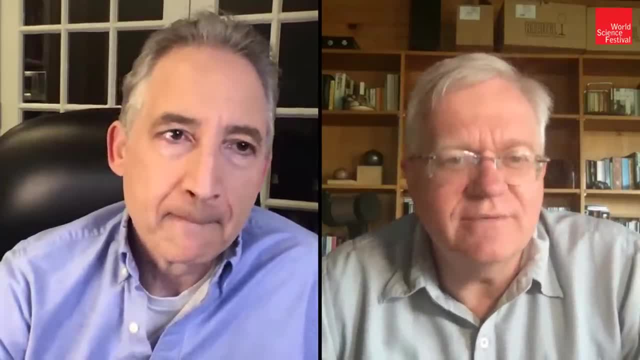 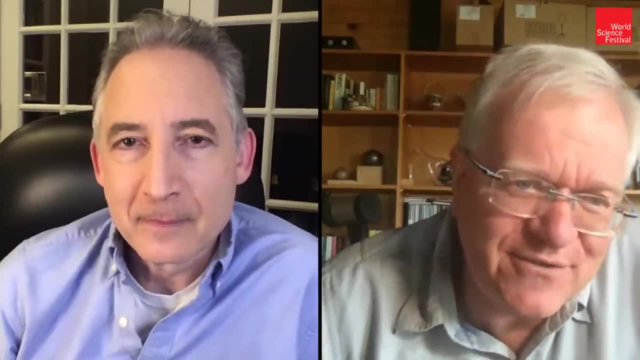 very close to flat. Well, guess what The universe was, despite me going? come on, you guys don't know what you're talking about. it turns out it was very, very close to flat And it is the natural place. 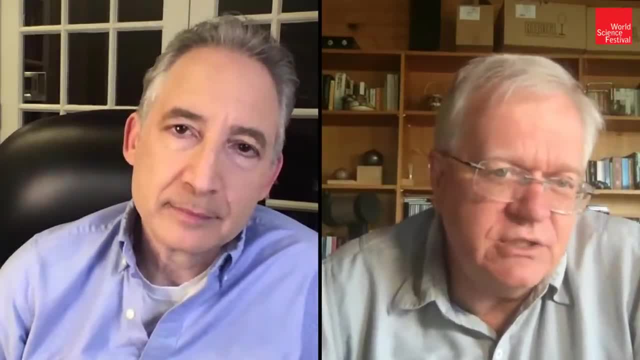 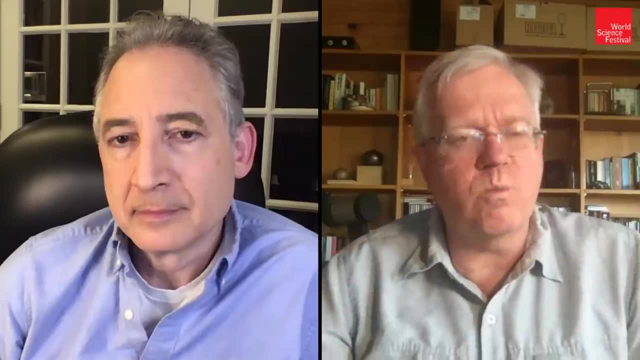 And it's why we think things like inflation have occurred, because it's the natural place for it to land. So I think there is clearly going to be a whole range of theories where you might expect W to be minus one, But you're right. 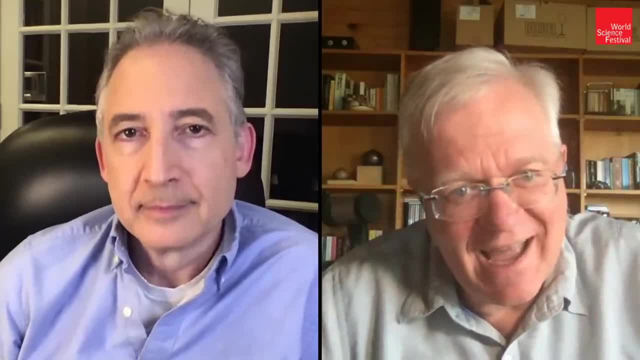 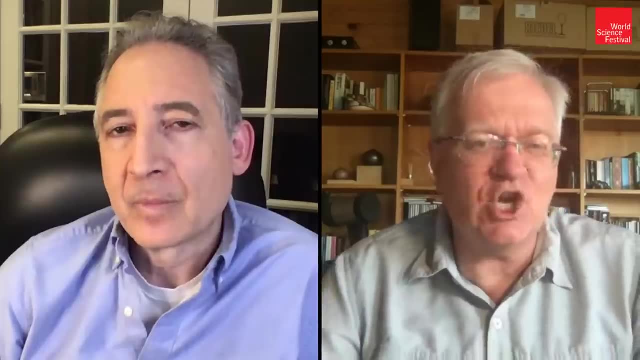 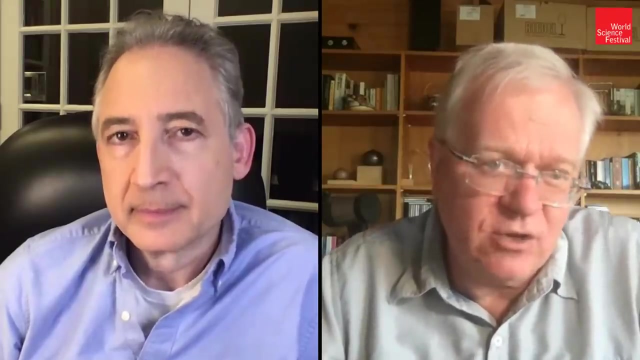 The real theory might be something else, And that's why it would be really, really nice to understand, have a theory that naturally says dark energy should be there at roughly the level that it is, Because naturalness, the reality, is the number we have measured. 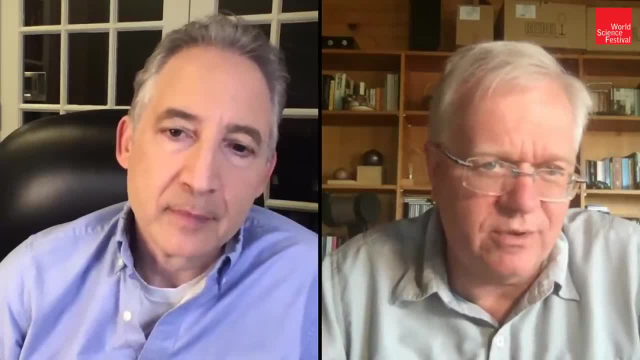 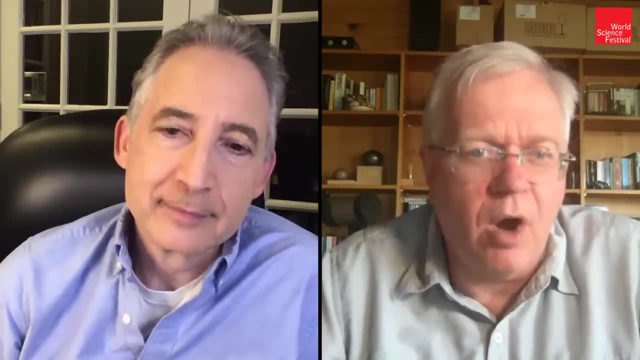 is not a natural number. It is a terrible, weird number. that is one of the reasons it's so hard is why on earth would it be not zero and a number so small, but big enough for us to measure? It's kind of crazy. 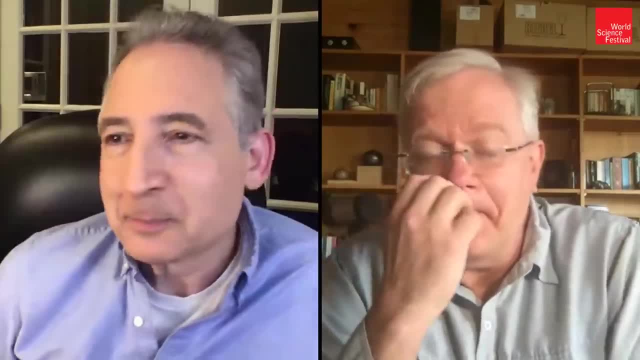 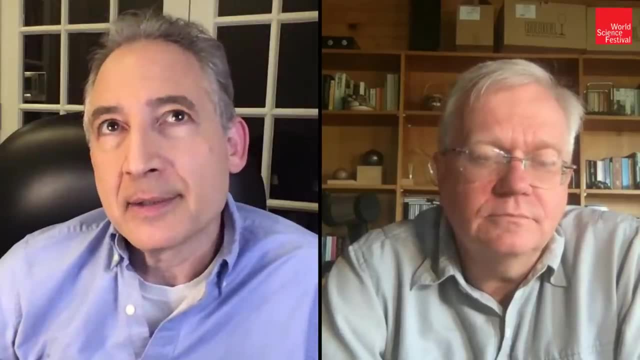 Yeah, All right, Let's assume that it is that And let's assume that it doesn't change. And then let's just for a moment think about the far future. Does it thrill you, distress you, to imagine that in some hundred billion? 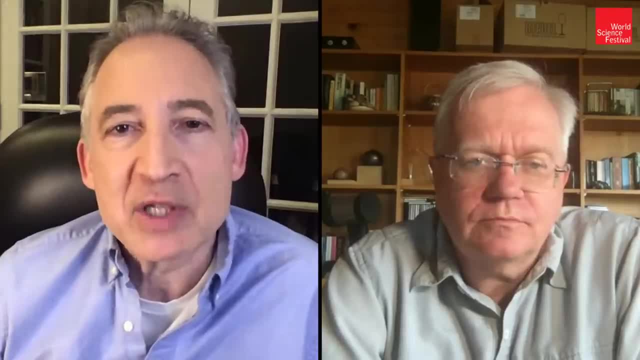 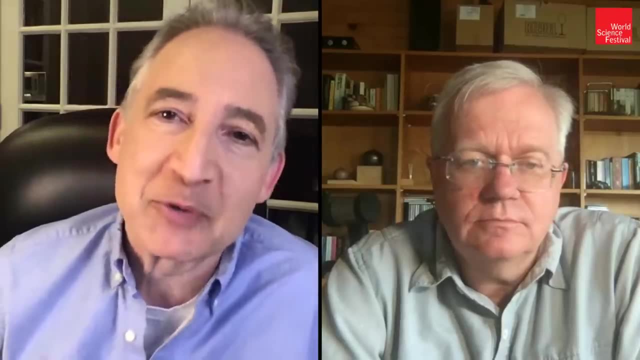 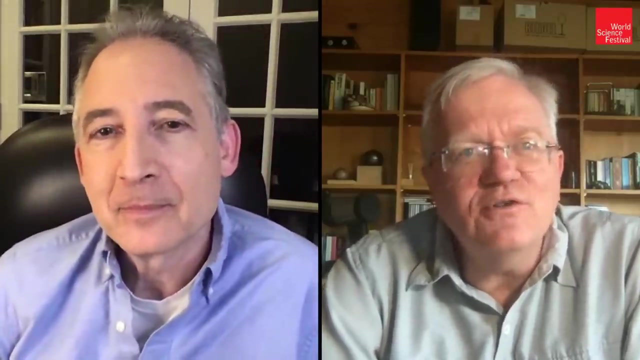 trillion years from now. the accelerated expansion, if it persists, will give a version of the universe that could itself deeply mislead observers in that distant epoch into thinking that there's nothing else out there. Yeah, And I've come full circle on this one over time as well. 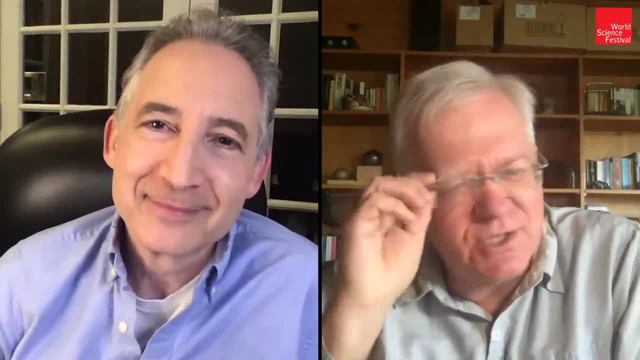 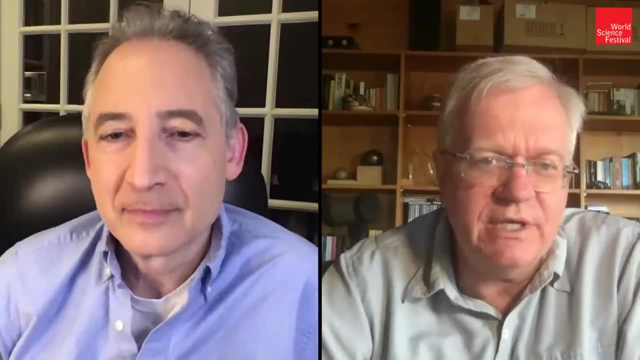 I think I hang out with you And people like you too much, Because I used to be. you would have you know 20 years ago when we did it. it bothered me. I'm like how can we be in a universe that has a beginning, has no end? 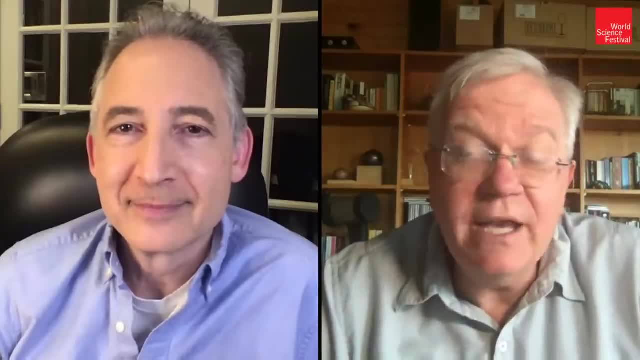 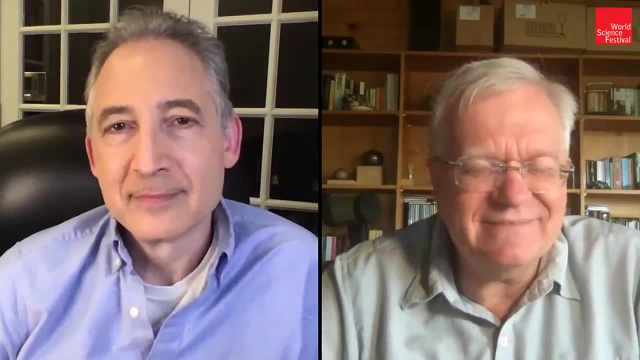 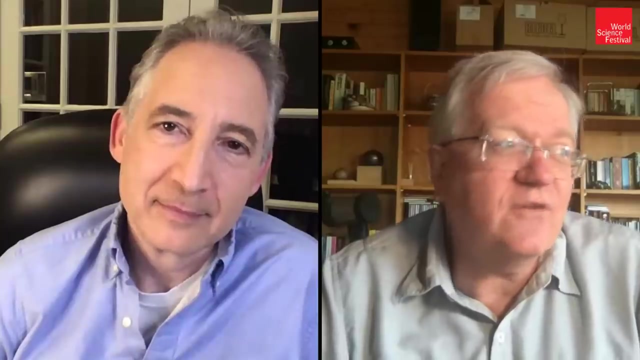 and we live in this special time where we can measure, And I find that very perplexing. I mean, you'd never want to be at a special time, but it does seem like the world we're in Now. that is why- aesthetically, but not for any other reason right now- for me, 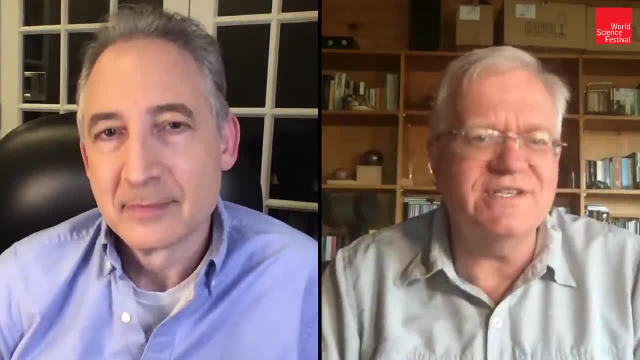 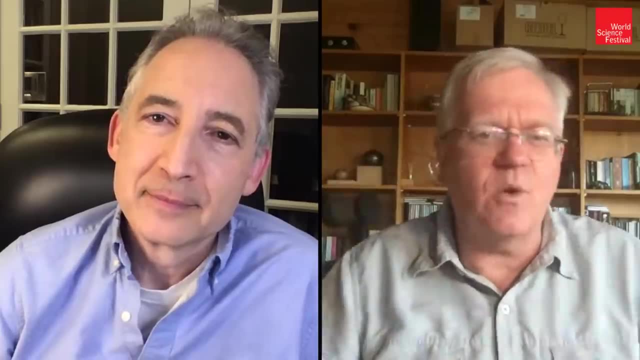 the idea of us being just one of a multitude of universes that are disconnected and go on. then, aesthetically, I can start dealing with it. This is okay, but it's just. there's an infinite number of these going on. 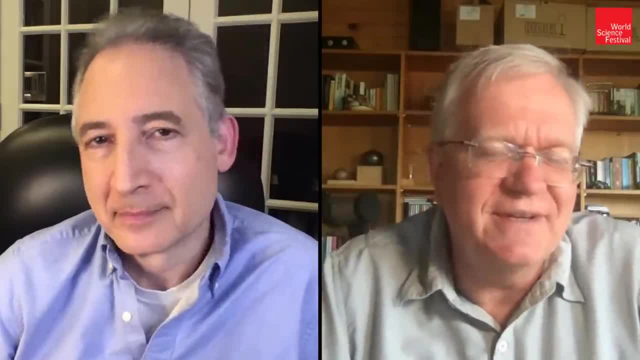 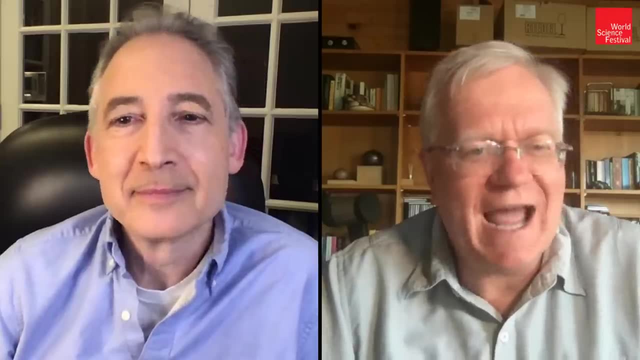 So that's just the way it works That I can deal with then. I'm not quite sure I can express why, but it seems like then it's quite a natural thing to be in. We're in a universe at a time when we can live and exist. 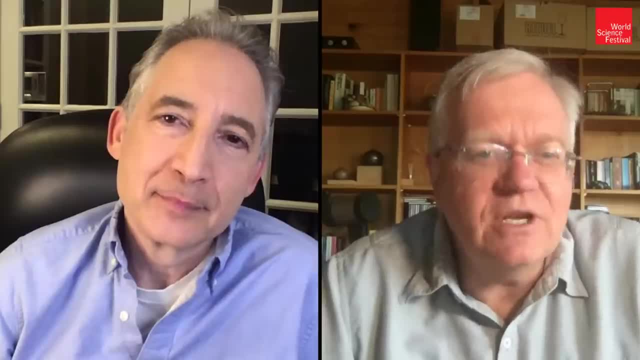 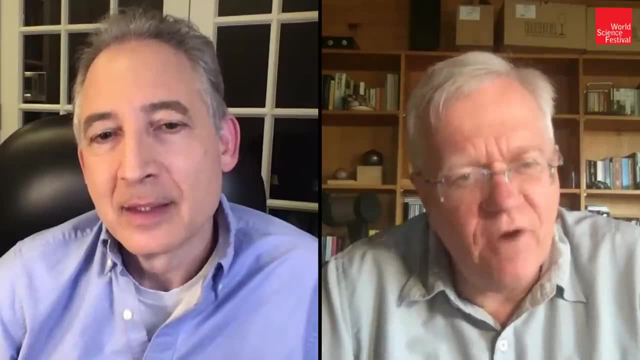 even though it's infinite. But there's an infinite number of them. It makes it less and less special. Yeah, sure, So that's sort of where I've come to on this. But if ours is the only universe, then I find it pretty deeply disturbing. 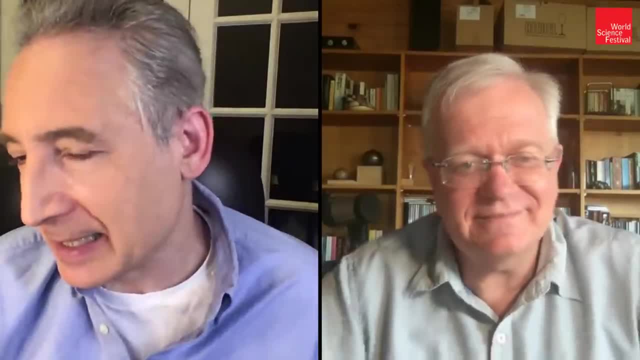 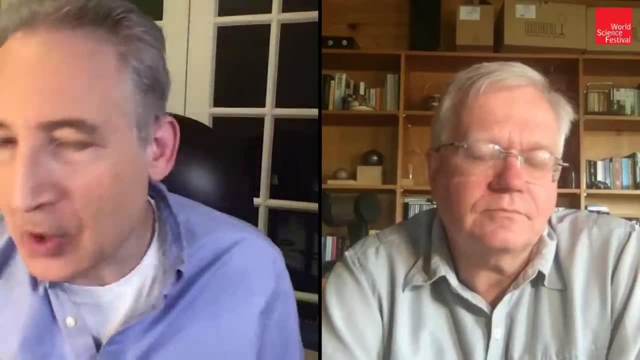 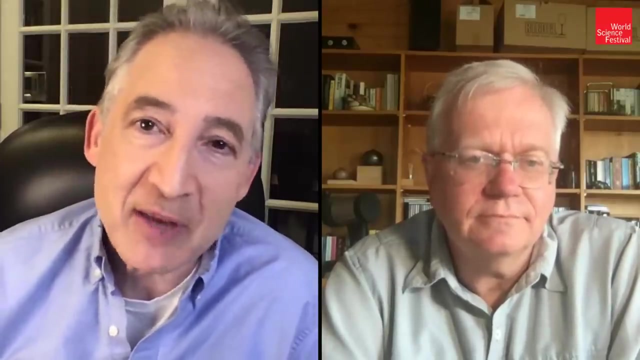 Yeah, yeah, No. you can sort of look at it two ways. Perhaps this special time is also characteristic of self-reflective beings, right? I mean the conditions necessary for us to even be here, to be able to talk and think about these things. 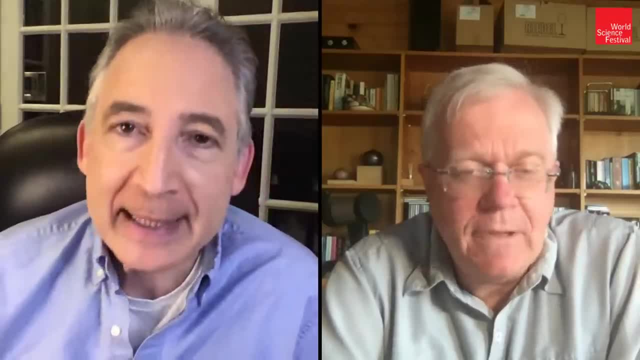 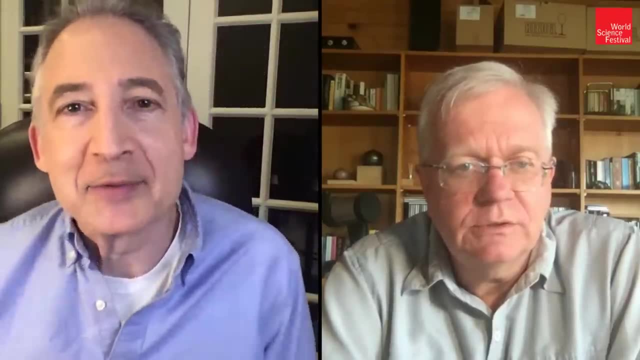 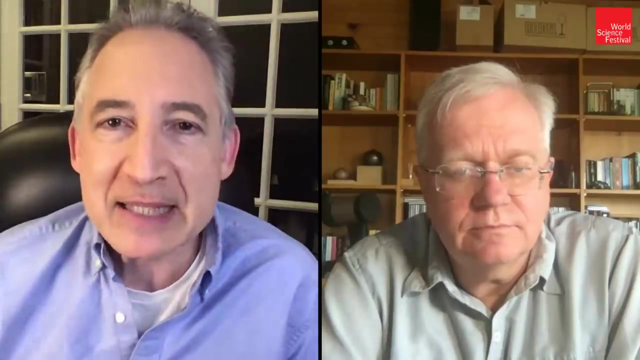 requires certain special conditions too, And they're not thoroughly independent of each other, As we know. if the cosmological constant had a very different value, you wouldn't have the formation of structures that are necessary for a living system such as ourselves. So maybe we should take the specialness and celebrate it. 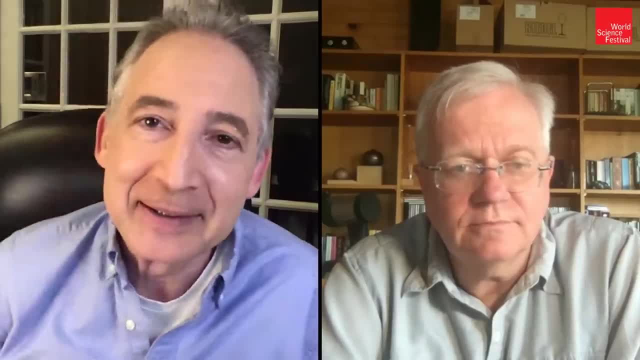 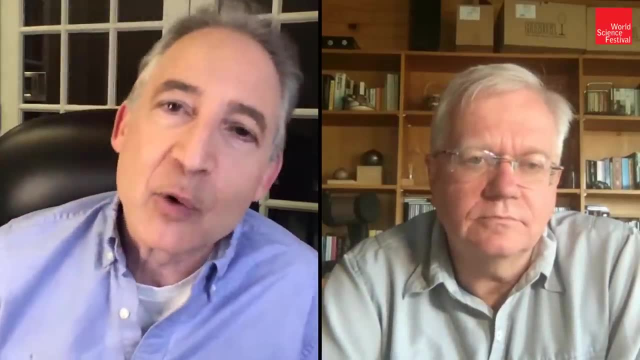 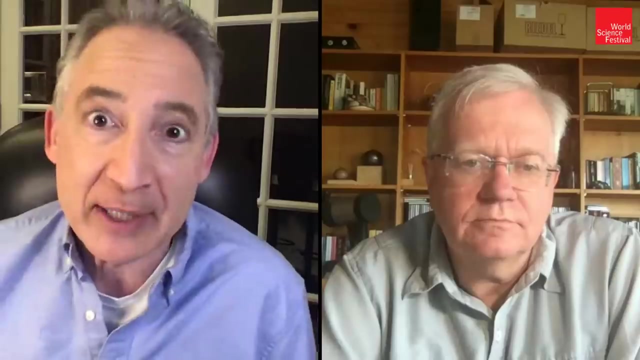 and thank our lucky stars literally that we're here and just interpret it in that most flat-footed of ways. But yes, we scientists, of course, are generally happier if we don't have to tune the dials, if it just turns out that the most generic conditions 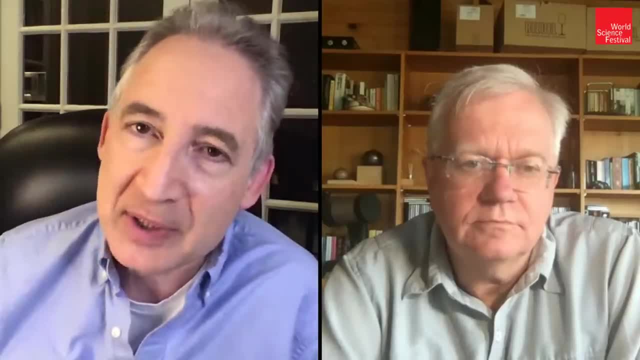 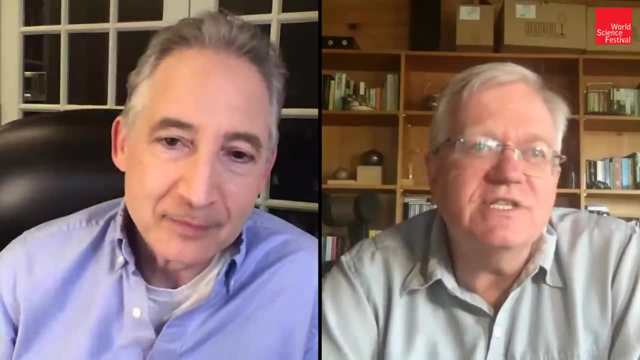 allow the universe as we know it to persist, But that certainly does not seem to be the universe at the moment that we're in. Yeah, but if there's a bazillion universes out there, of course we will be in the one that allows us. 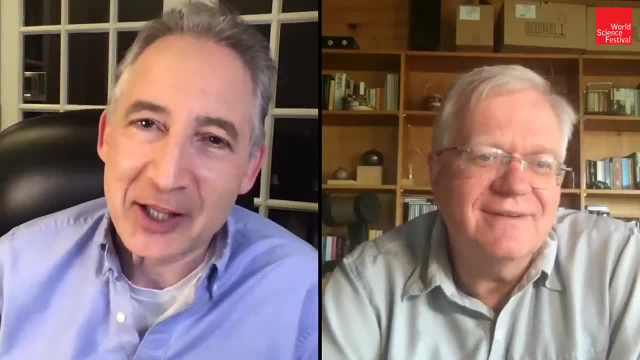 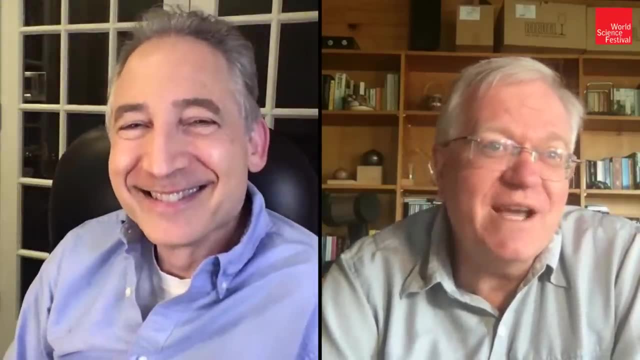 Yeah, so I can start. Now you're talking like a true string theorist, you know, No, I It's the only way I can reconcile the crazy universe we live in. It doesn't mean it's right, but at least I can deal with it aesthetically. 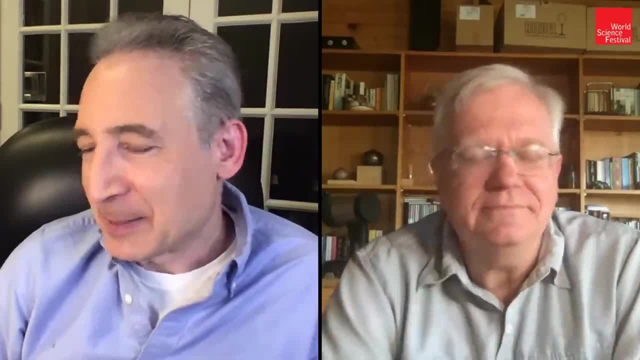 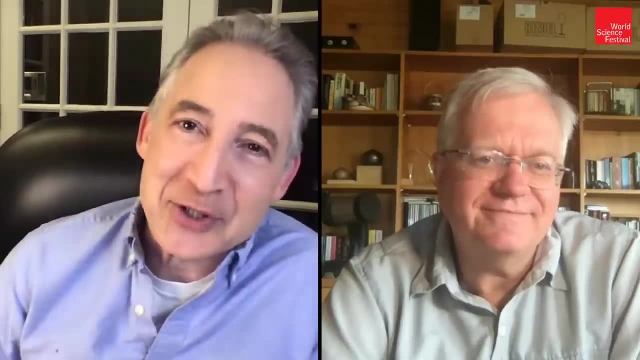 Yeah. no, it's To make it just an environmental condition that has to happen somewhere in a multiverse that has enough universes certainly at least gives some semblance of an explanation. So I think many people have taken solace in that. 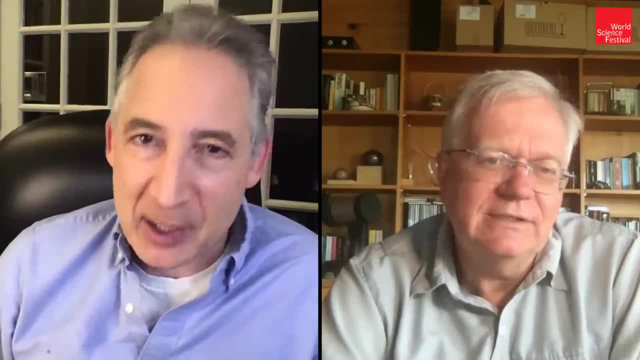 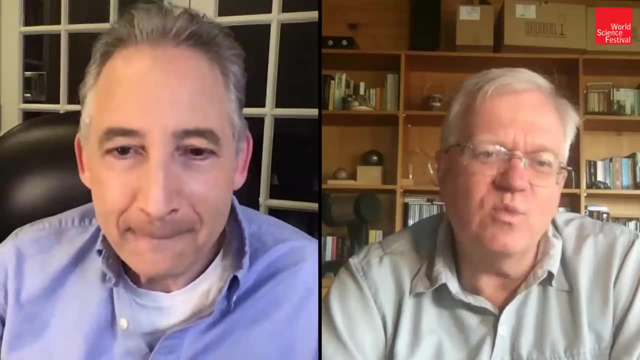 But, as you say, it's a pretty dramatic move. It's the anti-Ockham's razor approach, if you will. so, Yeah, well, I would say it's almost like finding religion again, In a sense. yeah, And so where did? 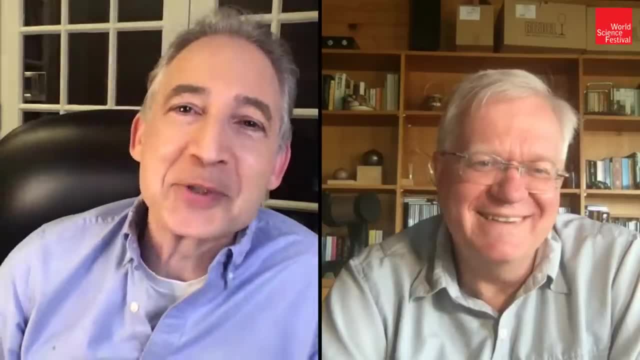 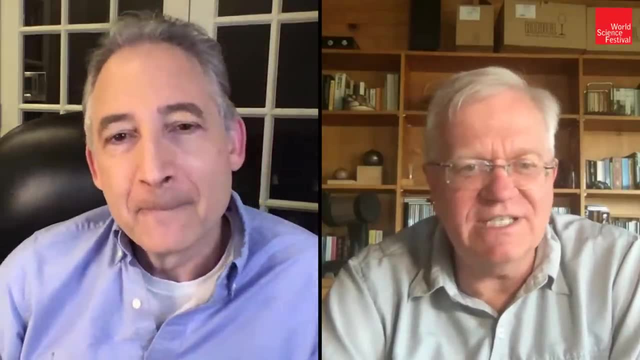 I wasn't going to bring it up, but you did So. where do you stand on the? I assume that you're not religious. Is that I am what I describe as a militant agnostic? I fiercely defend the fact that I don't know. 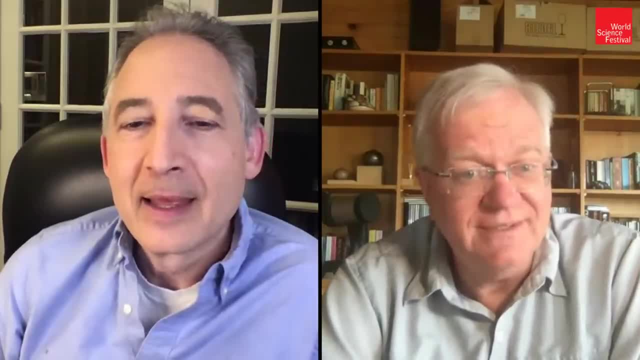 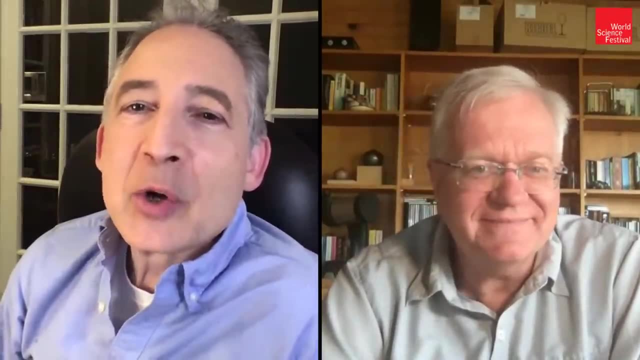 And at some level I fiercely defend the fact that I don't care. So I have no problem with people being religious, but I'm not, And that's fine. Go do what you need to do. So Einstein in some ways had a similar view. 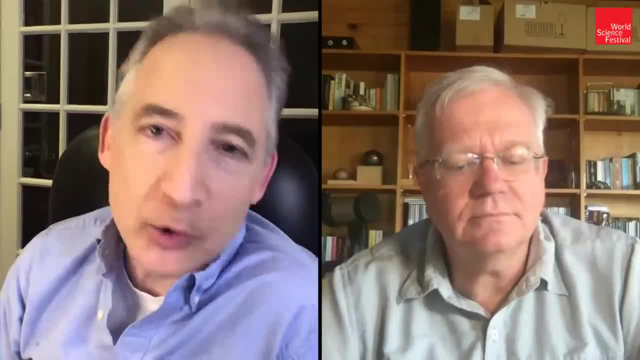 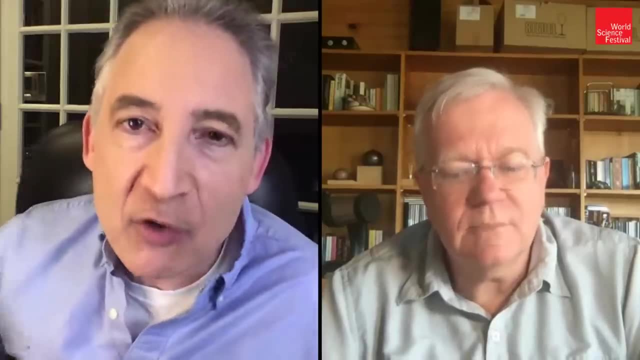 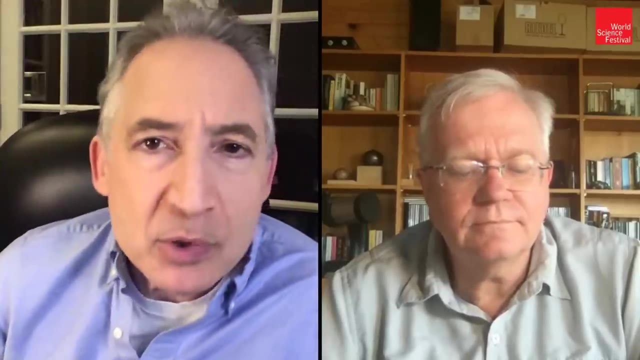 but people love quoting the fact that he would often invoke the old one God, things of that nature. Many of us interpret that as Einstein simply talking about the laws of physics. Yeah, in some poetic language. But would you consider yourself to be a spiritual person? 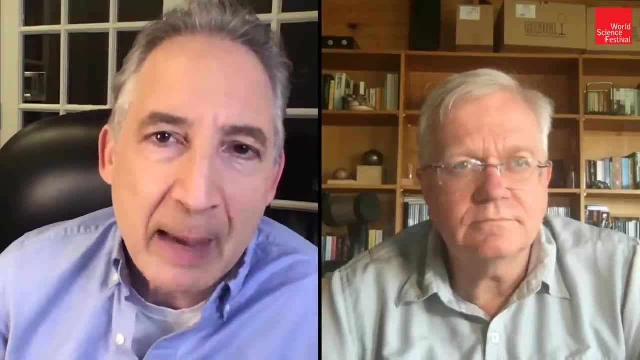 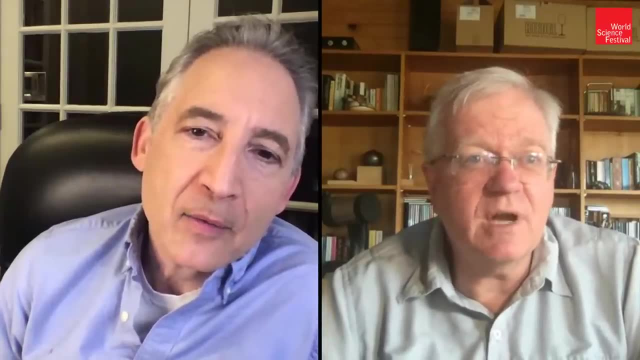 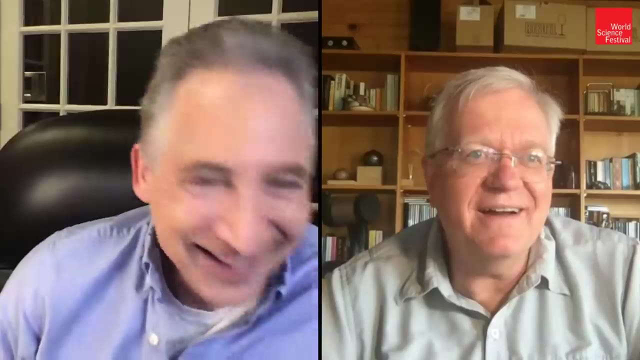 or is that also too far afield for that word to be applicable? No, I'm not spiritual at all. I'm quite the opposite. I'm kind of dry and boring. I'm really. I live through life as a Bayesian And I don't. 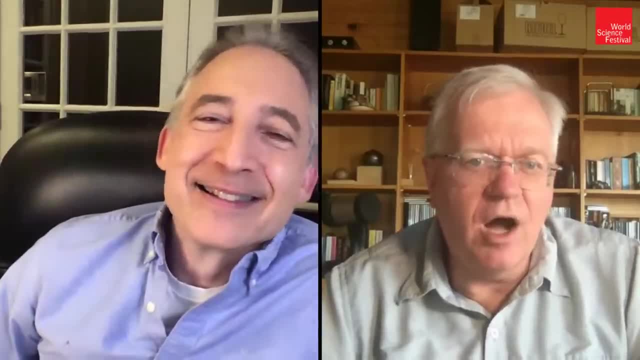 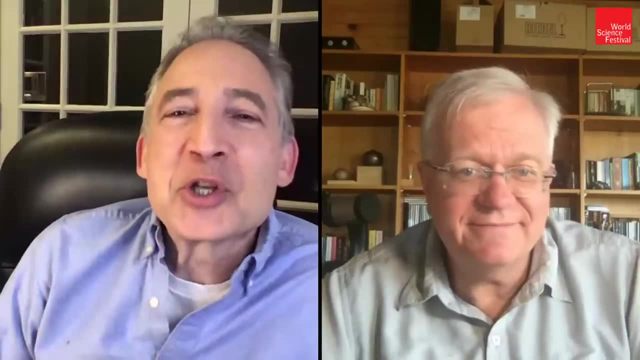 I talk about concepts like God and fate and stuff, but I don't believe them at all. I just like you know, life sucks sometimes. You just got to move on. So but when, for instance, you first stared at the data, 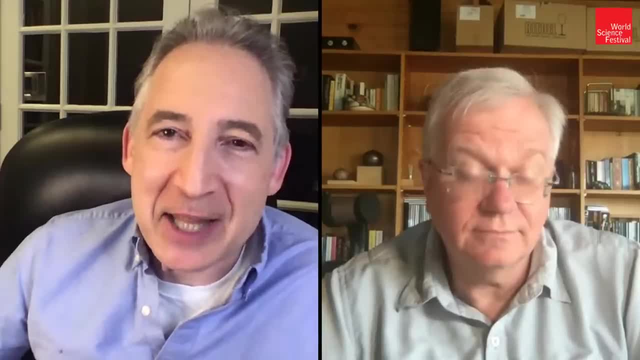 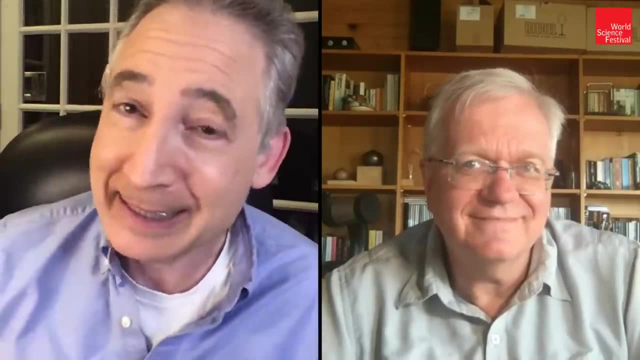 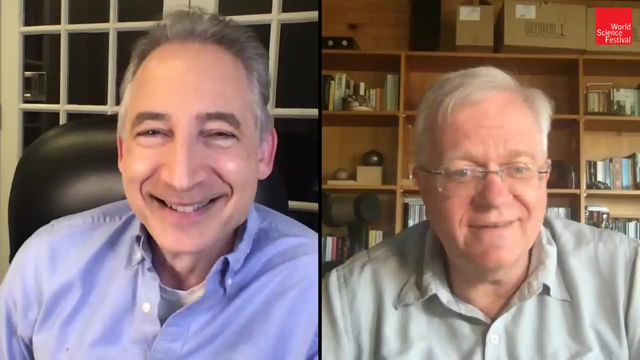 and see that the expansion is accelerating. did you get a little tingle in the spine, a little catch in the throat, or was it again just hey? okay, Bayesian, that's where the Bayesian analysis has taken us. No, my reaction was: oh Christ, there goes my job. 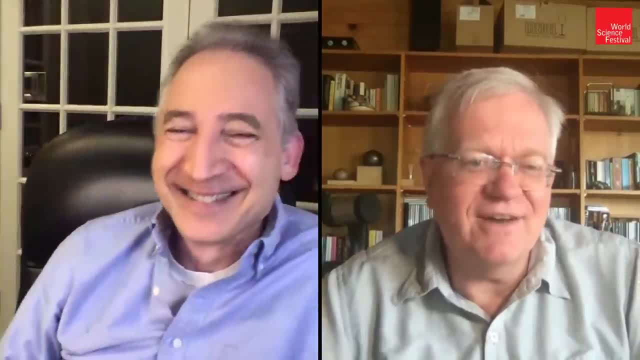 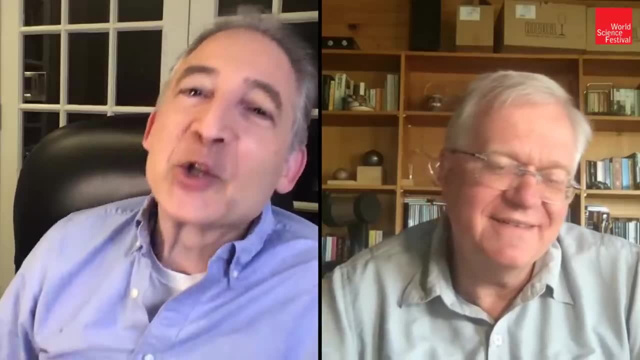 Oh, we're going to be a laughingstock. This is awful. This is a career-ending discovery. That's what I thought it was going to be. All right, final attempt As you look back on the discovery with you know hindsight. 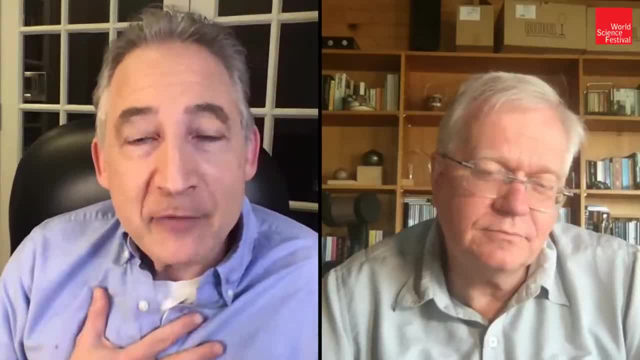 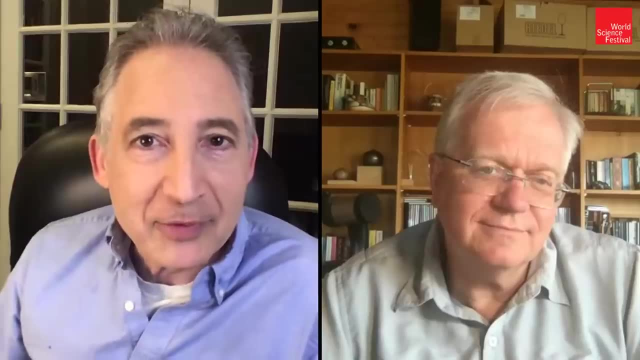 20 years of hindsight. does it give you an emotional reaction or is it still very cut and dried, the data that's where it led, and so forth? Oh no, I mean it was emotional. I mean, but, as I said, 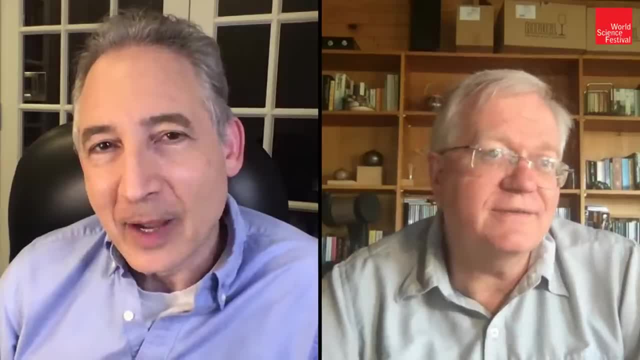 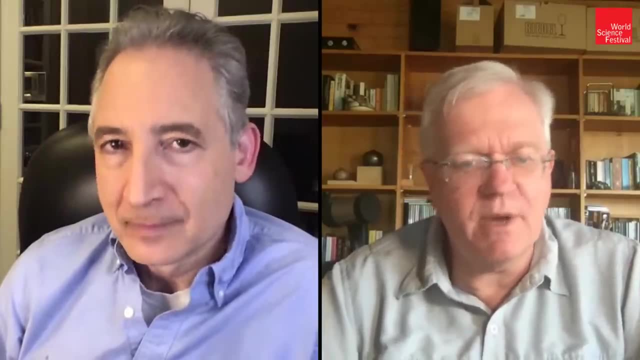 I was more than happy. I was more worried of it just being crazy and wrong Right. But no, the journey and the excitement of realizing it was right- that still gets my heart going. It was just an amazing thing to be part of. 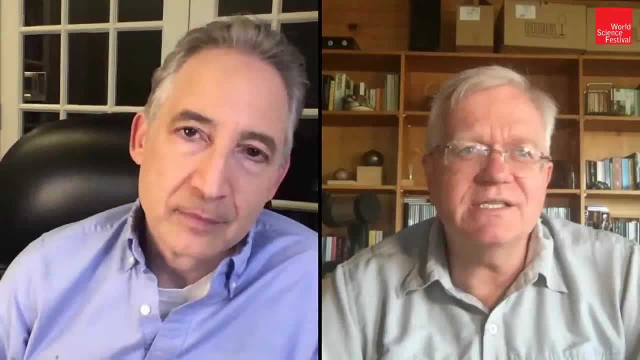 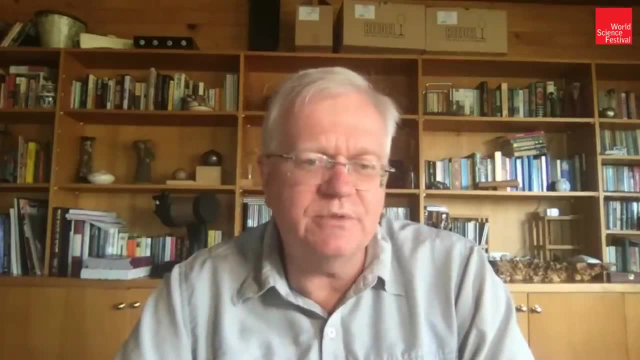 You know, one of the problems of a Nobel Prize, I guess, is that it's like: oh, but you guys are these amazing geniuses who made this discovery? And the answer is no. We were normal people doing good work, like most scientists are. 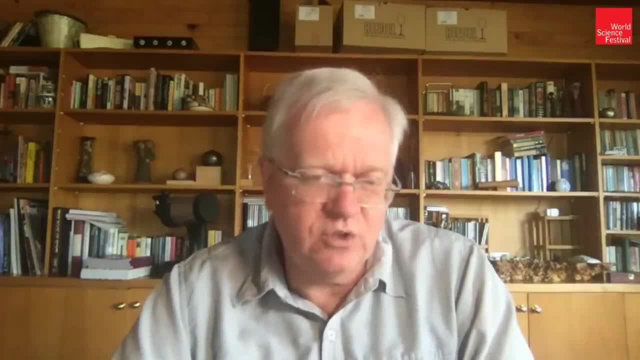 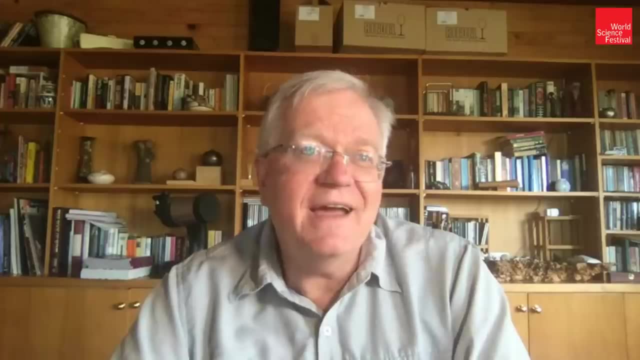 and we ended up being at the right place at the right time, doing good work, And it's sort of like we got the ticket to be on the roller coaster at the right time. Yeah, And it's a privilege. you know, It's a real privilege to have been in such an interesting time. 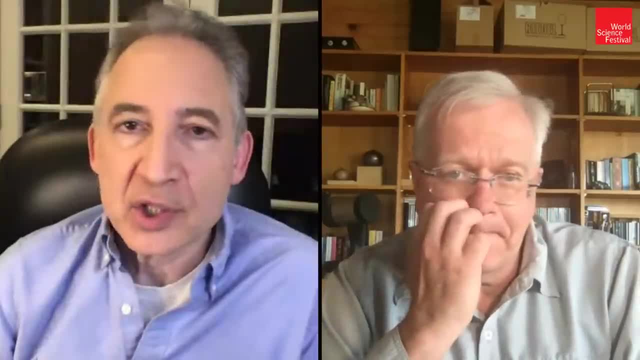 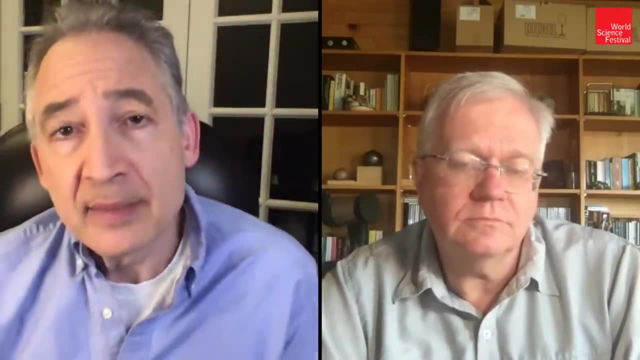 in cosmological history. Yeah, I mean, that's such a profoundly important message and lesson, especially to the younger folks who may be listening to us now, that in the end, you follow your passion, you see where it leads and, if you're lucky, 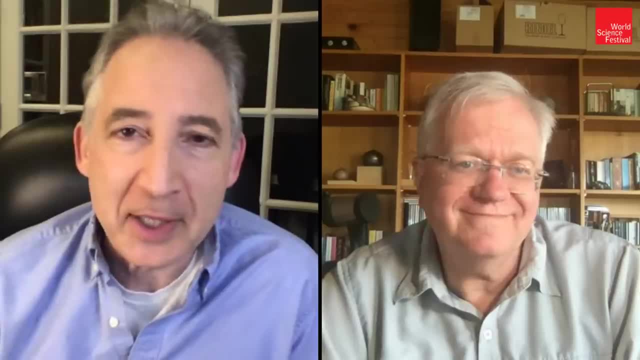 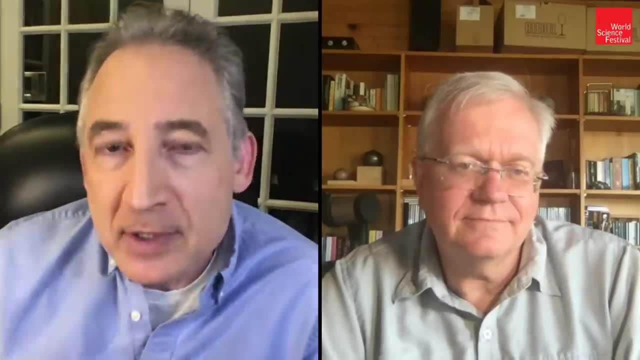 you'll have a few moments of great discovery And if you're really lucky, one of those will yield something like a Nobel Prize. But in the end you're doing it because you're driven to do it. It's exciting, It's something that catches you at a deep level. 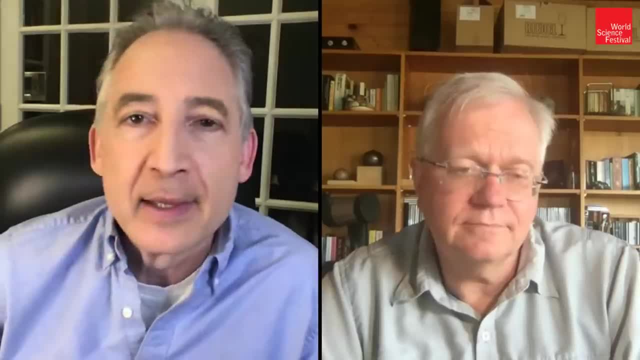 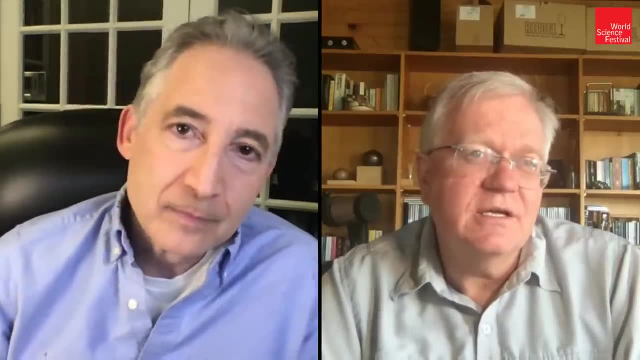 and it's something that you want to do And the prizes are kind of the icing on the cake. I think that's Yeah, And that's why when you said, you know, the highest achievement, Nobel Prize, is the highest recognition. 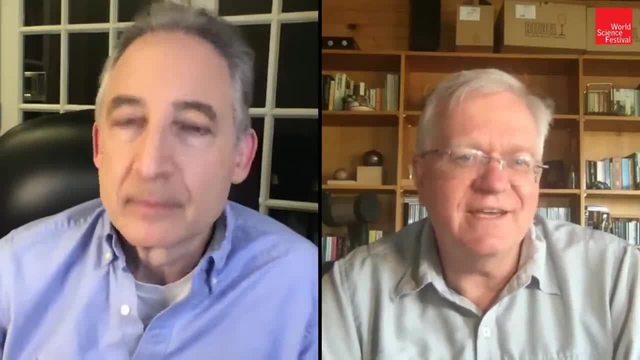 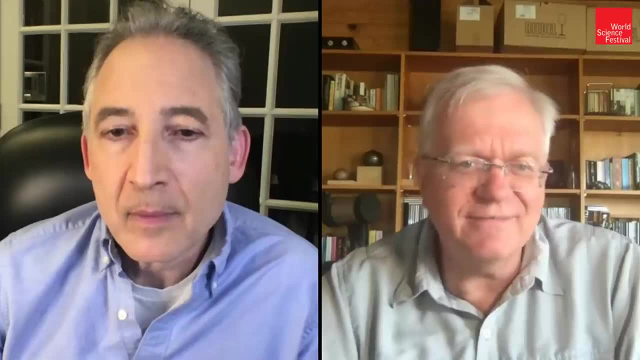 Recognition. Absolutely The highest achievement was the discovery in 1998.. That to me is: you know, that is my People, you know they say: what is your highest achievement? I'm like, well, I'll have to admit it was this. 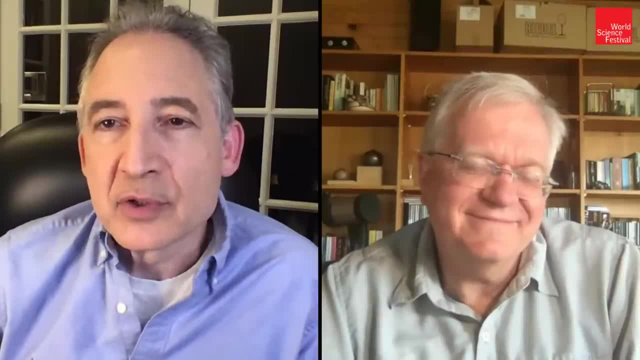 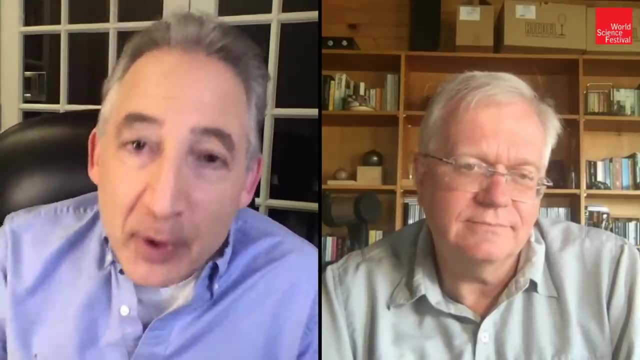 and nothing else is really going to be close. Yeah, Without a doubt. Well, Brian, thank you so much for joining us. This is a great, fascinating conversation. I have no doubt that our audience was thrilled to go on this journey of. 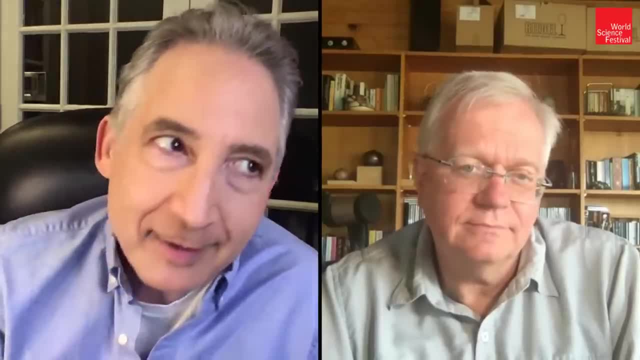 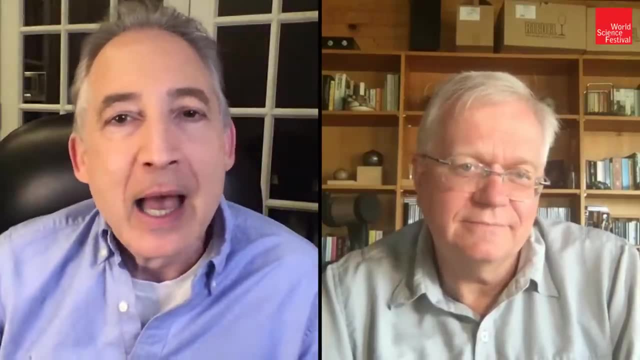 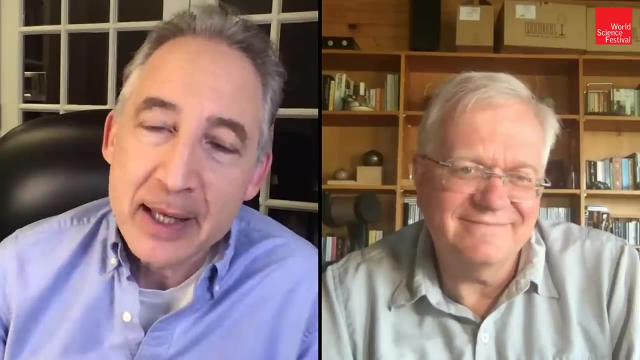 your life and this great discovery and this great achievement and this great recognition all wrapped together into one powerful package. I hope to see you next year at World Science Festival of Brisbane, assuming that the world allows that kind of travel to take place, And no doubt. 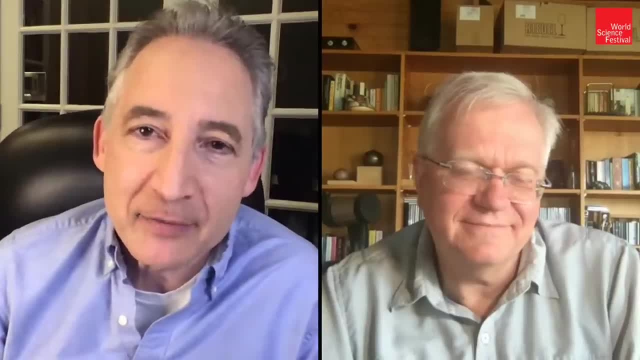 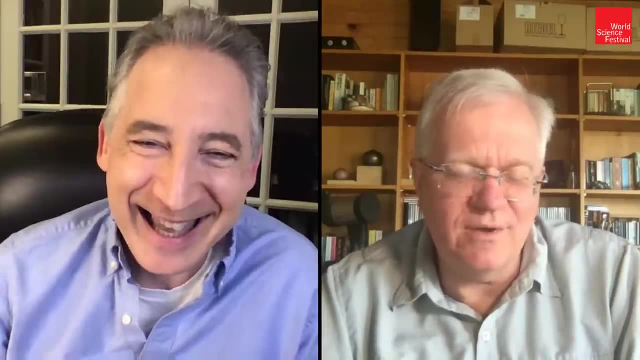 maybe there'll be an opportunity for our paths to cross before then, But if not, thank you for joining us and I look forward to seeing you then. All right, Thank you very much, Brian. Be well, Absolutely, You too. All right. 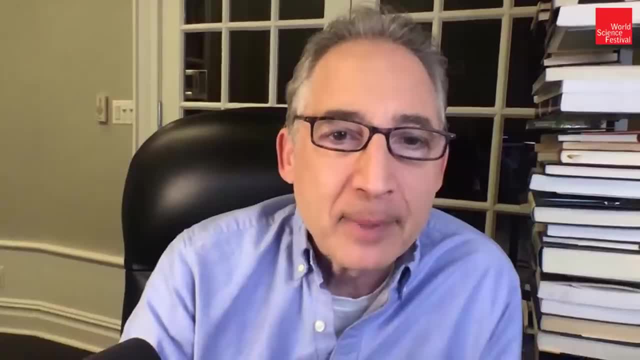 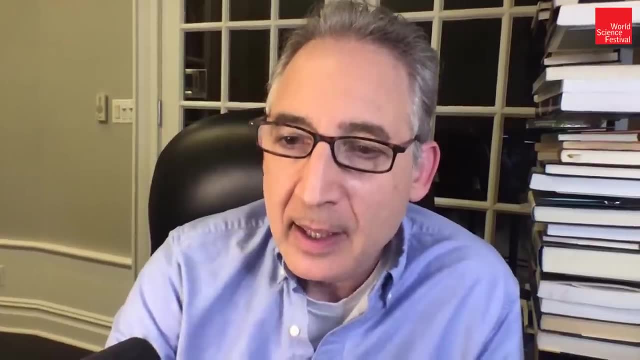 guys, that was our conversation with Brian Schmidt. Before we wrap up here, let me just see if there are a couple of questions in the chat that I might address. There was one, actually that came in a little bit earlier. I think I may have written it down. 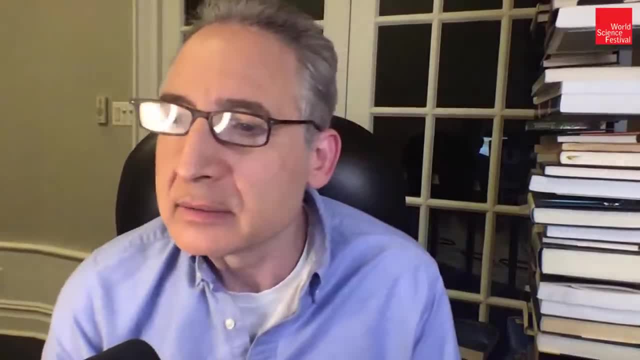 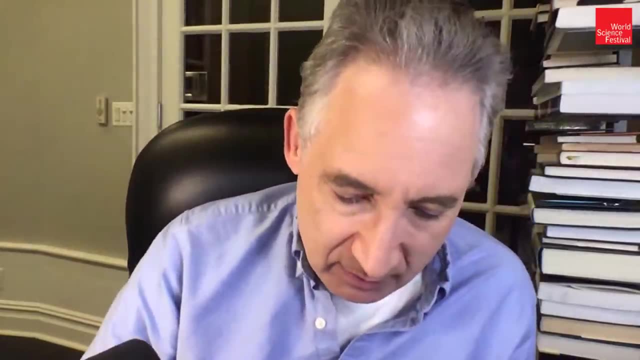 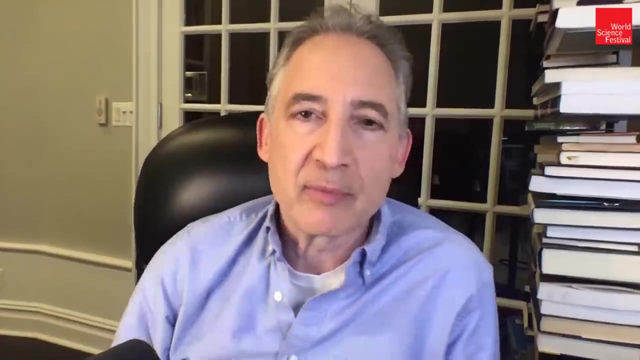 David Perry sent me an email having to do with the microwave background radiation, And it's a worry that David raises in his question to me that I think others may have, So it's perhaps worth spending just a brief moment on it. Sometimes, when we talk about the heat, 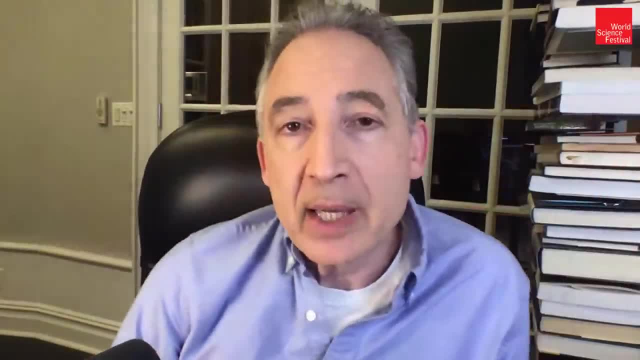 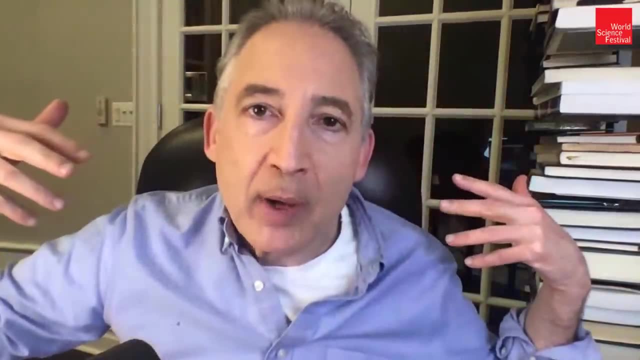 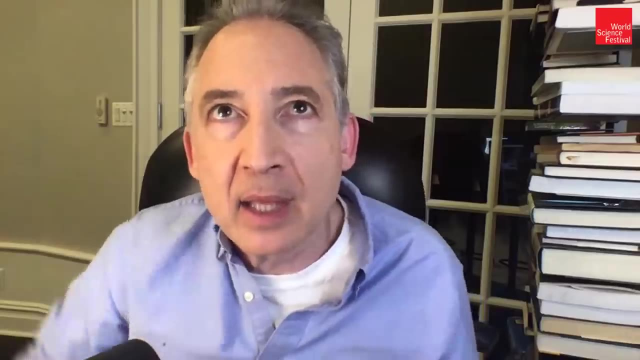 the light left over from the Big Bang, you might ask yourself. well, when we look up, isn't it a coincidence that that light just happens to be blowing by planet Earth at this moment so that we can measure the microwave background radiation? You might think that once it blows by us, 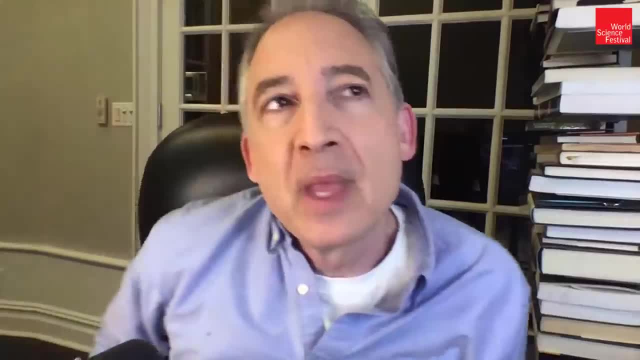 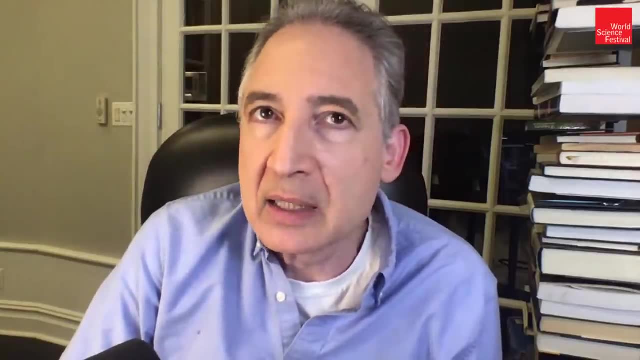 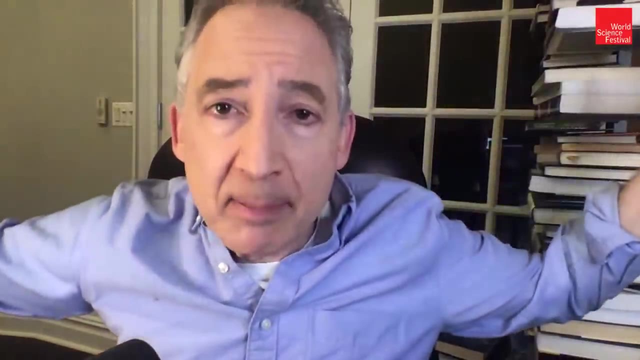 the radiation will be gone right, And it's a natural thought, but it brings forward a quality of cosmology, as we understand it, that's quite distinct from the intuition that that question illustrates, Because let's imagine a possibility that the universe is infinitely big. 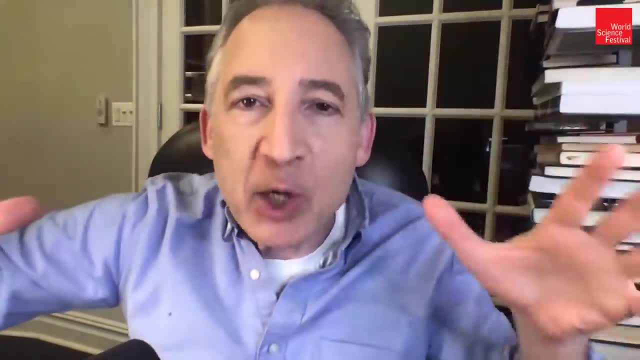 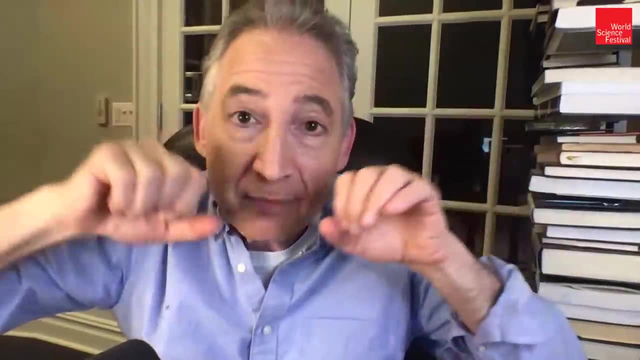 Space might go on forever, And if that's the case, this microwave background radiation permeates all of space. It's not as though it took place at one location and has been traveling outward from that one location. If that were the case, then yeah. 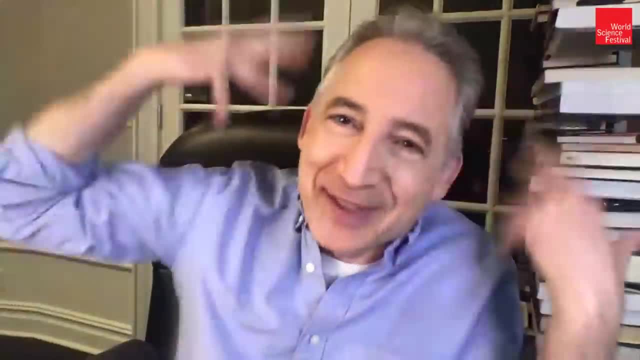 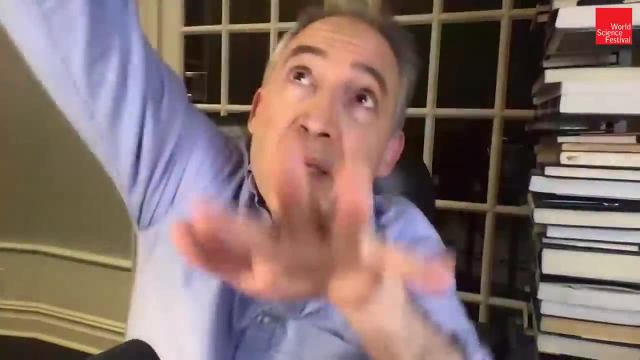 you better be at the right spot at the right moment for that radiation to blow by you. But if that radiation fills all of space, then it is going this way and that way and this way still all of the time. So whenever you look out into the cosmos, 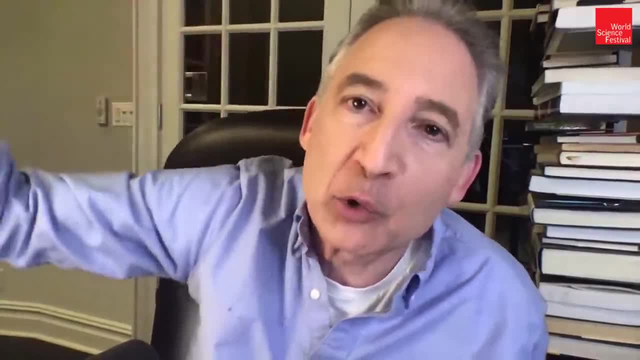 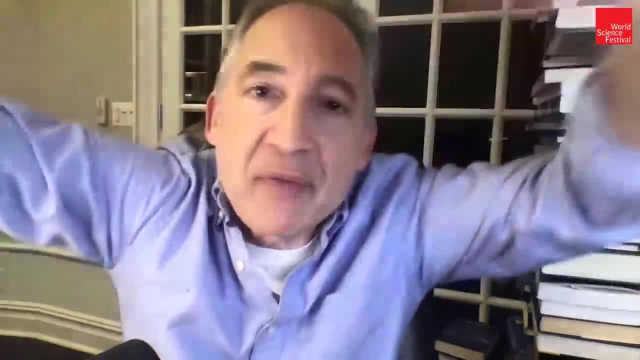 there will be a point from which a photon from that early epicenter, a photon from that early epoch, is just reaching you, because those photons were released from every location throughout this infinite cosmos And therefore there's always a source that will be the relevant one. 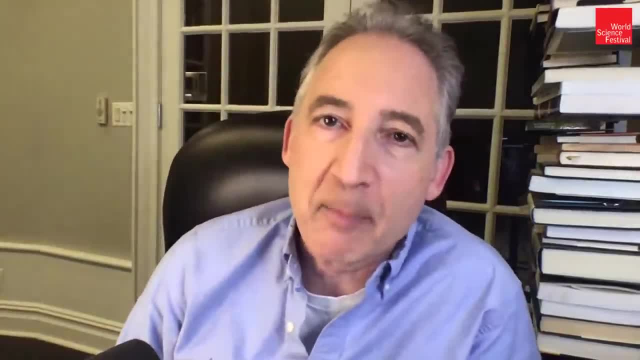 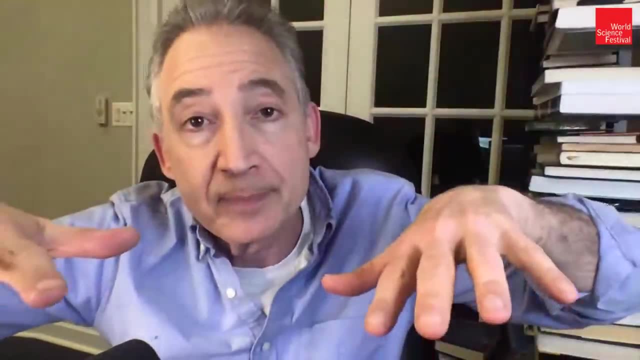 regardless of when you look out into the night sky. So the microwave background radiation will be with us in some sense forever. It is the case that in the far future, the temperature and the redshift of that radiation, the temperature, will get so low. 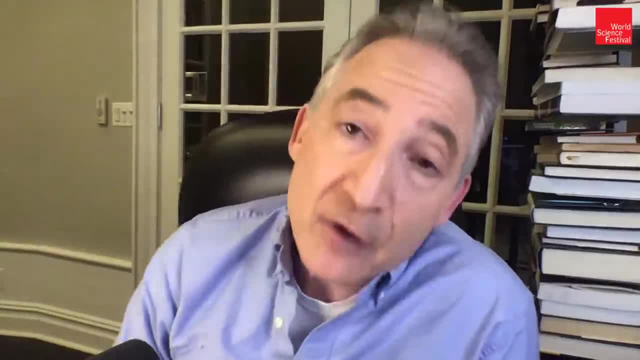 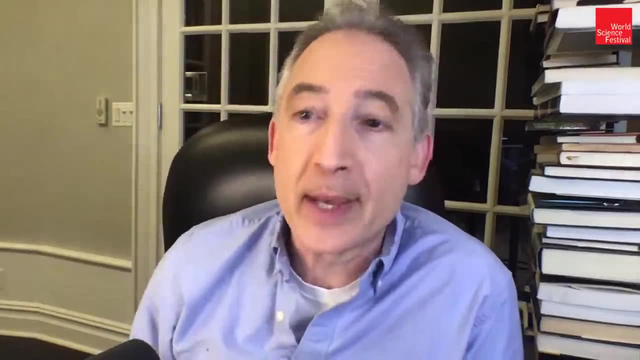 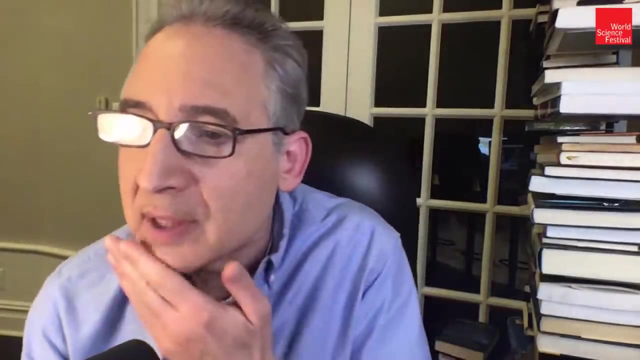 the redshift will become solar right. It will become so large that in the future it will be very difficult to detect the microwave background radiation, but it will still always be there Nevertheless. another question about the microwave background radiation I see here from Maximilian Egger. Have we measured the CMB from other vantage points, like the moon? Well, the measurements of the microwave background have largely been taken either from balloon based experiments, where people will go up above the atmosphere with specialized equipment, or from a telescope that we've launched. 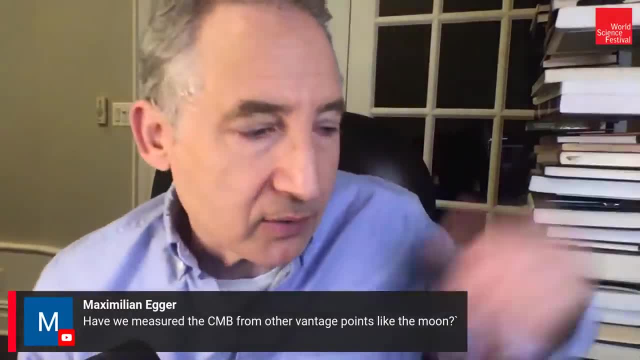 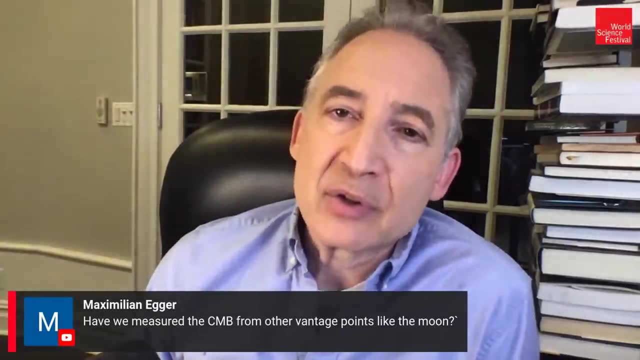 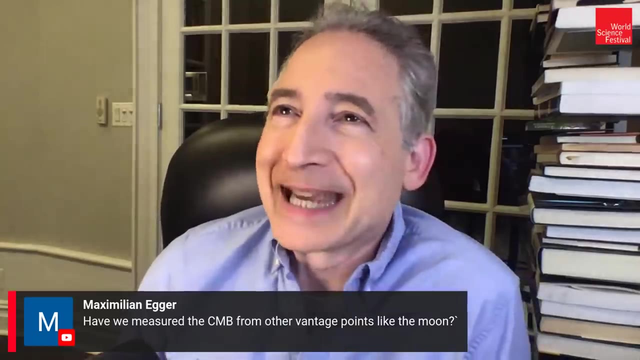 like the Hubble Space Telescope or the James Webb, when it ultimately goes up. These machines, these instruments, have the capacity to measure the microwave background radiation. I do not believe that anyone's ever. I think the answer is no, that we've never taken it from them and I've never heard of it. So I do not think so, But ultimately it will be the case. that will. you know, once humanity spreads to other planets and other star systems, then, yeah, we'll be able to, in principle, measure the microwave background from another vantage point. 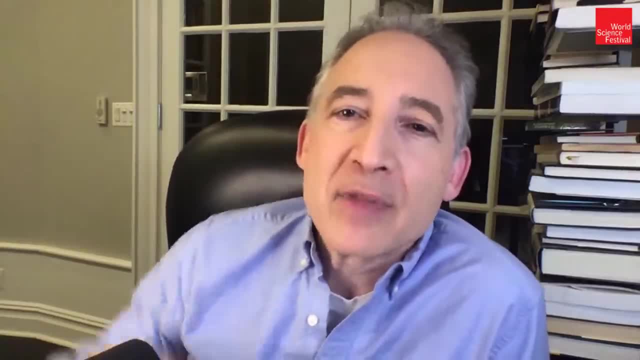 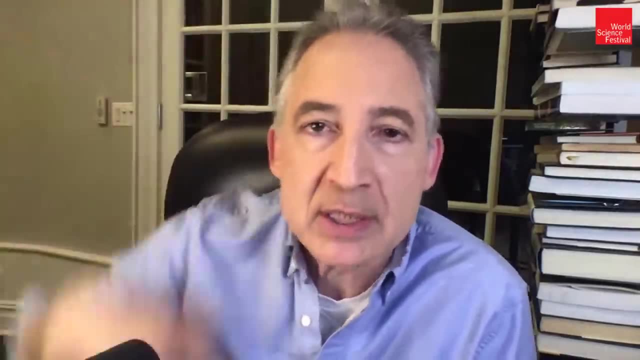 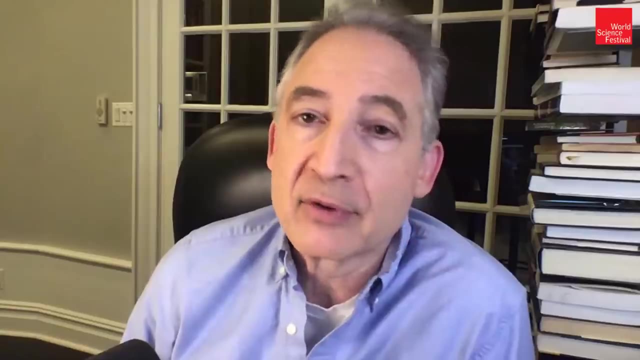 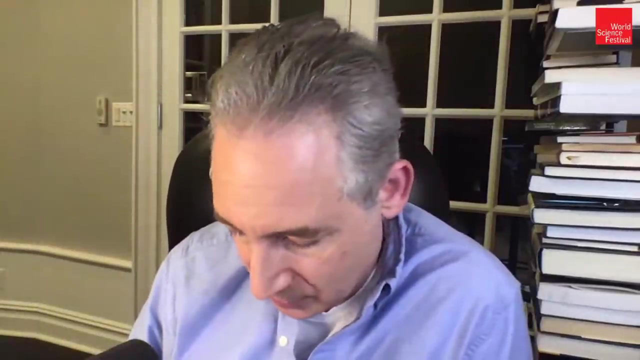 Now, our belief is that, because of the homogeneity, overall homogeneity and isotropy, no special directions and no special positions in the universe- our expectation is that the measurements won't matter really where we take them from. But certainly the confirmation of that expectation by virtue of taking the measurements from other locations will be a valuable thing that ultimately will be done. 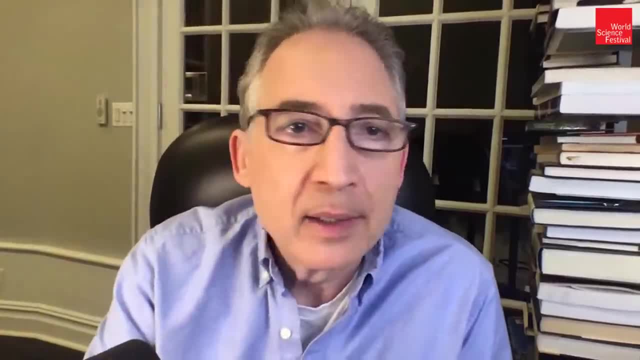 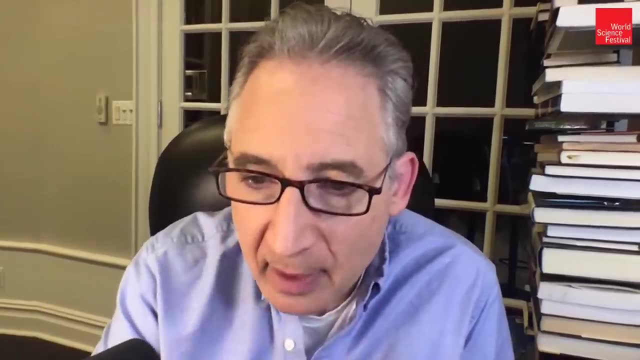 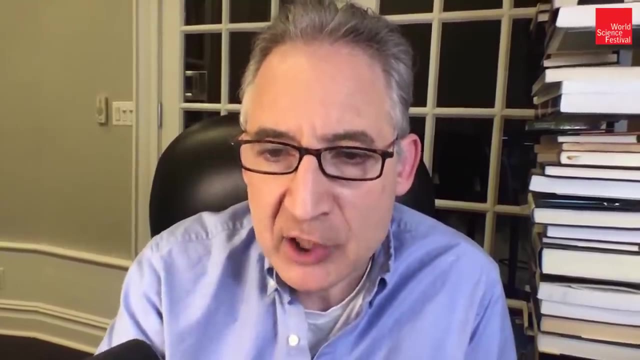 What else do we have here? Let me switch over to the live chat. And yeah, I am, I cannot read anything without my glasses on. So Let's see what we got. Alexander Johnson, what does the expansion of space look like from the perspective of string theory? 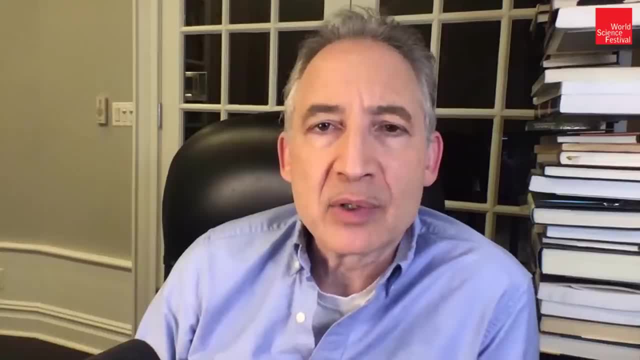 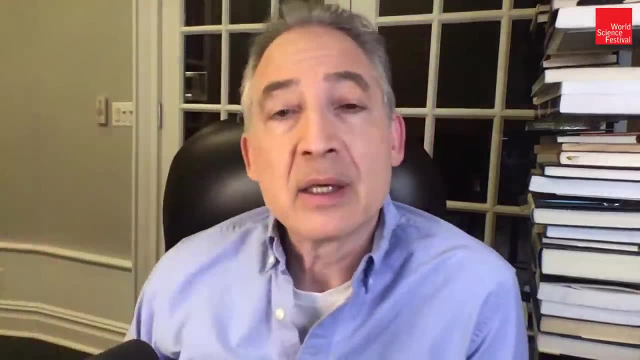 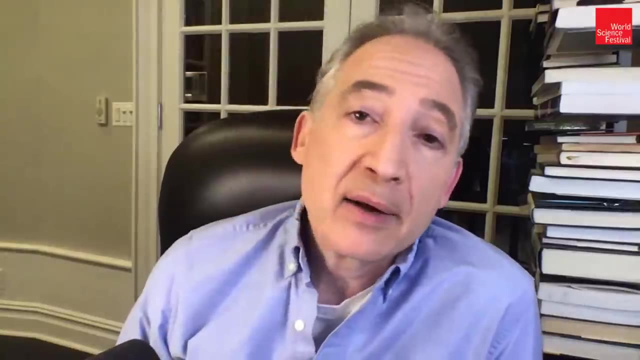 And not much different from what Brian Schmidt and I were talking about just a moment ago. Within string theory, you can have cosmological models that address the accelerated expansion in much the same way. Imagine that there's a cosmological constant. You can have other models of expansion. 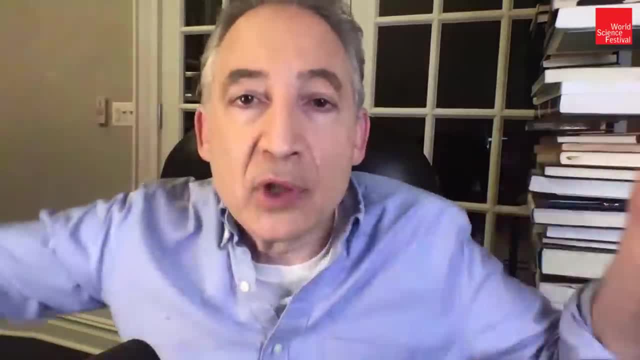 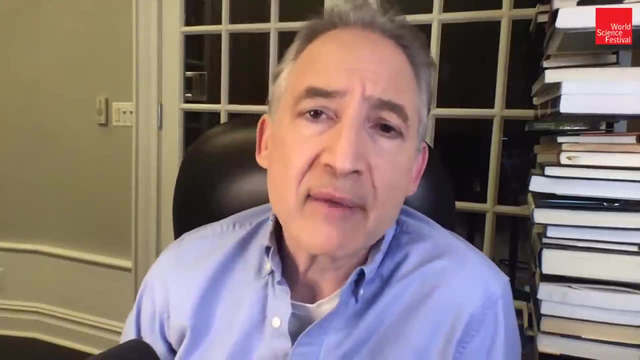 in string theory that allow for the universe to expand and then come back and then perhaps undergo a bounce-like solution. These kinds of evolutions are compatible with our understanding of string theory. They're not picked out by string theory- String theory, unfortunately. 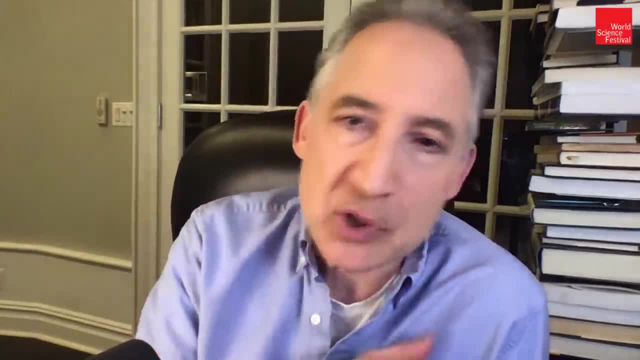 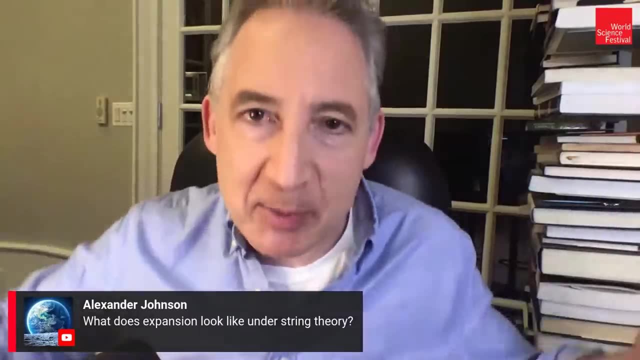 isn't understood at a level yet where, from first principles, you just follow the equations and you say, aha, this is what happens in the cosmos: Accelerated expansion for ever or for a while. Unfortunately, you can't get that from first principles. 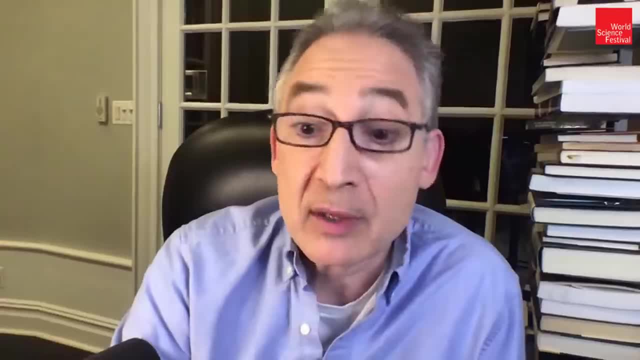 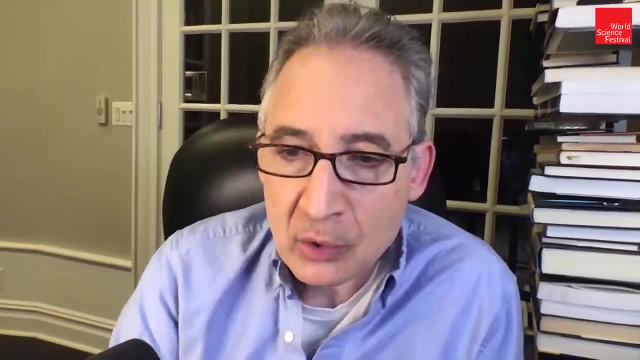 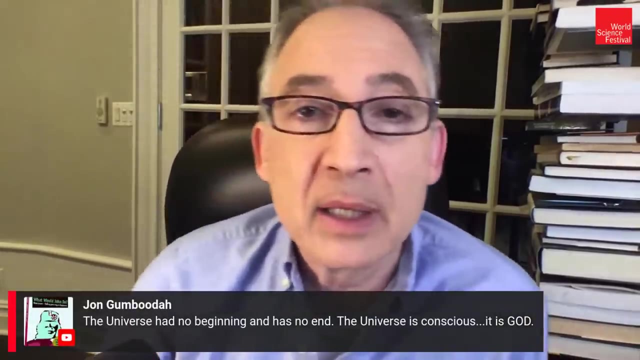 but you certainly can make models within string theory that are compatible with those observations. John Gumbuda says the universe had no beginning, has no end. The universe is conscious. It is God. I don't know, I guess I'm not. 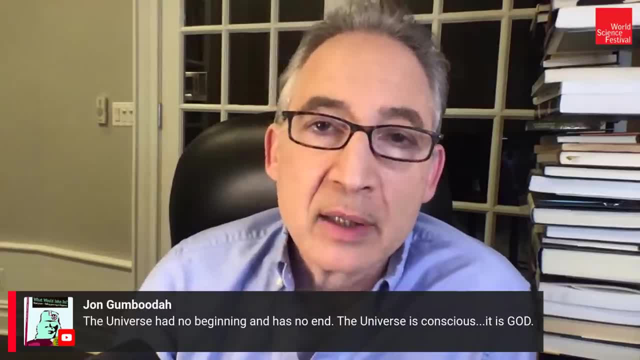 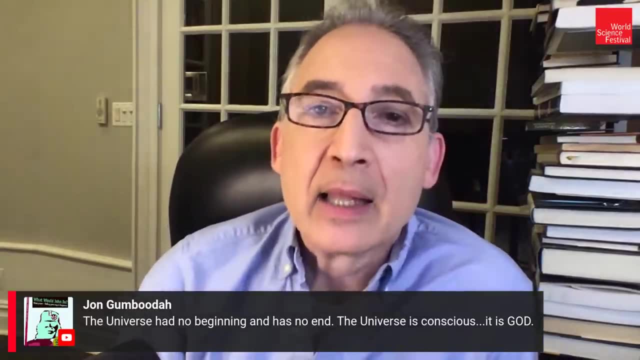 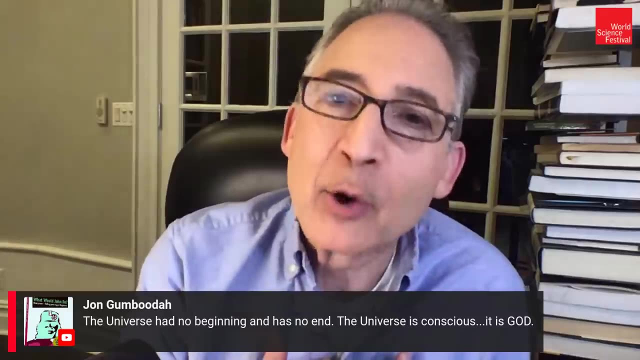 It's hard for me to respond much to that, John. Yeah, I mean it's hard for me to respond much to that, but the powerful tools of mathematics allow us to make calculations and predictions. that a God-like explanation would be, at least from our understanding. 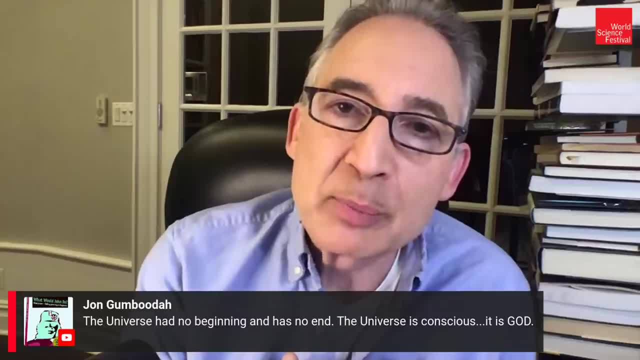 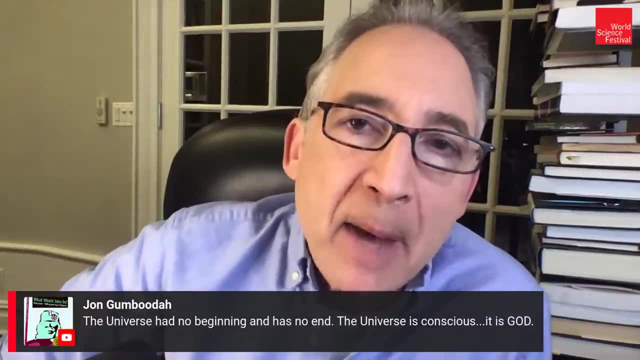 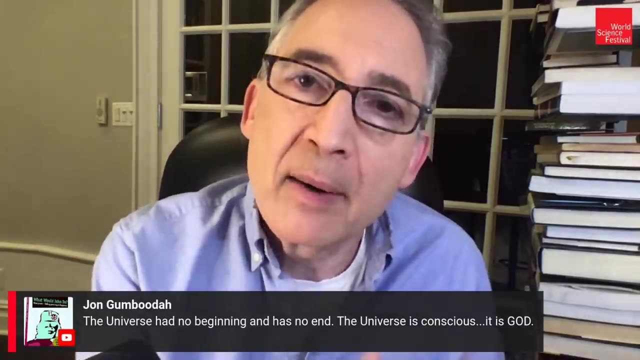 not able to do. I've never seen any theological perspective that can, for instance, predict the anisotropies in the microwave background radiation. Has anyone ever done that, by just positing God and then deducing from that assumption the anisotropies in the microwave background radiation? 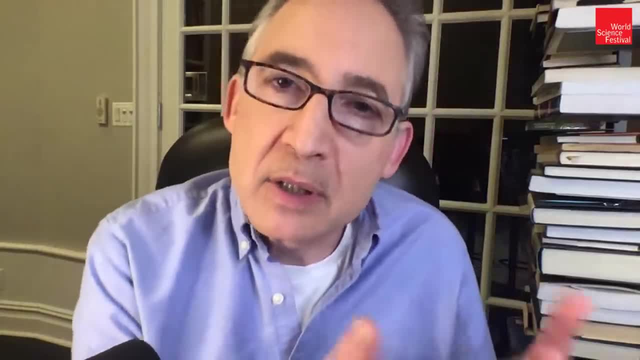 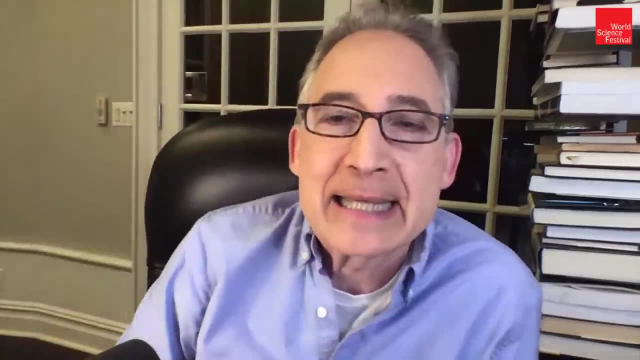 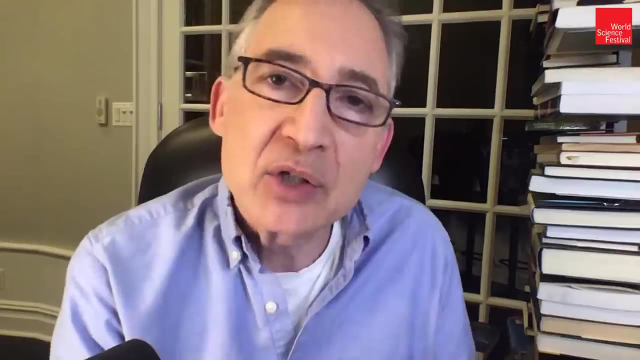 I don't think so, But under modest assumptions, using the general theory of relativity and quantum mechanics, we can make calculations of the temperature variations across the night sky and compare those to our observations, And so the agreement between our observations and the mathematical calculations gives us confidence. 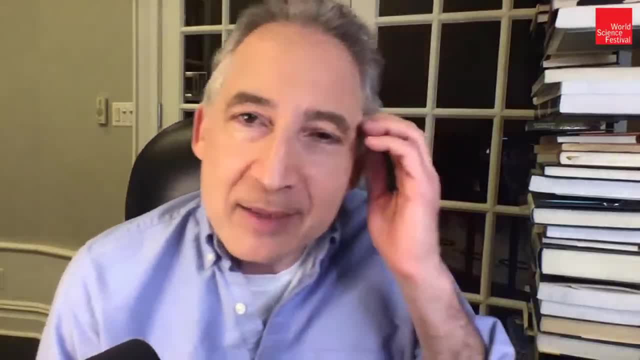 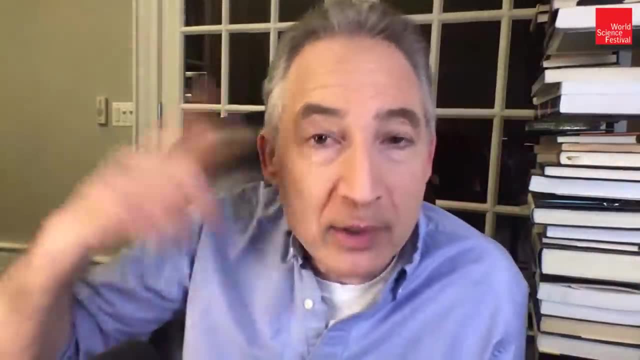 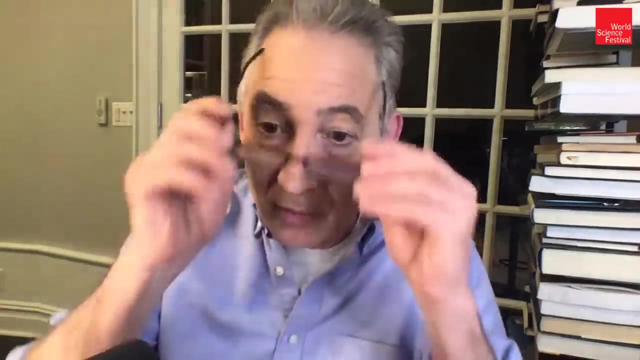 That, yeah, we don't have the full story, but the mathematical story that does involve a beginning and does evolve things evolving over time according to the mathematical equations, gives us confidence that we're tapping into some kind of truth, because the calculations agree with what we see. 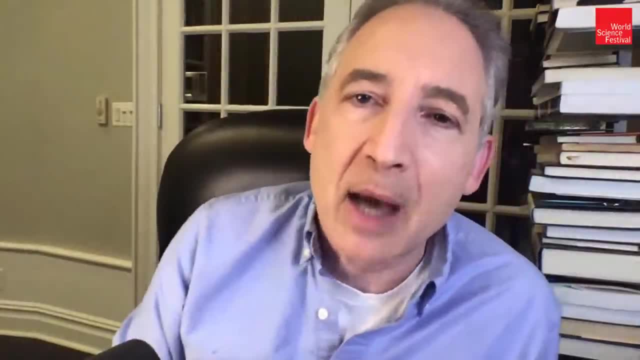 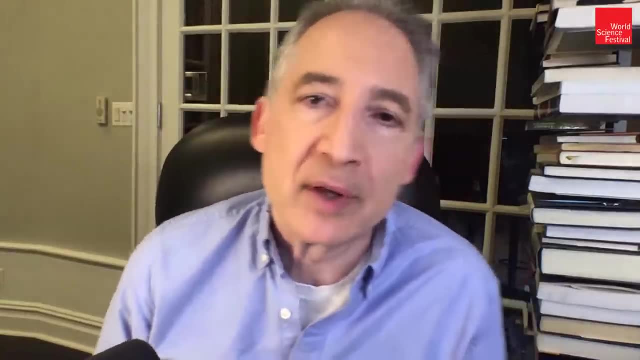 And that, unfortunately, is not something that we can do with God. That doesn't mean that God is wrong. It just means that the barometer by which you measure your beliefs are quite different in the two fields: In cosmology, in science. 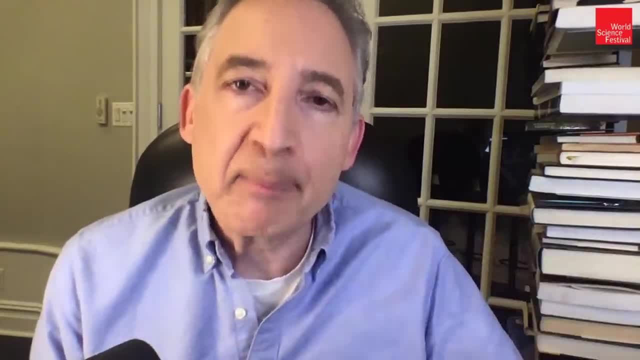 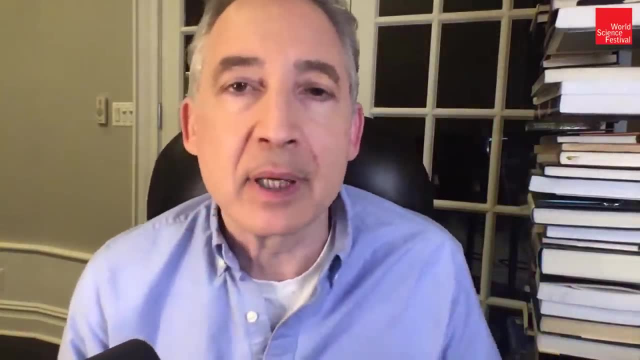 we use a barometer of predictive power of your ideas to match observations. In a theological setting, people can use a different barometer. They can use a barometer of. does it help me make sense of my life? And if it does, 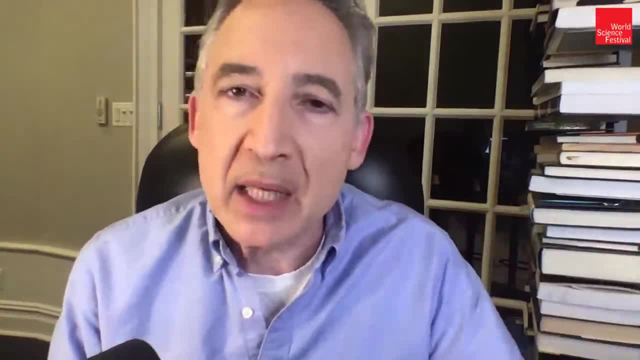 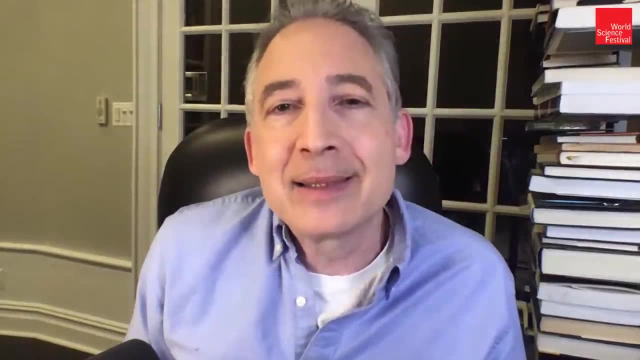 fantastic. Does it give me some sense of meaning and purpose? Yeah, for some, God is able to do that, and the laws of quantum mechanics are not able to do that. So it's not that they're really in competition with each other. 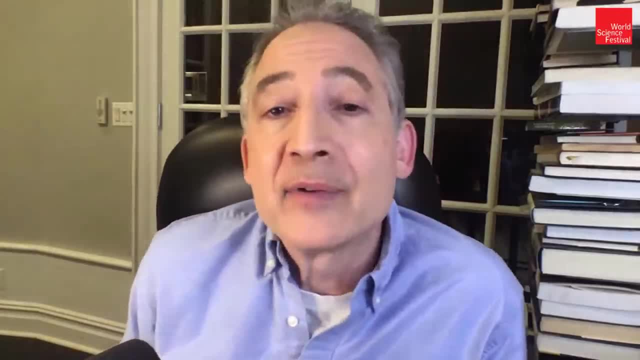 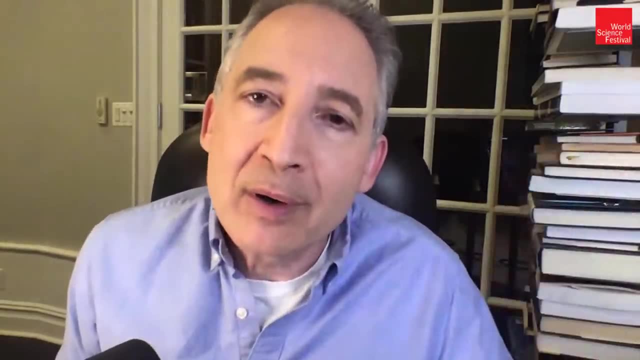 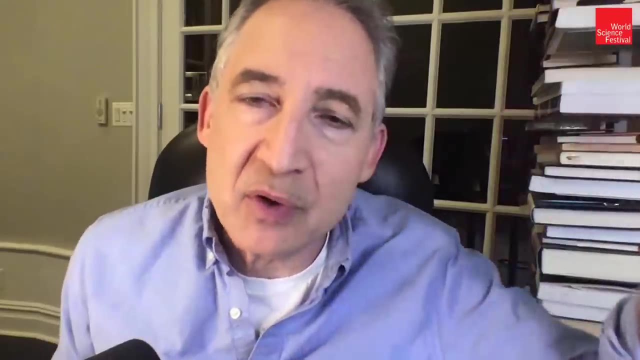 John, I wouldn't frame it the way that you did. personally, I would frame it that there are distinct stories that we tell about the universe for different purposes. For the story that aims to understand the microwave background radiation and the evolution of the cosmos and the far future of the cosmos: 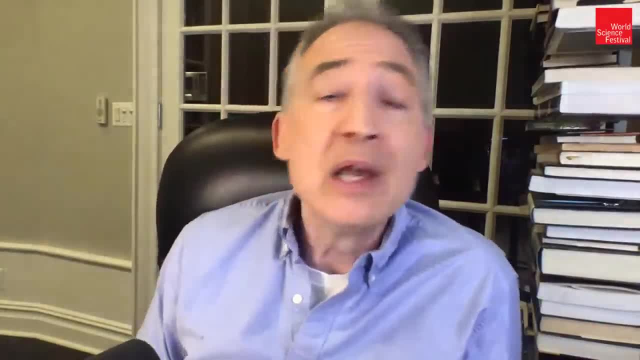 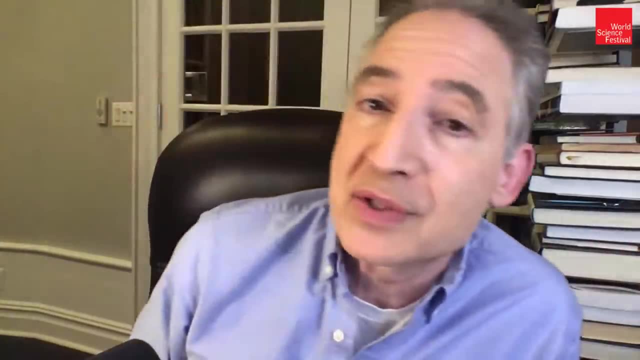 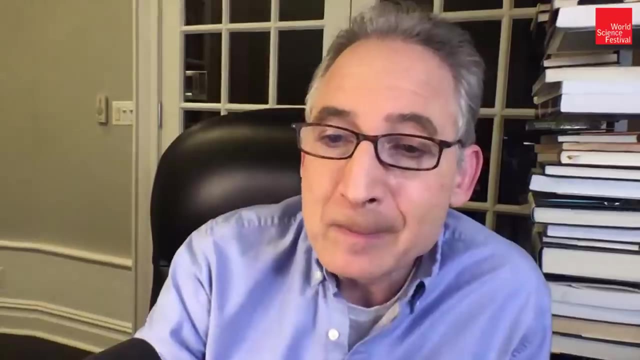 yeah, that scientific story is pretty good For another story that tries to give us some sense of purpose and meaning. the theological story for some does a very good job in that domain And those stories need not be at each other's throats. 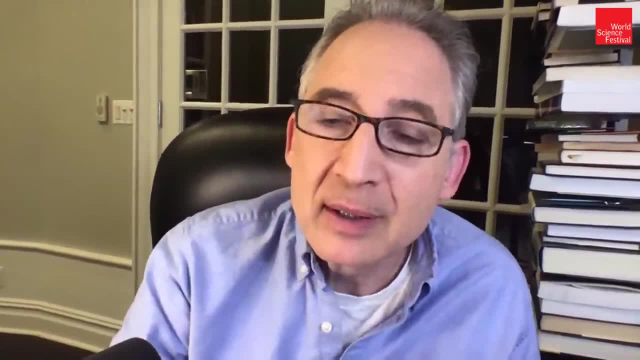 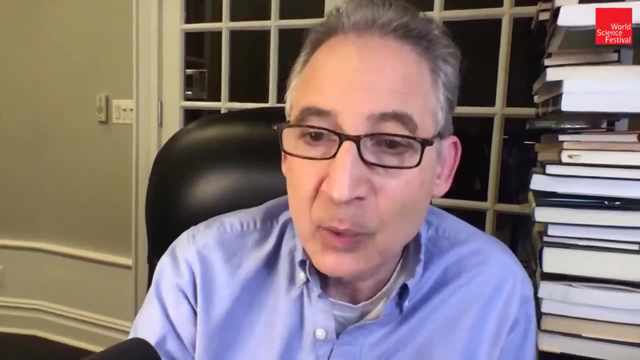 Those stories can just be viewed as parallel accounts that play a different role in our attempt to understand who we are, how we got here and what the universe within which we find ourselves, what that universe is. All right, maybe one or two. 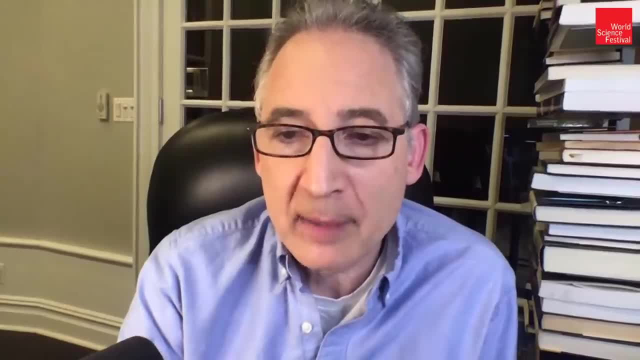 Oh, I see, So I'm going to go to the next slide. So this is a question from Vanessa. She asks: why did you stop your daily equation? I stopped your daily equation because it was a lot of work, I mean. 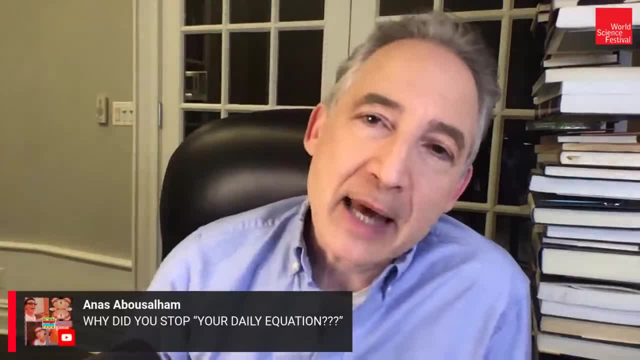 it may not have seemed like a lot of work, but you know every single day to sit down and try to think up. okay, what's today's equation? How am I going to explain it? You got to film it. You got to put a little visual in it. 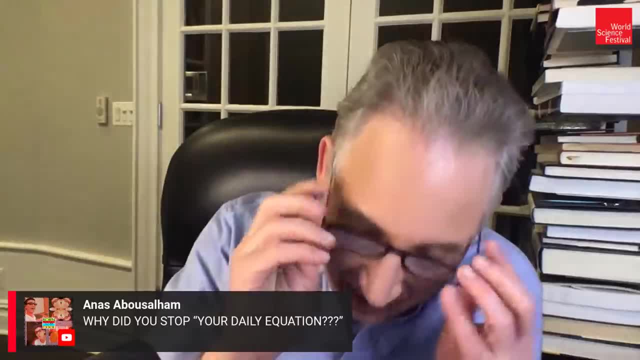 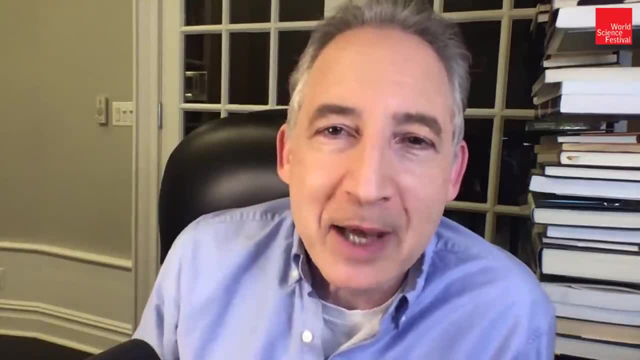 You got to write out the equations and so forth. It just became. you know, it's like many people. they have a diary right And they keep their diary for, I don't know, a couple of weeks, a couple months. 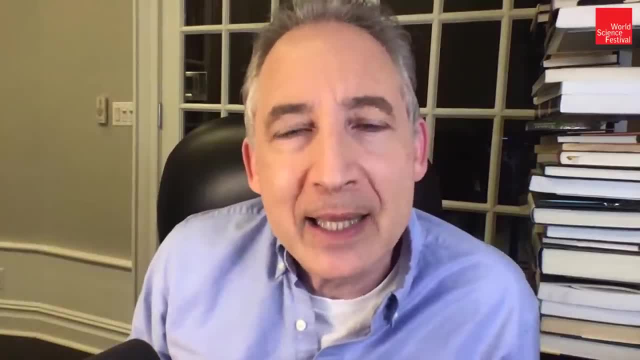 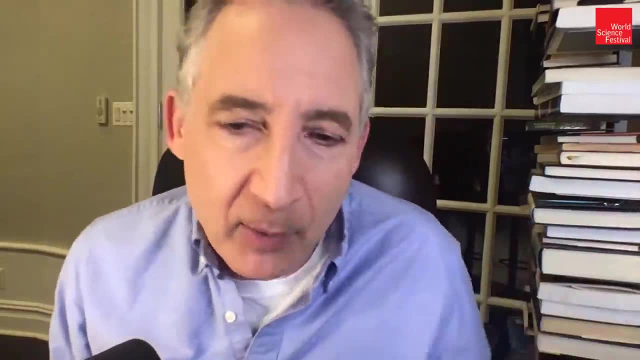 They keep it forever, but very few. Why? Because every day writing in that diary, it becomes a burden, right, It becomes a chore, becomes something that you do instead of the other things that you might want to do in your life. 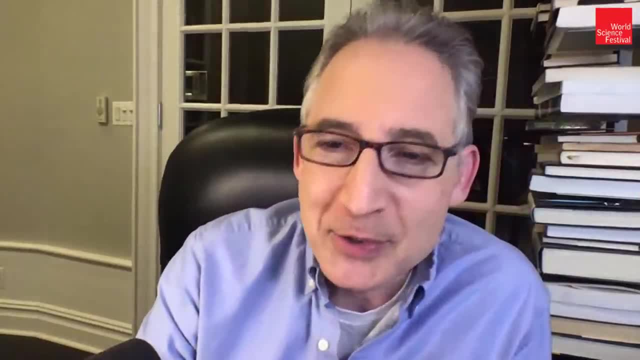 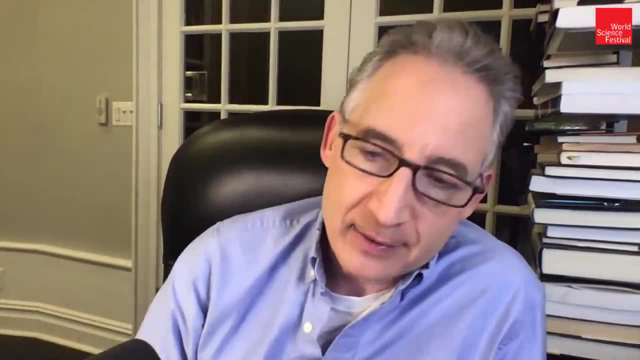 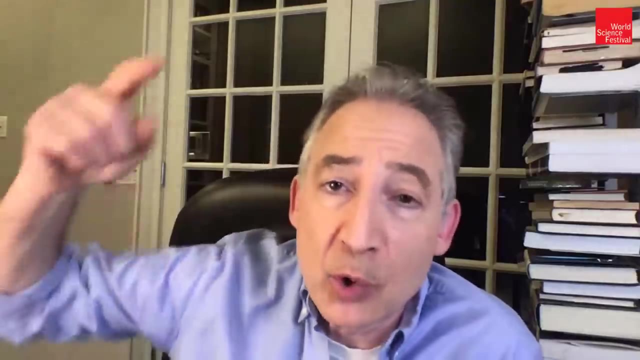 And that's certainly what happened with your daily equations. So that was what led us to shift over to these kinds of conversations, And I should note that we are getting to a place soon where the World Science Festival, New York. I mentioned World Science Festival. 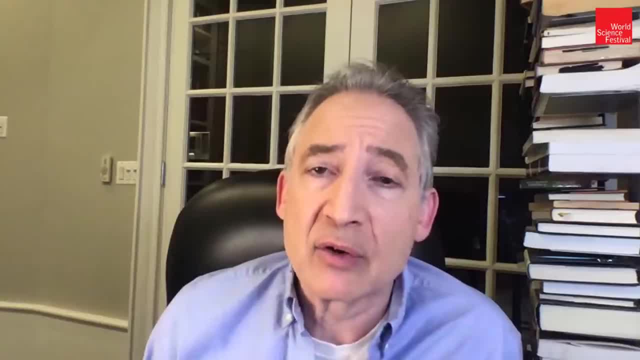 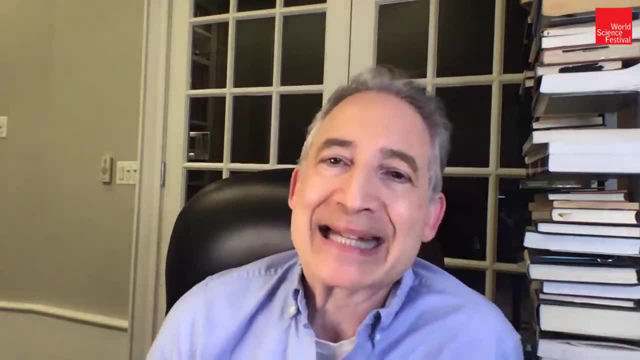 Brisbane. that's happening right now And again for you guys in Australia. you know you should, you know, get up to Brisbane. If you're not there, partake of the weekend's activities. that are going to be a lot of youth and family events. 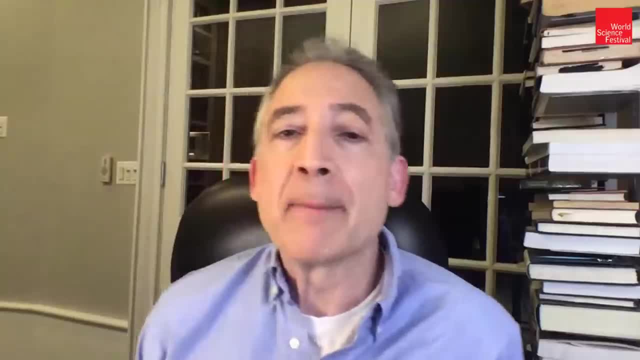 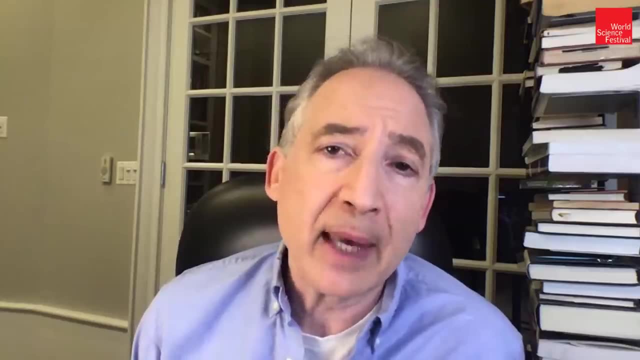 really a good time up there in Brisbane, So you should feel free to do that. But World Science Festival New York will be kicking into gear in a digital online way toward the end of May, early June, So there'll be all sorts of programs that will be far. 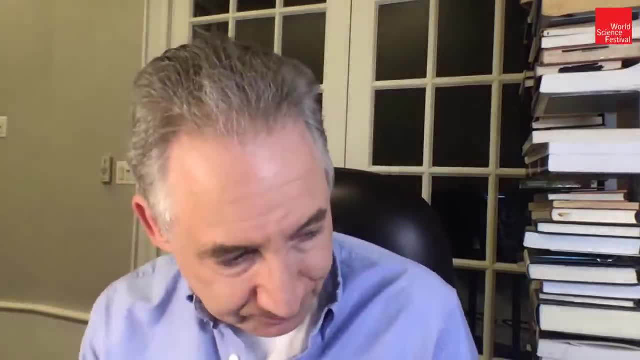 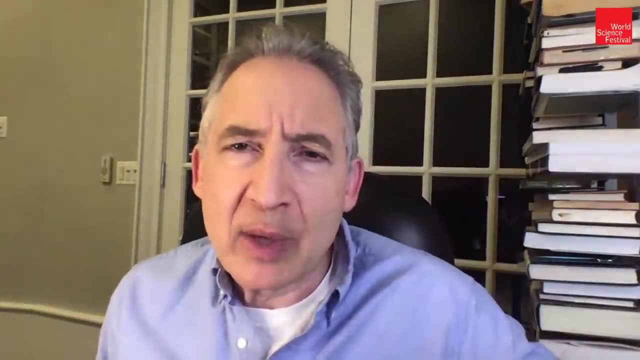 far more produced than your daily equation. talking about all sorts of subjects, I'm going to be doing a program on the relationship between math and reality. We had a little bit of that conversation with Brian Schmidt- but I'm going to be in conversation with a handful of other people. 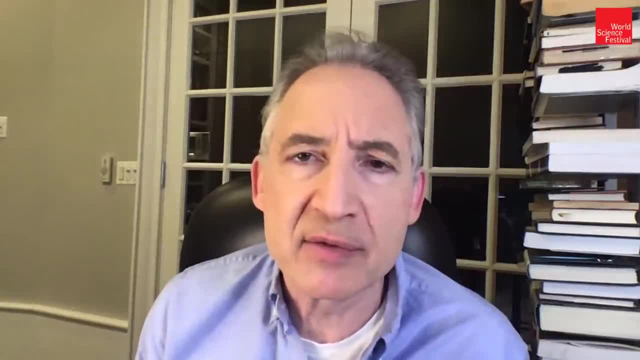 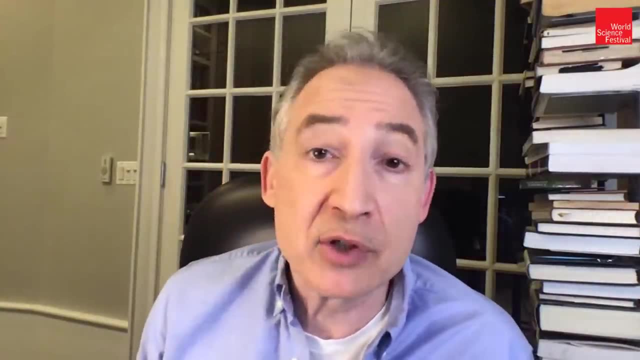 Philosopher, David Albert, mathematician, physicist, philosopher, Shelly Goldstein, a couple of other. Max Tegmark will be in that program. Sylvia Jonas will be in that program as well. May also do a program on a book. 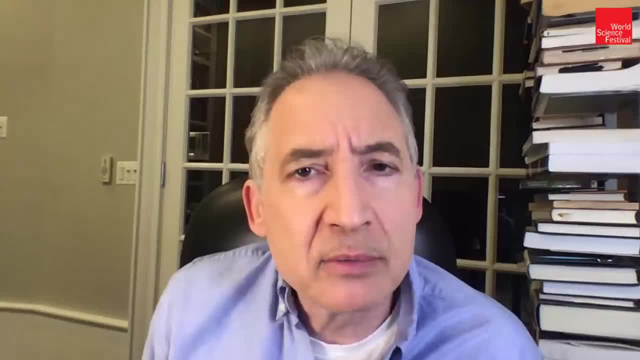 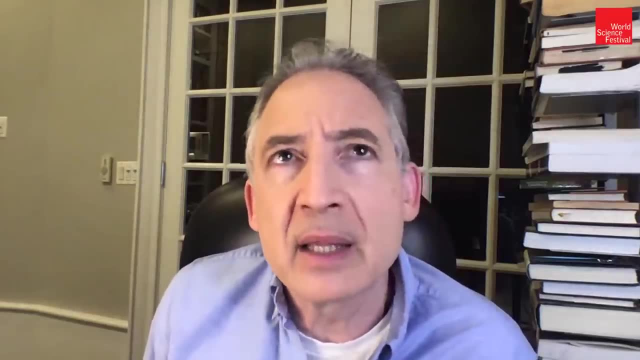 recent book that I wrote until the end of time. We're thinking of making a sort of stage, digital stage version of that, making that available during World Science Festival New York. Anyway, these are all plans in the making, but there's a lot of stuff. 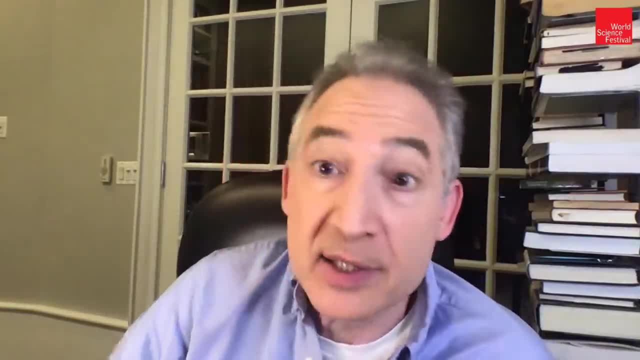 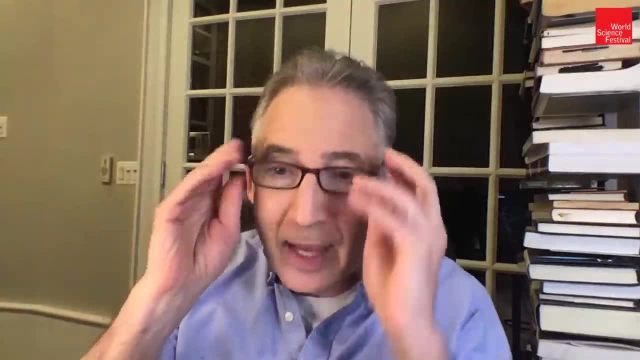 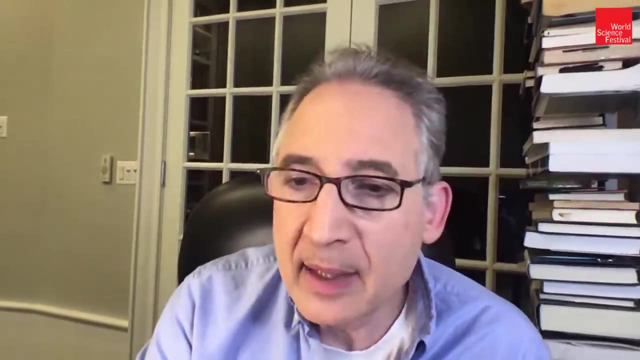 So you should keep your eyes out and you will not miss your daily equation One single bit. When all of that program starts, programming, starts to be released as soon as possible. So I'm looking forward to that. So I hope that this program starts to be released as we go forward. 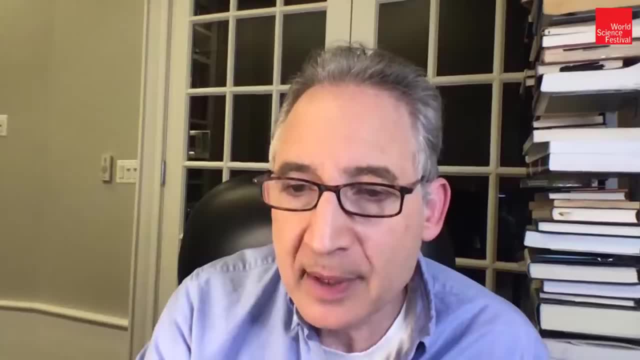 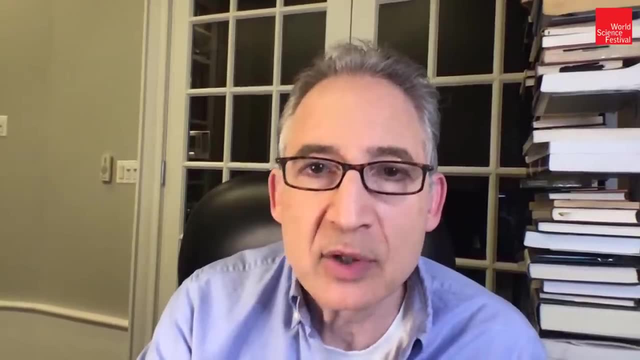 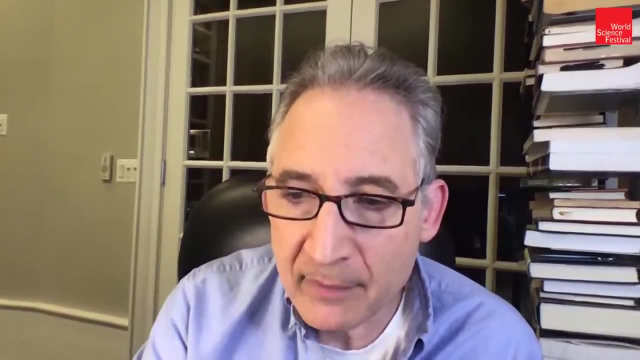 Okay, Anything else that I should talk about before we wrap this up? Let's see Canon. Carol says he is too smart. I guess you're talking about Brian Schmidt, sadly not me, but okay, no problem. What do we have here? 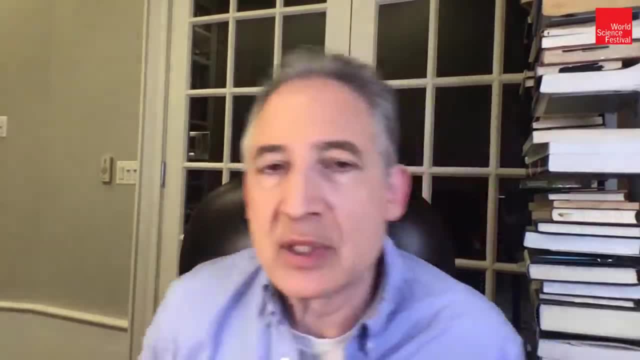 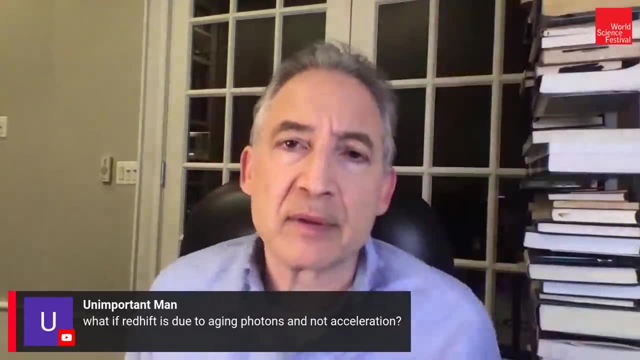 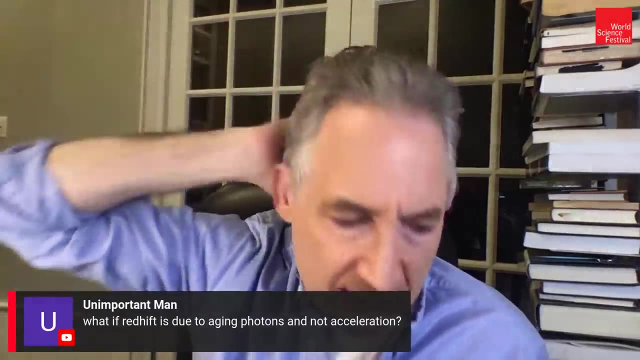 Oh, unimportant. man asks: what if the redshift is due to aging photons and not acceleration, an idea that that people floated or continued to float from time to time? we use the red shift, as brian schmidt was talking about, to understand the motion of of distant galaxies, and the idea is: 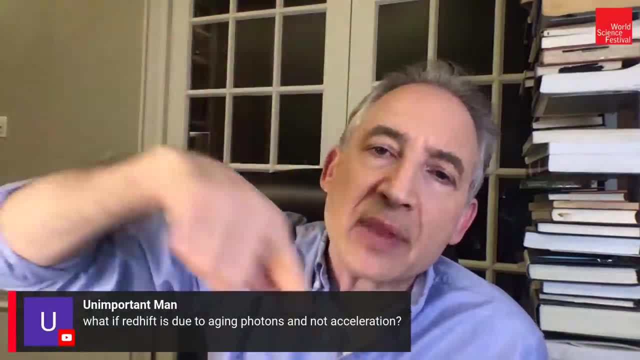 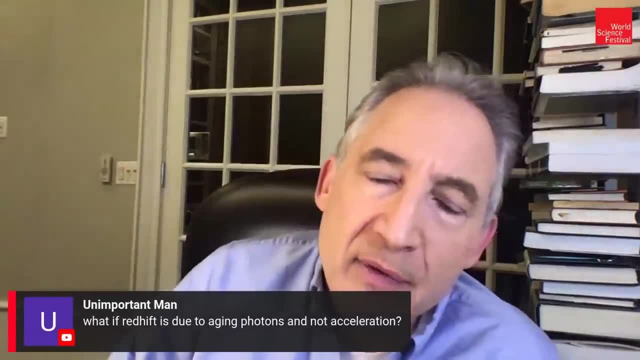 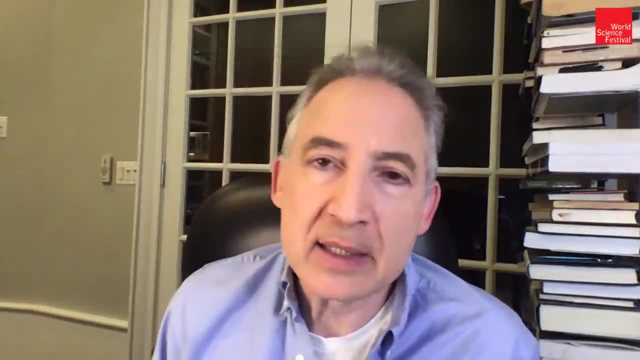 if distant galaxies are rushing away from us, the light that they emit gets stretched out by the cosmic expansion and root as a photon is traveling en route to us, and that, we believe, is the explanation of why it is that the light is shifted toward the red. others said: well, maybe. 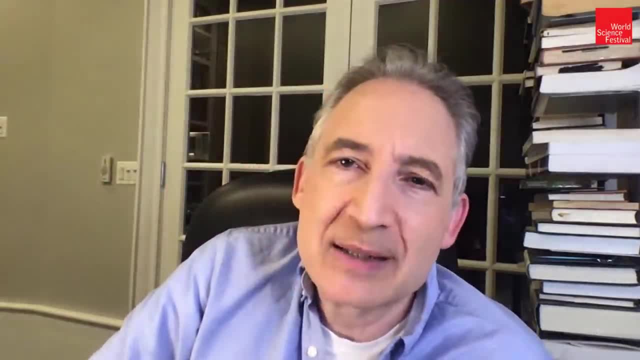 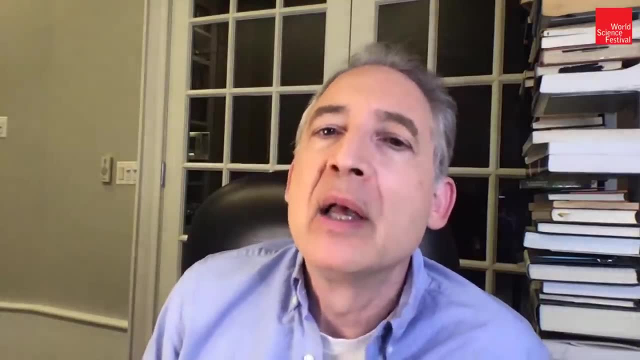 that's not what's going on. maybe you know the photons just get tired. they just kind of lose energy in some sense. even that's compatible with the explanation i just gave. but some tried to argue that you don't need the expansion of the universe, you don't need distant objects to be. 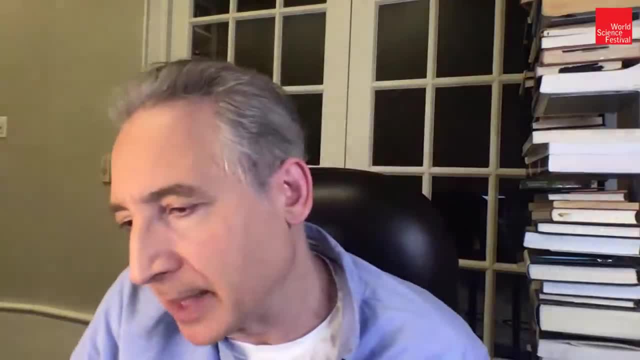 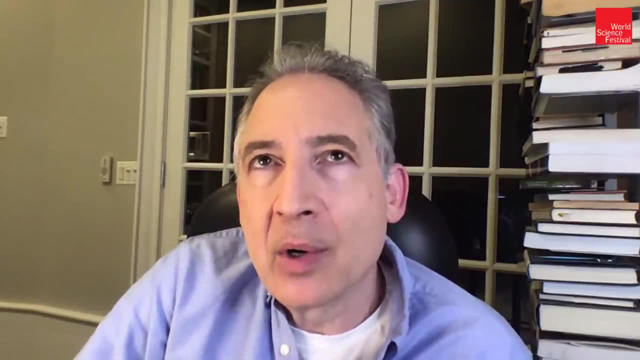 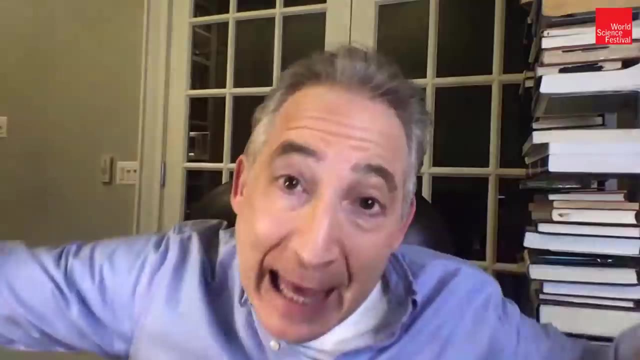 rushing away from us and a point that brian schmidt made is really worth bringing up in answer to this question, which is we don't base our conclusions about the expansion of the universe, the accelerated expansion of the universe, the flatness of the geometry of space. we don't. 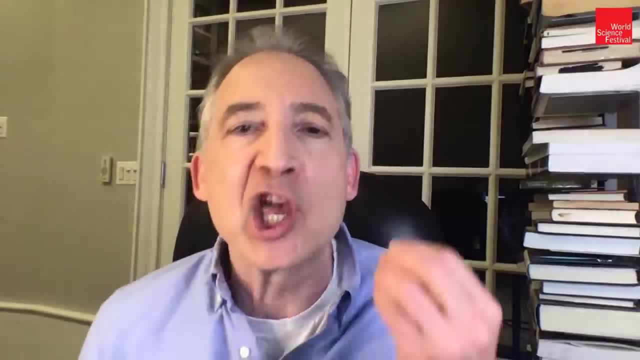 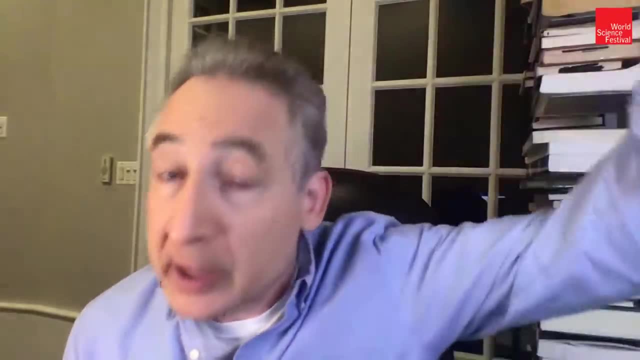 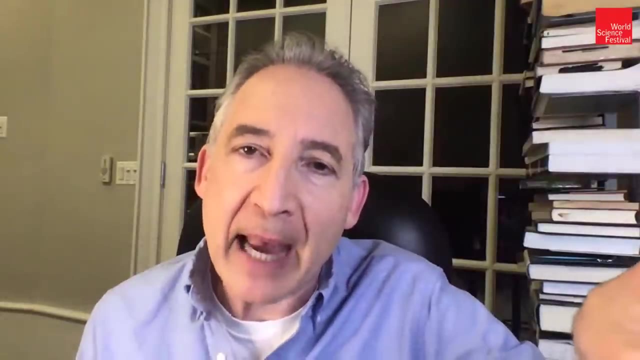 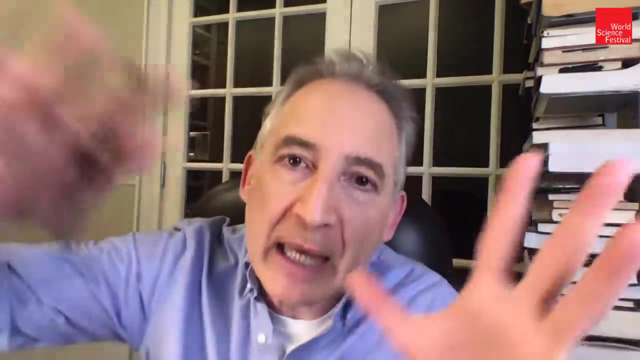 base that on one observation. we base it on a concordance of a whole variety of observations that have to do with looking at the distant objects, looking at the size of the temperature microwave background radiation, looking at the theoretical structures that can explain these qualities of the world, looking at the baryon acoustic oscillations that give rise to a very 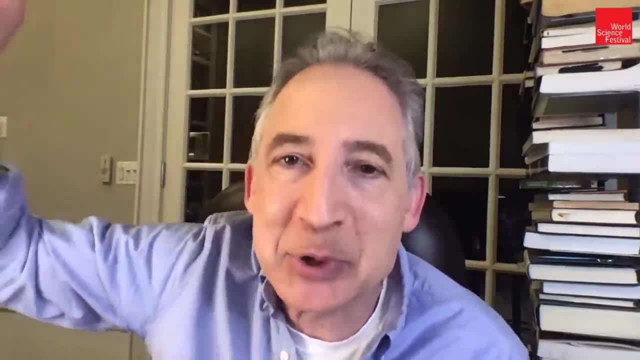 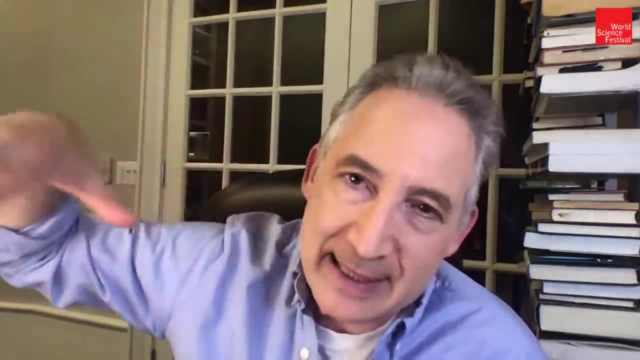 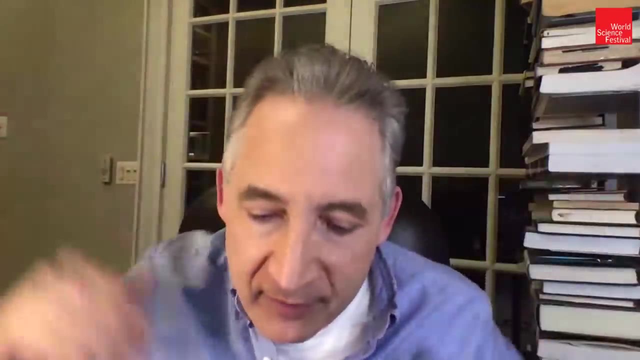 precise statistical variation of the temperature in the microwave part of the spectrum. and it's by collecting all of this data and finding a model that's able to explain the intricacies of all of these observations that we are led to the picture that we espouse, this idea of an expanding 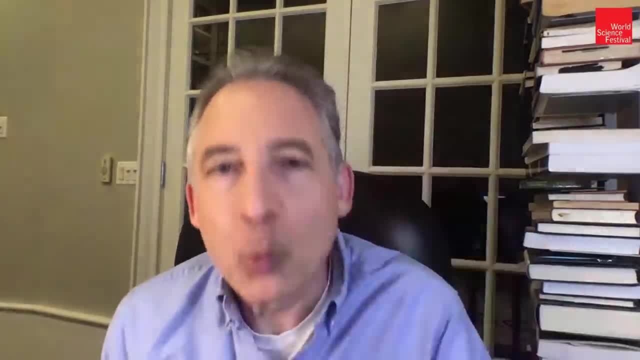 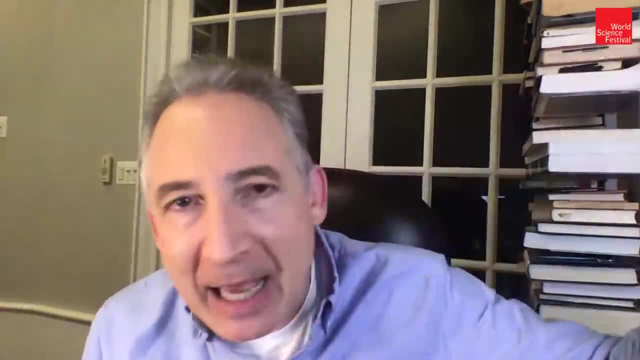 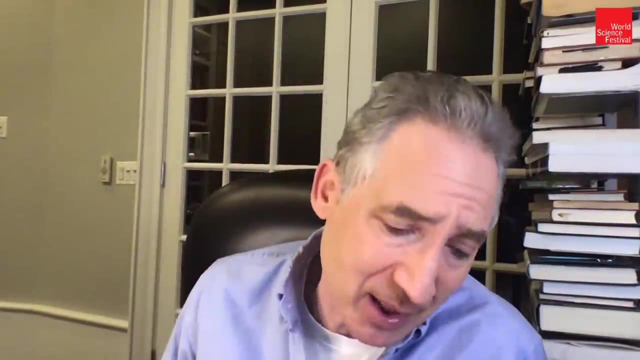 universe and accelerating, expanding universe. so it's not, it's not one observation which perhaps you may find some way of shaking confidence in that. it's many observations, many distinct and complementary observations that all come together to yield our most refined cosmological story, and so that's why we have confidence. 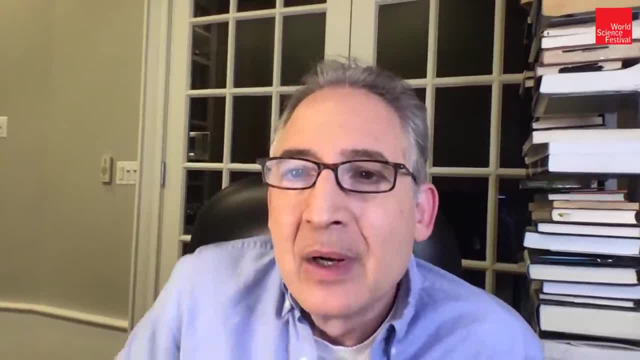 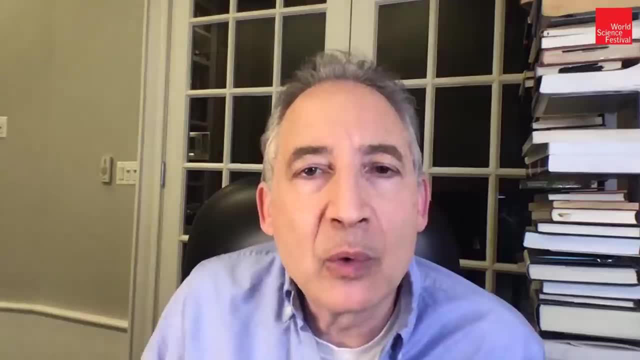 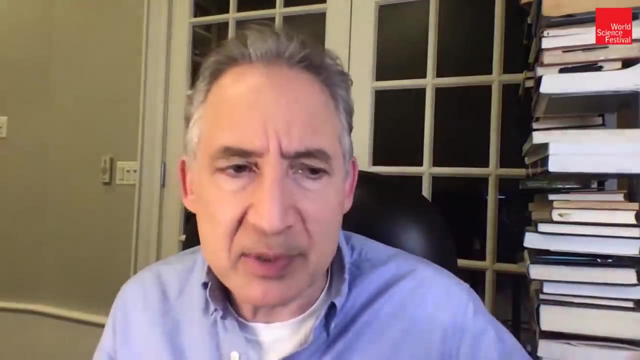 in that it all holds together. all right, i think i'm gonna wrap it up now, guys. um, so keep your eyes out for another one of these sessions, probably in a couple weeks. we took a little time off because of world science festival of brisbane happening right now. around the end of may, early june we'll 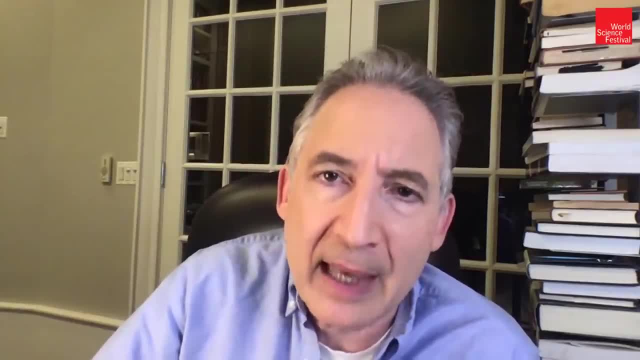 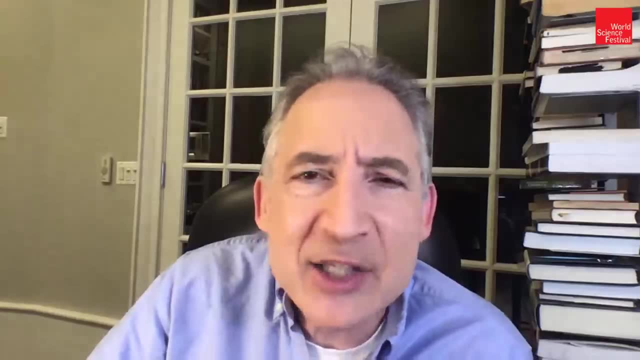 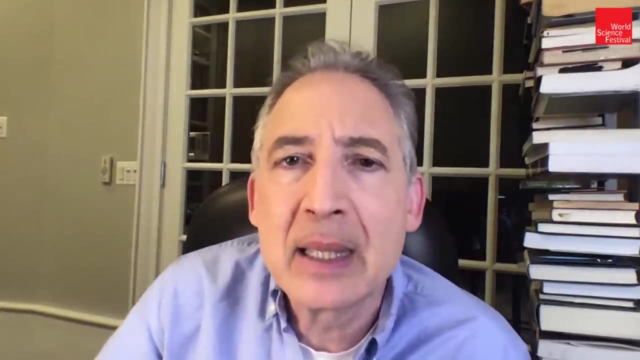 probably also take a break because we'll be focusing on getting the programming out for world science festival new york. mark your calendars: world science festival new york. i think we'll start wednesday, june 2nd. i could be wrong, but roughly the first wednesday after memorial day in the united states will be the launch of the digital version of world.